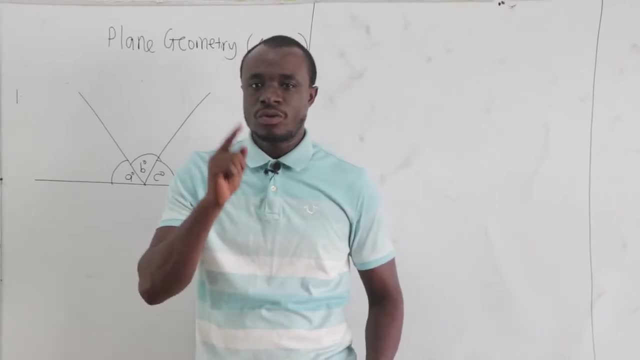 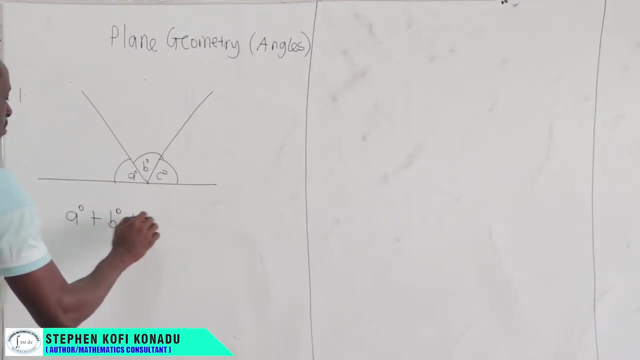 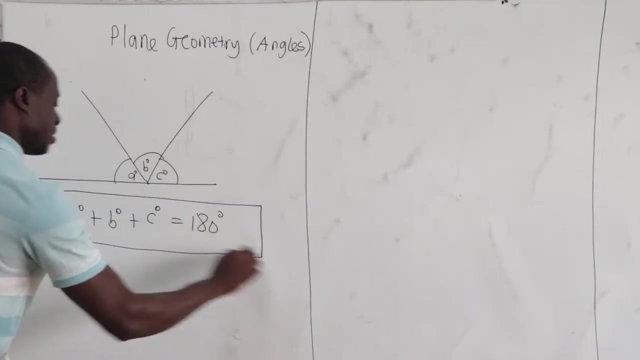 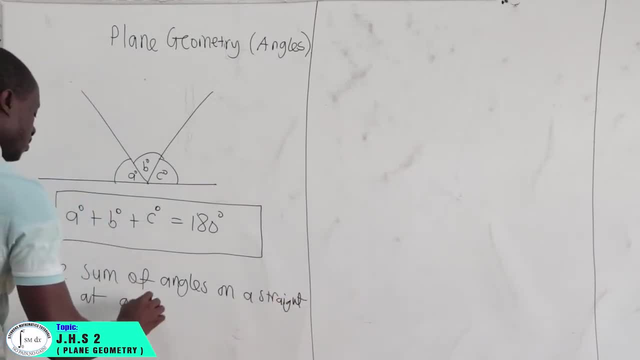 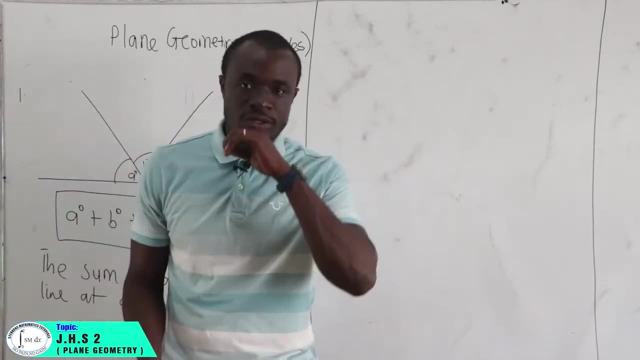 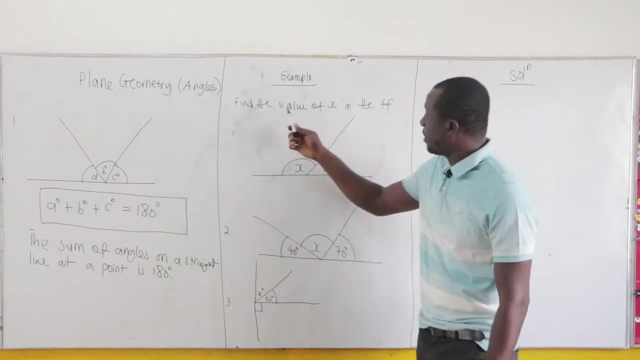 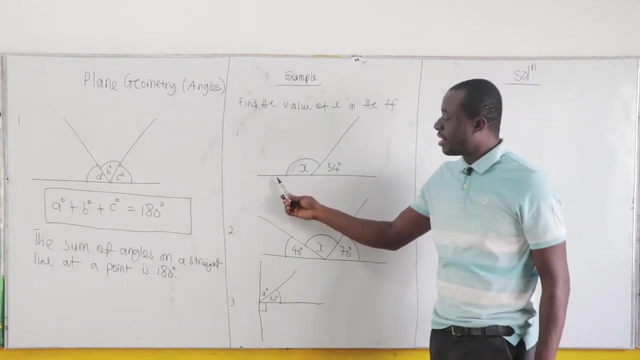 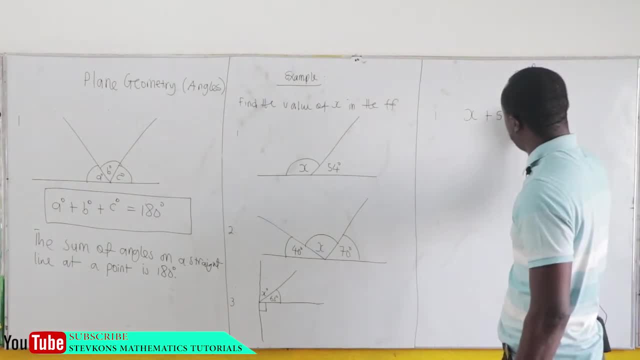 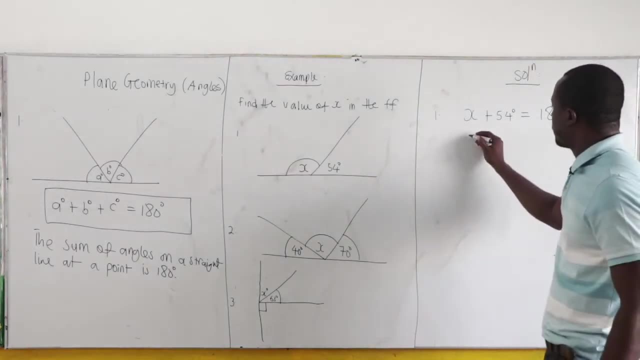 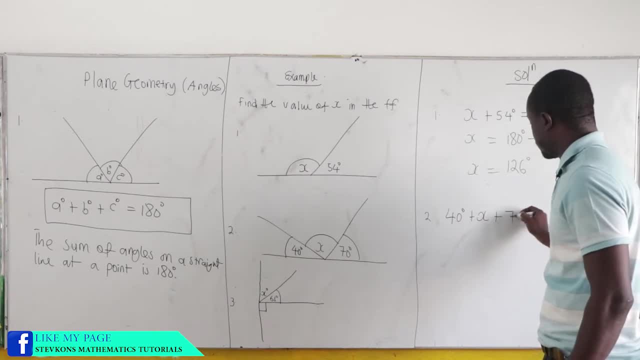 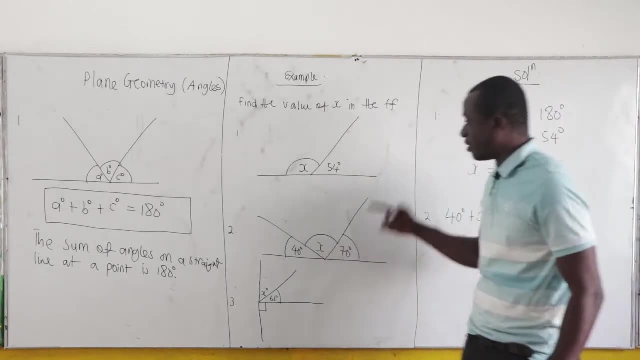 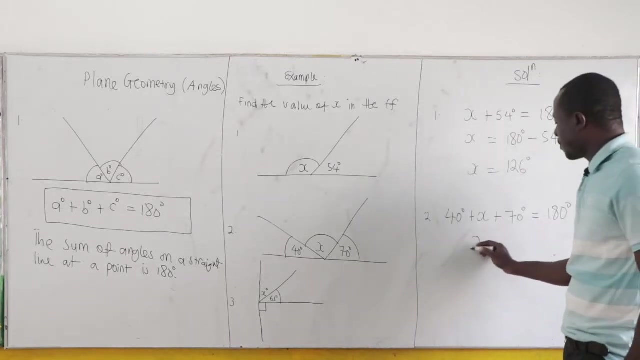 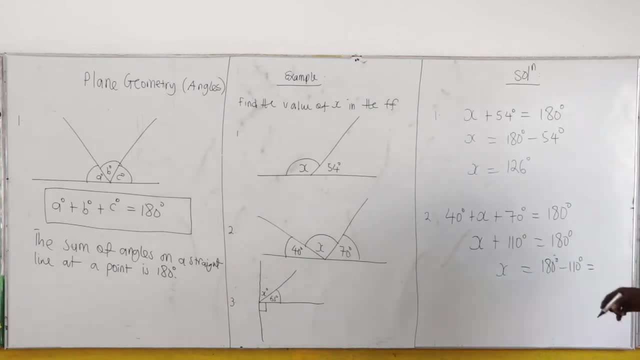 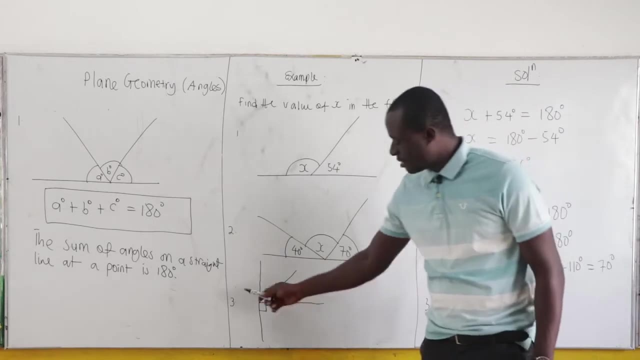 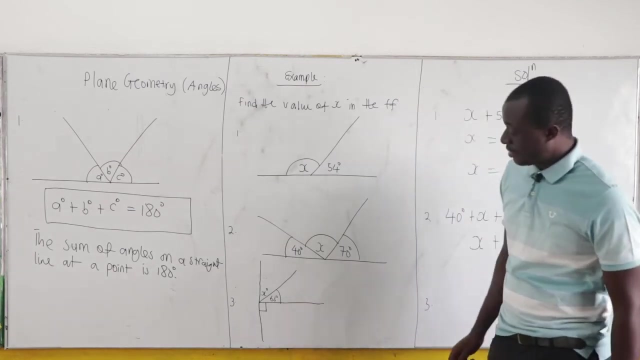 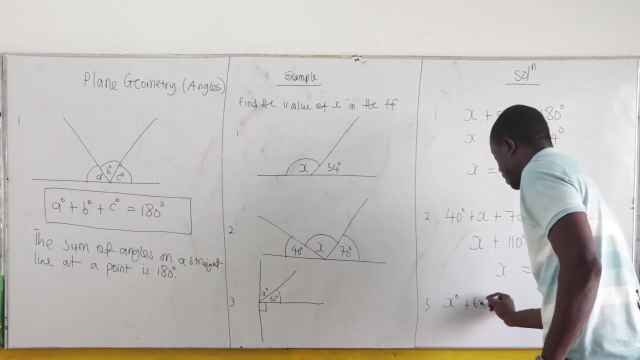 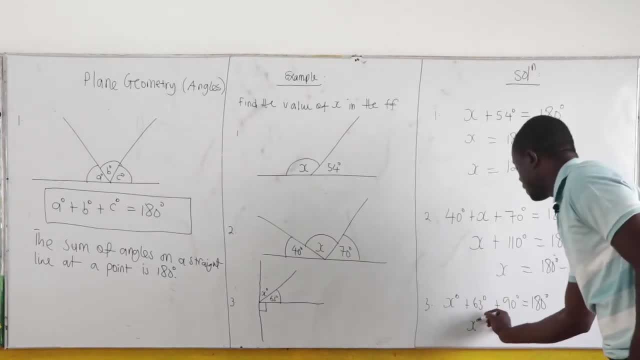 is A. So, if you have, let's suppose that we have a straight line and at this particular point, if this is A, the angle here is B and then the angle here is C. Now we are saying that the sum of angles on A is B and then the angle here is C. Now, if you have, let's suppose that we have a straight line and at this particular point, if this is A, 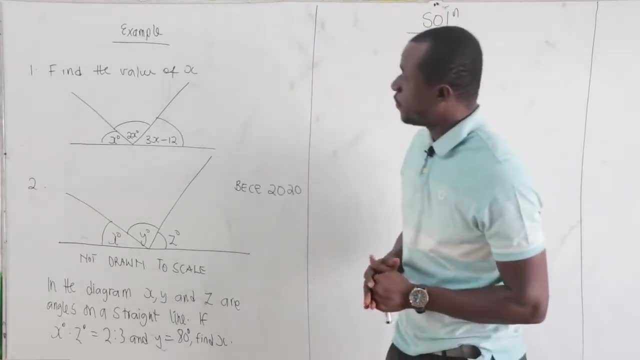 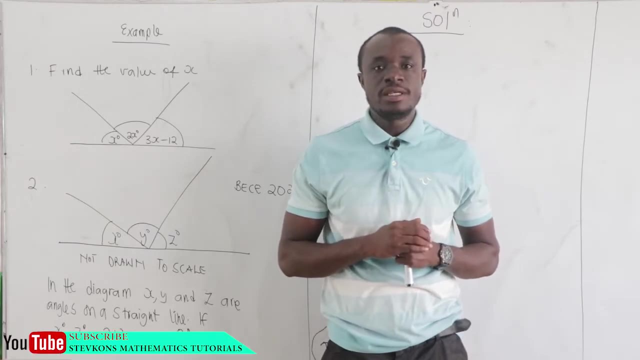 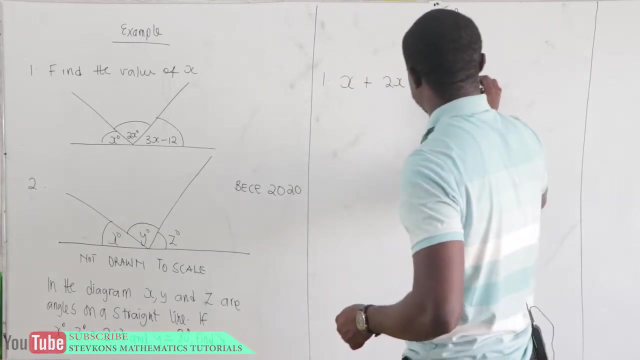 Now let's consider the following examples. The first one says: you find the value of x. Now we know that the sum of angles on a straight line at a point is equal to 180 degrees. Hence the first one. we have x plus 2x plus 3x minus 12.. 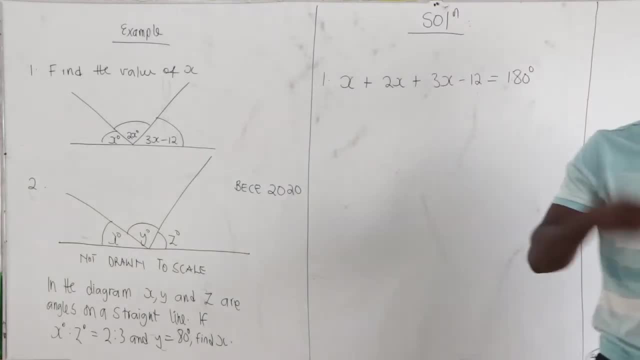 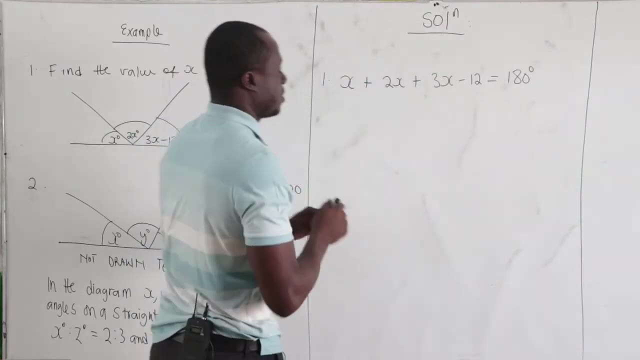 This is equal to 180 degrees. Why The sum of angles at a point is equal to 180 degrees. Now let's see x plus 2x plus 3x. This is given as 6x minus 12, equal to 180 degrees. 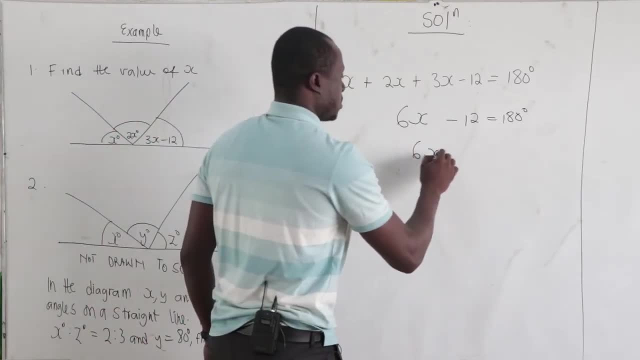 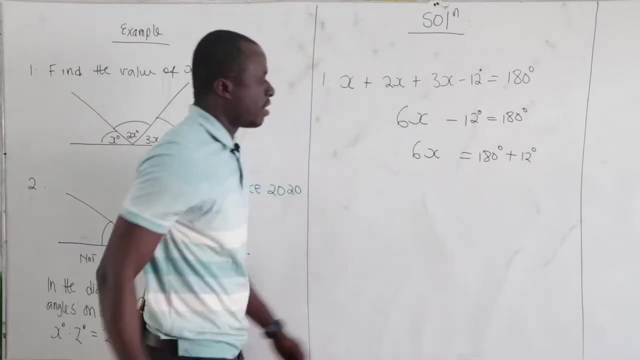 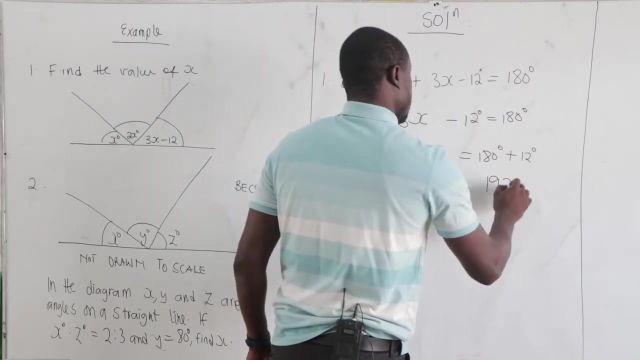 Now we have to group like this. So we have 6x, equal to 180 degrees, plus 12 degrees. Now let's see 180 plus 12.. This is giving us that is, 192 degrees. We want to find x. 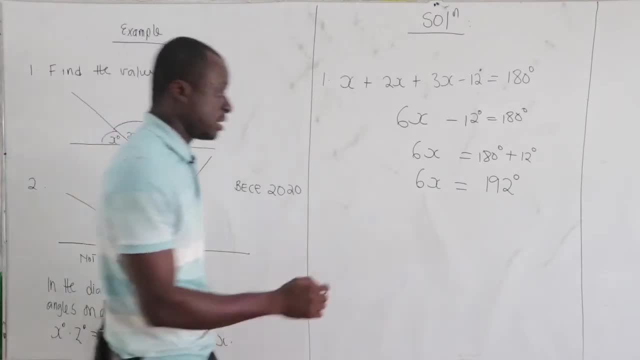 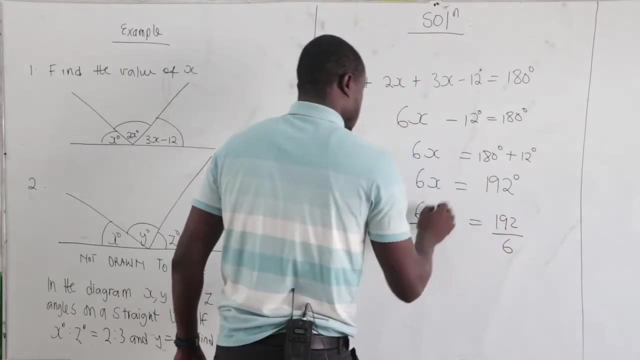 So we divide both sides by what is multiplying The x, which is 6.. So we have 6x all over 6 equals 192 all over 6.. This is canceling out that. Now, how many times does 6 go into 19?? 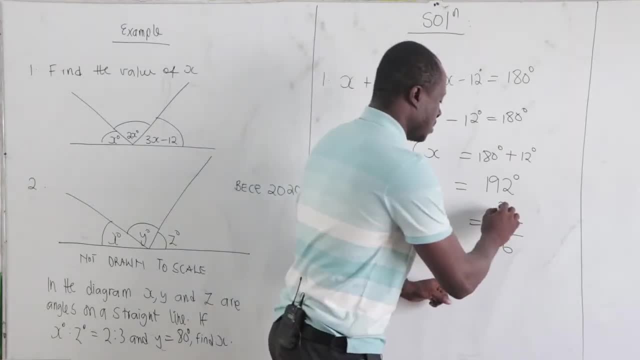 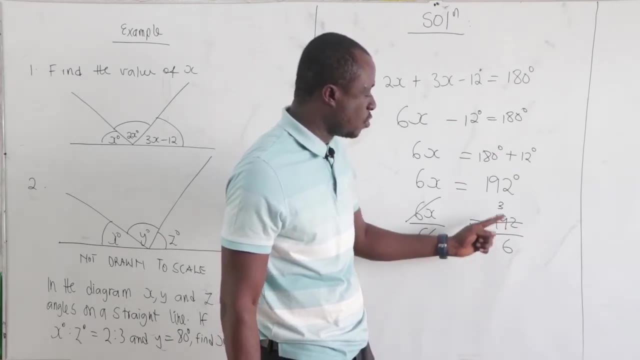 Since we go into 19, 3 times 3. Remember that: 1. We have to add the 1 to that will be 10 to 2. That's 12.. Since we go into 12, that is 2 times. 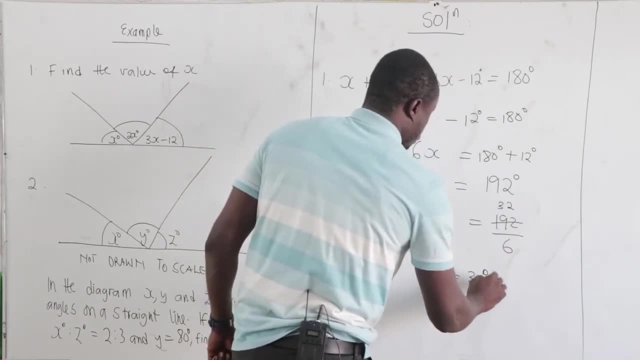 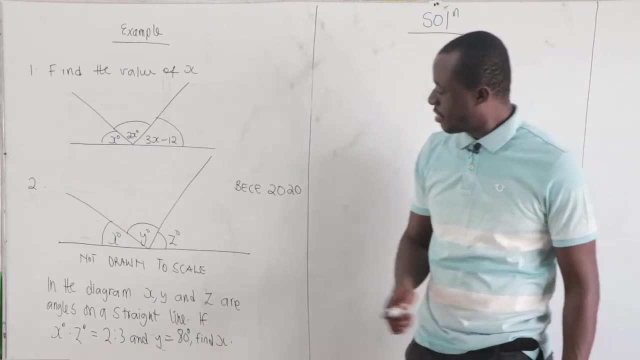 Hence our x is 32 degrees. Now let's consider the second question. The second question is a past question, which is BEC 2020.. Now we have this straight line. We are going to note down to scale. 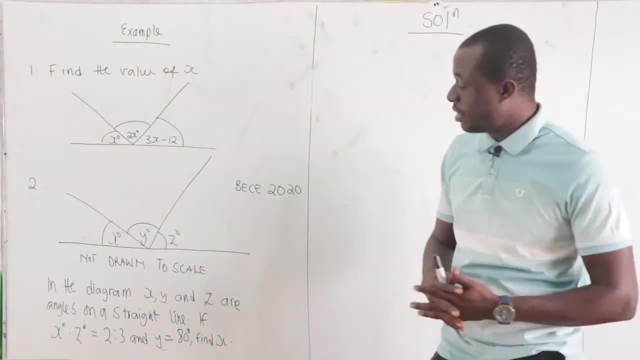 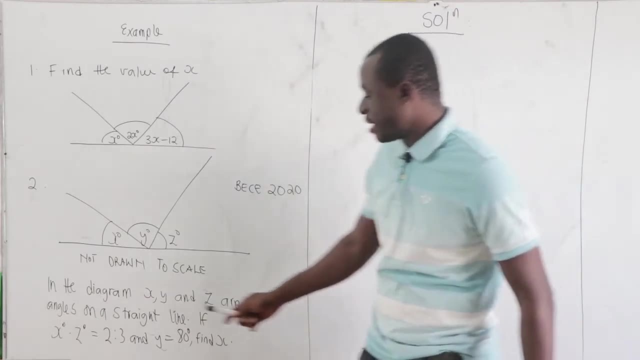 So x degrees plus y degrees plus z degrees is equal to 180.. Why Sum of angles on the straight line is equal to 180.. Now the reason is that in the diagram, x, y and z are angles on the straight line. 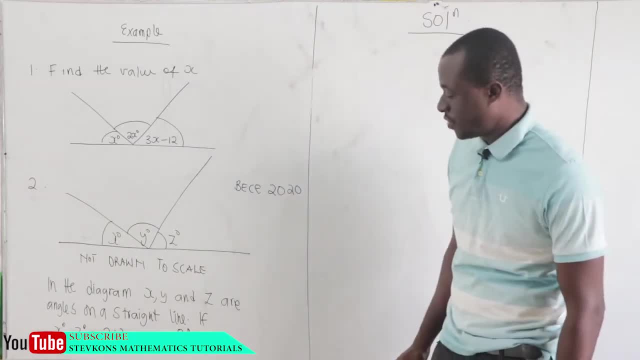 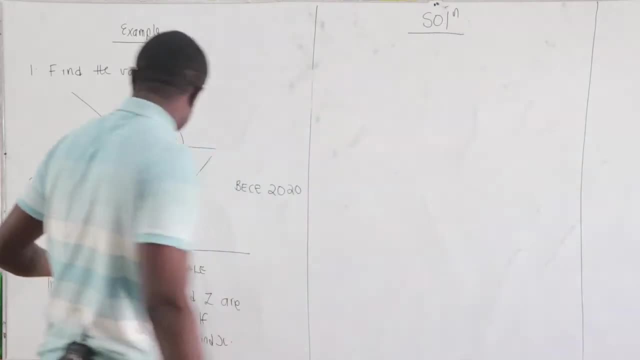 If x degrees is to z, degrees is equal to 2 is 3. And y is equal to 8.. We should find the value of x. Now what do we know? Sum of angles on the straight line at a point is equal to 180 degrees. 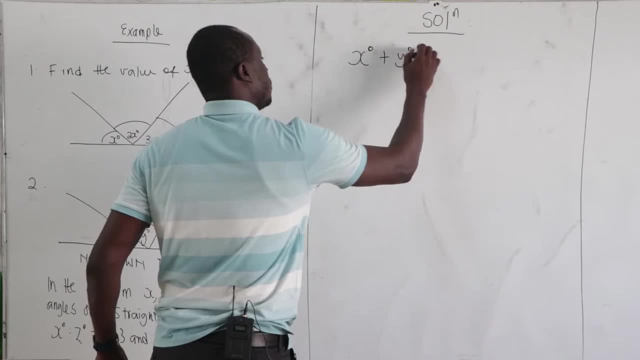 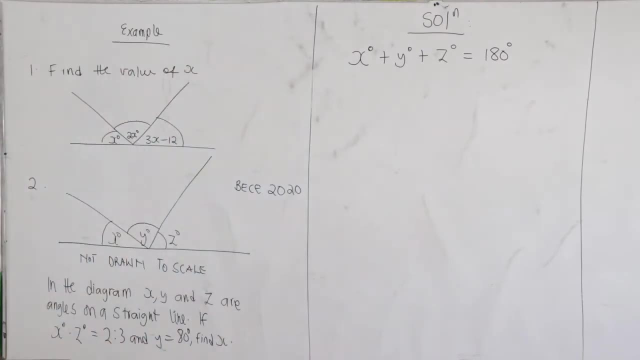 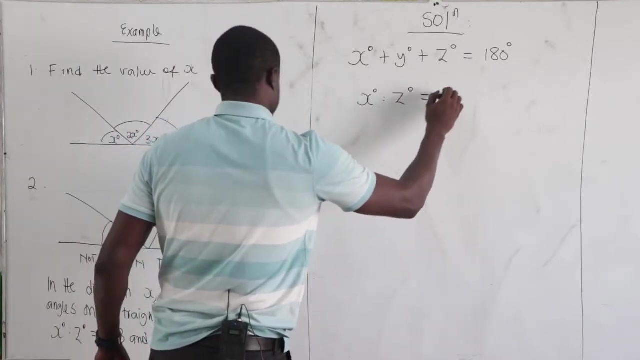 So basically, x degrees plus y degrees plus z degrees is equal to 180 degrees. Now, what were we given? We have been told that x degrees is to z degrees. This is equal to 2 is to 3. And this is just the same. 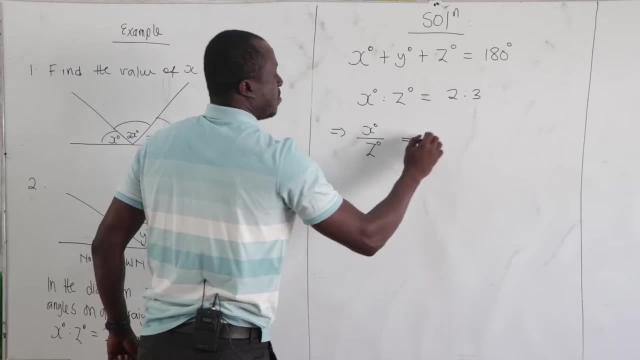 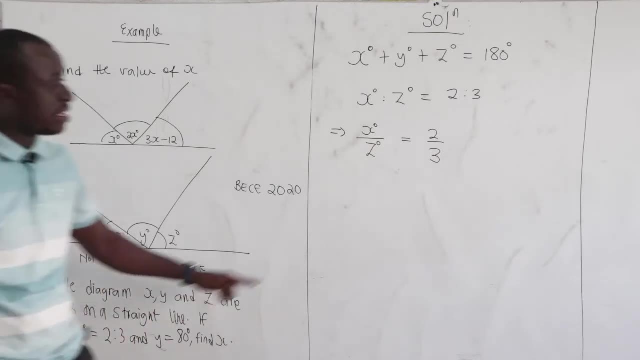 As x degrees over z degrees. This is the same as 2 all over 3.. Now the question is: we should find x, And because we want to find x, it is better we rather make z the subject and put it in the main equation. 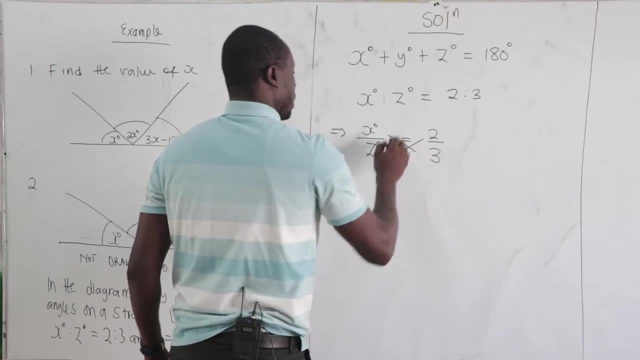 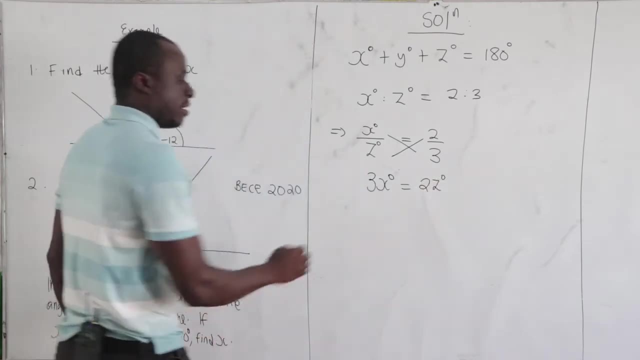 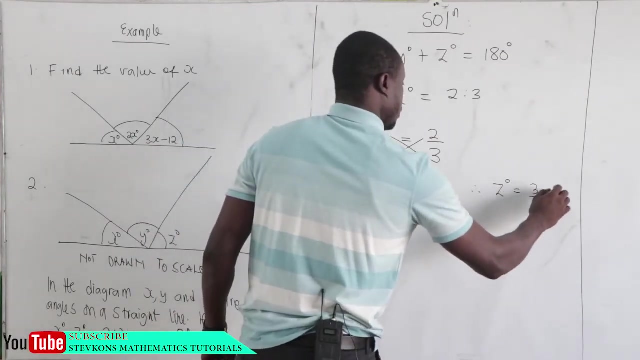 So clearly, let's cross multiply. So when we cross multiply we are going to get 3x degrees equal to 2z degrees. Hence z It is equal to, that is, 3 over 2x degrees. 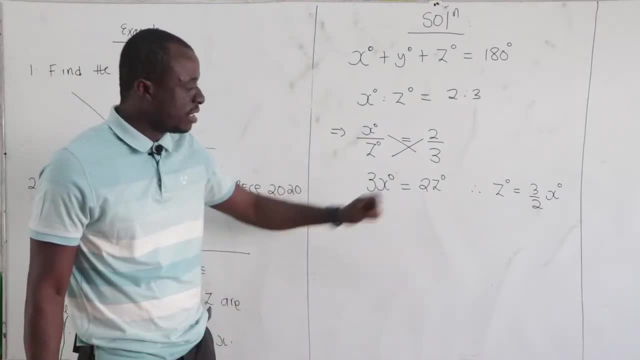 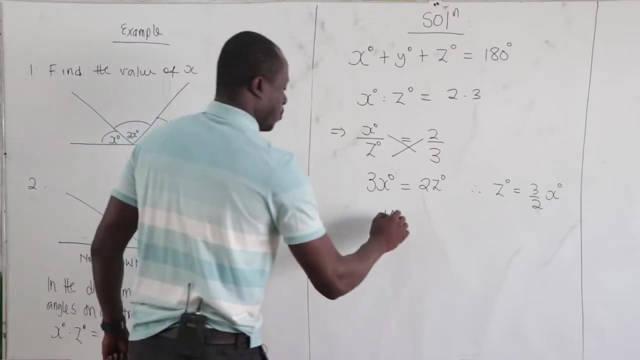 Why We want to make z the subject. What is multiplying it? That is 2.. So we divide it by 2.. Now, what again were we given? We are also given that y is 2.. We are given that y is 80.. 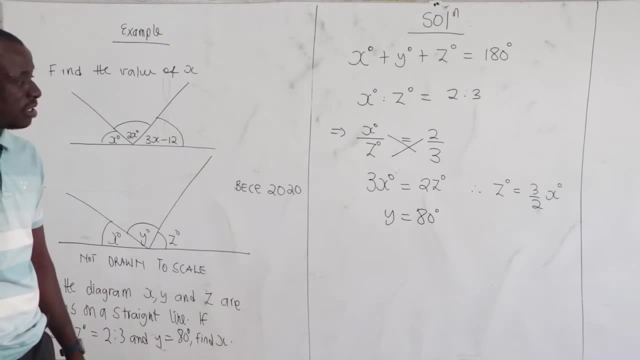 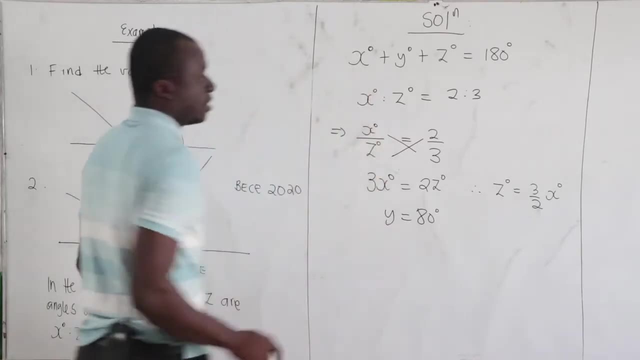 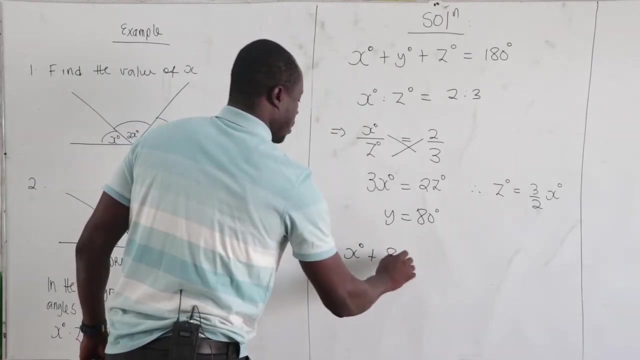 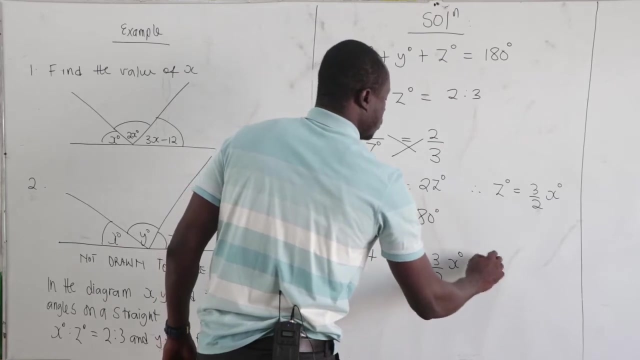 We are given that y is equal to 80. Now we substitute it. This is the main equation. So we have x degrees plus y degrees. What is y? 80 degrees plus z. What is z? 3 over 2x degrees, equal to 180 degrees. 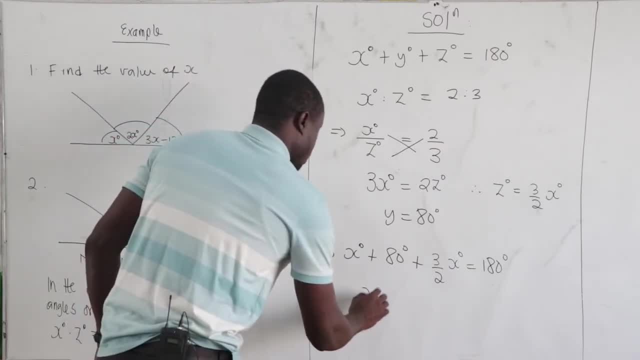 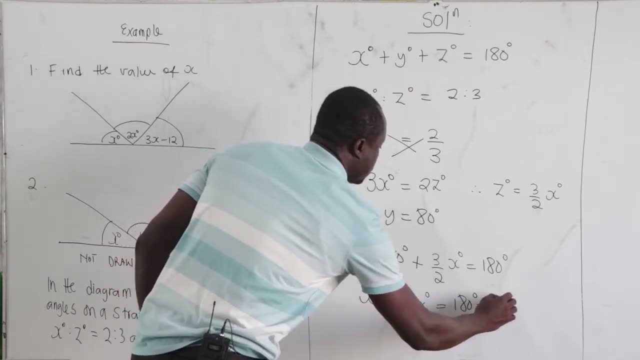 Now let's group like this: This can go to this side. So we have x degrees plus 3 over 2x degrees, equal to 180 degrees minus 80 degrees. Now, clearly from here. Now, clearly from here. 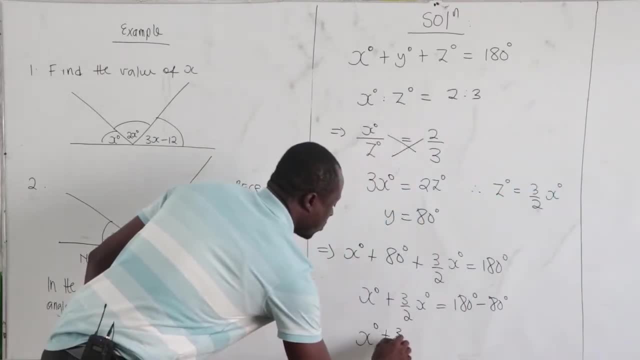 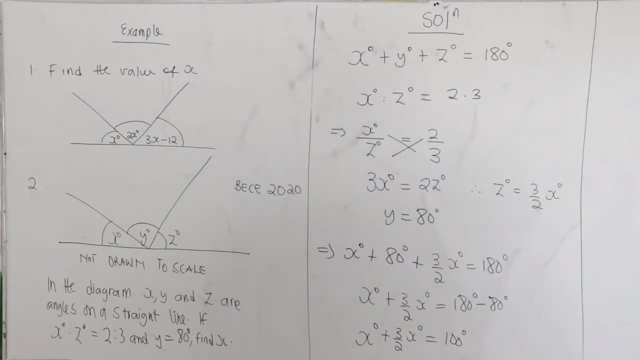 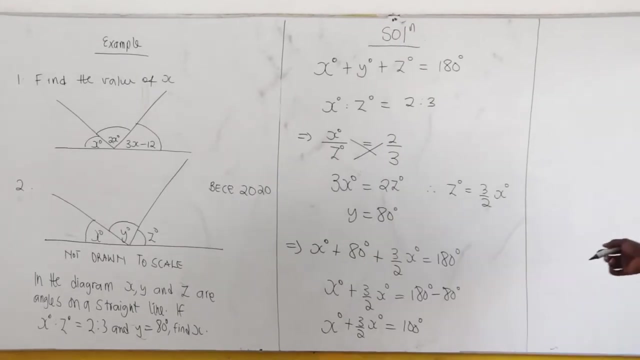 We have. that is x degrees plus 3 over 2x degrees, equal to 100 degrees: 180 minus 80.. That is 100 degrees. Now from here, what is the LCM? LCM is 2.. So we multiply both sides by each term by 2.. 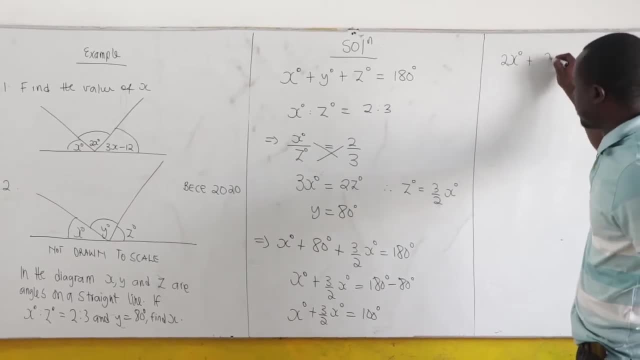 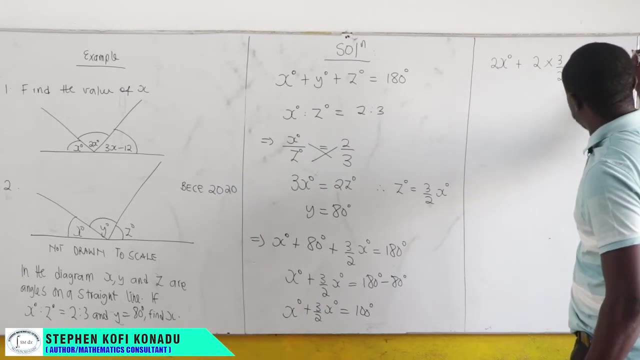 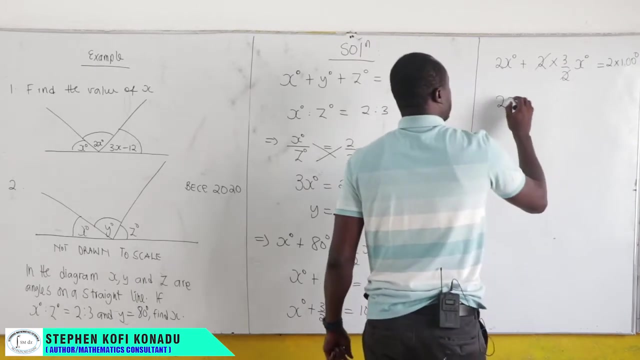 So we have 2x degrees plus 2 times 3 over 2x degrees, equal to 2 times 1.. That is 100 degrees. Now these two will cancel that too. So we have 2x degrees plus 3x degrees, equal to 200 degrees. 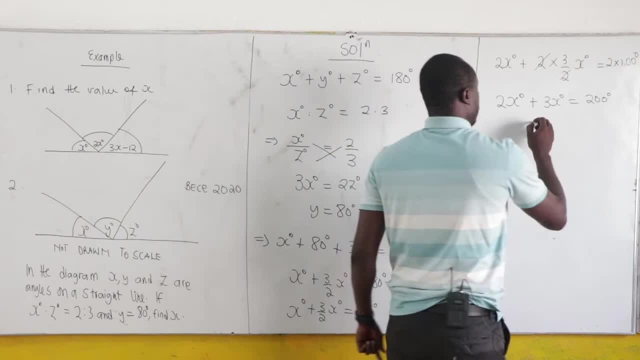 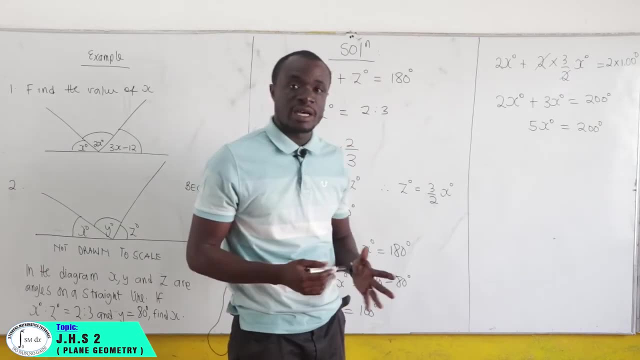 Now what is 2x plus 3x? We have 5x degrees equal to 200.. We want to find x, So we divide both sides by what is multiplying it, which is 5.. So 5x degrees all over 5.. 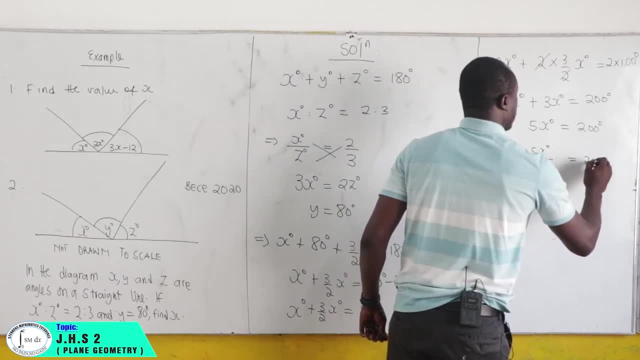 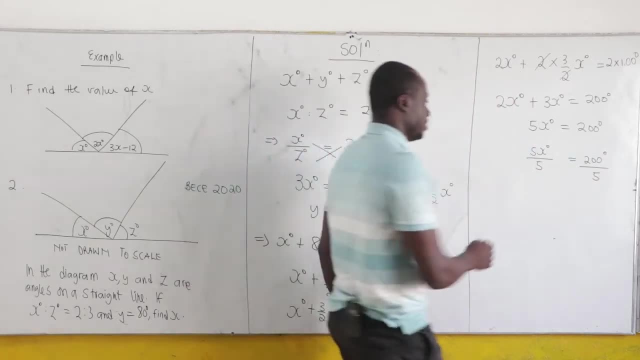 5x degrees all over 5, equal to 200 all over 5.. Now, how many times would 5 go into 100?? That is 40. So we have our x. This 5 is canceling out that 5.. 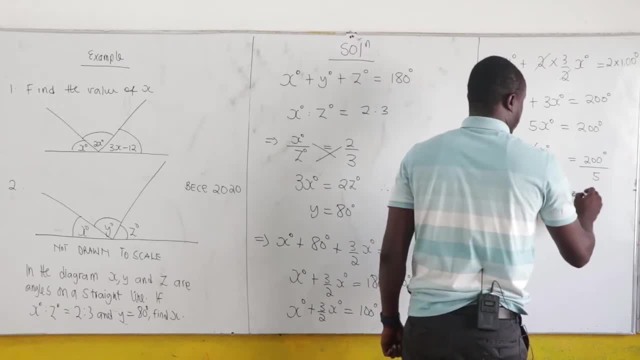 5 will go into 20.. That is 4.. 5 will go into 0. That is 0. So we have 40 degrees. So we have our x to be equal to 40 degrees. This is very, very trivial. 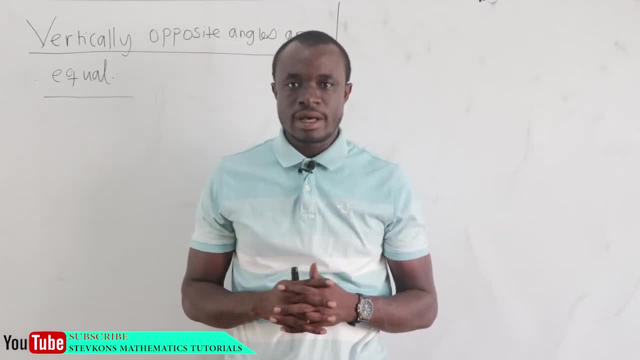 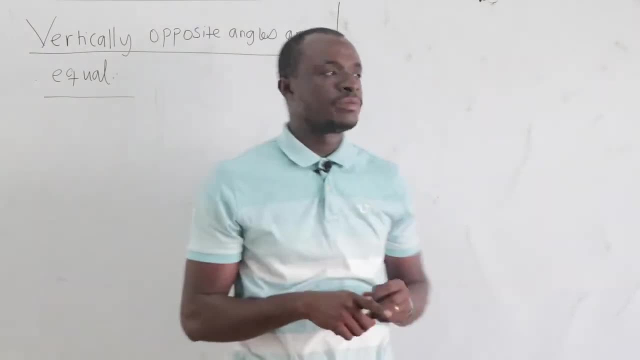 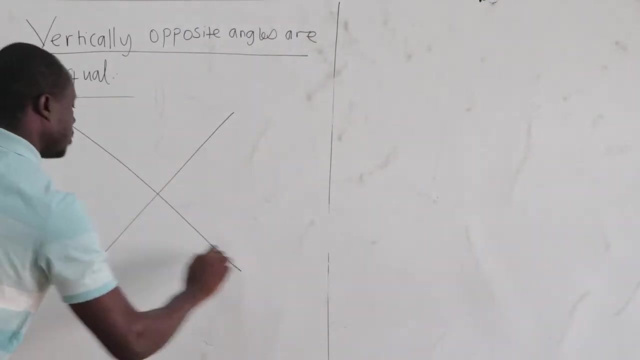 Let's consider more examples Now. the next one we like to look at is vertically open. This is vertically opposite angles, And vertically opposite angles are equal Now if we have two straight lines. So let's say we have one straight line, another straight line. 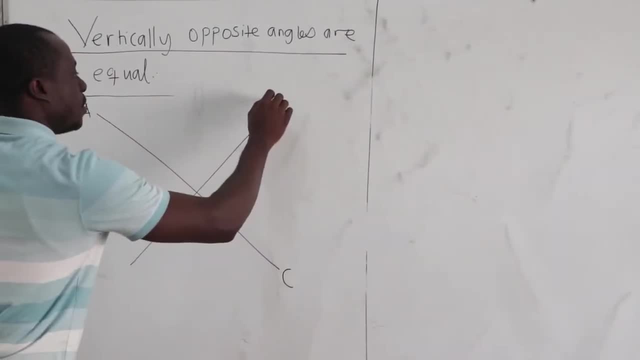 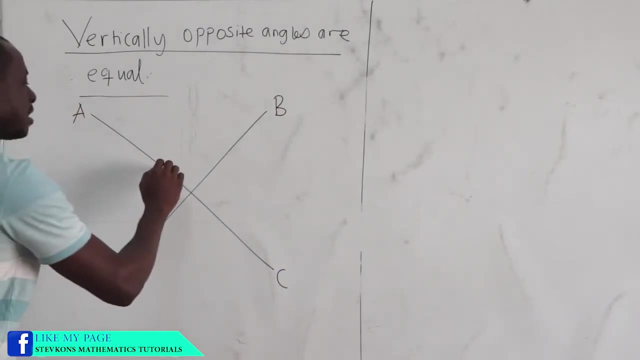 Let's call this AC And let's call this BZ. Now, these are two straight lines, So the angle and this is meeting at this particular point Now, opposite angles are equal, So the angle over here is the same as the angle over there. 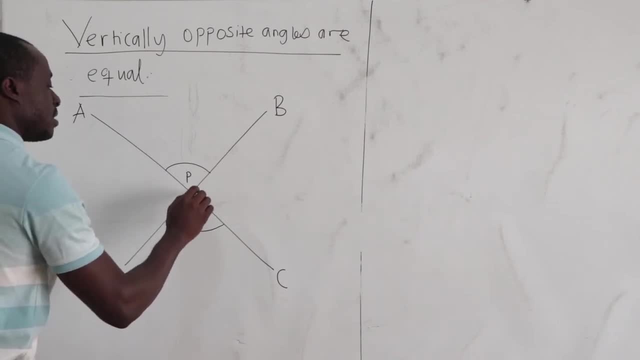 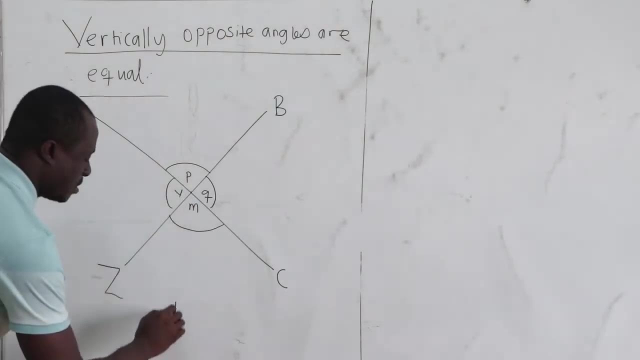 Now let's call this P, Let's call this M, Let's call this Q And then let's call this V. So opposite angles are equal. So all that we are seeing is that P is equal to M And then V is equal to Q. 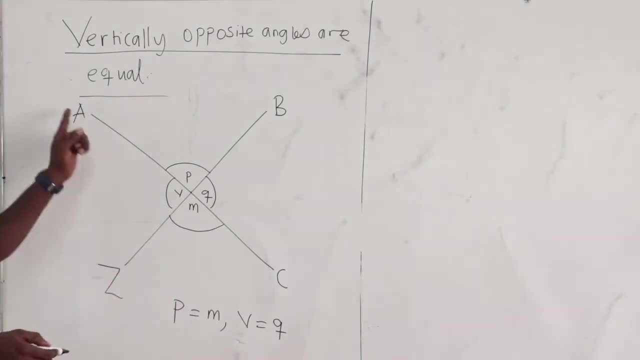 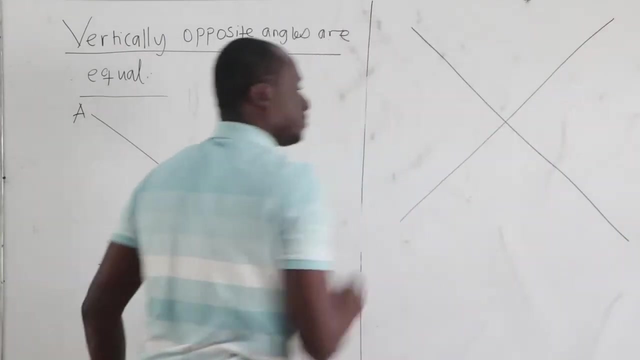 So we say opposite angles are equal. So we have vertically opposite angles. When two straight lines are meeting at a point, the angles formed at opposite sides are equal. So the angle here is equal to the angle over there. Now let's note if we have this straight line here. 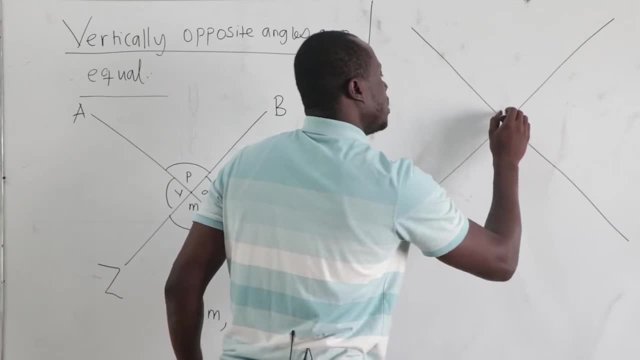 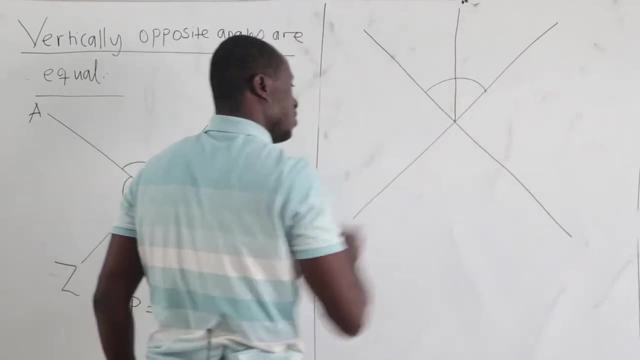 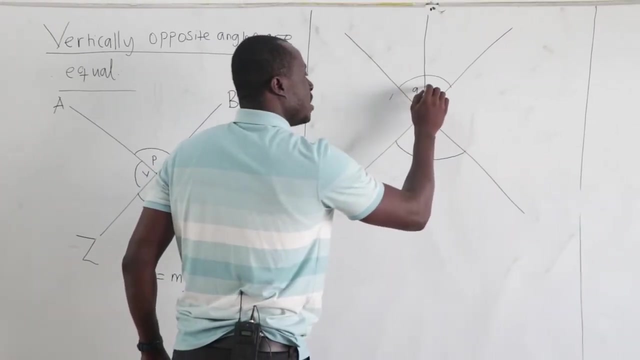 And then this one. probably there is a line going through it. Note that all the angle over here- because this is a straight line- This is also a straight line- All the angle over here is equal to the angle over there. So if this is A and then the angle here is B, 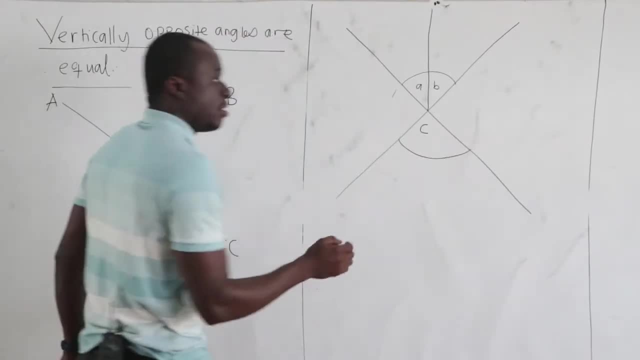 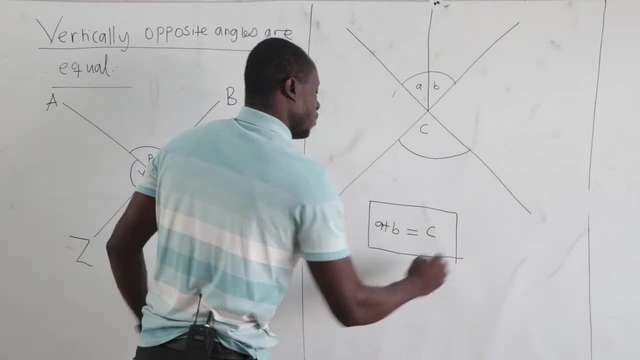 And let's suppose that the whole angle here is C, Then all that we need to know is that A plus B is equal to C, From where Vertically opposite angles, The whole of the angle here is equal to the angle over there. 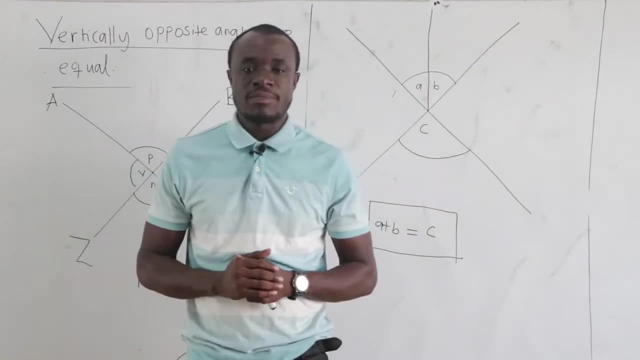 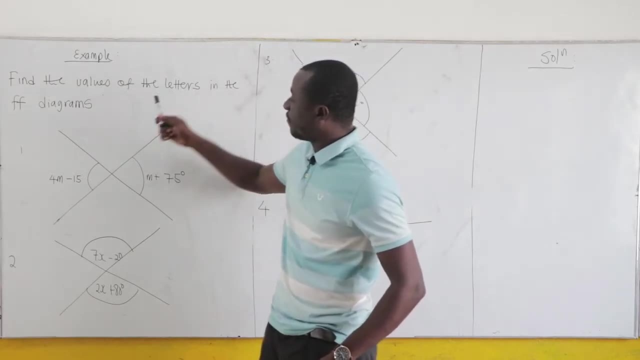 Now let's consider examples for better understanding. Now let's consider the following examples. Now find the values of the letters In the following diagrams. Now let's see question one. Now, this is a straight line. This is also a straight line. 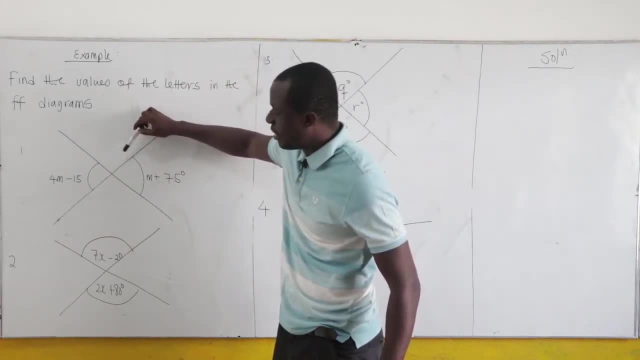 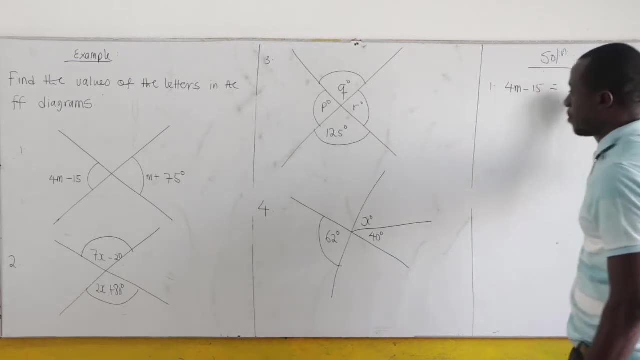 So the angle over here is vertically opposite to the angle over here. So with the first one we have, that is, 4M minus 15, equal to M plus 75 degrees. Now what do we do? We group like this: 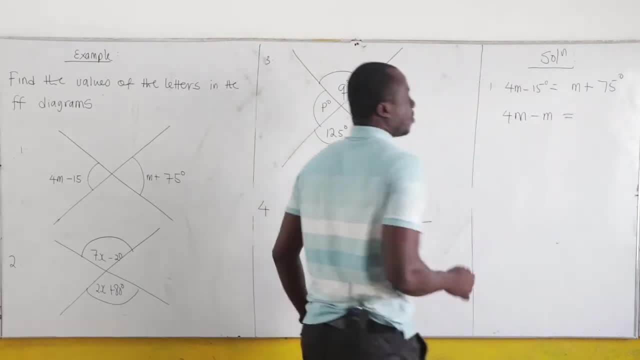 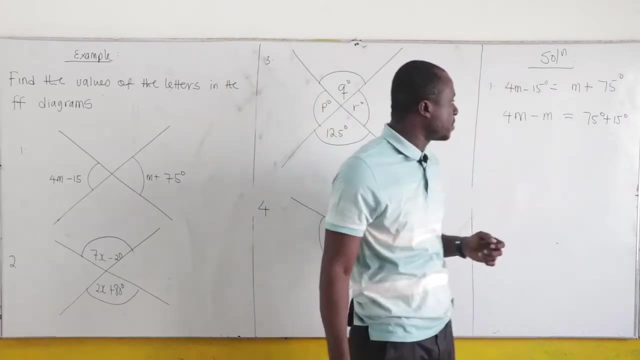 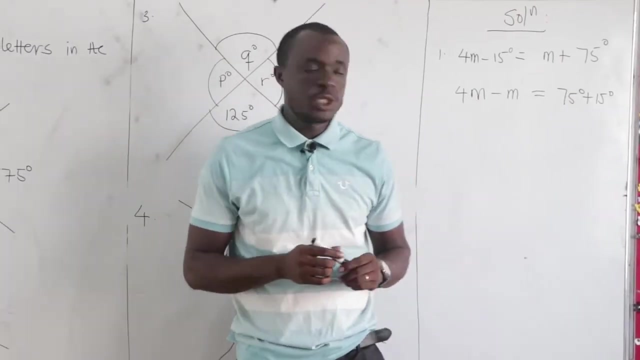 So we have 4M minus M, equal to 75 degrees Plus 15 degrees. Why, plus This negative crossing becoming positive, This is positive crossing becoming negative: 4M minus M. From our idea of algebra, This is just. 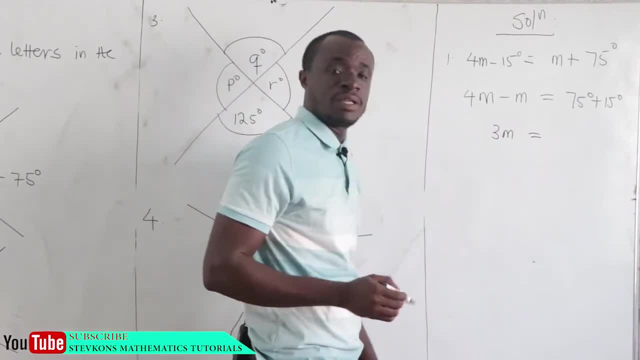 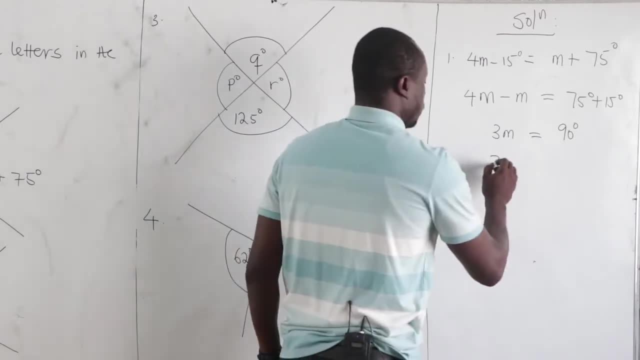 That is 3M, And then 75 degrees plus 15 degrees. This is just 90 degrees. Now I want to find M, So we divide both sides by 3.. So 3M all over 3, equal to 90 degrees all over 3.. 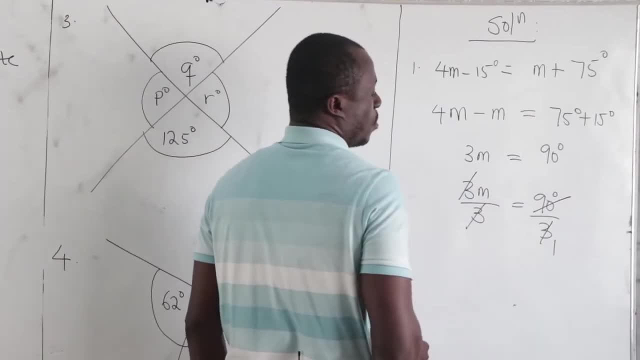 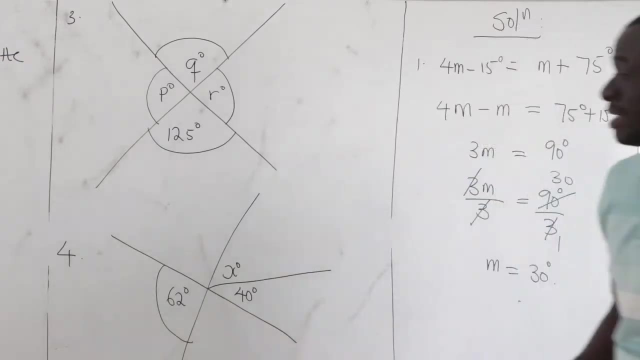 So this is canceling out that. 3 go here 1. 3 will go into 90. That is 30. So we have our M to be equal to 30 degrees. Now let's see the second one. 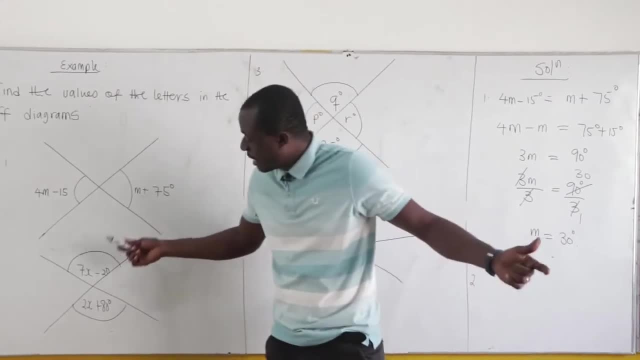 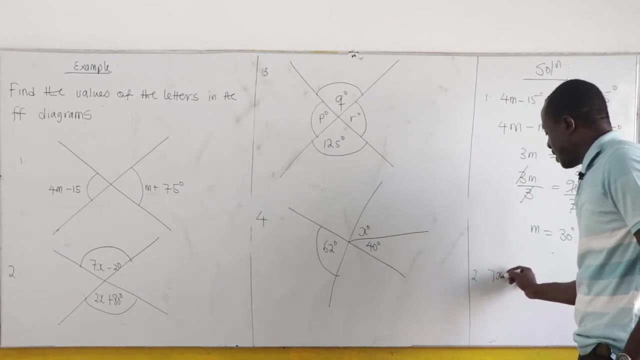 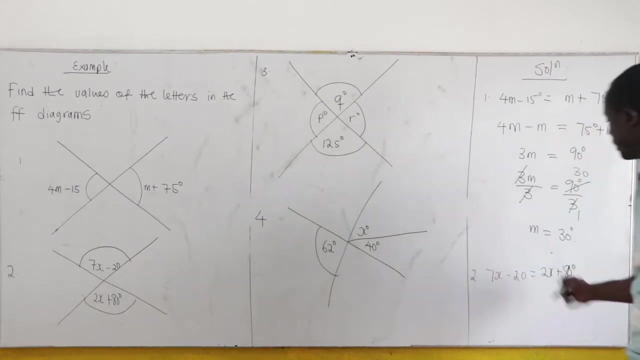 So the second one to the same thing. Vertically opposite angles are equal. So the angle here is vertically opposite to the angle over there. So we have 7X minus 20, equal to 2X plus 80. And we group like them. 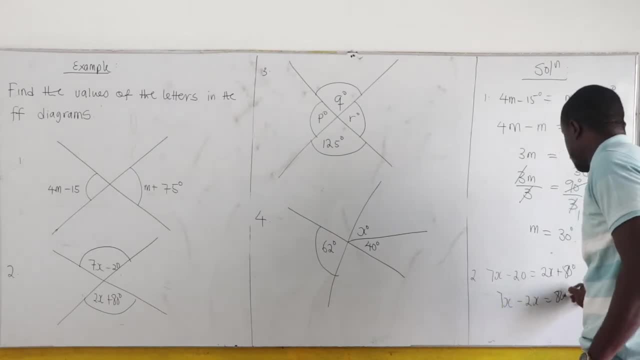 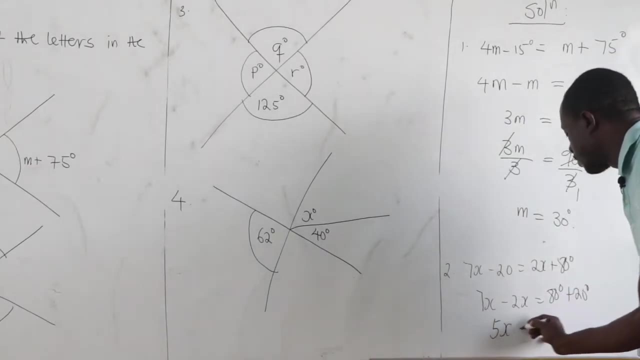 So we have 7X minus 2X, equal to 80 degrees plus 20 degrees. 7X minus 2X, This is just 5X, 80 plus 20.. This is just 100 degrees. We want to find X. 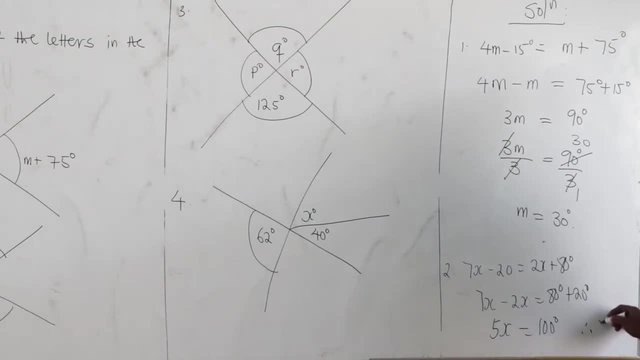 How many times will X go into 100?? That is. how many times will 5 go into 100?? That is 20 times. So X is equal to 20 degrees. Now let's consider the third one. Now there is a straight line. 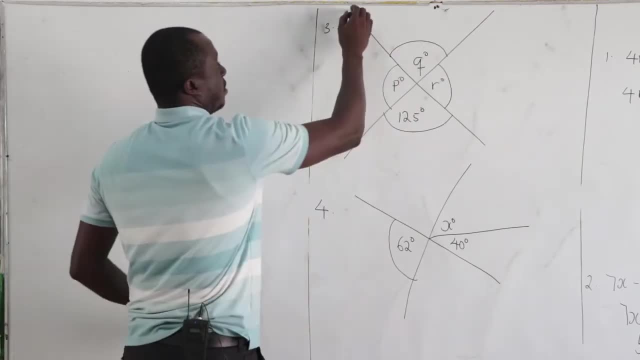 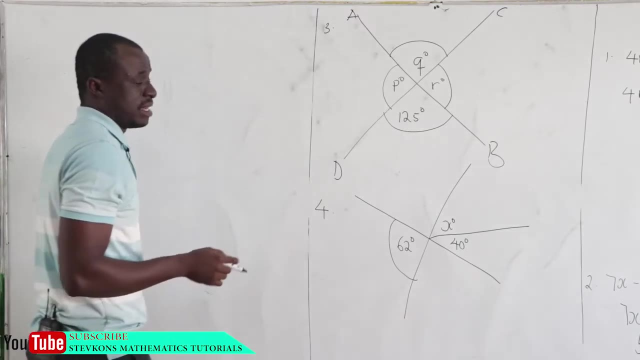 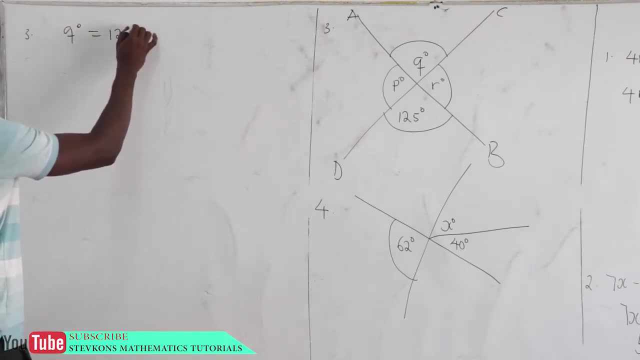 There is also another straight line. Okay, If this is AB and then this is CD. Now, so AB and CD are straight line, intersecting So clearly. what can we see? Q degrees is equal to 1,, 2,, 5 degrees. 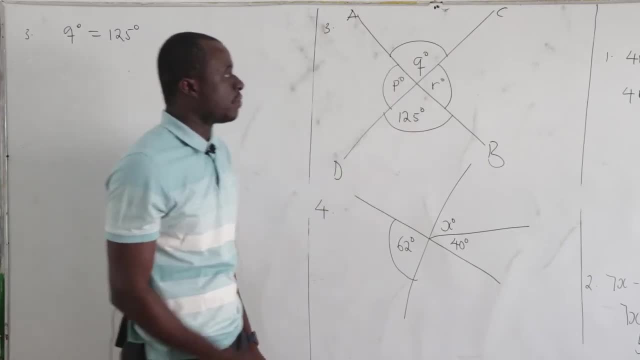 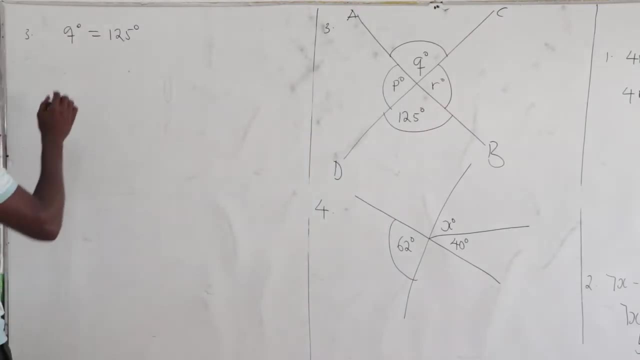 5 opposite angles are equal. Now on the line, CD 125 plus R degrees is equal to 180.. Sum of angles on a straight line. So we have R degrees plus 125 degrees equal to 180 degrees. Sum of angles on a straight line. 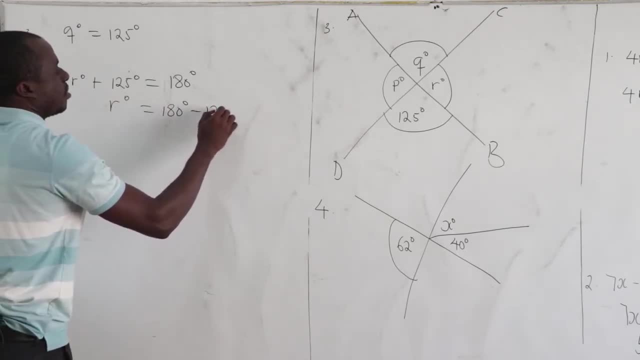 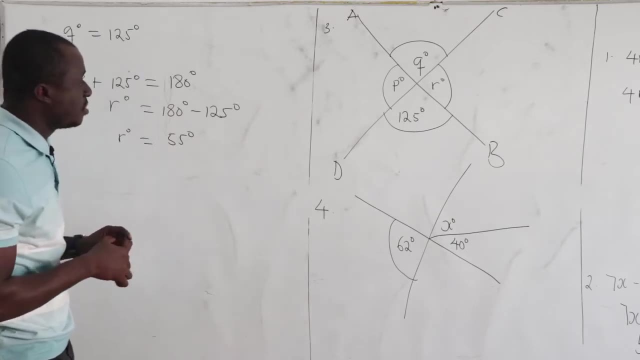 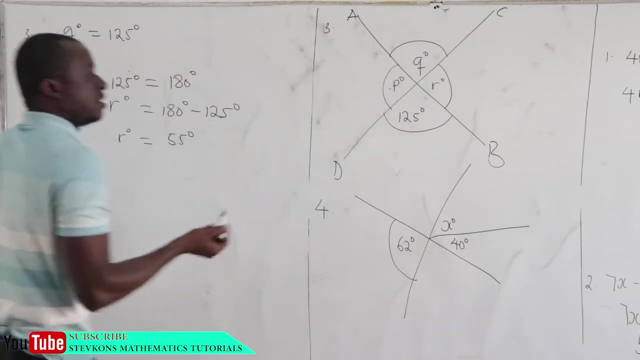 Clearly, R degrees is equal to 180 degrees minus 125 degrees. So R is just 55 degrees, 180 minus 125 degrees. Now P and R. P and R are also vertically opposite, So our P degrees is the same as our R degrees. 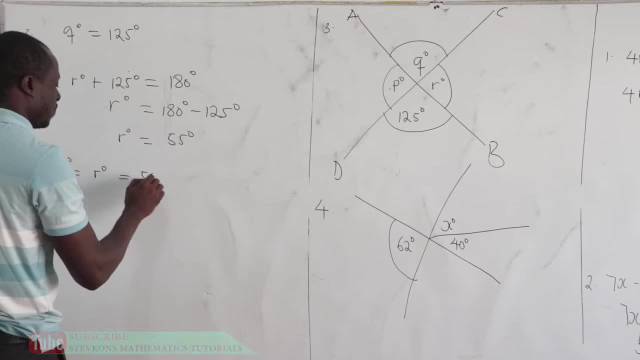 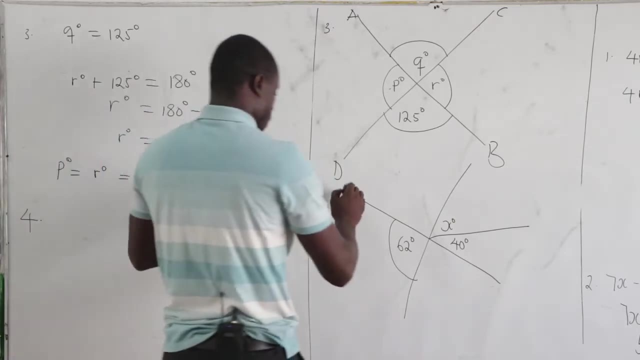 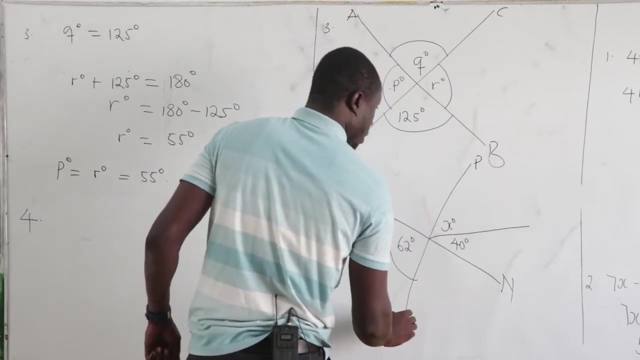 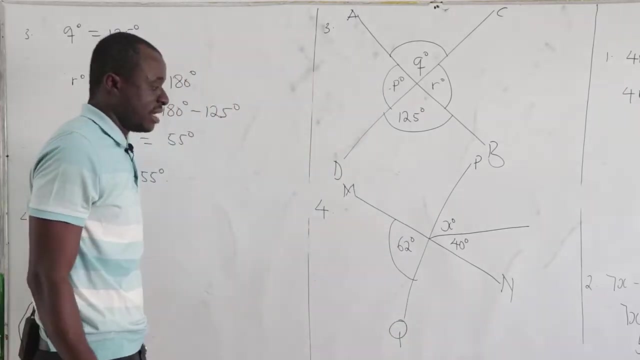 Why Vertically opposite degrees, And this is just 55 degrees. Now let's consider our fourth question. Okay, Let's name this. Probably, if this is MN, and then this is PQ, Now PQ and MN are straight lines. 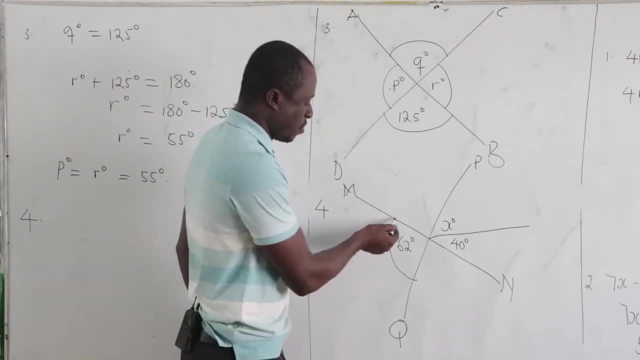 Now, hence, because they are straight lines, We can conclude that the angle over here is vertically opposite to the angle over there. So over here we are saying that X degrees plus 40 degrees equal to 62 degrees. So our X is equal to 62 degrees minus 40 degrees. 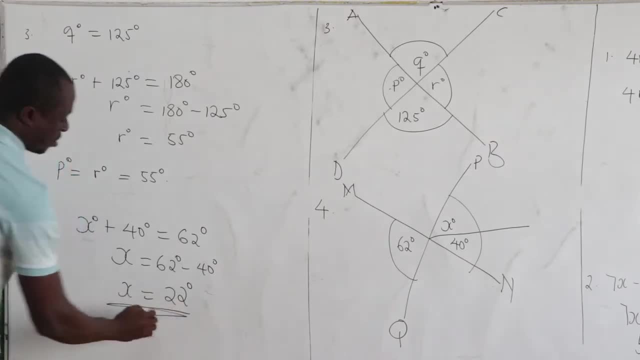 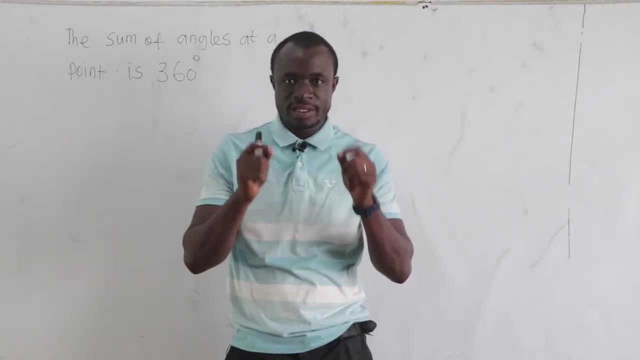 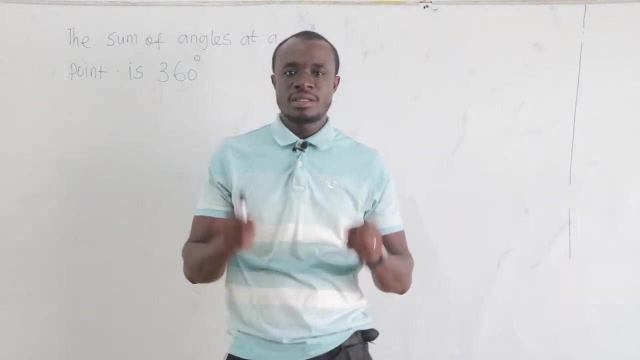 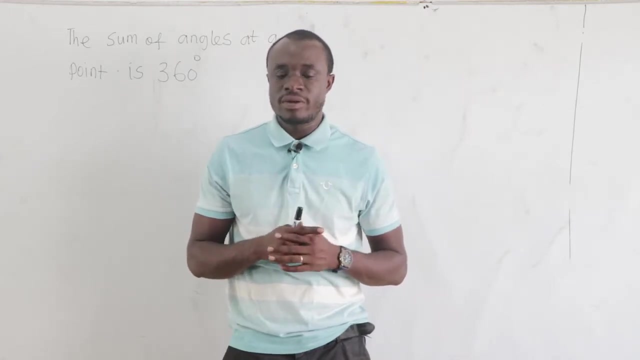 So X is equal to 22 degrees. This is very, very trivial. The sum of angles at a point is equal to 180.. The sum of angles at a point is equal to 360 degrees. The sum of angles at a point is equal to 360 degrees. 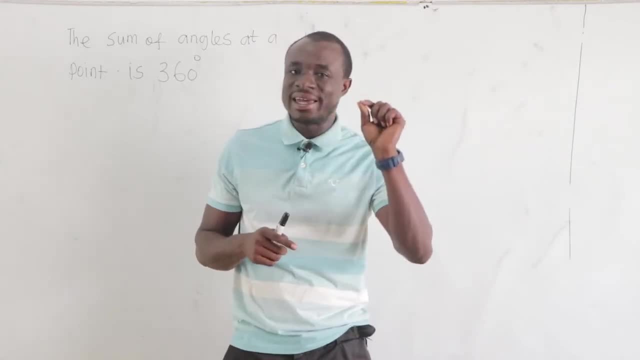 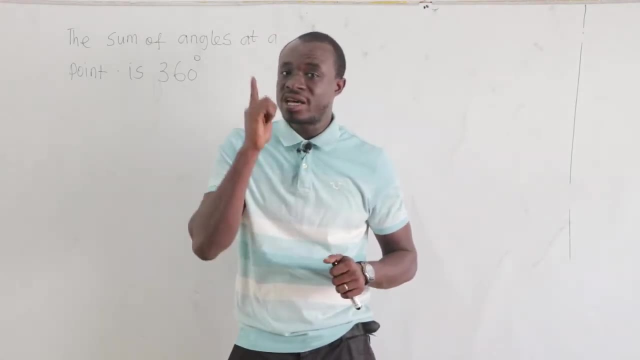 We learnt earlier that the sum of angles on a straight line at a point That one is equal to 180 degrees, But in this case we are saying that the sum of angles at a point The straight line is not there At a point is equal to 360 degrees. 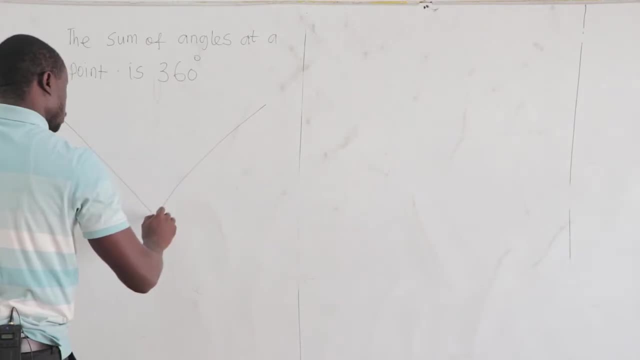 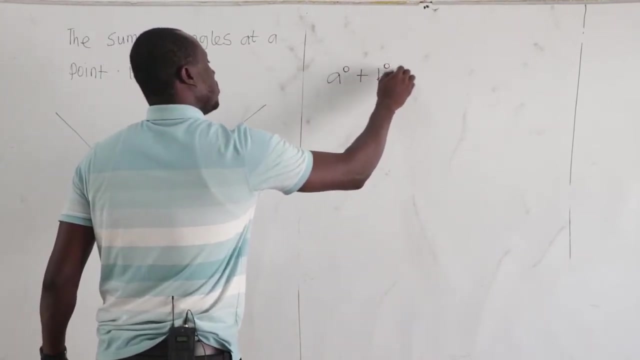 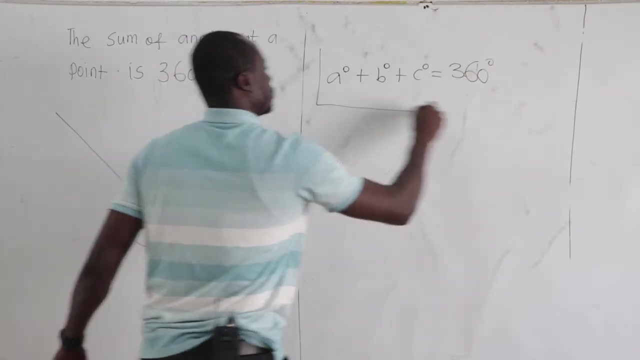 So let's suppose that we have this diagram. Let's suppose this is our A, B and C. Now what are we saying? All that we are saying is that A degrees plus B degrees plus C degrees, This is equal to 360 degrees. 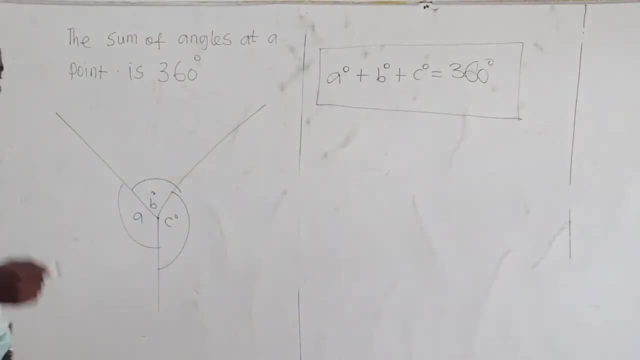 The sum of angles at a point is equal to 360 degrees. So this is the point over here. So the sum of angles all around it, This is equal to 360 degrees. Let's consider the following examples for better understanding. 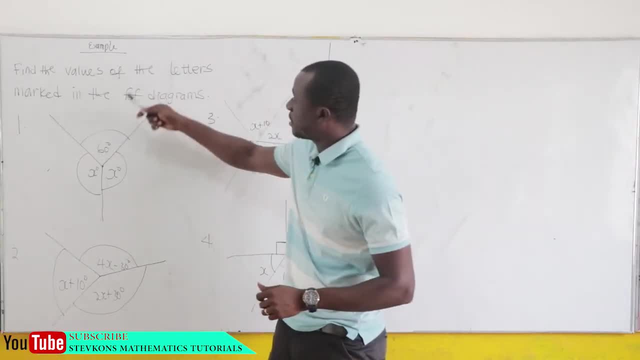 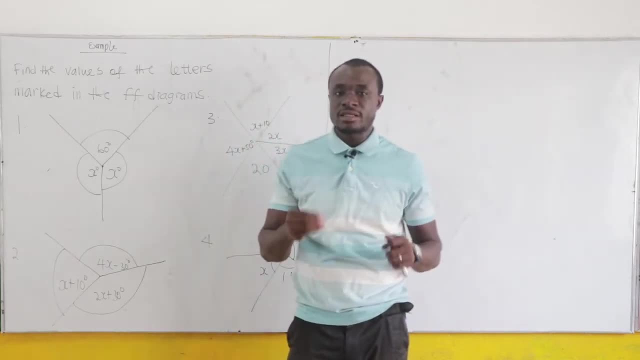 Now let's consider the following example. Find the values of the letters marked here In the following diagram. So there is a diagram. So which principle are we going to use over here? The sum of angles at a point is equal to 360 degrees. 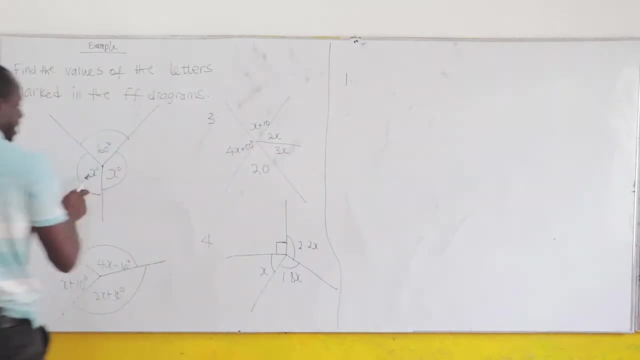 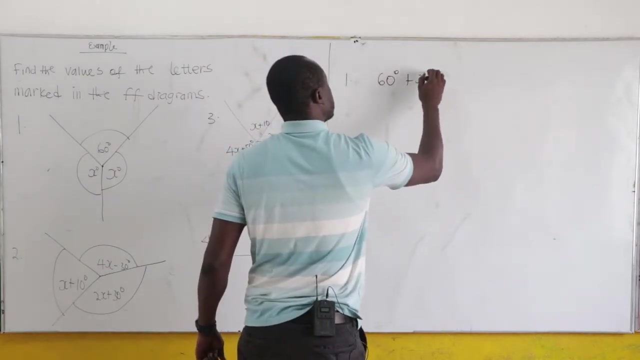 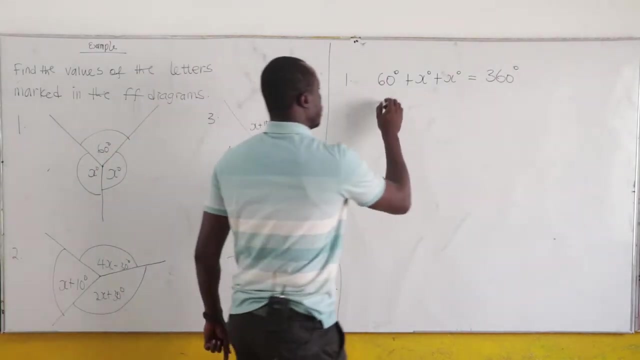 So the first one: What are the angles at the point? That is, X degrees, X degrees, 60 degrees. So we have 60 degrees plus X degrees plus X degrees, And this is just 360 degrees. Now we have 60 degrees. 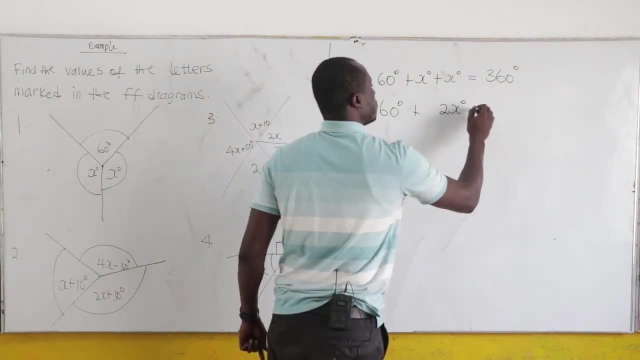 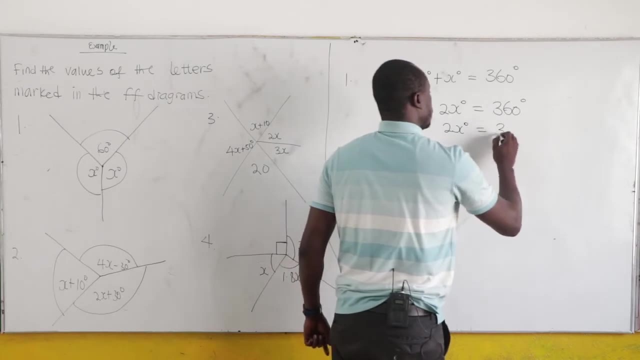 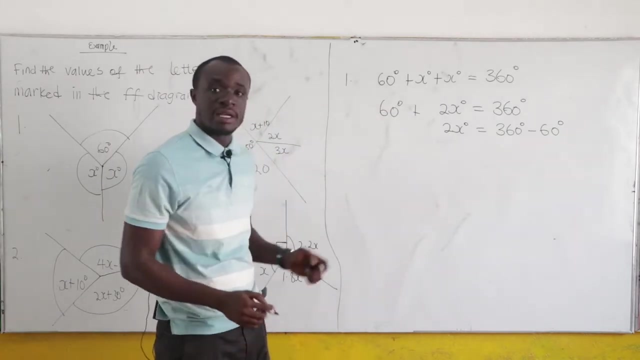 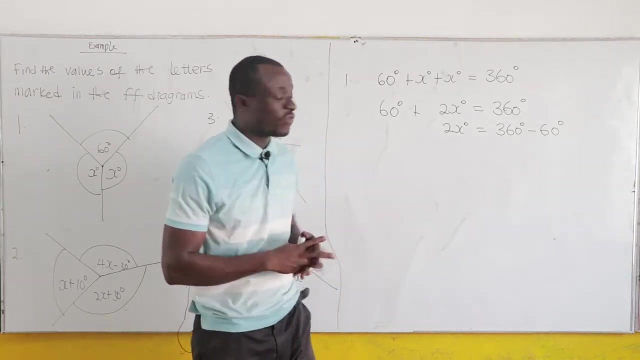 X plus X degrees, That is 2X degrees equal to 360 degrees. So we have 2X degrees equal to 360 degrees minus 60 degrees. We are grouping like firm. This is just a linear equation. If you have forgotten, kindly visit my page for more tutorials for revision on linear equations. 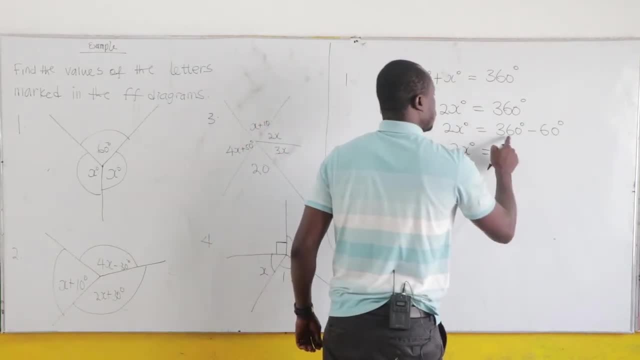 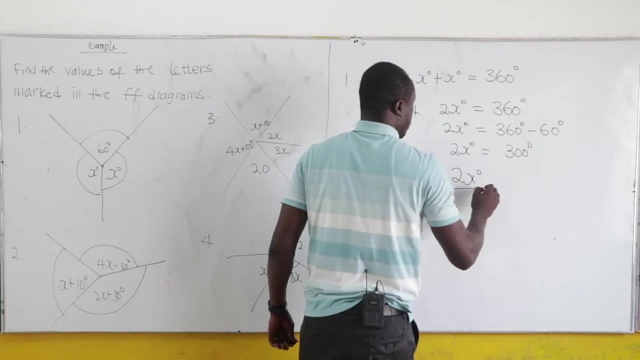 Now we have 2X degrees equal to 360 degrees, X degrees equal to 360 degrees minus 60 degrees, That is, 300 degrees. We want to find X, So we divide both sides by 2. So this is constantly like that. 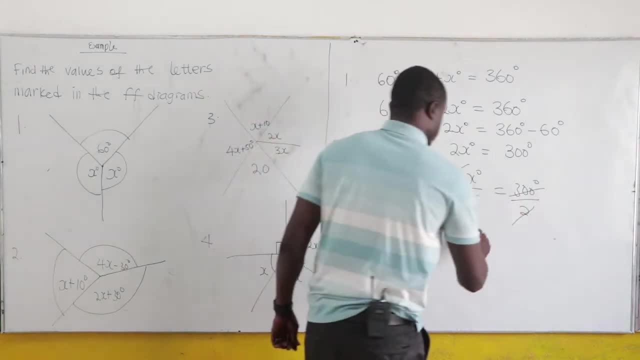 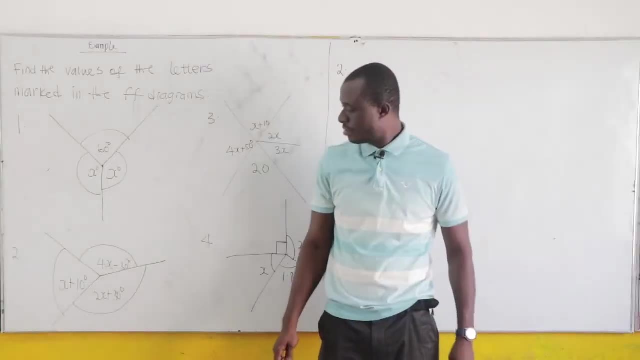 Now how many times would 2 go into 300?? That is 150 degrees. So X is equal to 150 degrees. This is very, very trivial. Now let's consider the second question, So angles at a point. 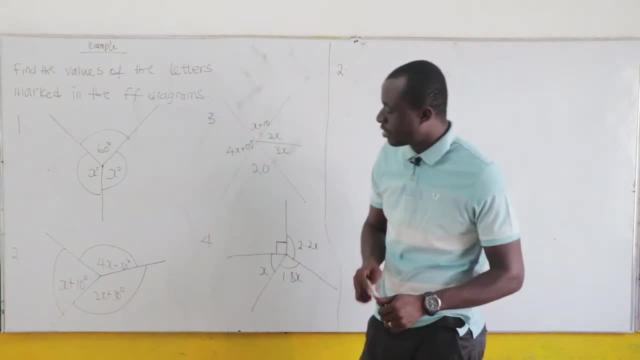 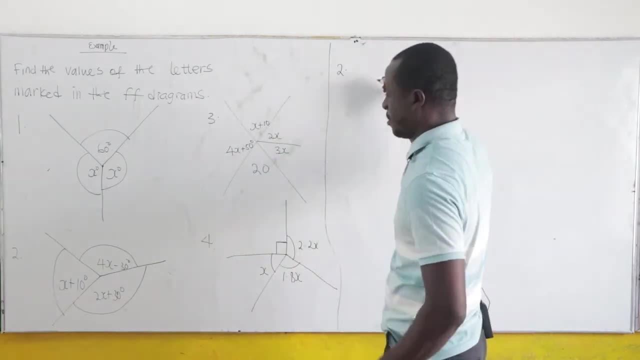 What are the angles? That is, X plus 10 degrees, 4X minus 30 degrees, 2X plus 30 degrees. Now this is a busy past question. So here, sum of angles at a point is equal to 360 degrees. 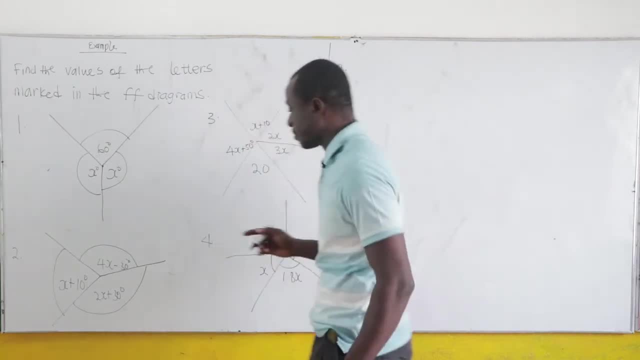 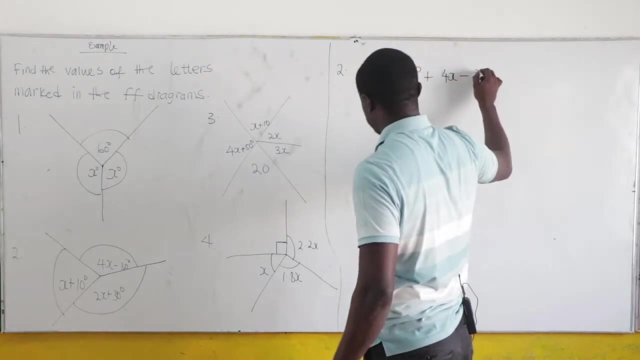 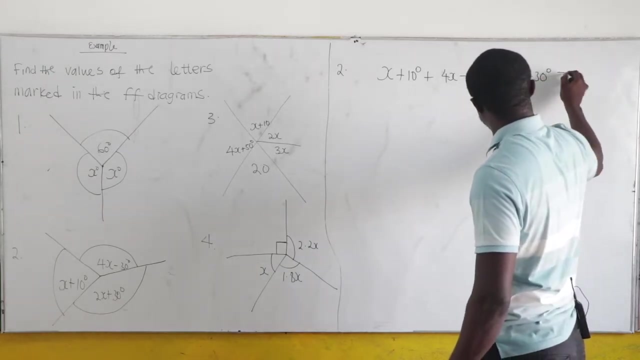 Sum of angles at a point is equal to 360 degrees. So we have X plus 10 degrees plus 4X minus 30 degrees plus 2X Plus 2X plus 30 degrees, equal to 360 degrees. Now let's group the terms. 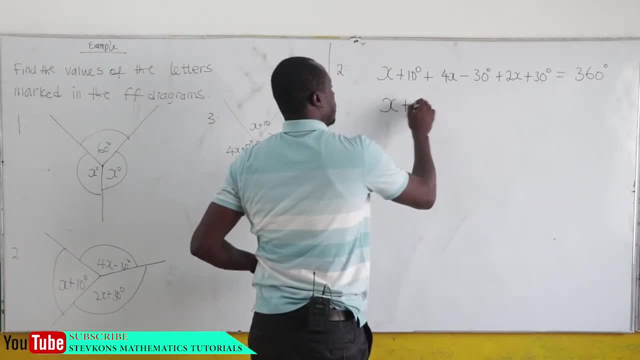 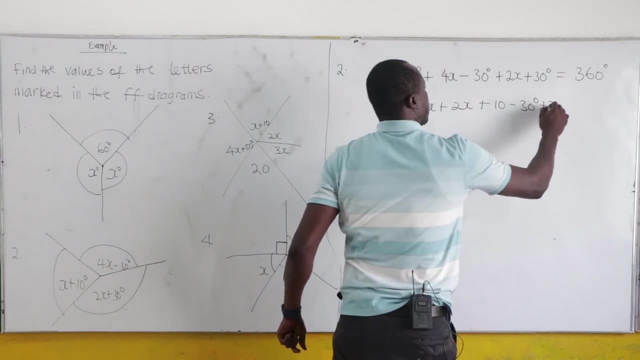 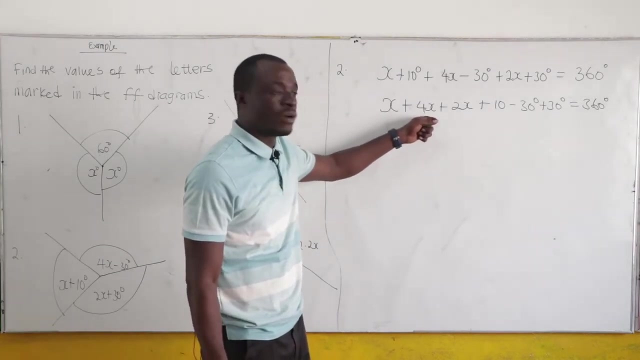 We have X, 4X- 2X. So we have X plus 4X plus 2X plus 10, minus 30 degrees plus 30 degrees, equal to 360 degrees. Now let's see X plus 4X. 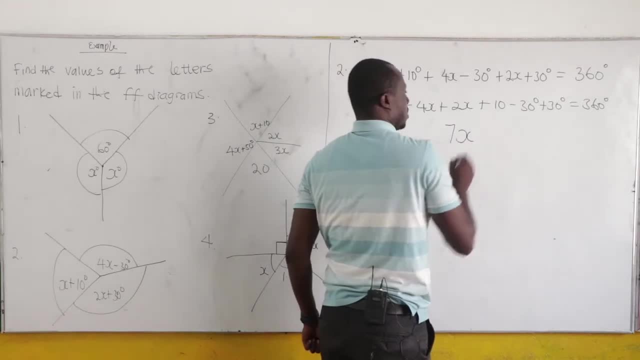 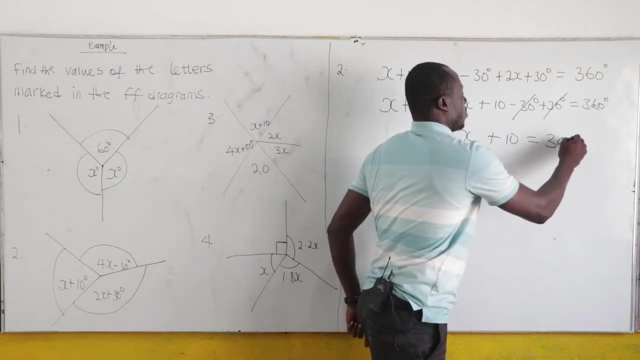 That is 5X plus 2X. This will give us that is 7X. Now negative 30 and positive 30 will cancel out. So plus 10 equal to 360 degrees. Now we want to find X. 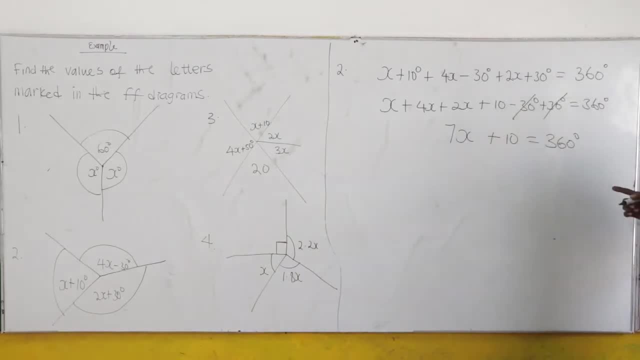 What do we do? We group like this: This has to come to the right hand side. So we have 7X, equal to 360 degrees minus 10 degrees. 7X, Now 360 minus 10.. This is just 350 degrees. 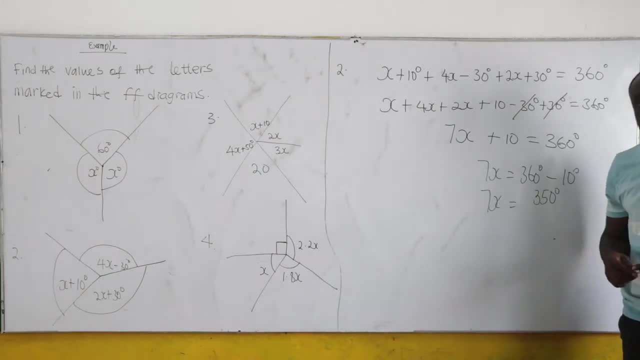 We want to find X. So we divide both sides by what is multiplying the X, which is 7.. 350 all over 7.. This is canceling out. So we go here 1.. So we go into 35.. 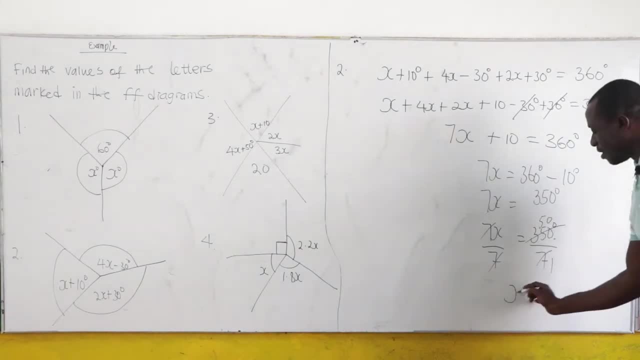 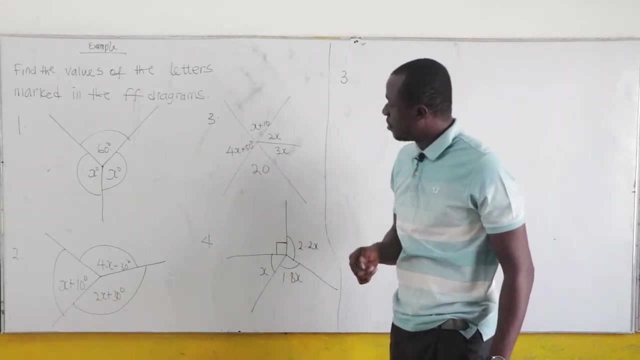 5. So we go into 0.0 times. So you have our X to be equal to 50 degrees. This is very, very trivial. Now let's consider the third question. So we know sum of angles at a point is equal to 360. 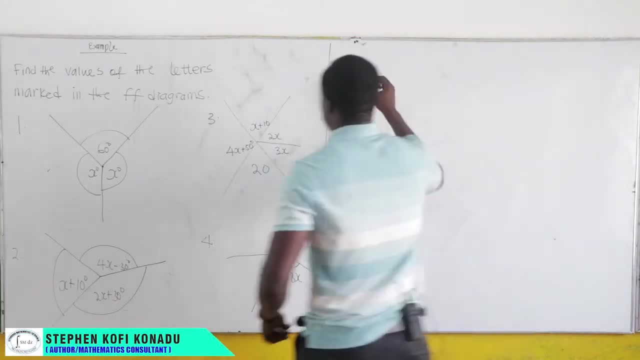 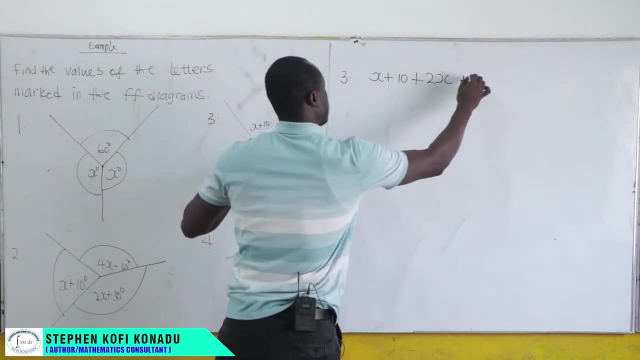 So we have to add all, We equate to 360.. So we have X plus 10.. That is the first one. Second one: we have plus 2X. Third one: we have 3X, We have 20 here. 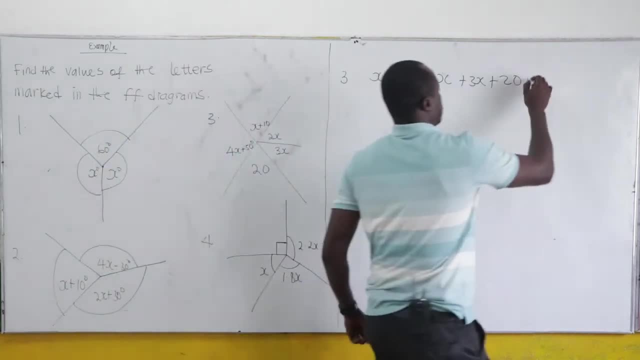 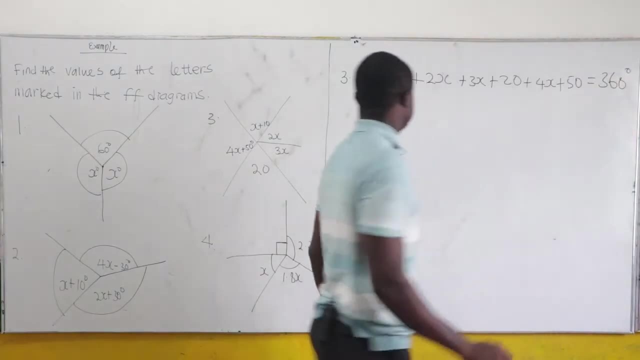 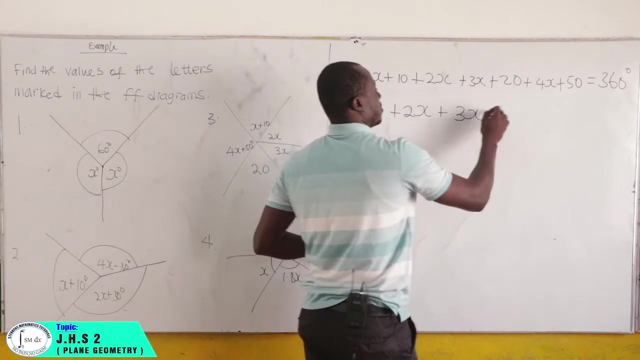 Make sure that we add everything Plus 4X, 4X plus 50. And this is equal to 360 degrees. Now let's group: We have X, We have 2X plus 3X plus 4X. 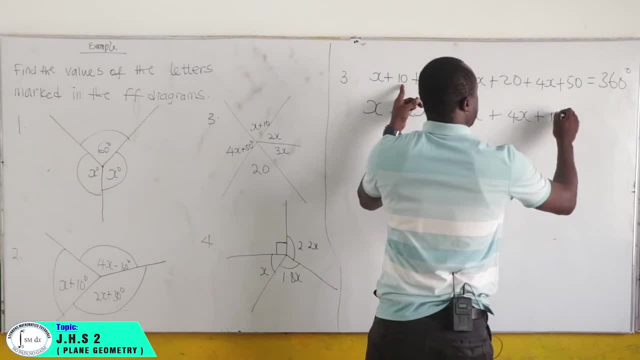 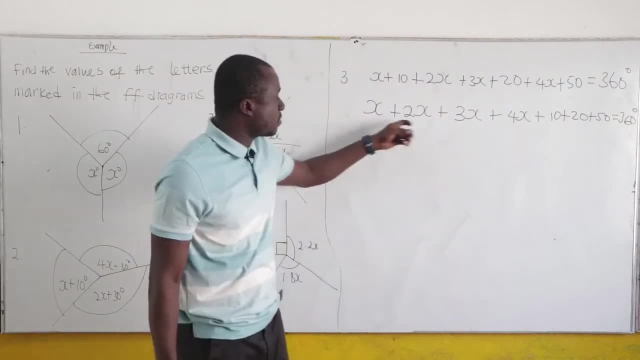 Now let's see The other one. we have 10 plus 20 plus 50. And this is equal to 360 degrees. Now, X plus 2X, That is 3X, 3X plus 3X. 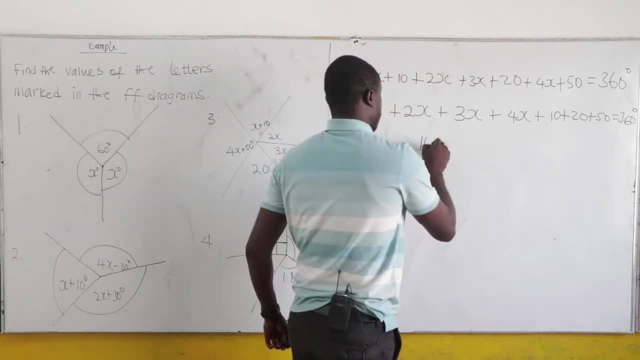 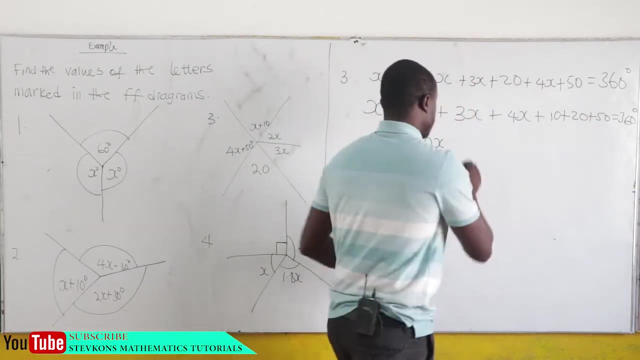 That is 6X. 6X plus 4X. This will give us: That is 10X. Now 10 plus 20.. That is 30.. 30 plus 50. That is 80.. Equal to 360 degrees. 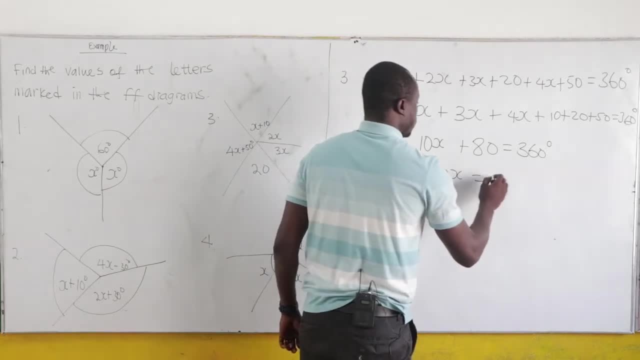 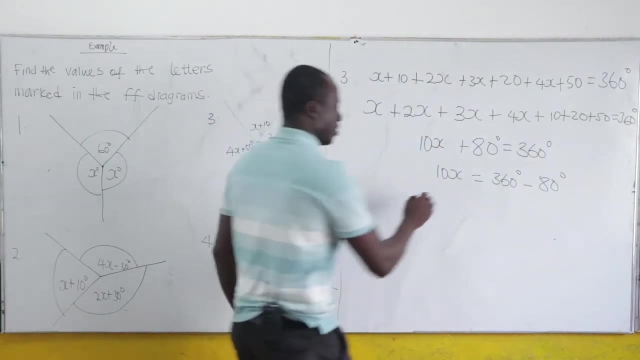 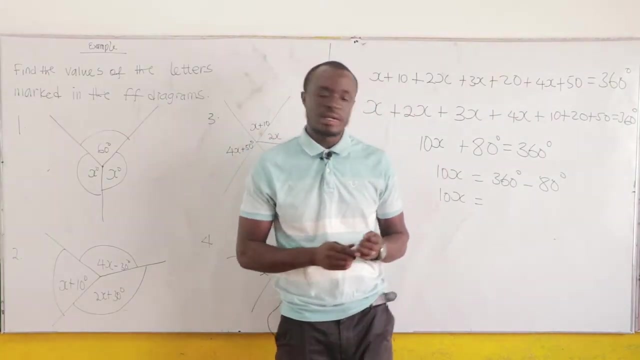 We want to find X. We group like this: We have 10X, equal to 360 degrees minus 80 degrees. Now 10X, What is? 360 degrees minus 80 degrees? 360 degrees minus 80 degrees, 280 degrees. 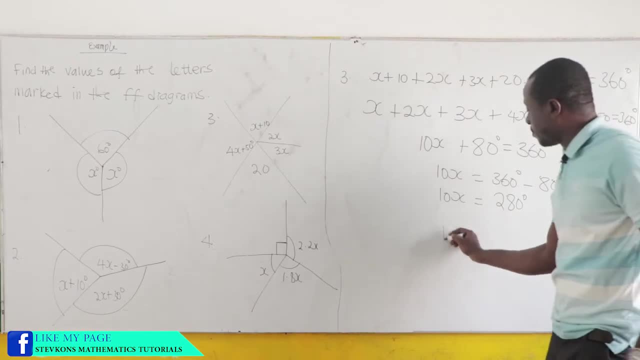 280 degrees. We want to find X. We divide both sides, But what is multiplying the X, Which is 10.. Now, what can we see? This zero is canceling out the zero over here. This 10 is canceling out that. 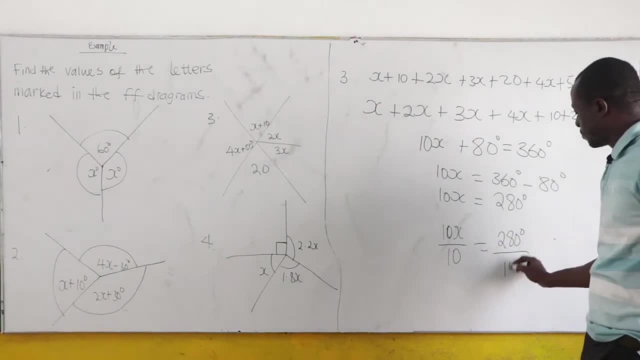 So our X is equal to 28 degrees. Now let's consider: We have 3X plus 3X plus 4X, 3X plus 4X plus 4X, 2X plus 3X plus 4X. 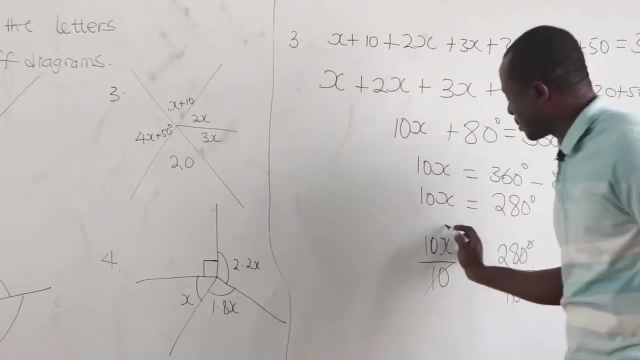 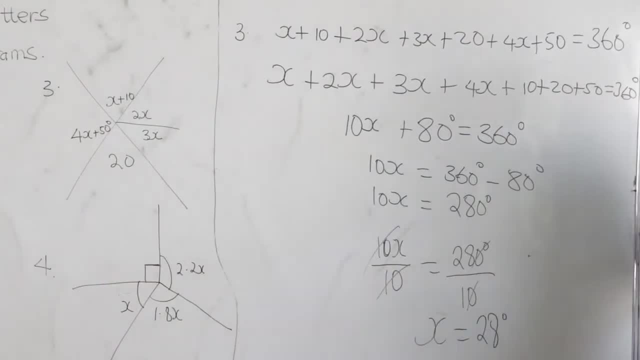 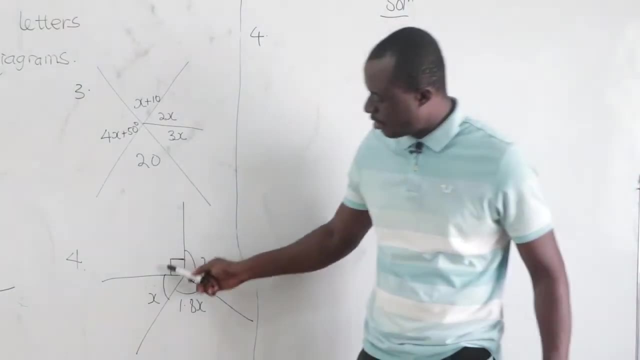 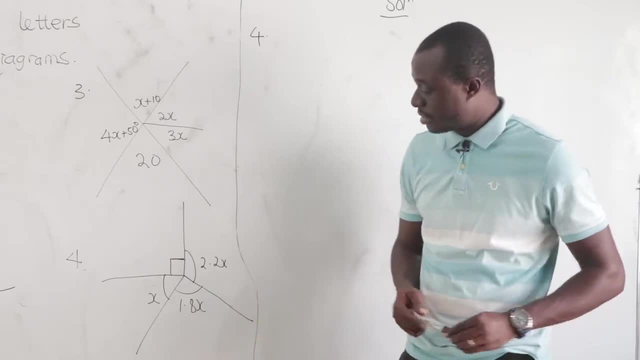 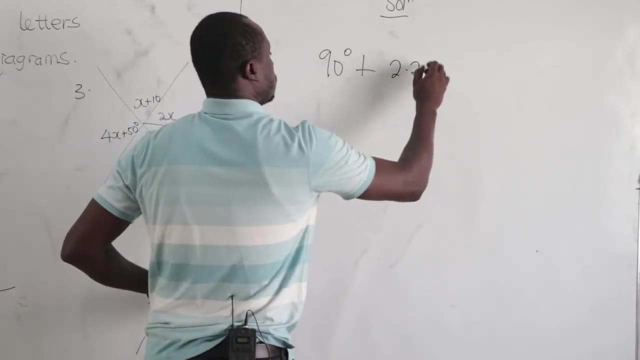 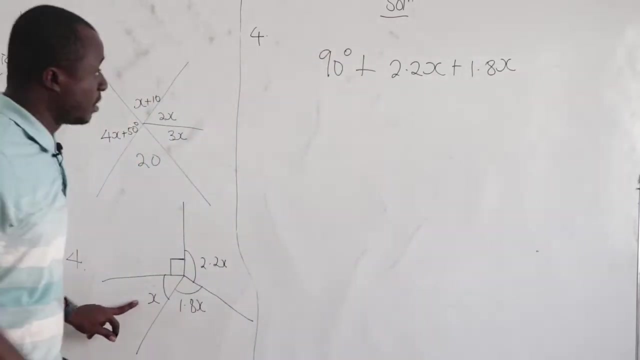 a point. so we can add all the angles, we equate to 360 degrees. so the angle here is 90, so we have 90 degrees. now what's the angle here? that is 2.2 x. what's the angle here? 1.8 x. what's the angle here? 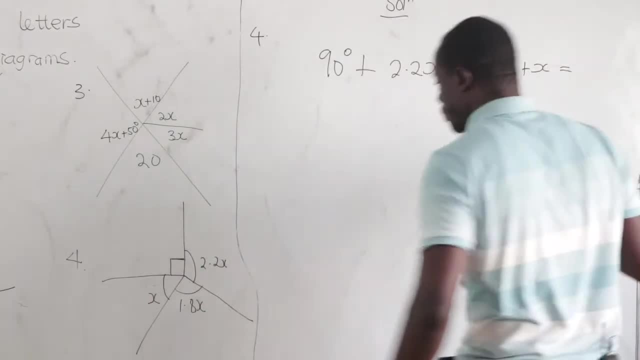 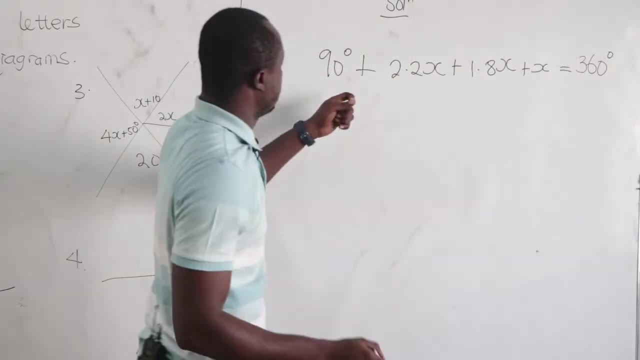 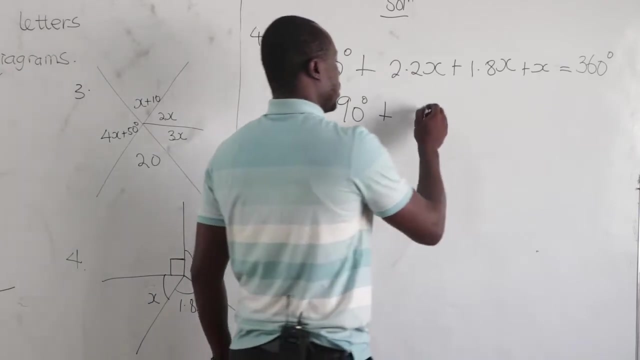 the angle there is x and this is equal to that is 360 degrees. now let's see. so we have our 90 degrees: 2.2 plus 1.8, this is 4 plus 1, so we have 5x equal to 360 degrees. 1, 5 x. we move like that: 5 x equal. 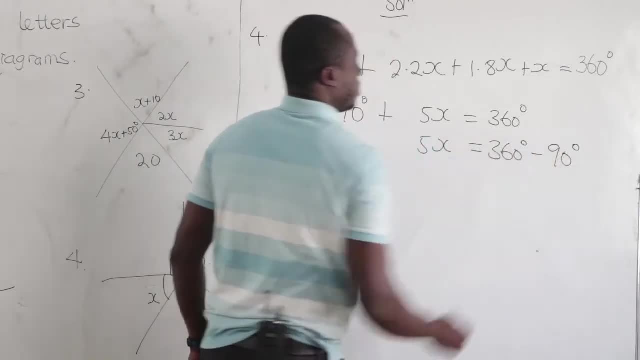 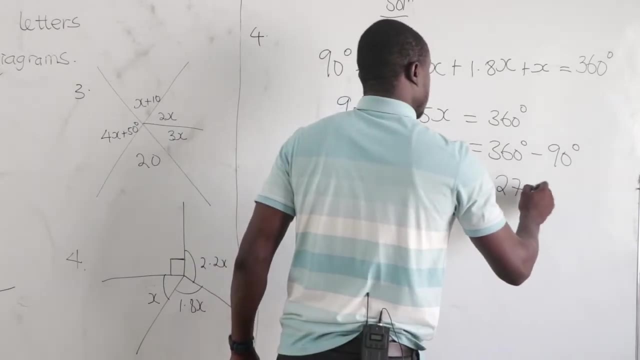 to 360 degrees minus 90 degrees. now what is 360 degrees minus 90 degrees? And this is giving us 270 degrees, 5x. We want to find x, so we divide both sides by what is multiplying the x, which is 5.. 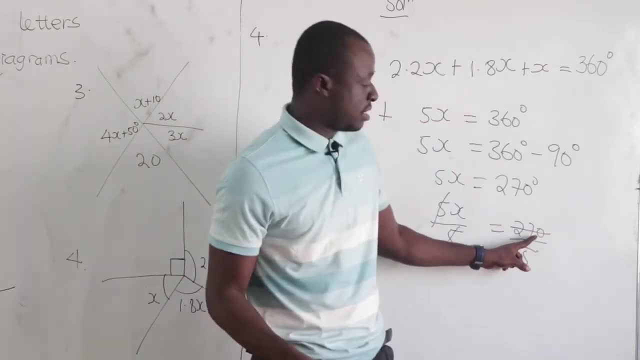 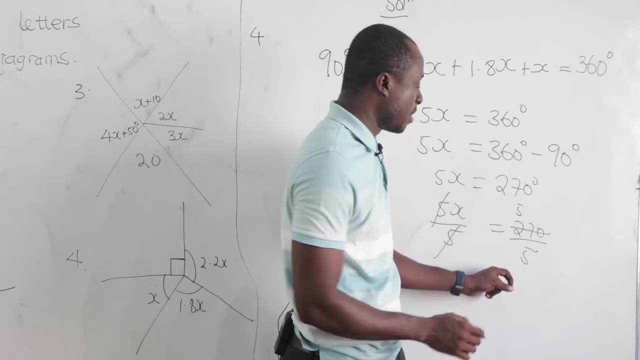 Now, how many times will 5 go into 27?? That will be 5 times 5, 5, 25.. What is remaining 2?. So that will be 20.. 5 will go into 20.. That is 4.. So we have. 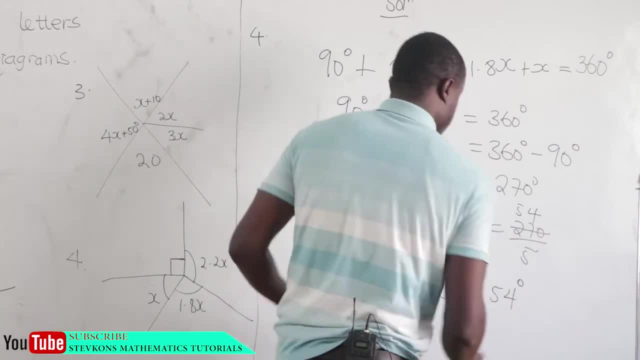 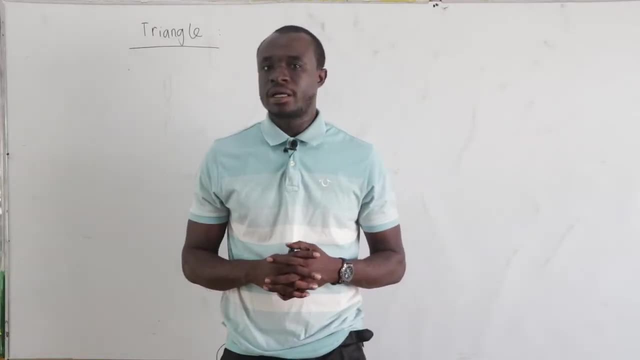 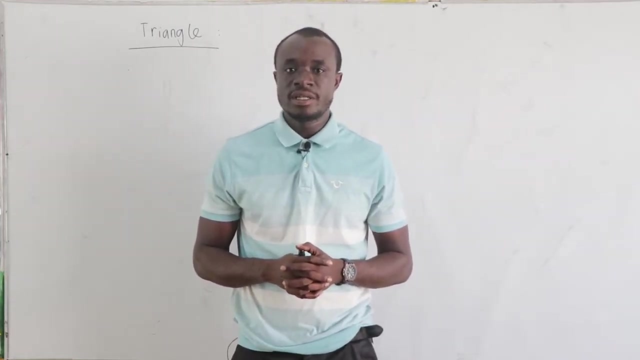 our x to be equal to 54 degrees. I believe you enjoyed the lessons So easy. We would like to look at triangles now. Now, what is a triangle? A triangle is a plain figure bounded by 3 straight lines. A triangle- 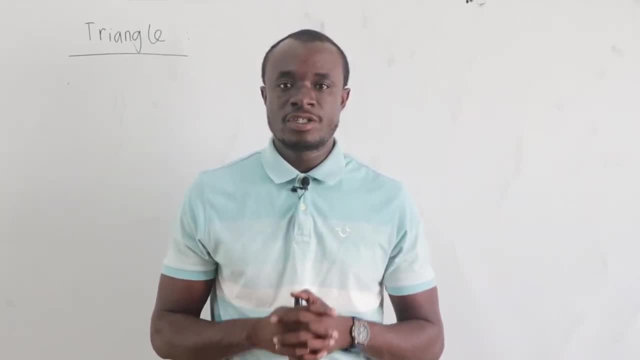 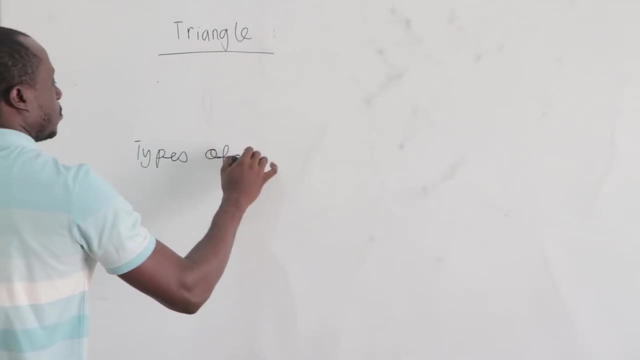 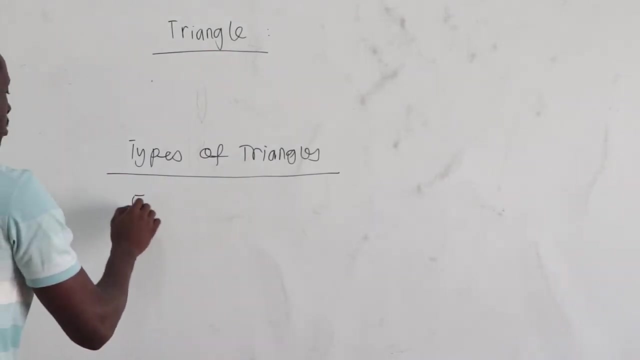 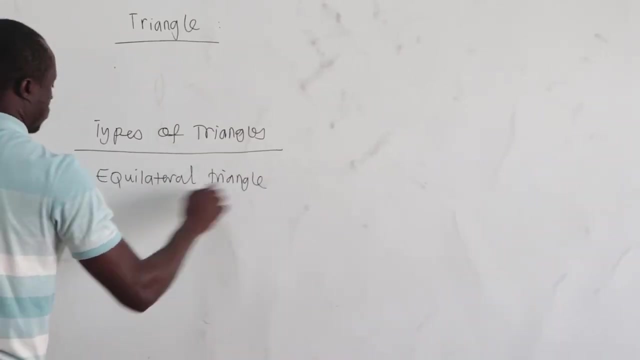 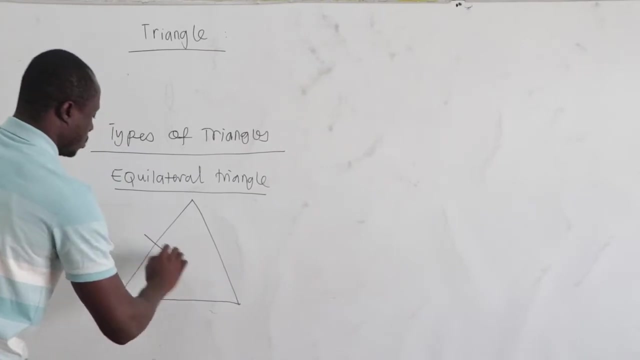 is a plain figure bounded by 3 straight lines. Now let's consider types of triangles Now. the first one is: we want to consider equilateral triangle. Now, if they are equilateral triangles, all sides are equal, So this side is the same as that side. 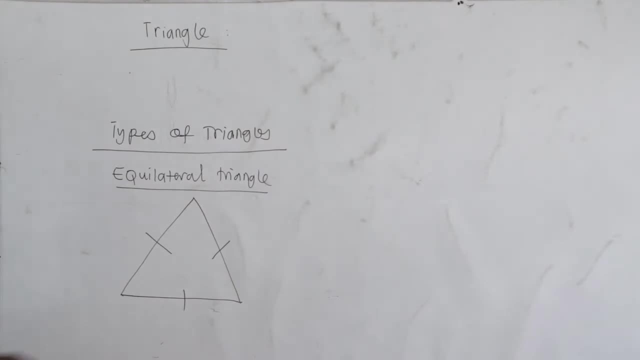 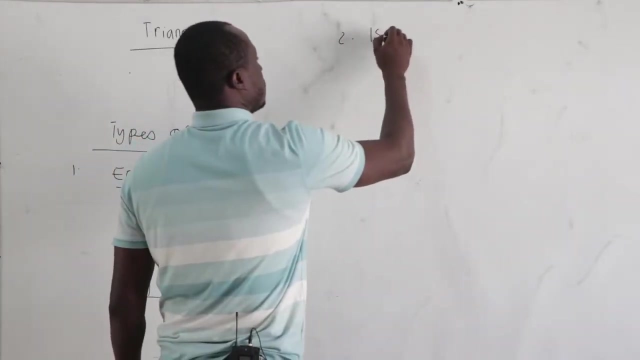 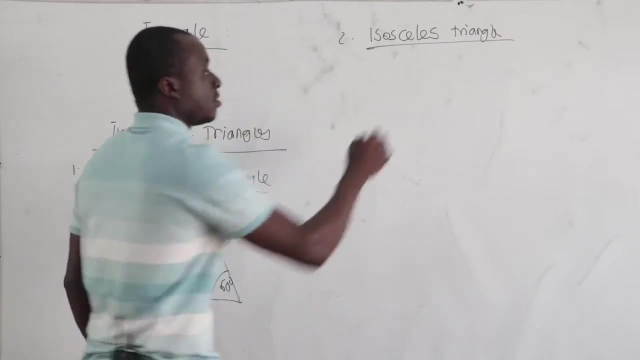 and is the same as the third side as well. Now all the angles are 60 degrees. If equilateral, All the angles are 60 degree. Now the next one you want to look at is isosceles- Isosceles triangle. With isosceles, 2 sides are equal. 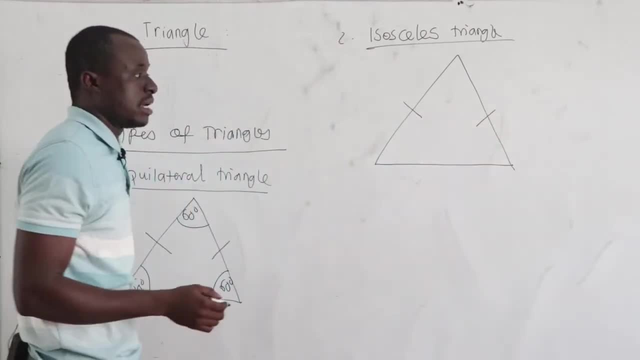 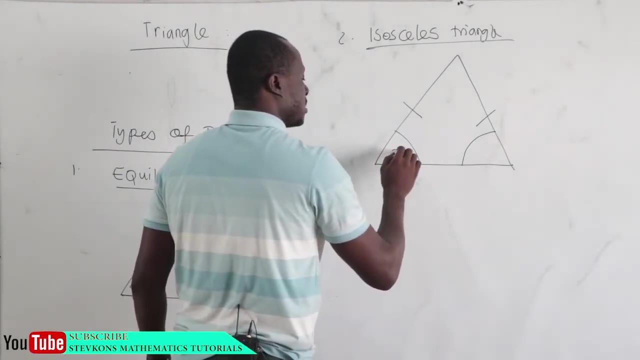 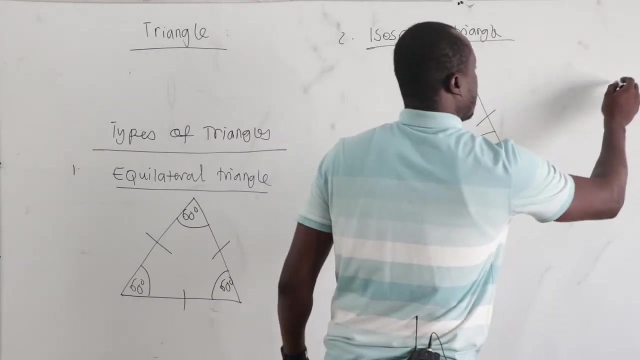 So this side and that side are equal, 2 sides, And the angle over here, the base angles to, are equal. so if the angle here is x, then the angle here to must be x. now you can have this diagram and we can also have a different diagram like this: now it can be that this angle, this side, 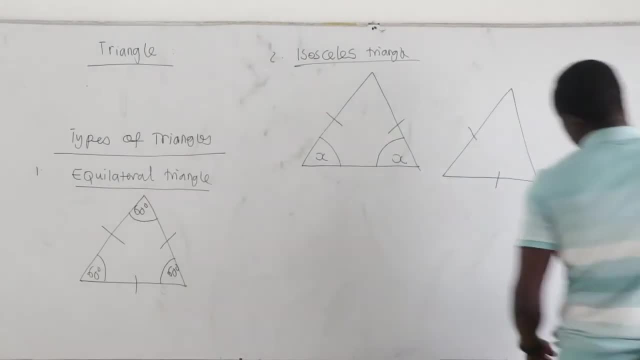 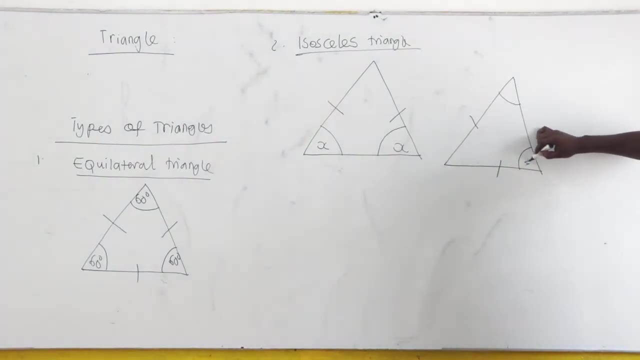 and that side are equal, and if this side and that side are equal, then the angle over here is the same, the angle over here. so if this is, if this angle is m, then the angle over here too is m. so two sides are equal. the base angles must also be equal. now let's see the third one we have. you call it skelim. 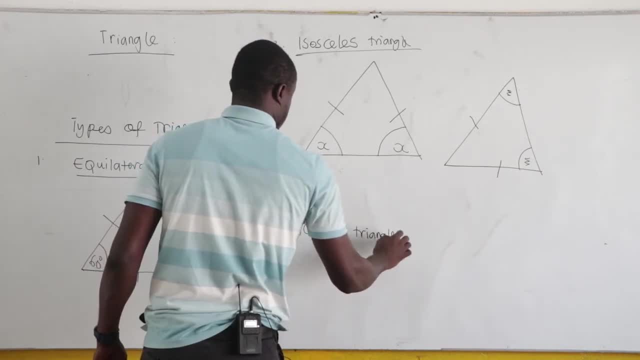 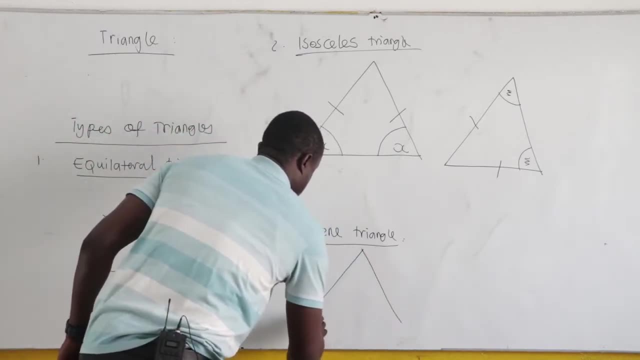 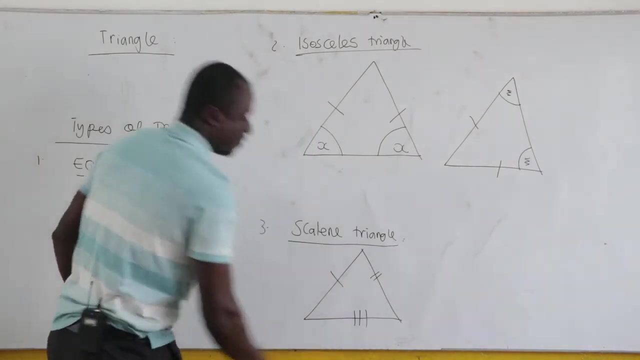 triangle, skelim triangle. now, with skelim, none of the sides are equal. so this: all the sides are of different length, so the side here is different from the side here, which is also different from the side over there. now the angles two. if this angle, let's. 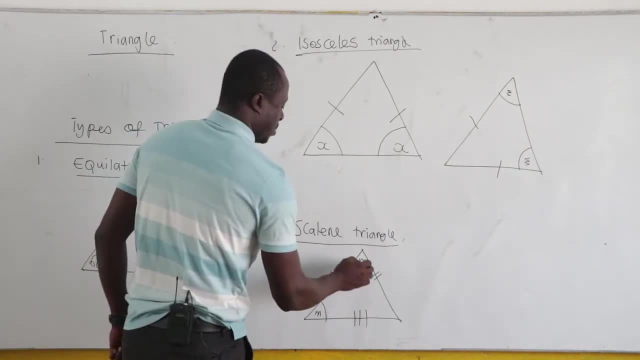 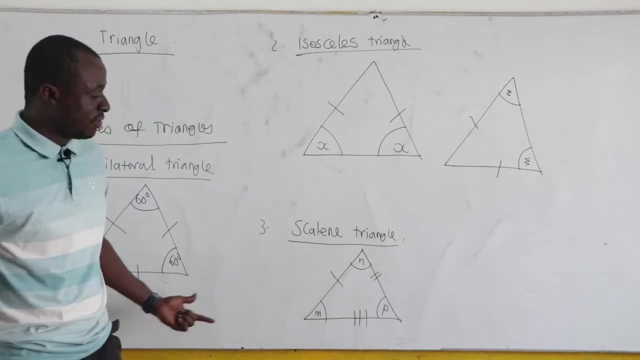 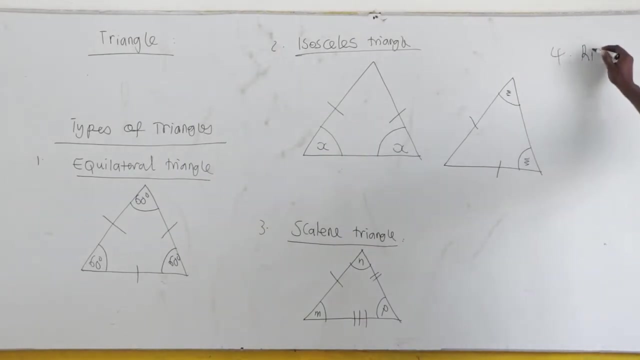 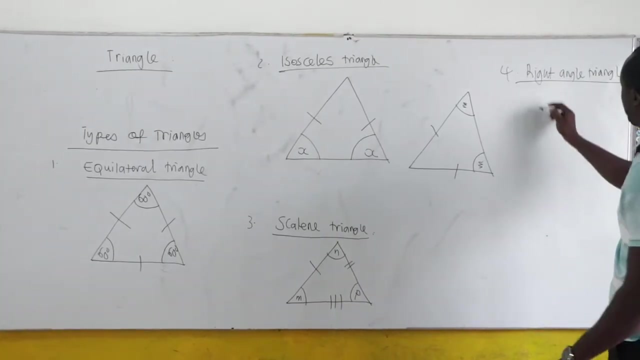 suppose that this angle is M, the angle here will be N, and then the angle here will be, let's say, P. so all the three sides are different, all the angles. two are different. now let's also consider the fourth one. we call it right angle triangle. now, with that, one of the angles must be 90 degrees, so the angle 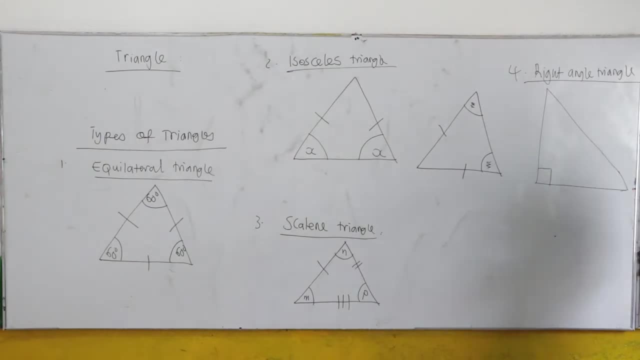 here must be 90, one of them. one of them must be 90 degrees and here, this side, the sides must be 90.. might be or may be either equal or different, But the one thing we have to notice is that the angle here must be 90 degrees. 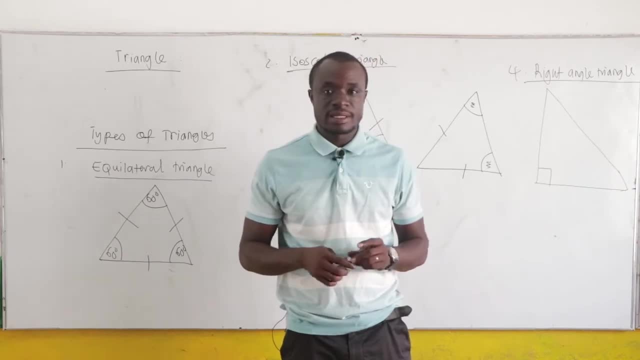 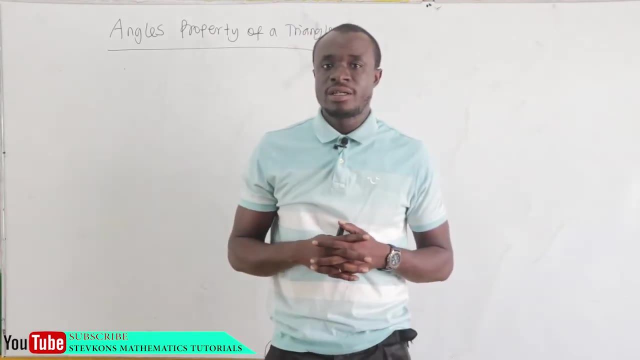 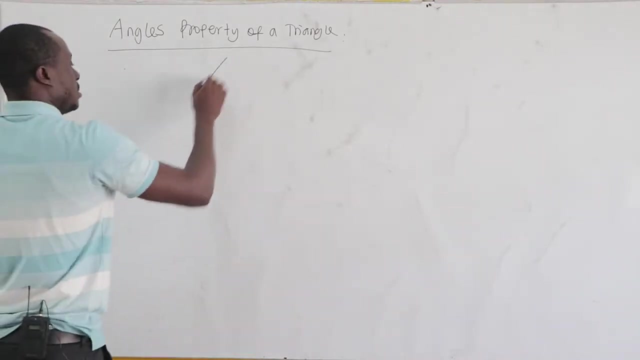 Now let's consider some examples for better understanding. Now we would like to look at angles property of a triangle. Now, the sum of angles in a triangle is equal to 180 degrees. So if we have a triangle, the sum of angles- so if this is A, the angle here is B. 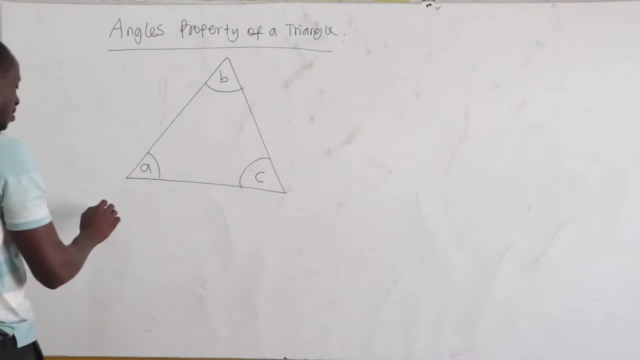 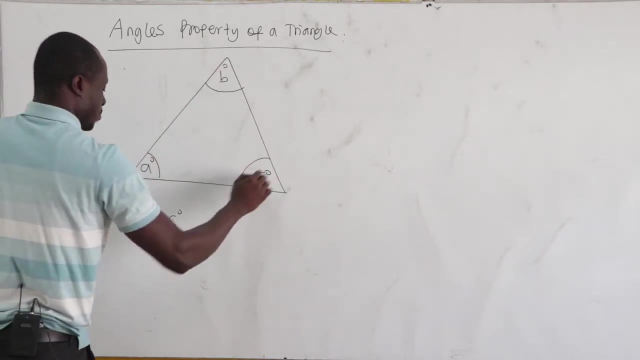 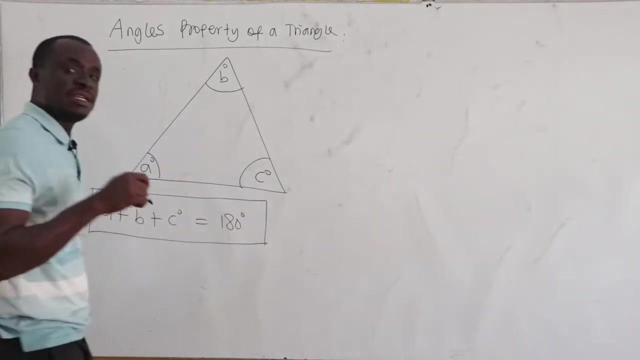 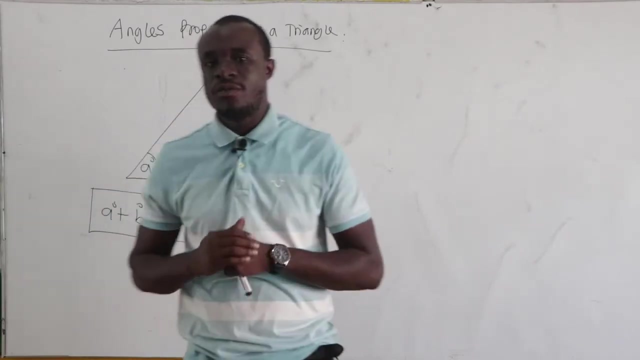 and then the angle here is C, Then all that you are seeing is that A plus B plus C is equal to 180 degrees. So sum of angles in a triangle is equal to 180 degrees. Let's consider some examples for better understanding. 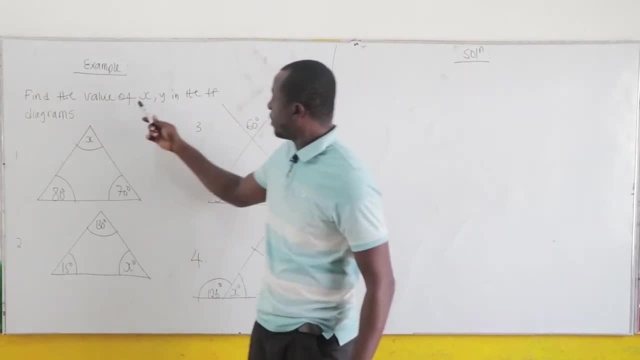 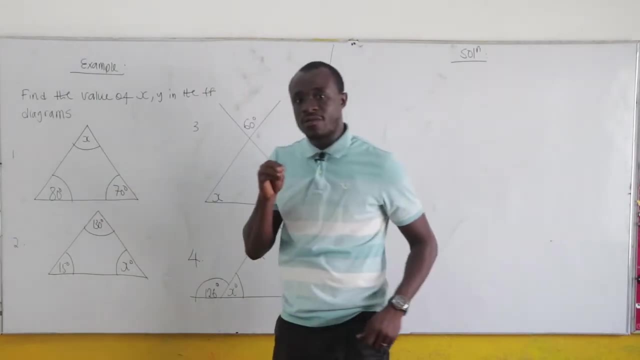 Now let's consider the following examples. The first one: find the value of XY in the following diagrams. One: we have X, 80 degrees, 70 degrees. Now, this is a triangle, and sum of angles in a triangle is equal to 180 degrees. Hence, 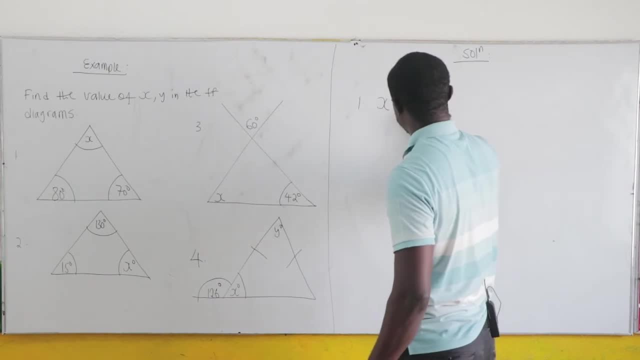 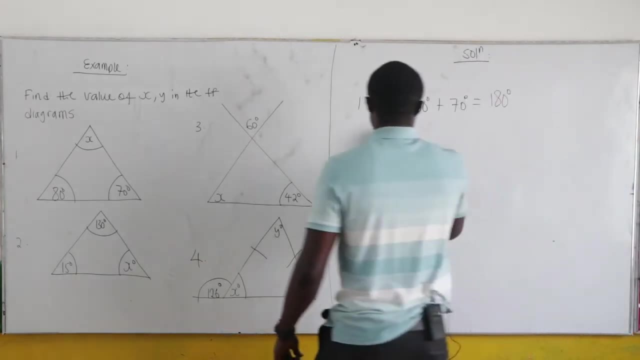 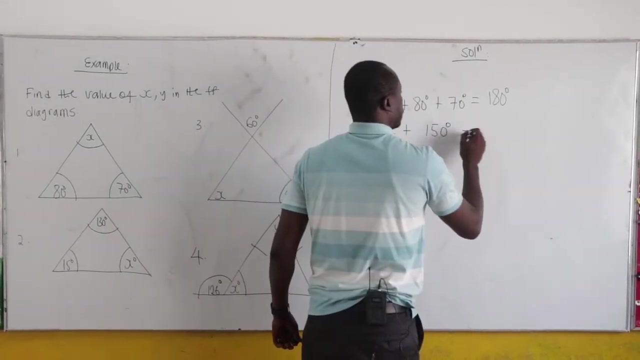 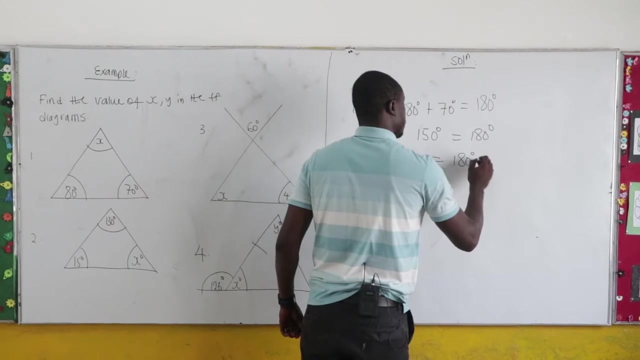 the first one, the angle X plus 80 degrees plus 70 degrees. So let's consider the expression for the triangle degrees. this is equal to what? 180 degrees? now we have x. what is 80 plus 70? that is 150 equal to 180 degrees. if we want to find our x group, like terms: 180 degrees. 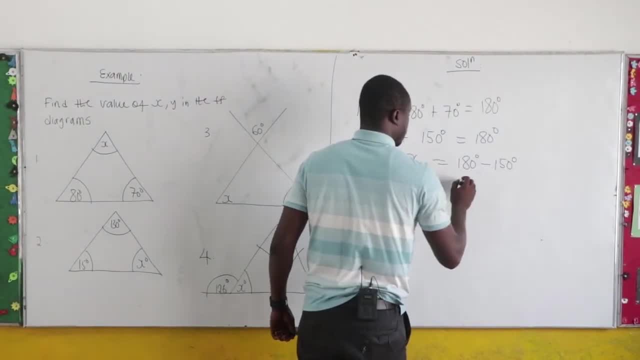 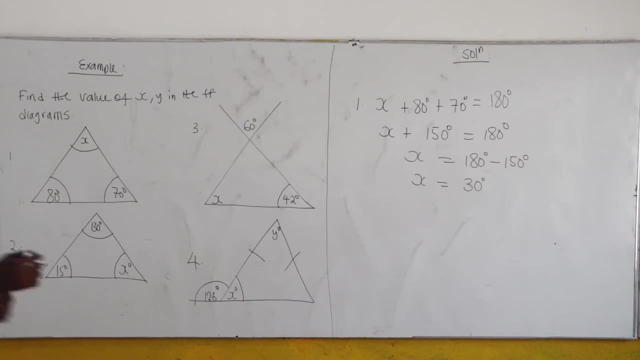 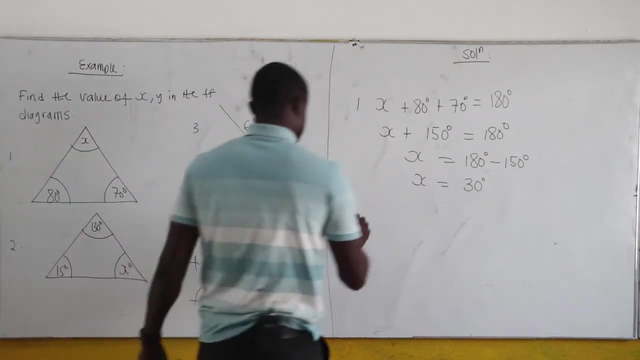 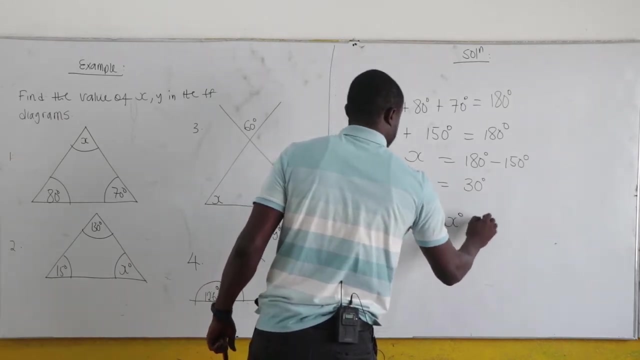 minus 150 degrees, and then our x is equal to 30 degrees. now let's see the second one. so the second one. we have a triangle, sum of angles in a triangle equal to 180 degrees. so we have 15 degrees plus 130 degrees, plus x degrees equal to 180 degrees. now, 15 plus 130, this is 145. 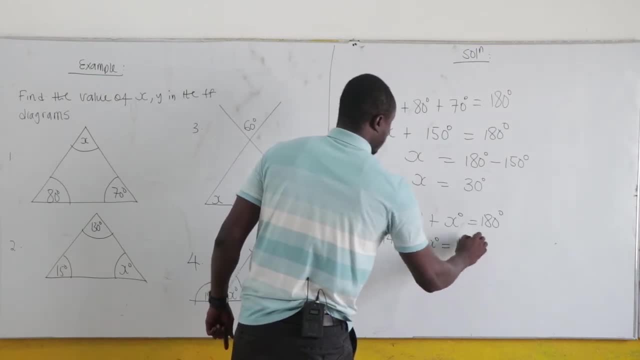 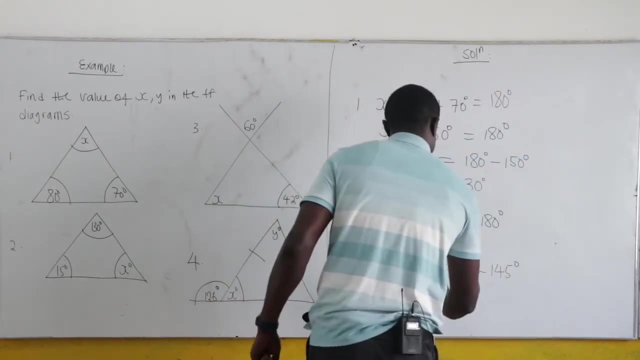 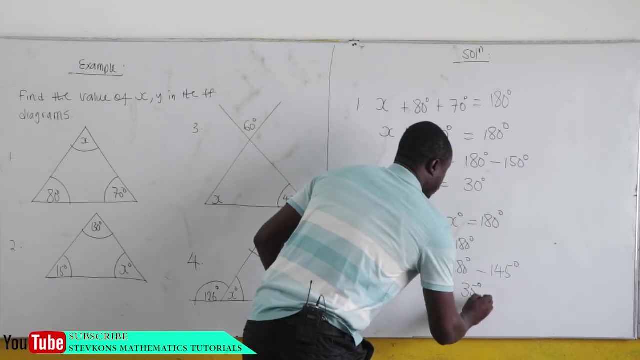 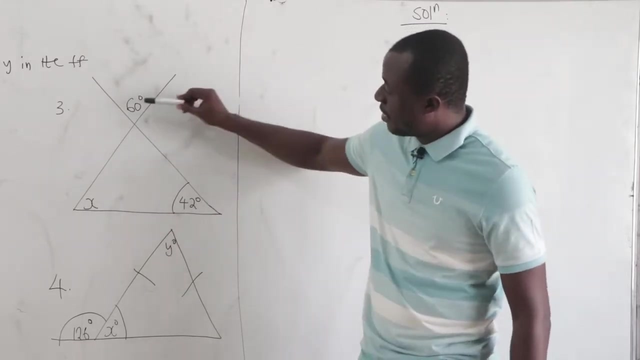 degrees plus x degrees, equal to 180 degrees. so x is equal to 180 degrees minus 145 degrees degrees. and what is 180 minus 145 degrees? this is just, that is 35 degrees. now let's see the third question. so you have x degrees here, 42 degrees here. now the angle here is vertically opposite. 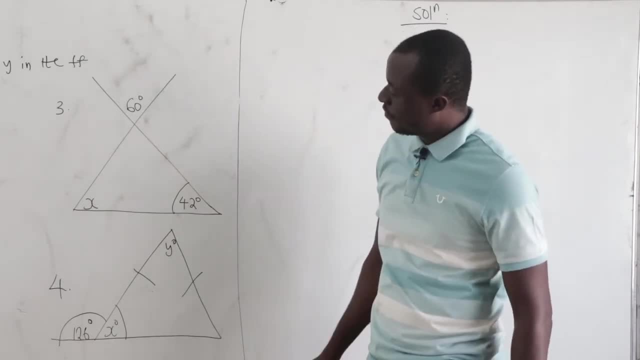 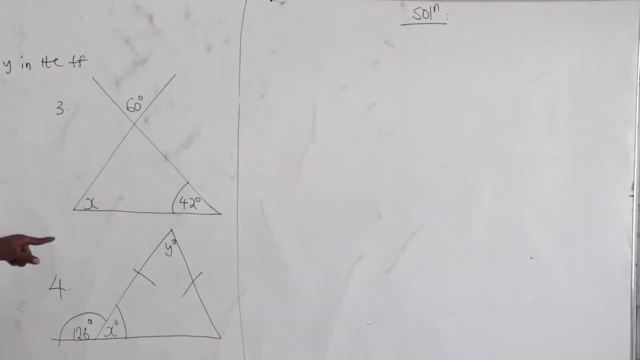 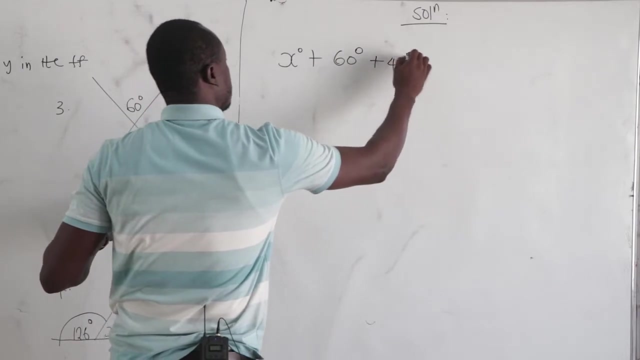 to the angle here, because this is straight line. this is straight line, so vertically opposite angle, so clearly this side becomes 60 degrees. sum of angles in the triangle is equal to what? 180. so x degrees plus 60 degrees plus 42 degrees, equal to 180 sum of angles in a triangle. 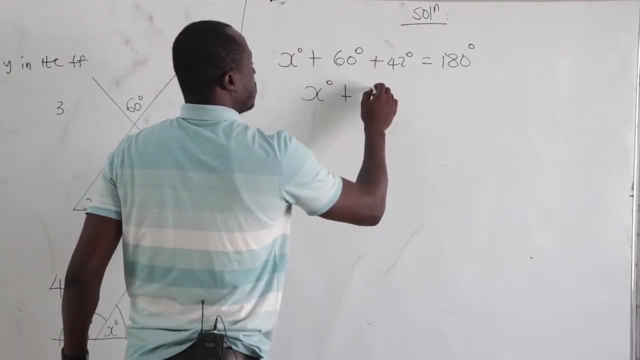 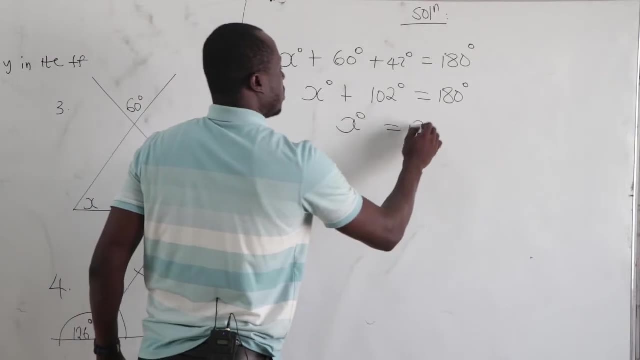 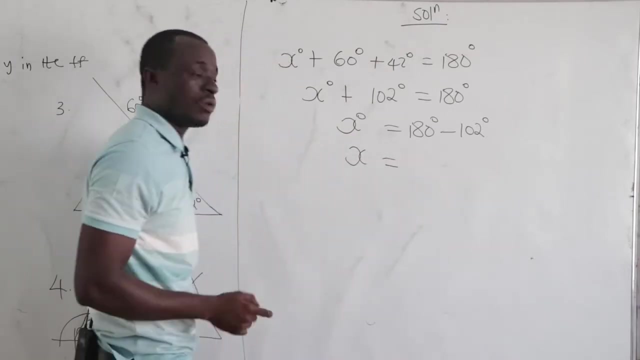 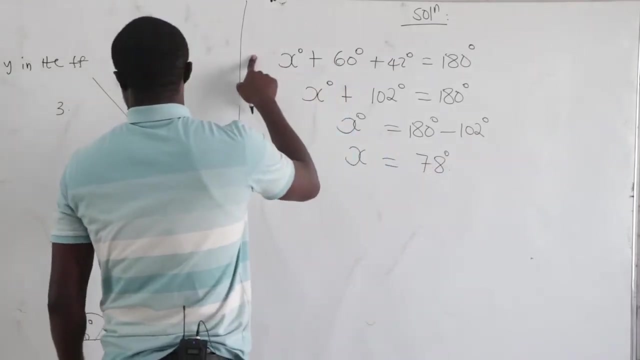 now we have x degrees, 60 plus 42. this given out, that is 102 degrees, equal to 180 degrees. once find x degrees, we have 180 degrees minus 102 degrees and this is just equal 180 minus 102. this is giving us that is 78 degrees. so that's question number three. now let's see question number four. 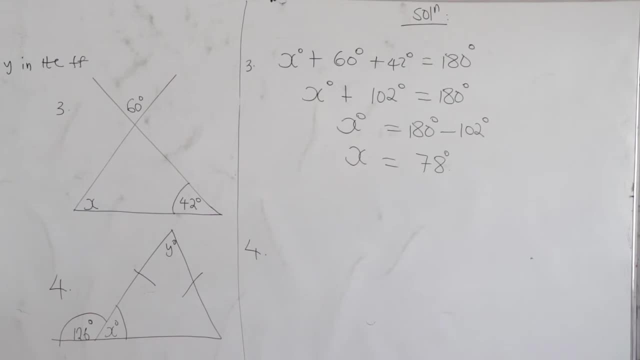 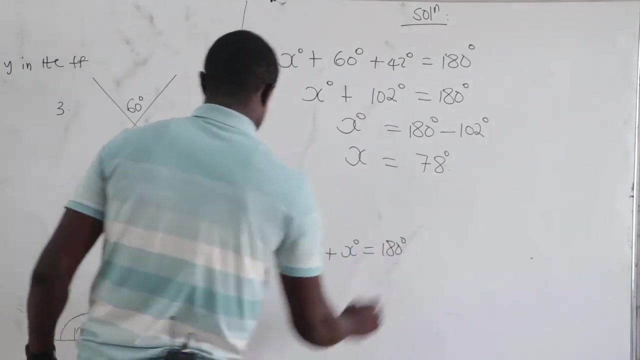 question number four: we can see isosceles triangle. the base angles are equal. now what can we see here? this is a straight line. this is a straight line. so angles on the sum of angles on a straight line at a point equal to 180 degrees. so what can we see? we can see that 126 degrees plus x degrees equal to 180 degrees. 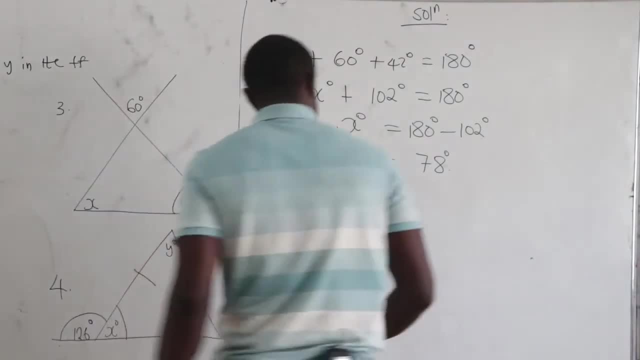 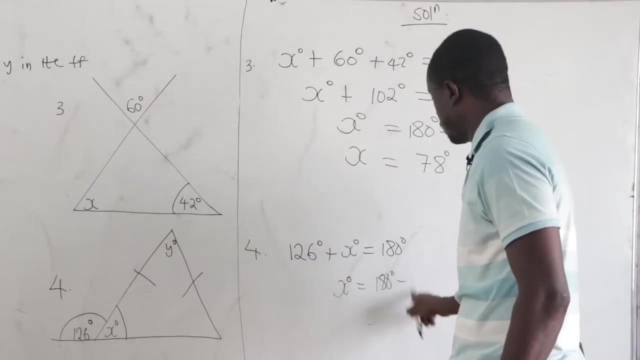 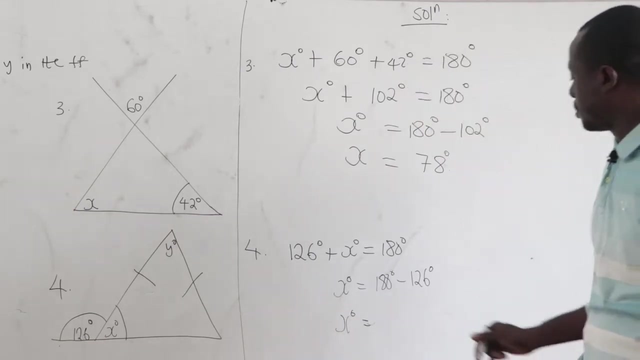 why some of angles on a straight line equal to that. now, from here, what is our x? we have our x degrees, equal to 180 degrees minus 126 degrees. now x degrees is equal to 180 degrees. so we have what is 180 minus 126 and it's giving us that is 54 degrees. now, if this is 54, 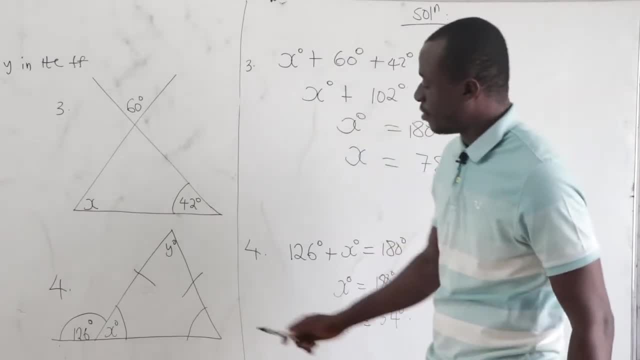 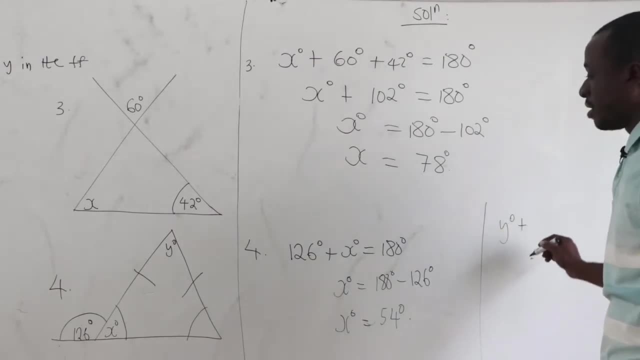 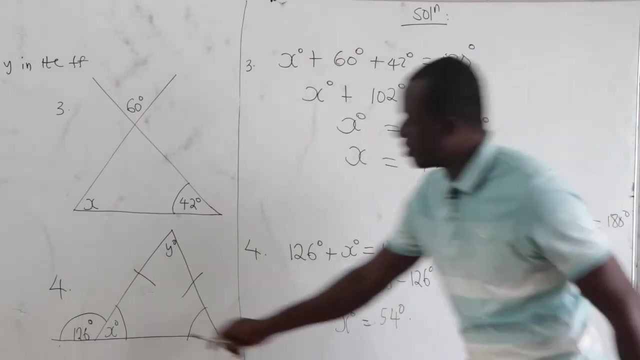 degrees. hence the angle here also would be what? 54 and sum of angles in a triangle is equal to 180 degrees. so you can say that Y degrees plus, that is, X degrees plus X degrees, equal to 180 degrees. if this is X, this is what X now. 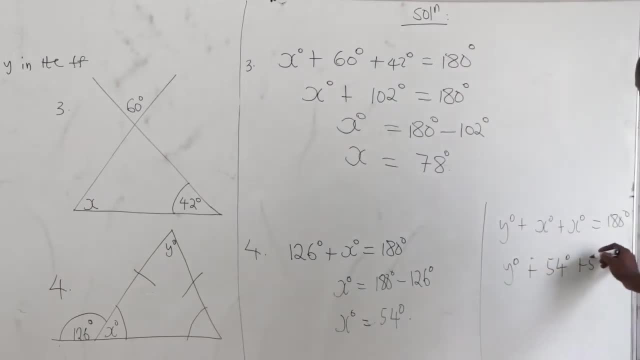 you know X. what is X? 54 degrees plus 54 degrees, equal to 180 degrees. Y degrees now 54 plus 54, that is 108 degrees equal to 180 degrees. so Y degrees equal to 180 degrees minus 108 degrees. clearly, our Y degrees equal to 72 degrees, and this is 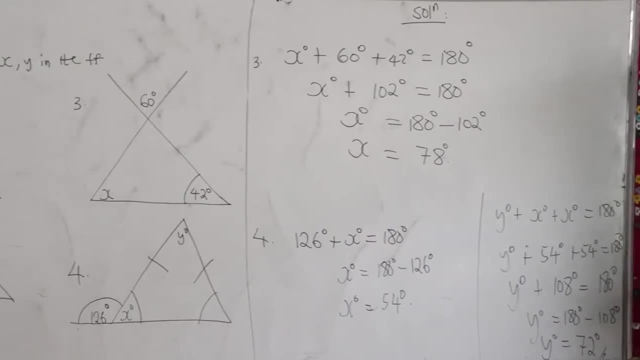 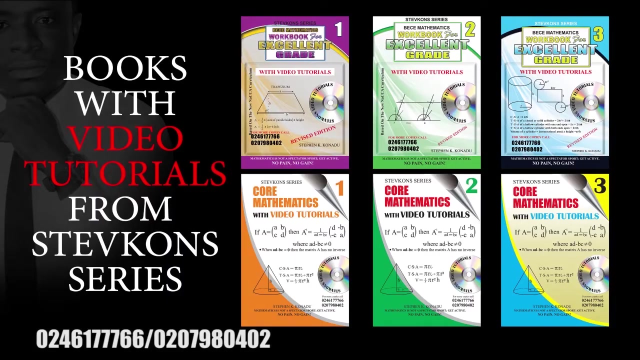 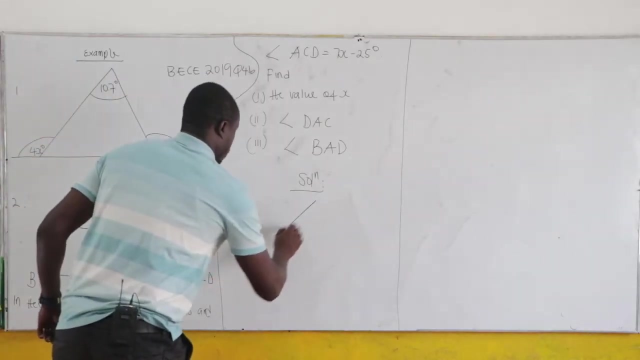 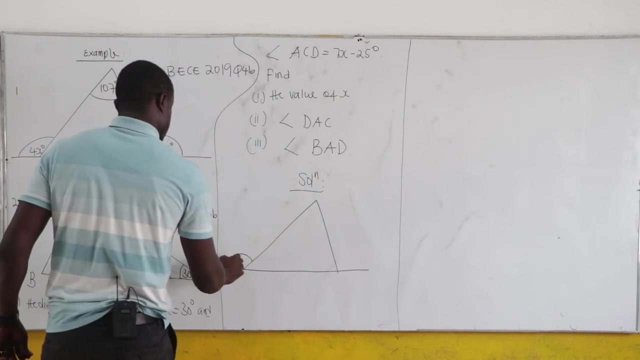 very, very easy. so Y degrees equal to 180 minus 108, this is just 72 degrees. let's consider the following pass questions. the first one: now let's redraw, so we have a triangle. now the自由 angle over here is giving us 4 X. 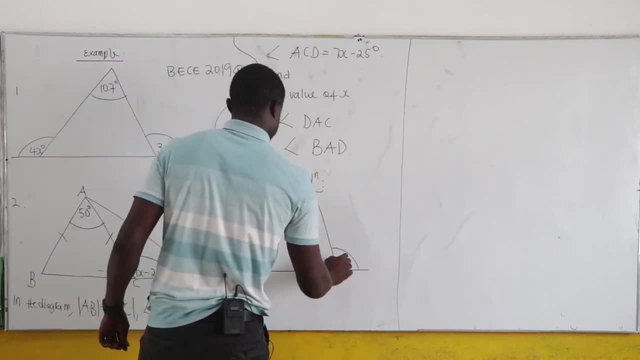 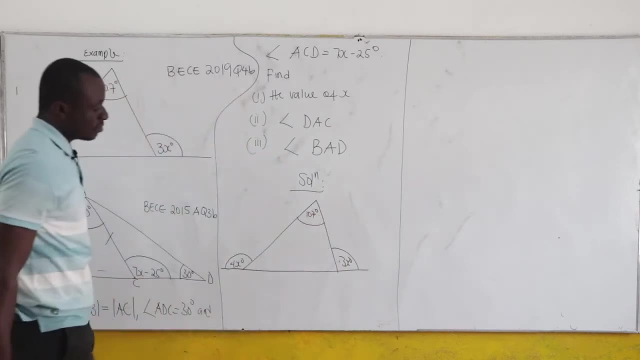 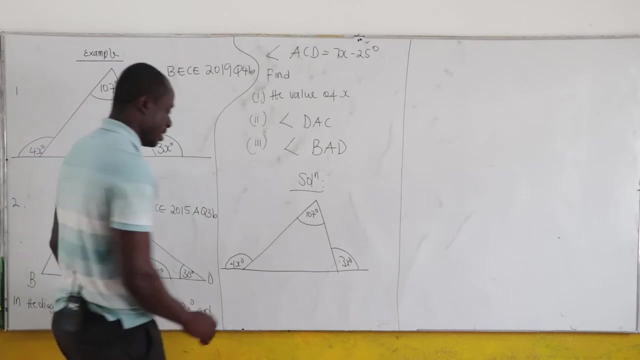 degrees. now the angle over here is exactly. It's also 3x degrees, So here is 107 degrees. Now we know we have a triangle And if we can load some of the interior angles, we know this is equal to 180.. 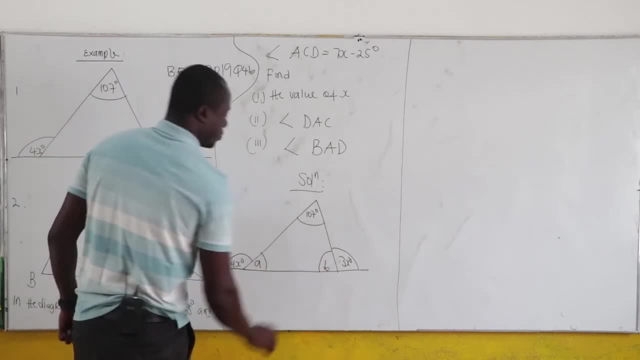 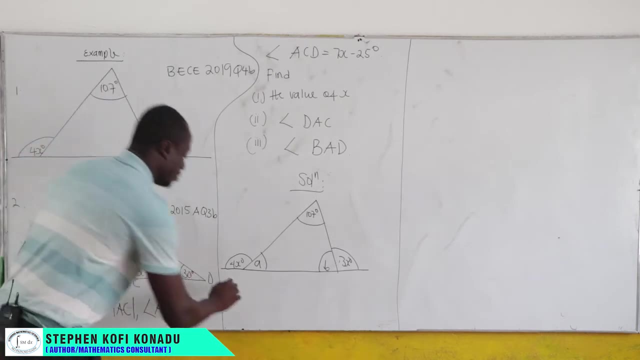 So let's suppose that this is A and then this is also B. Now this is a straight line. Some of the angles on the straight line at the point is equal to 180.. So our A plus 4x degrees is equal to 180.. 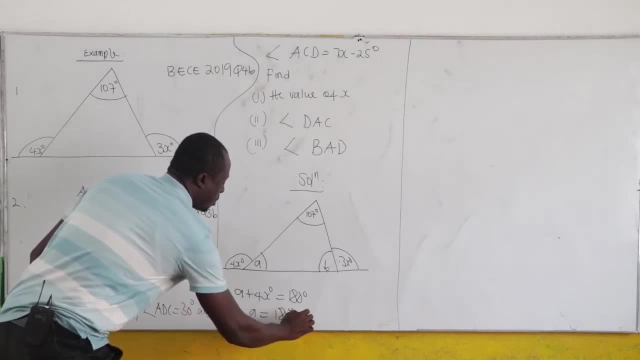 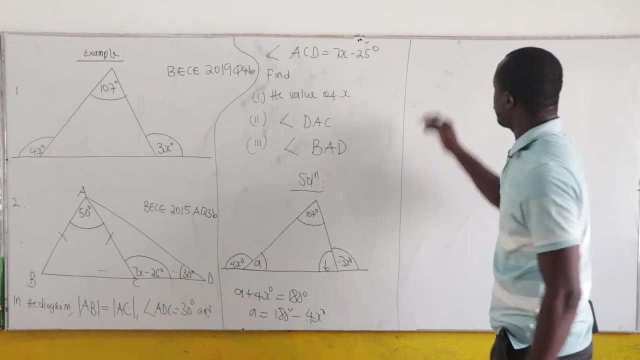 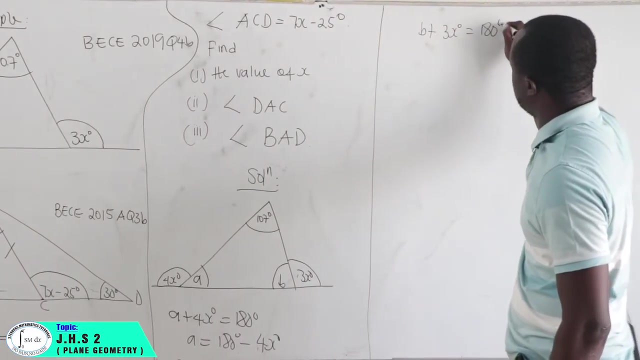 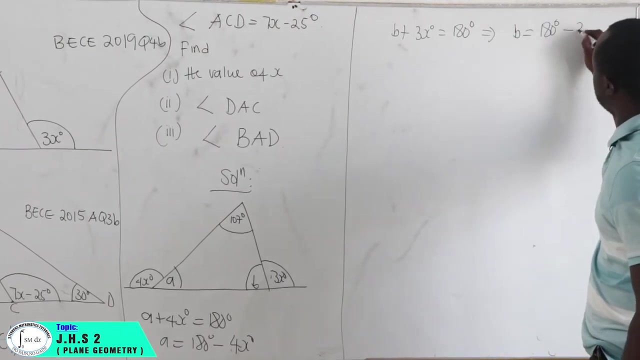 Clearly, our A is 180 degrees minus 4x degrees. Now, similarly, this side too, B plus 3x degrees, is equal to 180 degrees, And this implies that B is equal to 180 degrees minus 3x degrees. 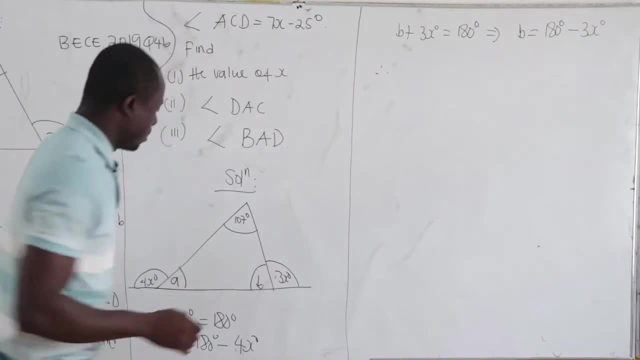 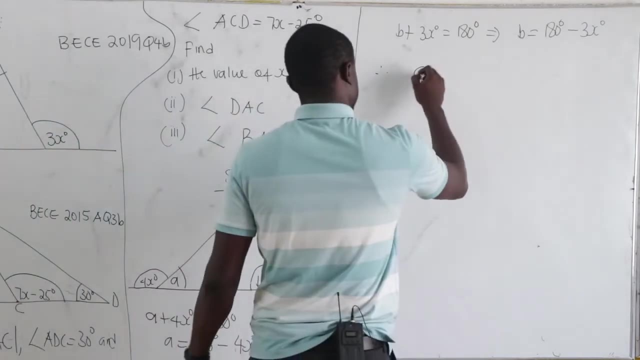 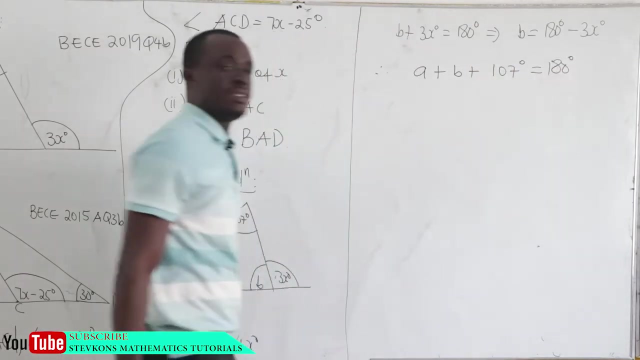 Hence now let's see. So we know the angle here, We know the angle here. Now, sum of angles in a triangle is equal to 180.. So A plus B plus 107 degrees is equal to 180 degrees. Now, what is the A? 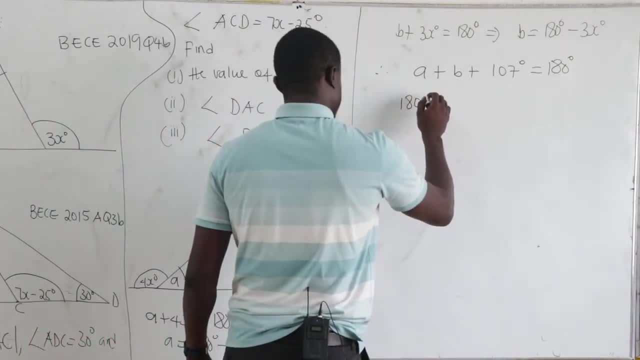 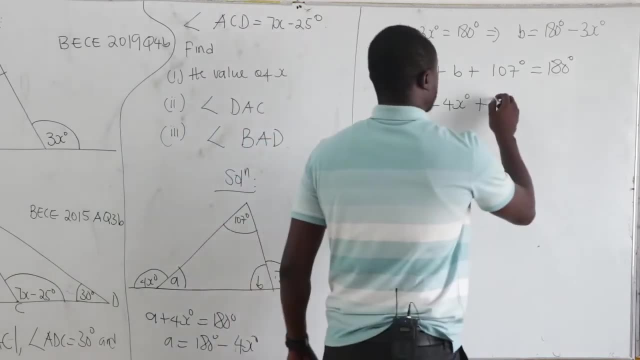 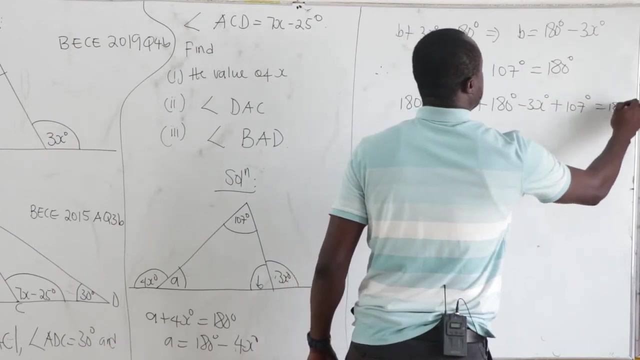 Our A is 180 degrees minus 4x degrees. What is our B? What is our B? Our B is also 180.. So our B is also 180 degrees minus 3x degrees. plus 107 degrees is equal to 180 degrees. 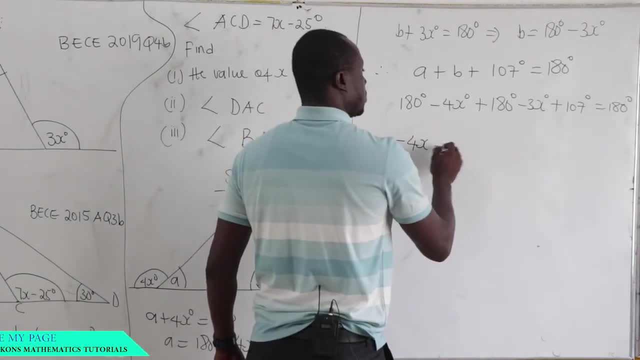 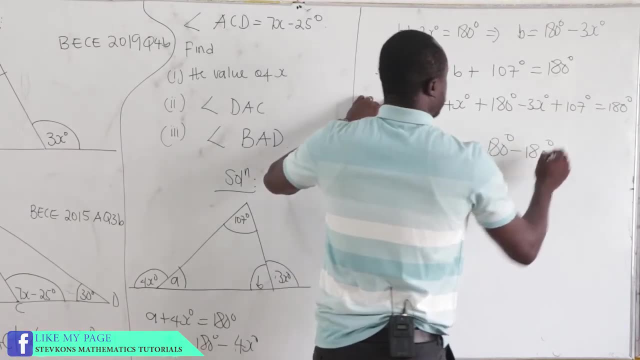 Now let's group like them, So we have negative 4x minus 3x. Let's take everything to the side, So we have 180 degrees minus 180 degrees minus 180 degrees. This is also going minus 107 degrees. 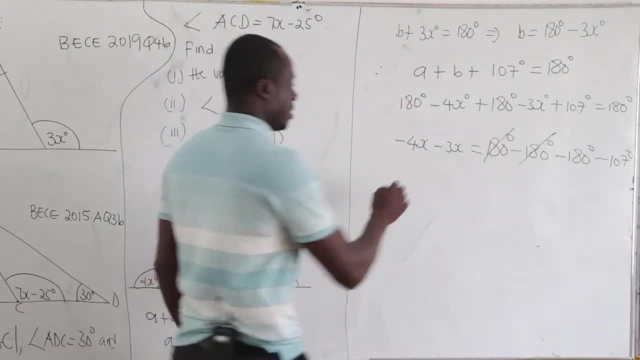 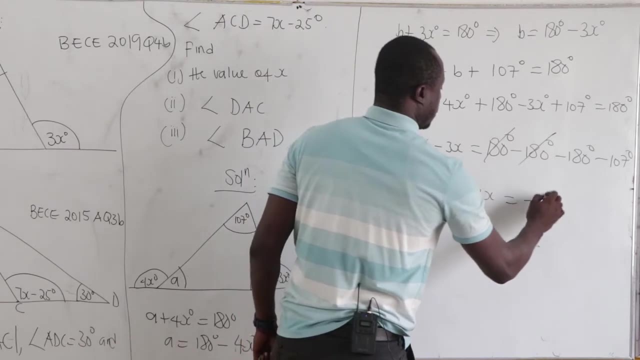 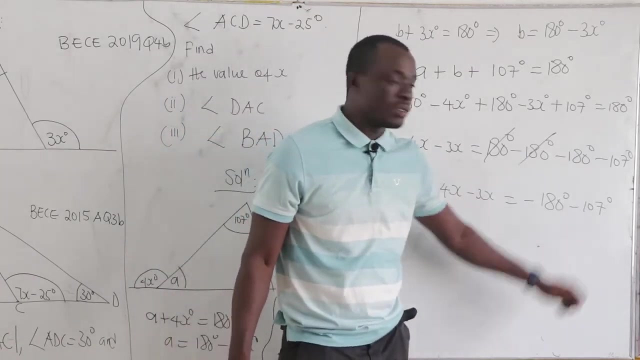 Clearly, what can we see? This and that is canceling out. So we have 180.. Negative 4x minus 3x. And then we have negative 180 degrees minus 107 degrees. Now, negative 180 minus 107.. 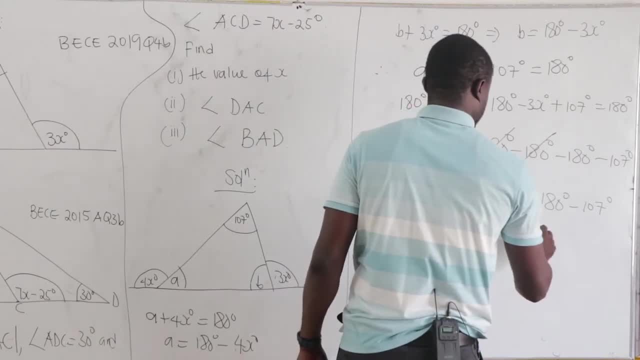 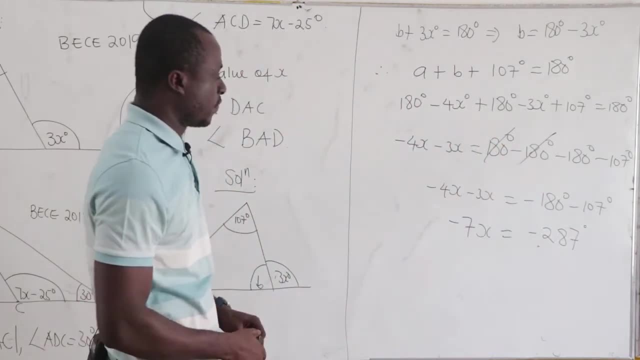 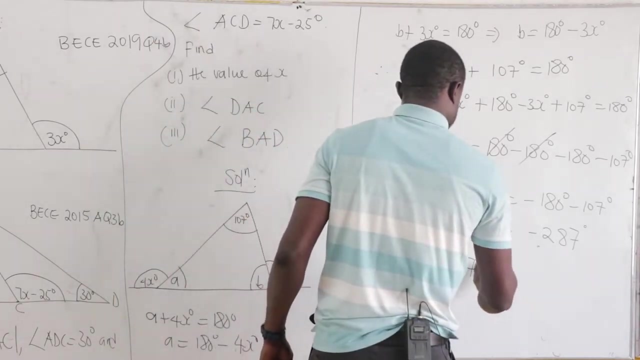 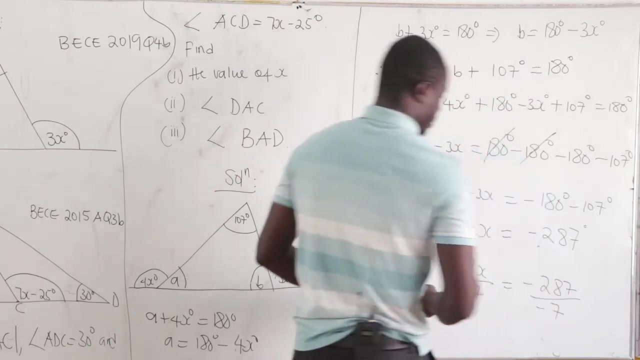 This is 287.. So we have negative 7x equal to negative 287 degrees. Now we want to find x, So we divide by what is multiplying the x. So clearly, negative 7x over negative 7 equals negative 287 all over negative 7.. 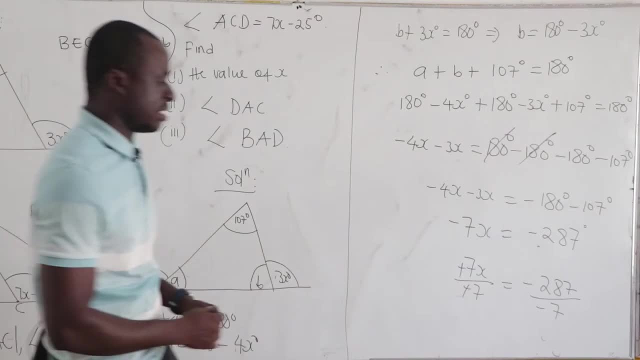 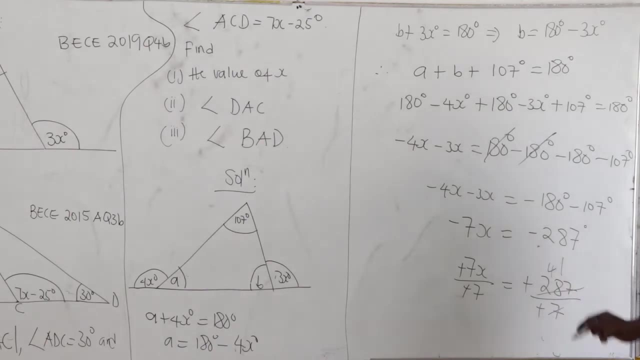 Now this is canceling out that. Now this is canceling out this. How many times does 7 go into 28?? That is 4.. 7 goes into 7.. That is 1.. So you have x to be equal to 41 degrees. 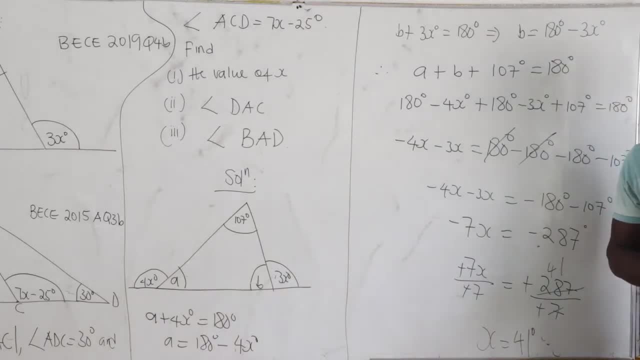 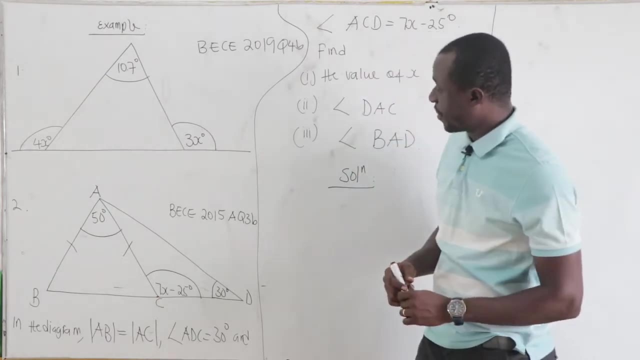 I believe you enjoyed it. This is something that is very, very easy. Now let's consider the second one. This is a past question B, C, 20, T 15.. Question number 3B: Now, this is the diagram we have. 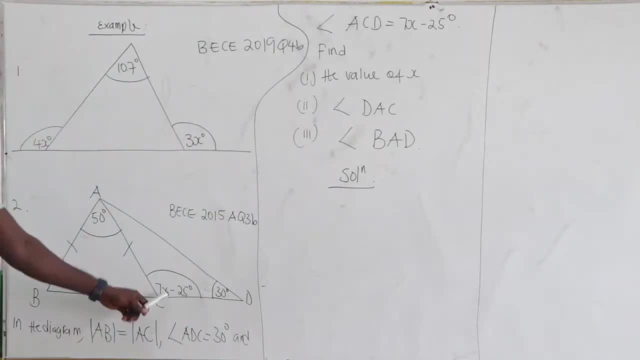 And then the first one says that we should find the value of x, And we know x is somewhere here. Now we can see we have. that is triangle ABC. This is an isosceles triangle, So the angle here is the same as the angle over there. 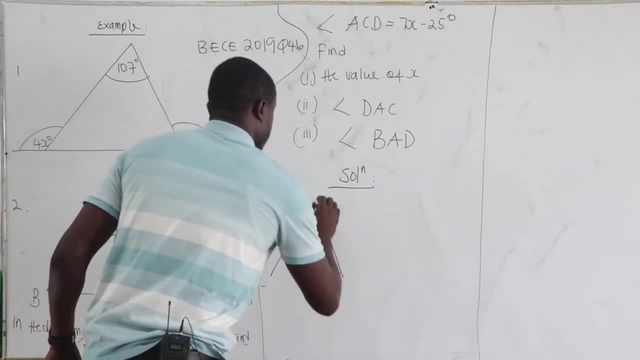 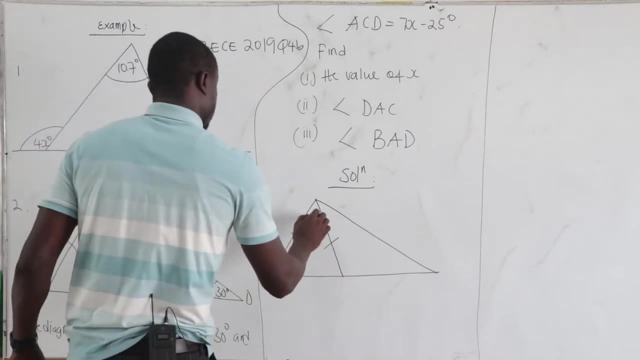 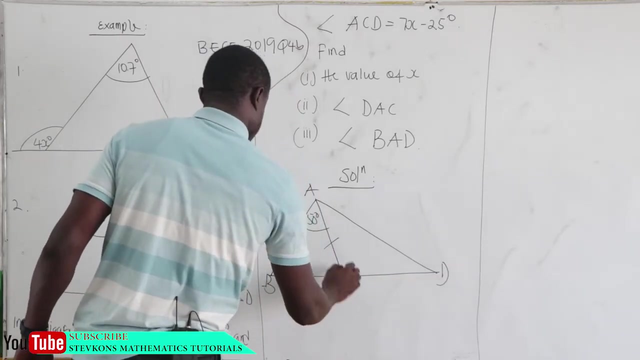 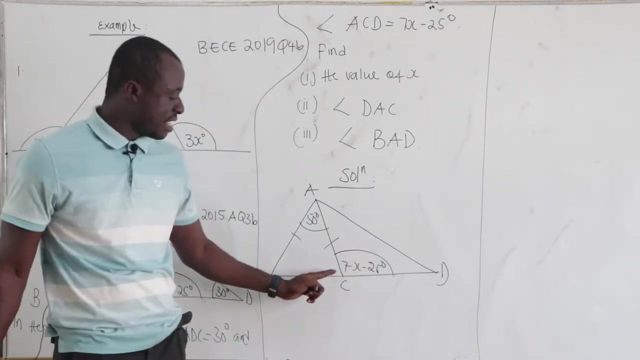 Now let's redraw this over here. Now this side is equal to that side. This is 50 degrees. Now we have B here, A, D and then C. This is 7x minus 25 degrees. Now, because there's x here, I shouldn't put x and x in it. 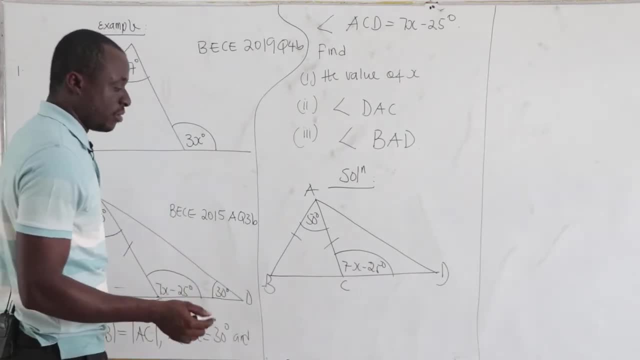 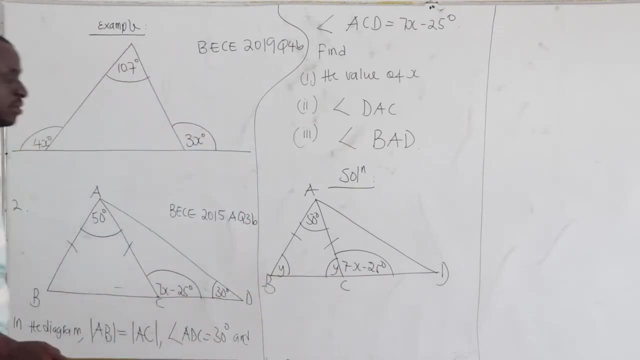 I can put any other variable, but not x. So here let's suppose that I can put y here, If this is y, and then the angle here too is y. Now, sum of angles in a triangle equals 180.. 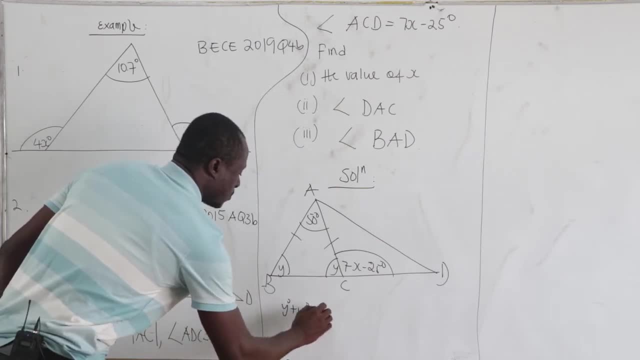 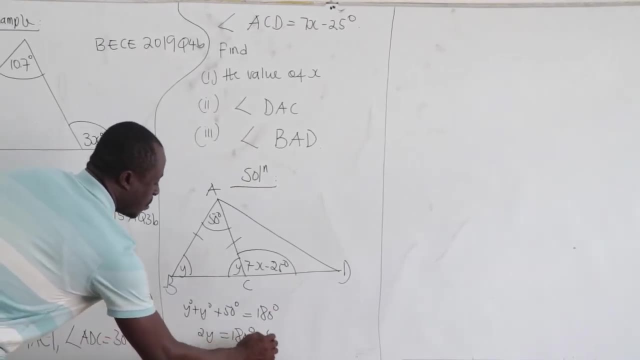 So I can say that y plus y degrees plus 50 degrees equal to 180.. Now 2y equals 180 minus 50 degrees. y plus y, that's 2y, And then this will go as 180 minus 50.. 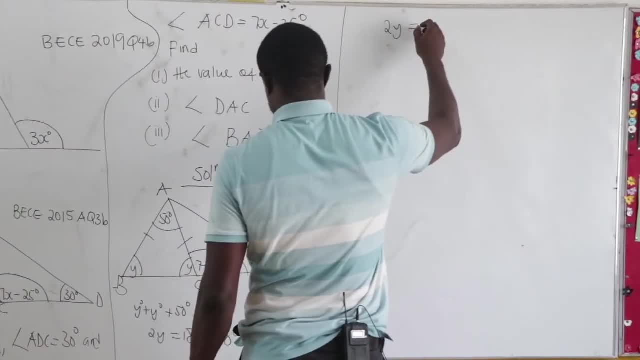 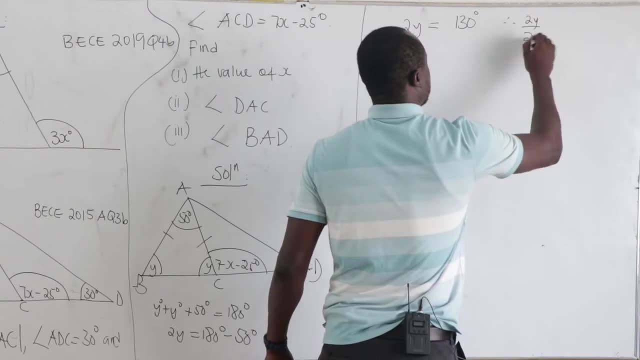 Now, what do you have? So we have our 2y equal to 180.. So we have our 2y equal to 180 degrees. Therefore, we have our 2y over 2 equals to 180, all over 2.. 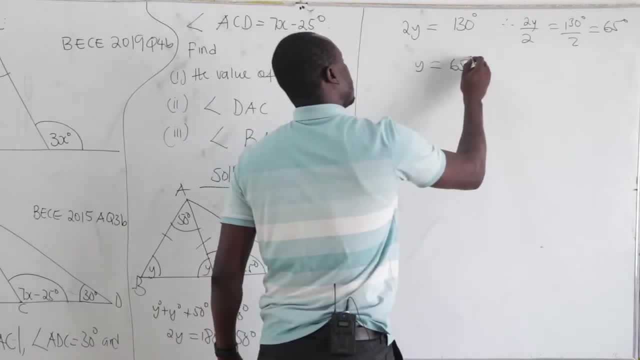 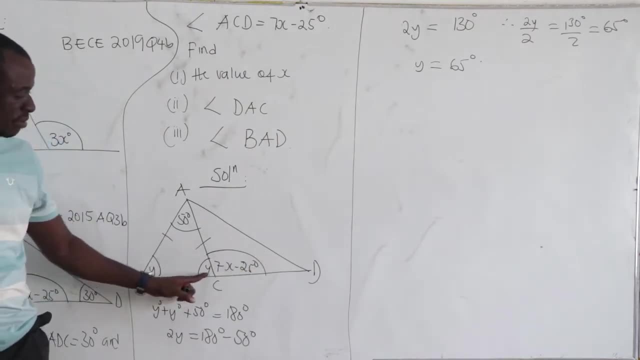 And this is giving us 65 degrees. So our y is 65 degrees. That's the value of y. Now we have a straight line over here Now, so sum of angles on the straight line equal to 180.. So 65 plus 7x, minus y. 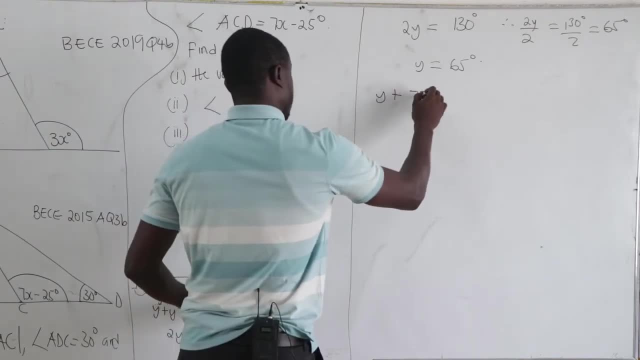 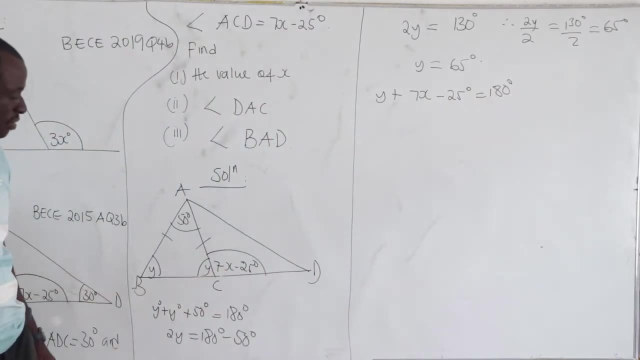 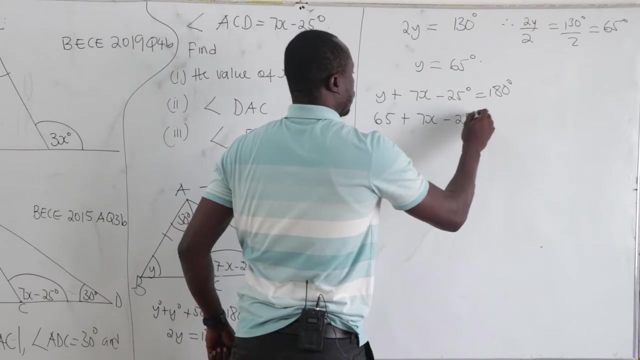 So that is y plus 7x Minus 25, equal to 180 degrees. Why: Sum of angles on the straight line equal to 180 degrees? What is y, y is 65. So we have 65 plus 7x minus 25 degrees, equal to 180 degrees. 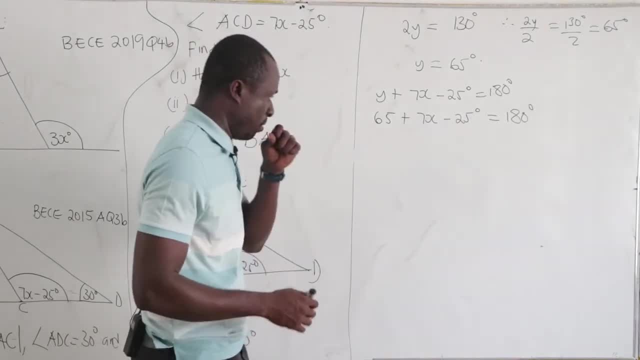 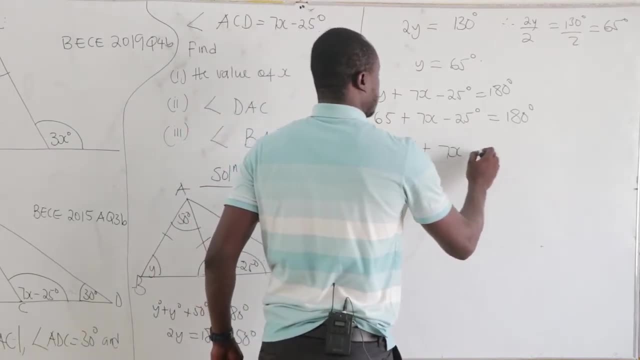 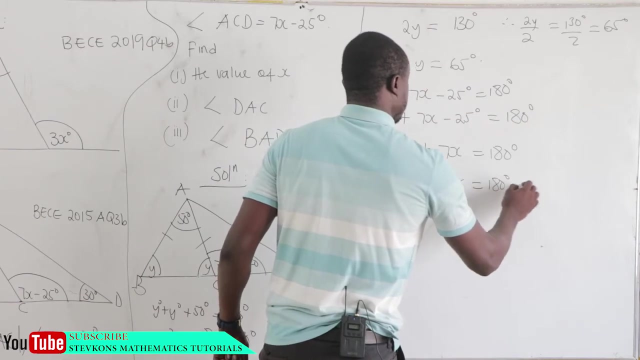 So 65 minus 25, this is 40 degrees plus 7x, equal to 180 degrees. Now, our 7x equal to 180 degrees minus 40 degrees, 7x. now what is 180 degrees minus 40?? 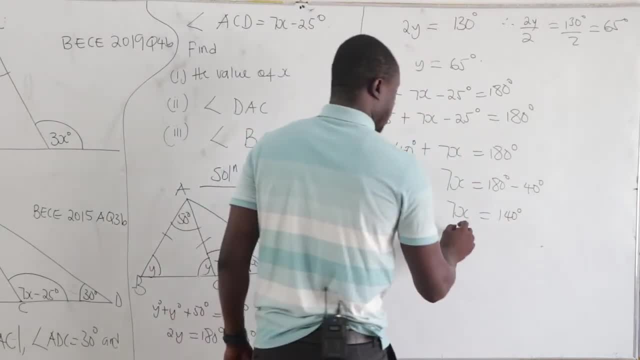 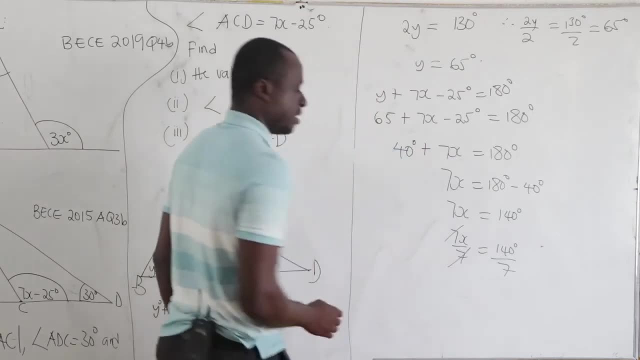 This is 140 degrees. I want to find x. So we divide both sides by 7.. So this is canceling out that Now 7 will go here, once 7 will go into 14.. That is 2.. 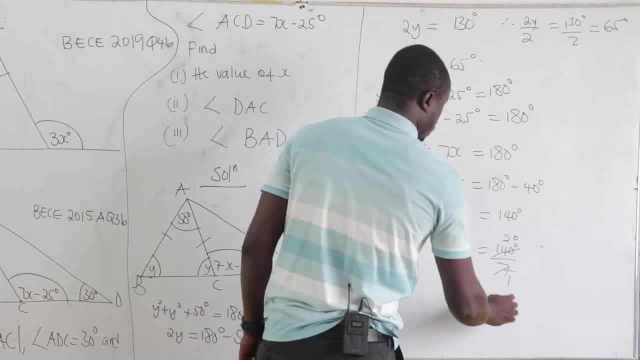 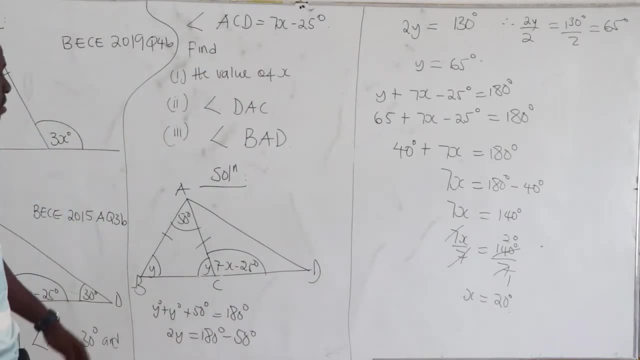 7 will go into 0. That is 0. So we have our x to be equal to 120 degrees. So our x is equal to 20 degrees. Now the second one says you find d a, c. 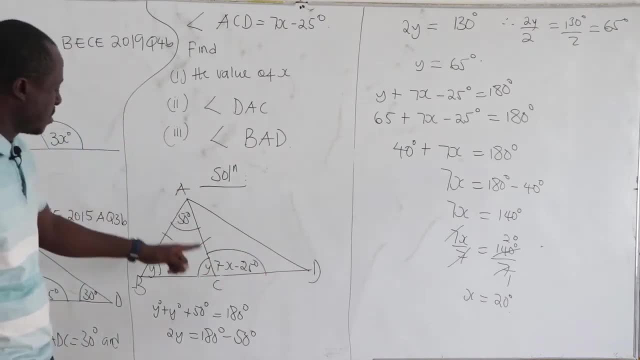 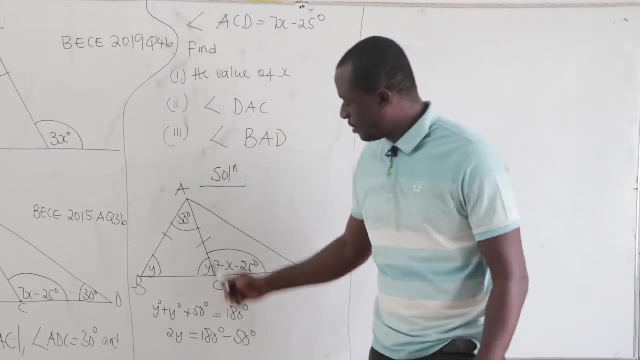 You want to find d a c. You want to find the angle over here. Now the second one says: you find d a c. Now what is the angle at d? The angle at d is 30 degrees. 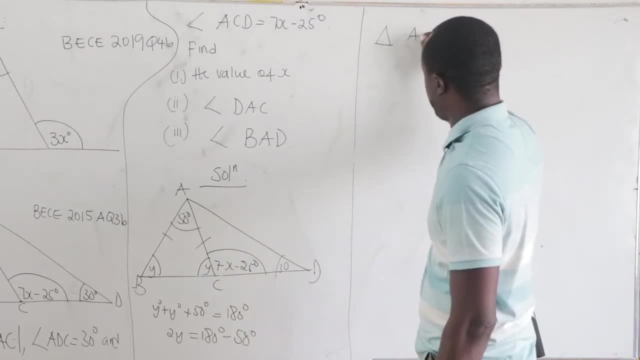 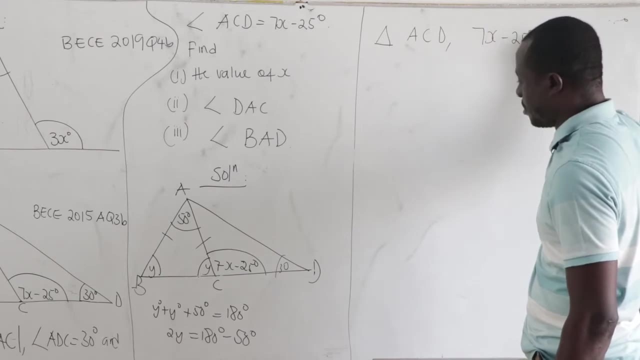 So when you consider that a triangle, a, c, d- sum of angles on this should be equal to 180 degrees, That is, 7x minus 25 degrees, plus 30 degrees, plus the angle that we are looking for, d a, c. 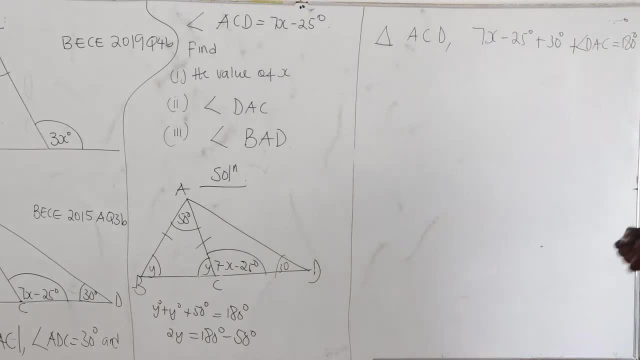 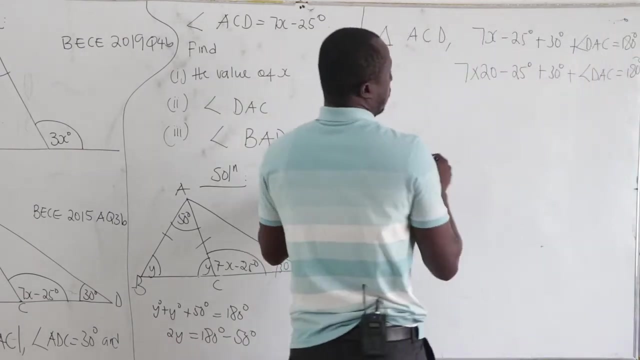 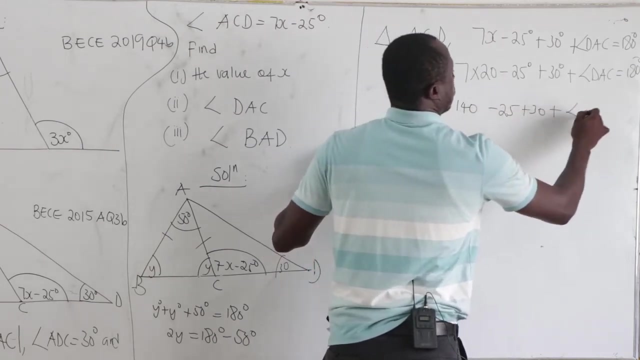 This is equal to 180 degrees. Sum of angles in a triangle equals 180.. Now what is x? We have x to be 20.. Now, 7 times 20, that is 140.. Now, minus 25 plus 30, plus d a, c equals 180 degrees. 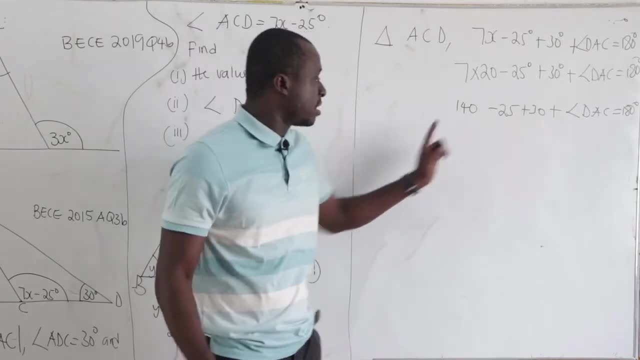 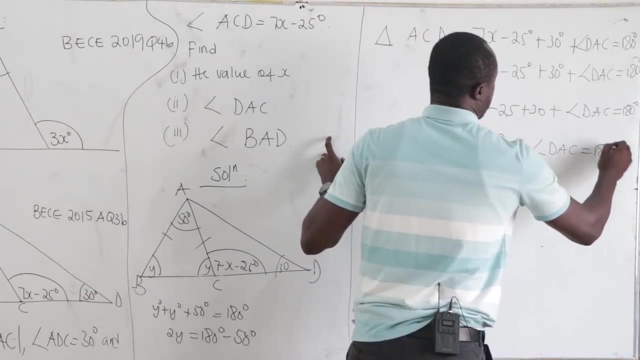 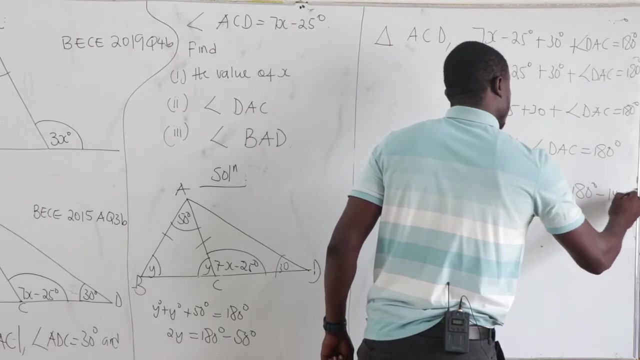 Now negative 25 plus 30.. That is 5 plus that, So this will be 145.. Plus d a c equals 180 degrees. Now, angle d a c equals 180 degrees minus 145 degrees. 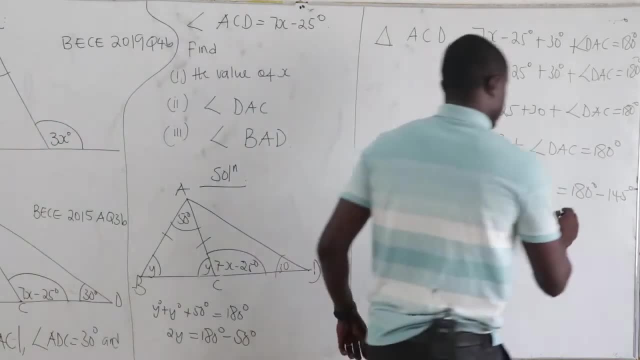 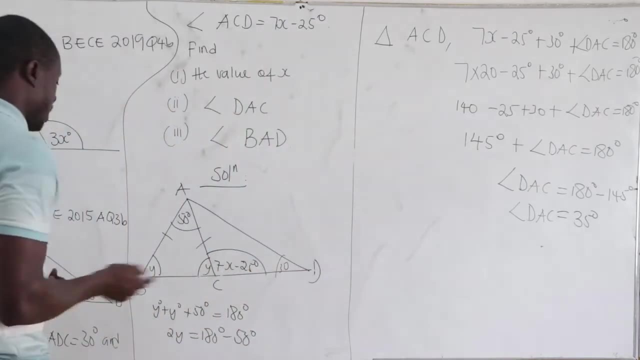 Now what is? 180 degrees Minus 145.. And this is just 35 degrees. So that is the second one. That is the second one. So i i Now let's see the third one, since we find b a, d. 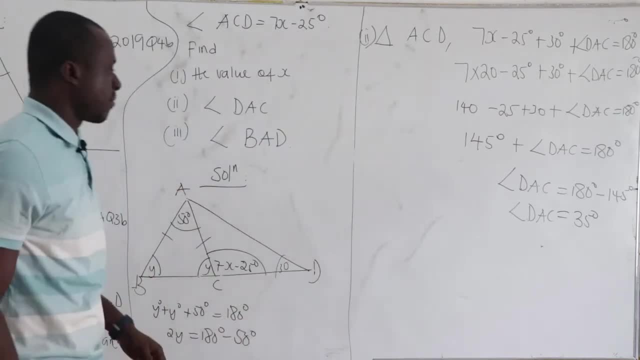 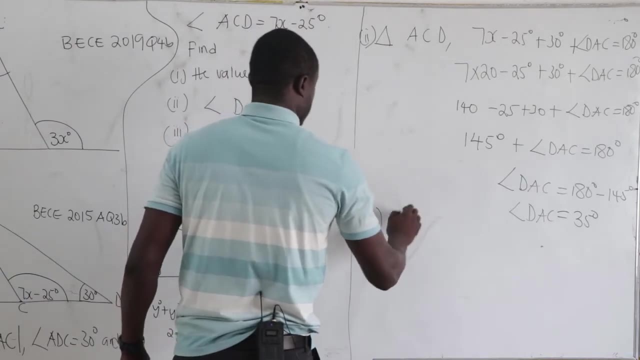 We want to find b a d, Now d a c. here we have it to be 35 degrees. So the third one: angle b a d, Angle b a d. What is the angle here? 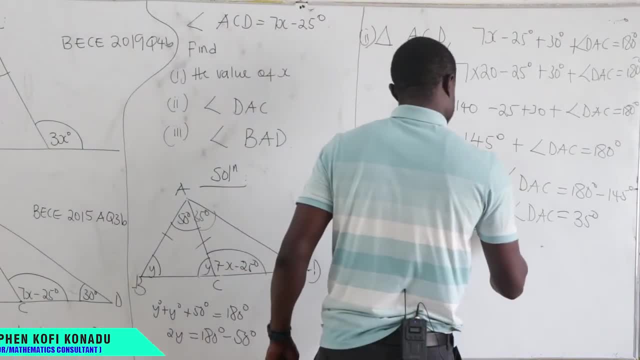 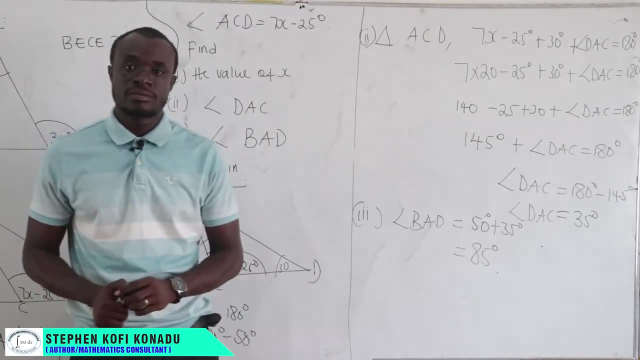 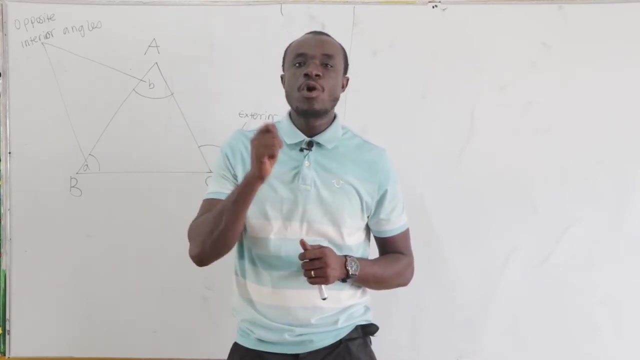 50? Plus 35. So that is 50 plus 35. And that is just 85 degrees. I would like to consider the next property Now. the next property says that the sum of the opposite interior angles is equal to the exterior angle. 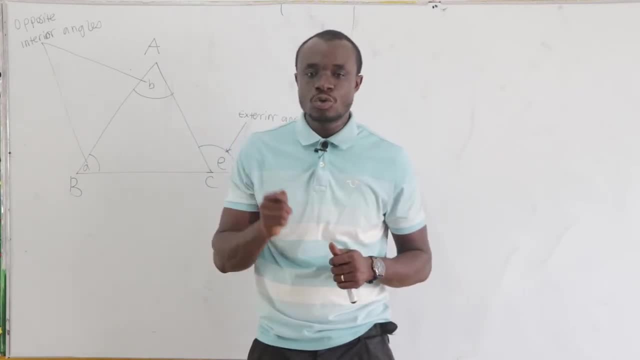 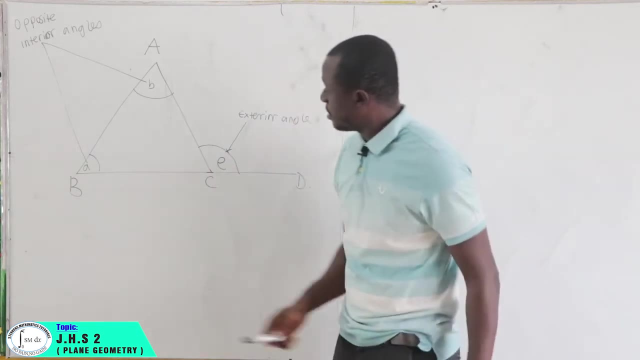 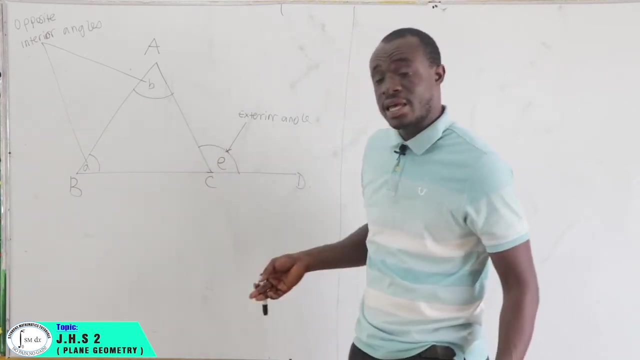 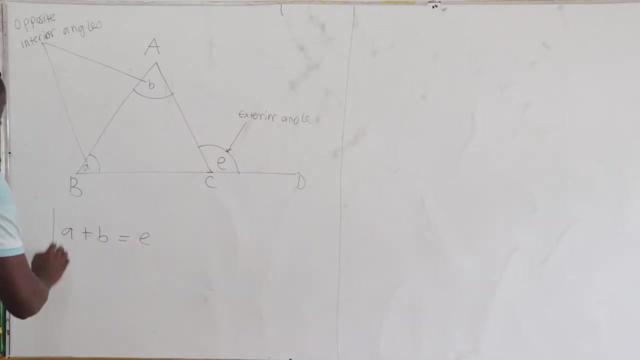 Let me take it again: The sum of the opposite two interior angles is equal to the exterior angle. So over here in this diagram, a and b is the opposite interior angles And then e is the exterior angle. So all that we are saying is that a plus b equal to e. 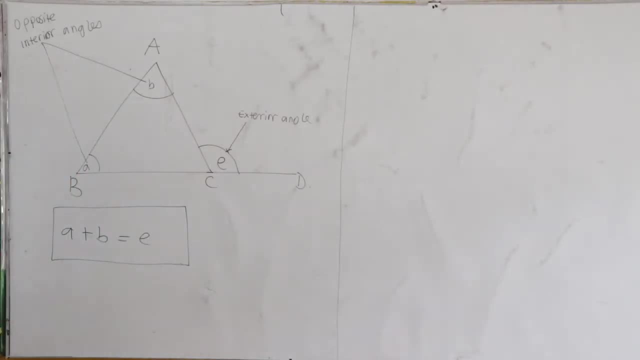 Please. this property is so important. It makes things so, so easier. The sum of the opposite interior angles is equal to what The exterior angle. The sum of the opposite two interior angles is equal to the exterior angle. So we are saying that angle a plus angle b is equal to e. 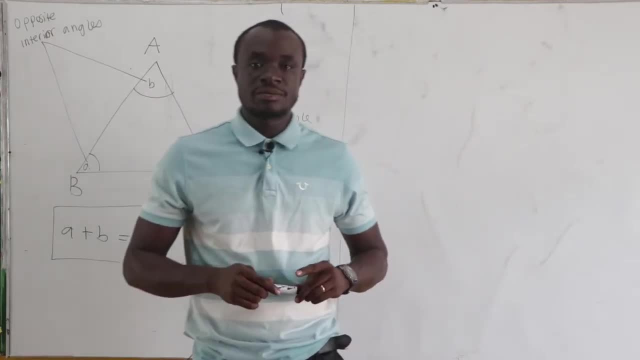 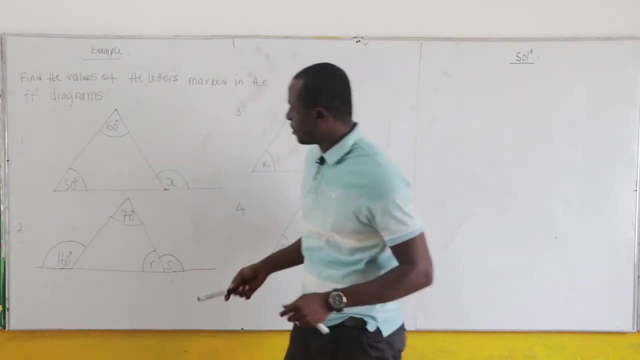 Let's consider some examples for better understanding. Now let's consider this example. Find the values of the letters marked in the following diagram, The first one we can see. okay, interior angles. we have an exterior angle. Now what do we know? 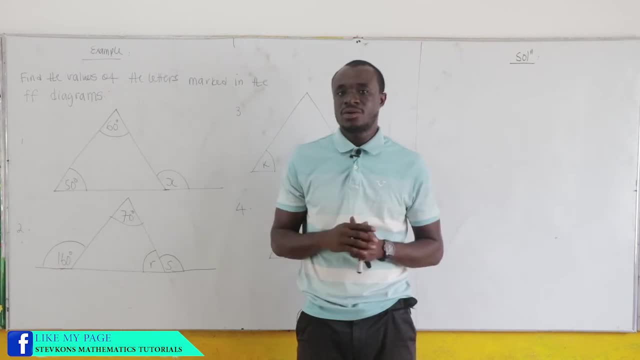 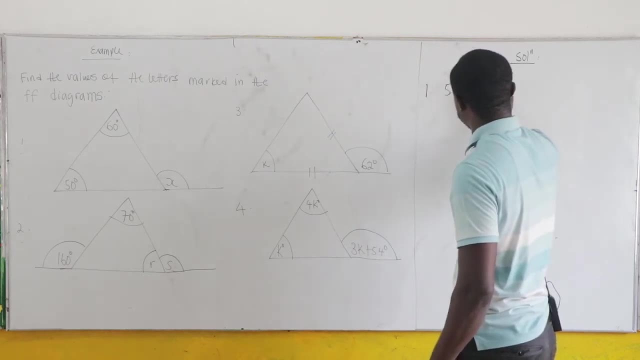 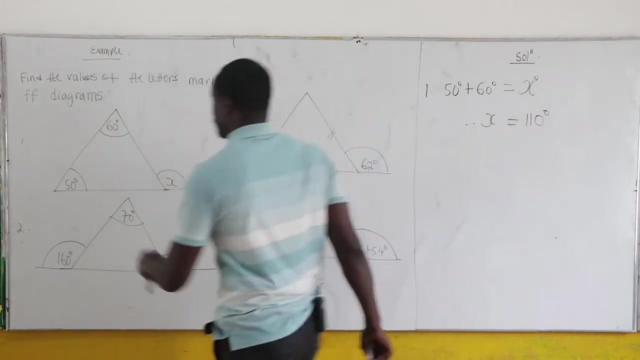 The sum of the two opposite interior angles is equal to the exterior angle, So with the first one just 50 degrees, plus 60 degrees equal to what X degrees? Hence our x is just 110 degrees. Why The angle here plus this angle, equal to that. 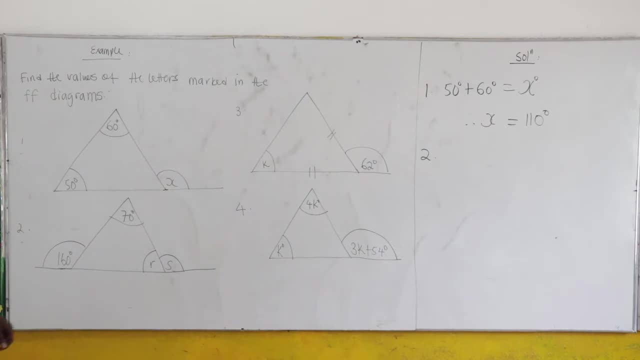 So our x is that. Now let's see the second one. Now let's see, we have two opposite interior angles, We have the exterior angle. So this plus is equal to what? 160 degrees from the property. So you can say r plus 70 degrees equal to 160 degrees. 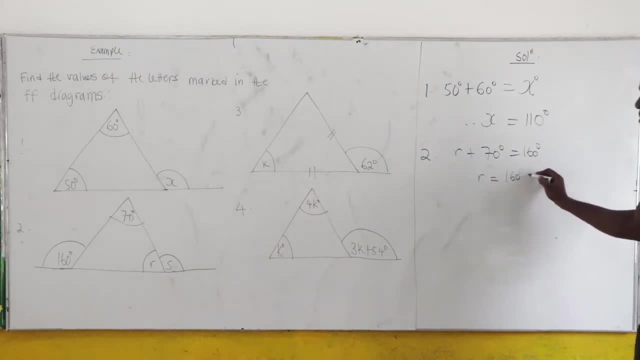 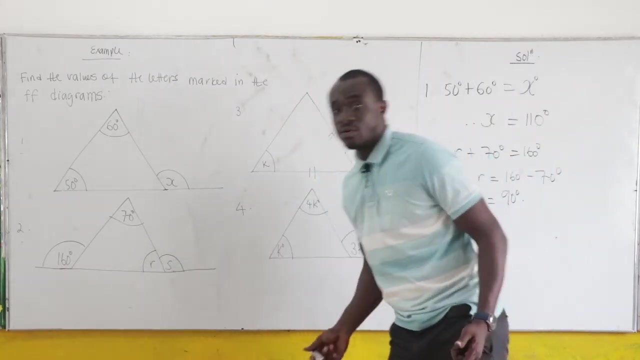 Now we have our r to be equal to what? 160 degrees minus 70 degrees. Our r will be equal to what, That is, 90 degrees. Now let's see Also, we have straight line over here. Sum of angles on the straight line equal to what? 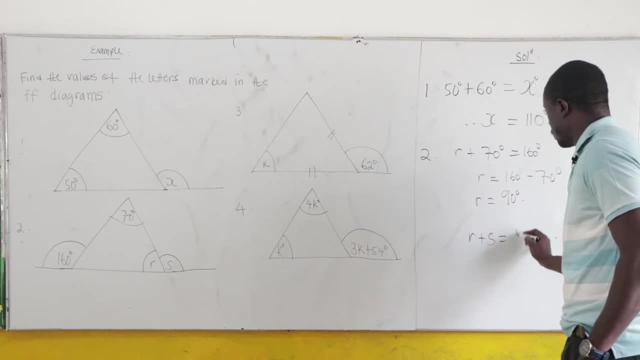 180.. So you can say r plus x, equal to 180 degrees, Our r is 90. So we have 90 degrees plus x, equal to 180 degrees, S, equal to 180 degrees minus 90 degrees. Our x is that is 90 degrees. 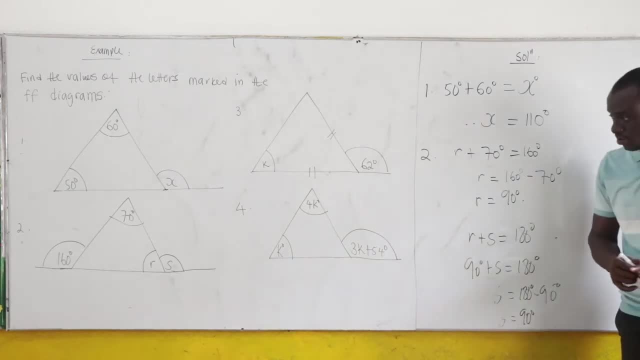 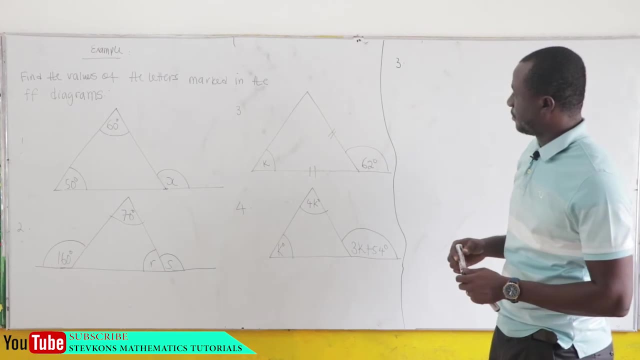 Why 180 minus 90?? This is what 90 degrees Remember. all these are not drawn to scale. Now let's see the third one. Now, what type of triangle is this? This is isosceles triangle. 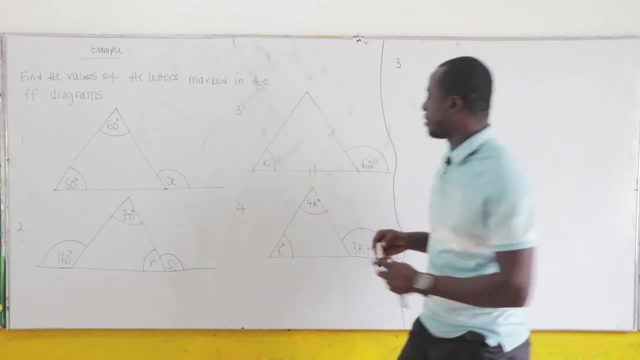 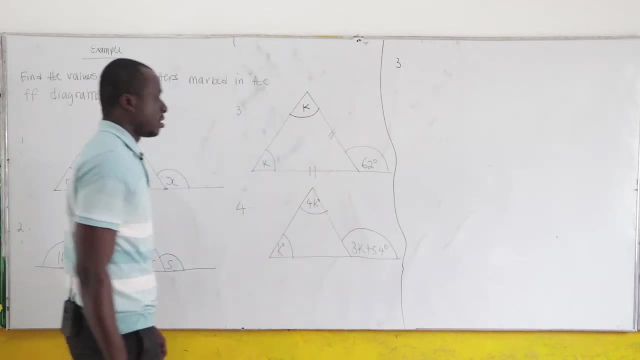 So the angle here will be the same as the angle here. So if this angle is k, then also this side also must be equal to k. So this is opposite interior angle. So this plus is equal to what, That is, the 62 degrees. 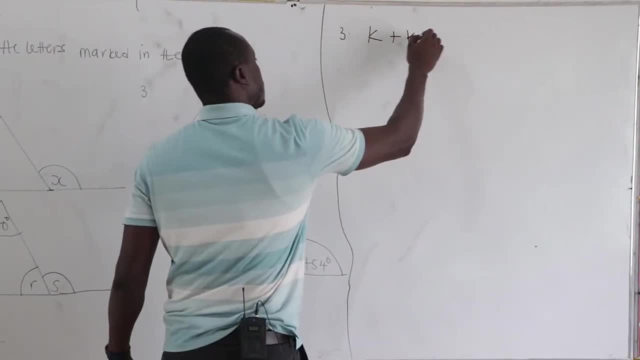 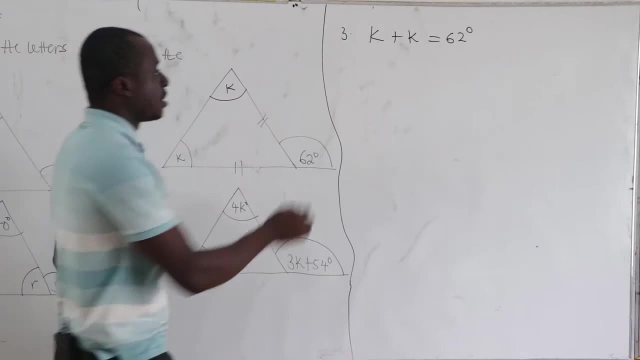 So you can say that k plus k equal to 62 degrees, The sum of the opposite two interior angles, The opposite two interior angles equal to the exterior angle. Now what do we have here? 2k equal to 62 degrees. 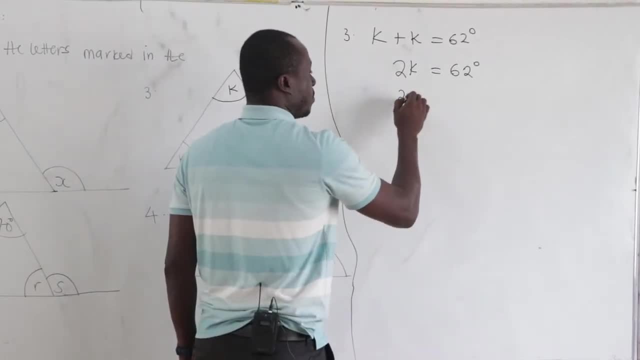 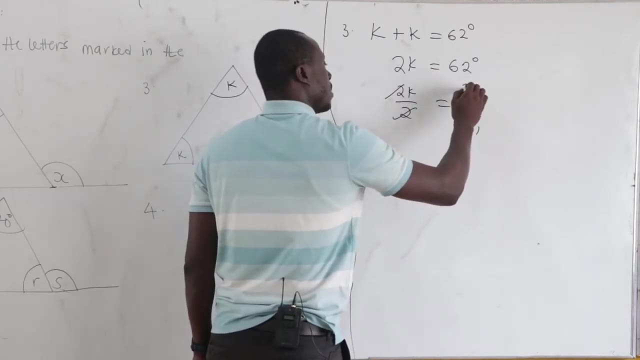 From my idea of algebra. Now I want to find k, So we divide both sides by what is multiplying it. This is canceling Now that 2 go here 1, 2 go here, That is 31.. 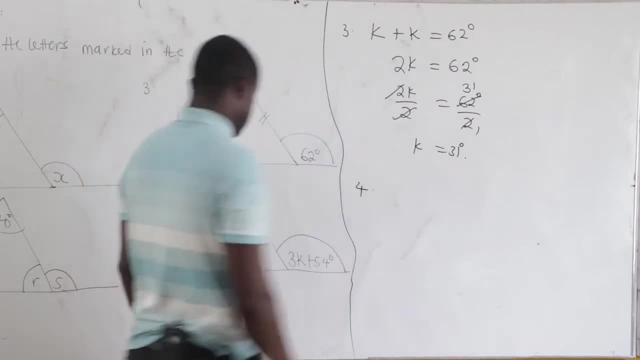 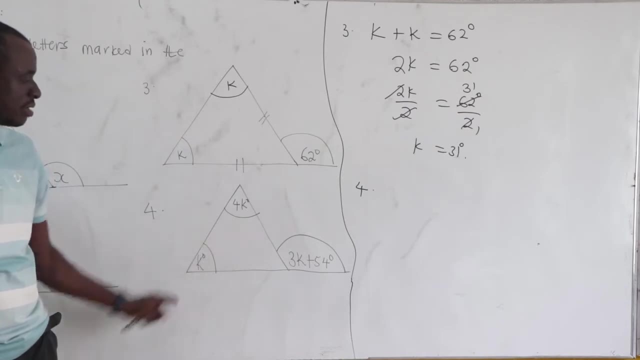 So we have our k to be equal to 31 degrees. Now let's see question number four. Now this is the exterior angle And this is the opposite interior angles. So the sum of the two opposite interior angles equal to the exterior angle. 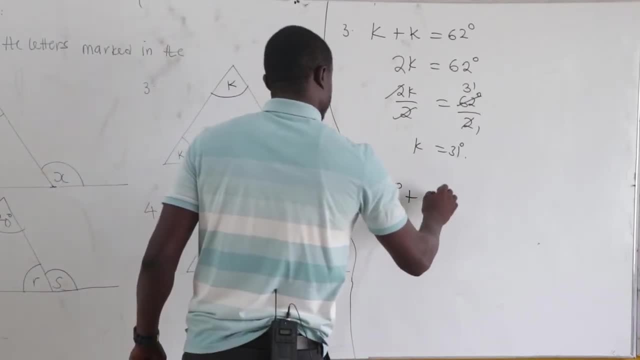 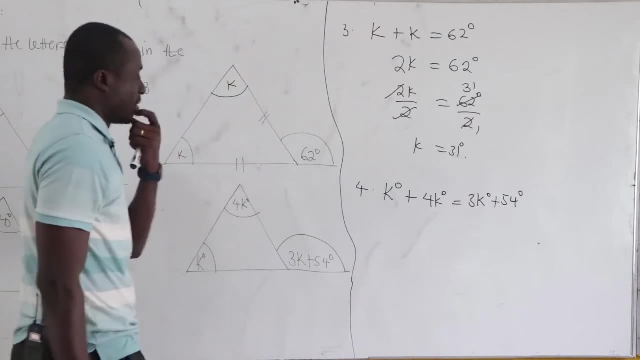 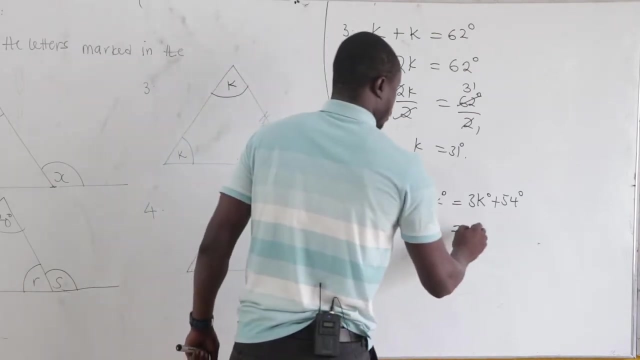 So our k degrees plus 4k degrees, equal to 3k degrees plus 54 degrees, Now k degrees plus 4k degrees, that is, 5k degrees equal to 3k degrees plus 54 degrees. Now this has to come here. 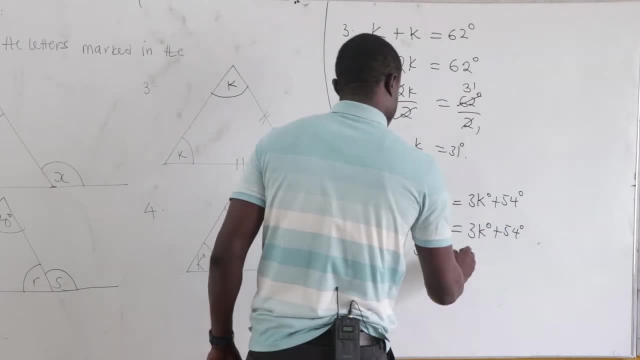 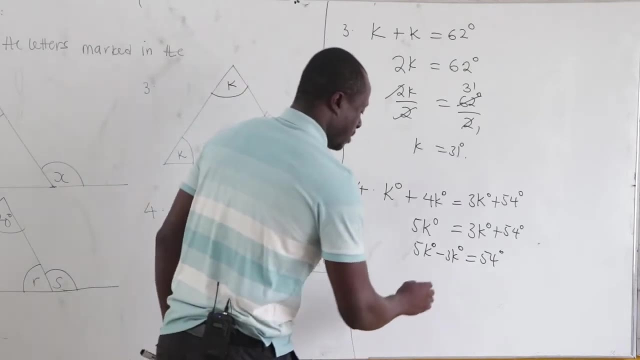 So we have 5k degrees minus 3k degrees equal to 54 degrees. Now, 5k minus 3k, from my idea of algebra that is just 2k degrees equal to 54 degrees. We want to find k. 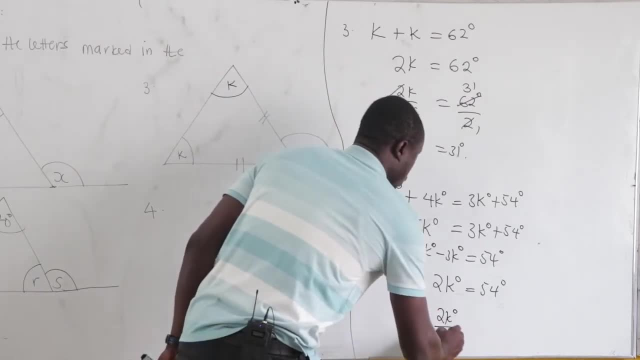 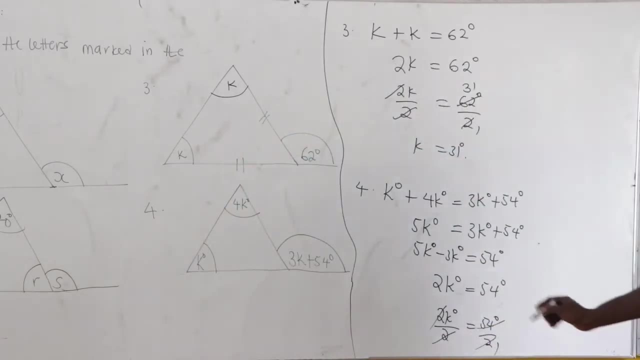 We divide both sides by 2. So 2k degrees all over 2, 54 degrees all over 2.. This is canceling, Now that 2 go here, 1. 2 go into 5. That is 2 times 14, 7.. 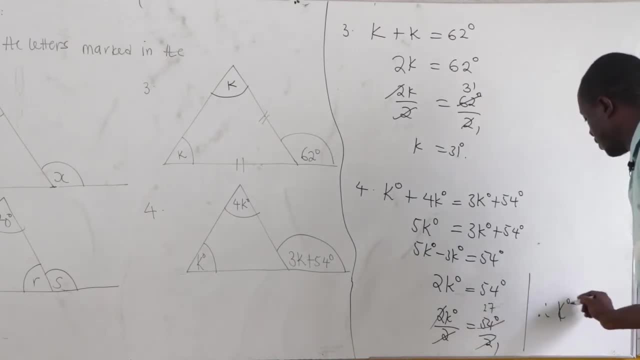 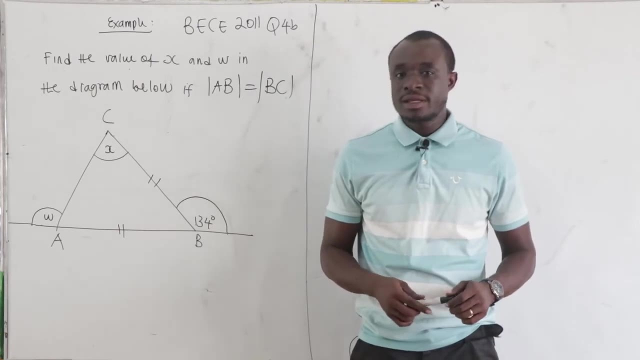 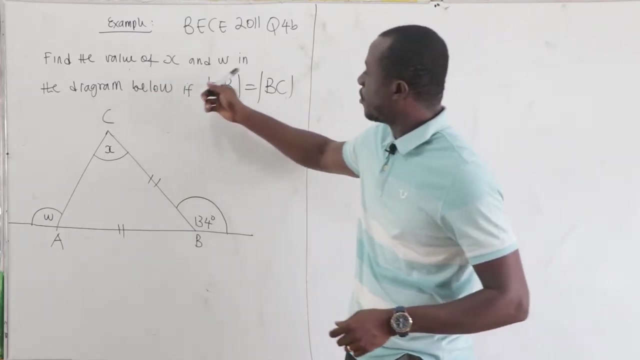 So that is 27.. Hence, our k degrees is equal to 27 degrees. Now let's consider this past question. This is 2011,. question number 4b: Now find the value of x and w in the diagram below. 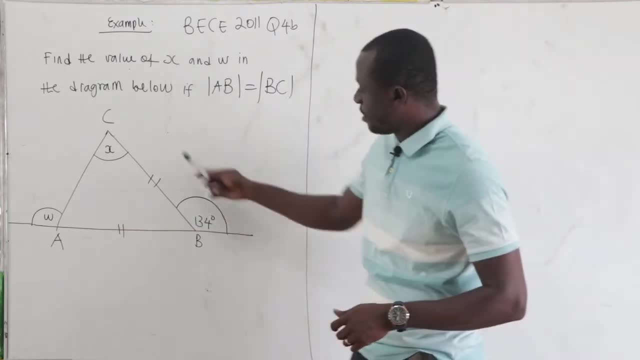 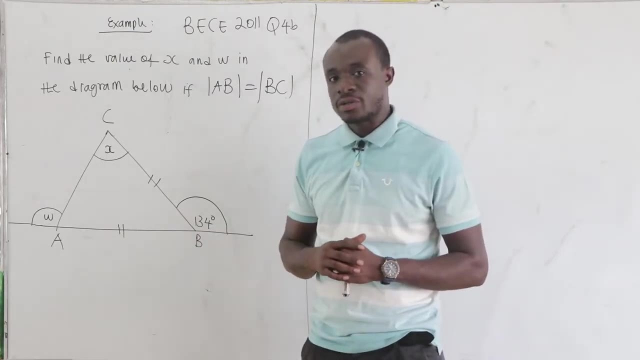 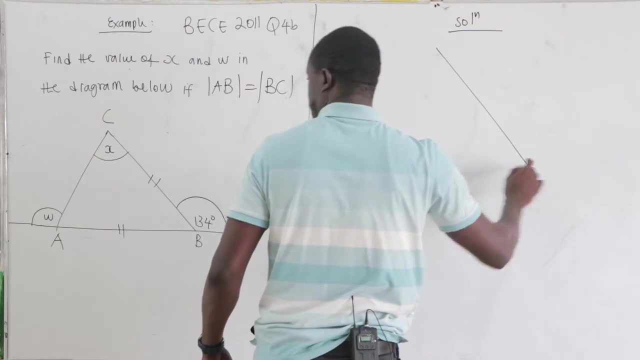 If ab, that is, ab is the same as bc, So what about? So what type of triangle is this? This is an isosceles triangle. Two sides are equal. Now let's redraw it Now. answer book. 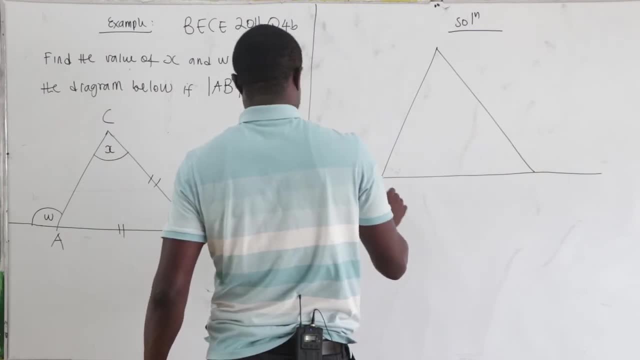 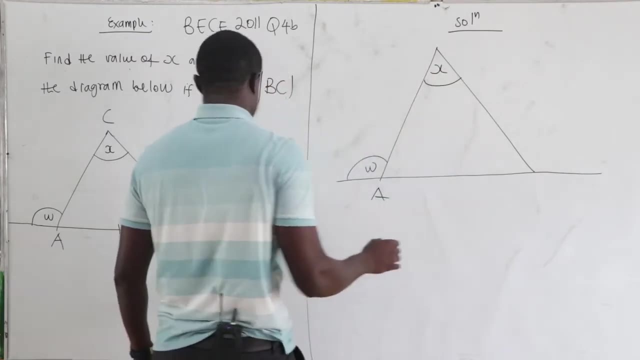 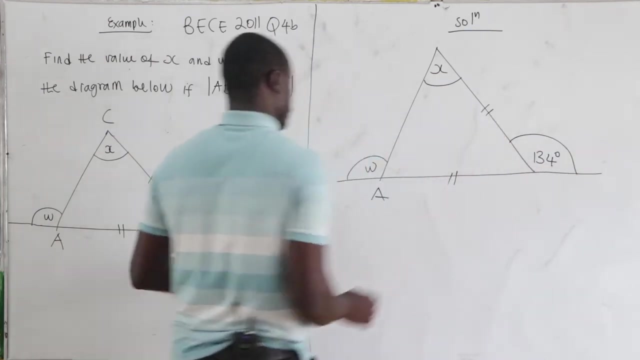 So we have here to be a. this is w Now the angle here is x degrees. The angle here is 134 degrees. Now this side is equal to that side. So this is our c. We want to find the value of x and y. 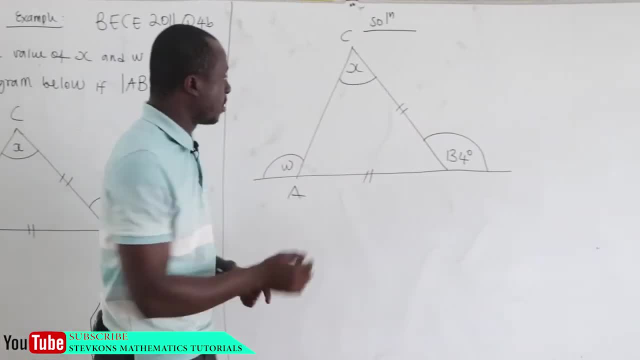 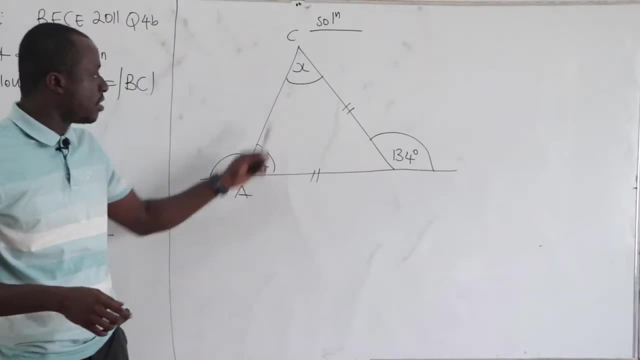 And because this is an isosceles triangle, if this is x, this is what X degrees. Now, how can we find x? We can say: this is exterior angle, This is the opposite interior angle And this is the exterior angle. 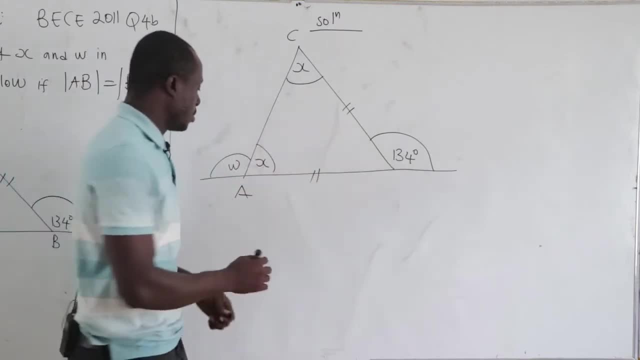 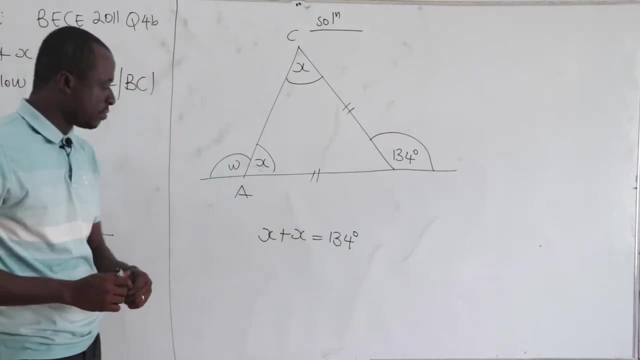 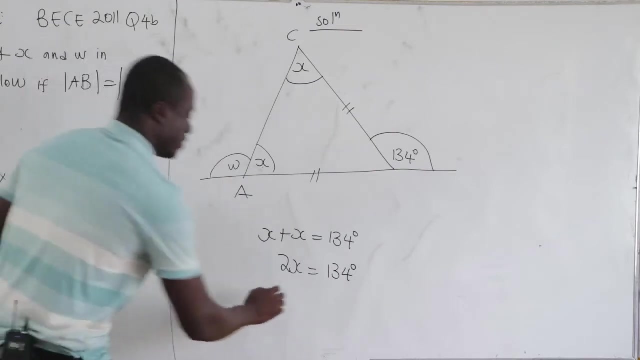 So this is the opposite interior angle, This is the exterior angle. Clearly, x plus x, equal to 134 degrees. Now x plus x, this is 2x equal to 134 degrees. I want to find x. I'll divide both sides by what is multiplying the x. 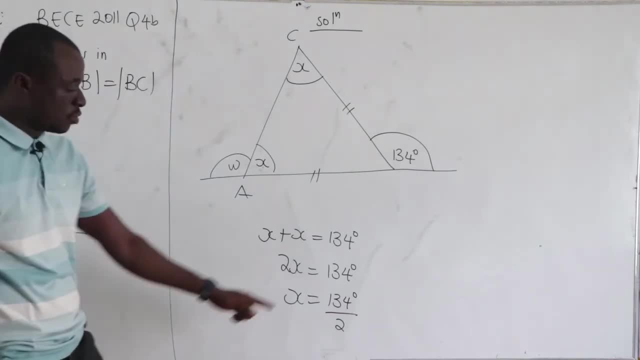 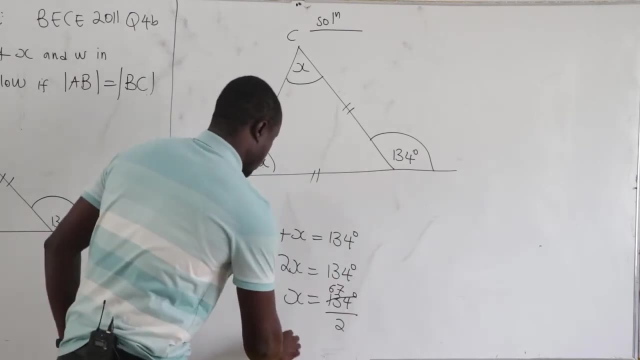 134 degrees all over 2.. Now 2 will go into 13.. That is 6.. 1, 14.. 2 will go into 14.. That is 7.. So we have our x to be equal to 67 degrees. 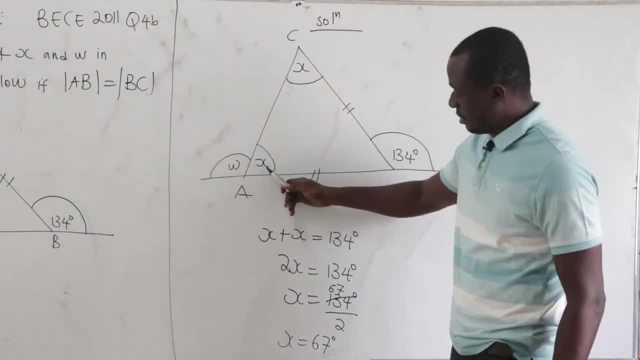 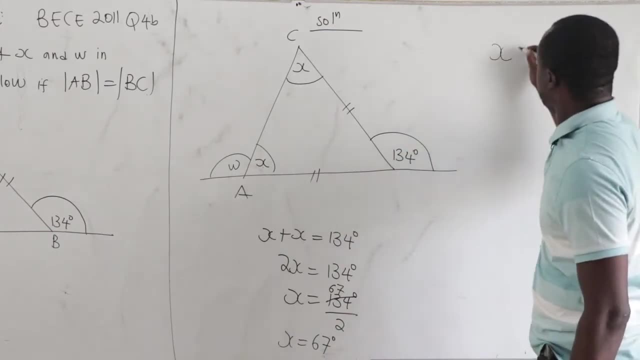 So this is 67, this is w. Now, angles on a straight line add up to 180.. So x plus w, this is equal to what? 180 degrees? What is our x? That is, 67 degrees plus w, equal to 180 degrees. 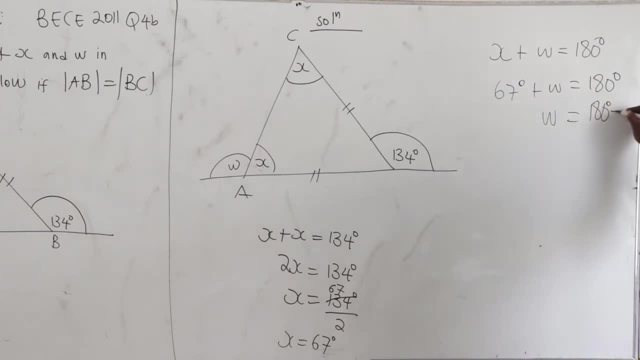 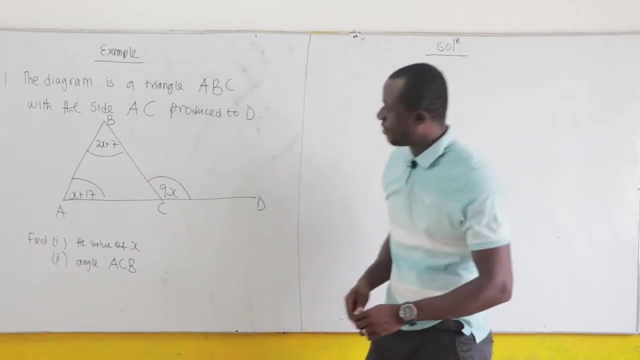 Hence our w equal to what? 180 minus 67 degrees, And 180 minus 67,, that is 113 degrees. Okay, So we have been able to find our answers for the x and then w. Now let's consider the past expression. 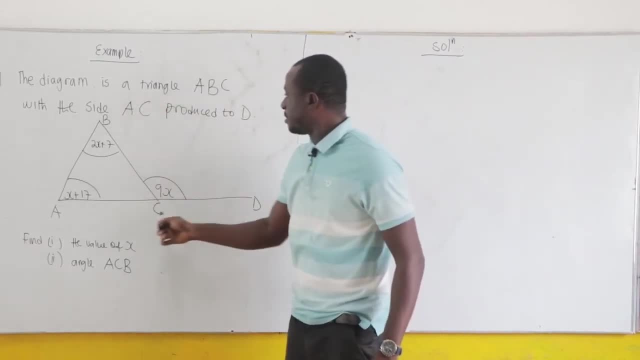 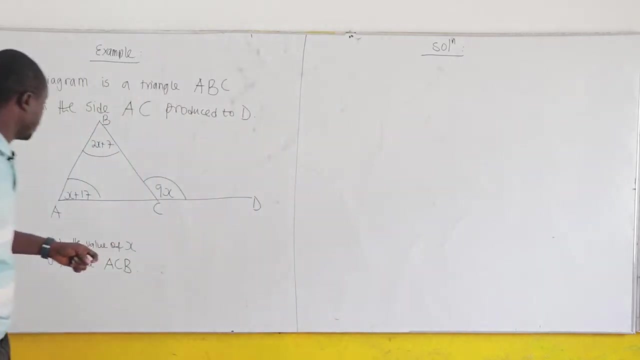 We have been told that the diagram is a triangle, ABC, with side AC produced to D. The answer is: you find the value of x. Now, this is the opposite interior angle, And then we have here to be the exterior angle. So clearly, how can we find it? 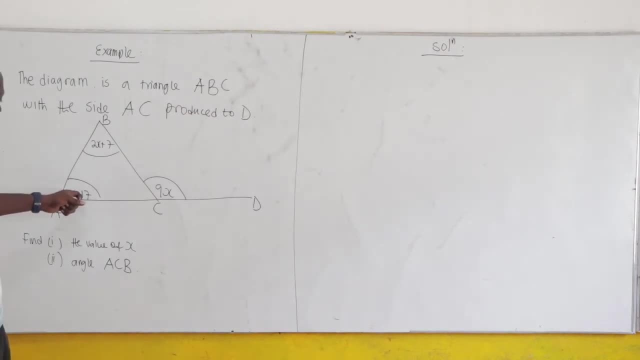 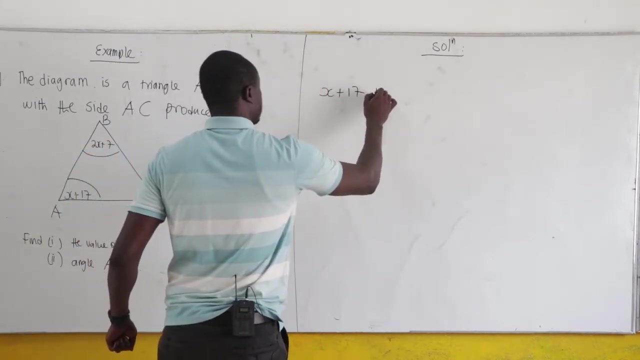 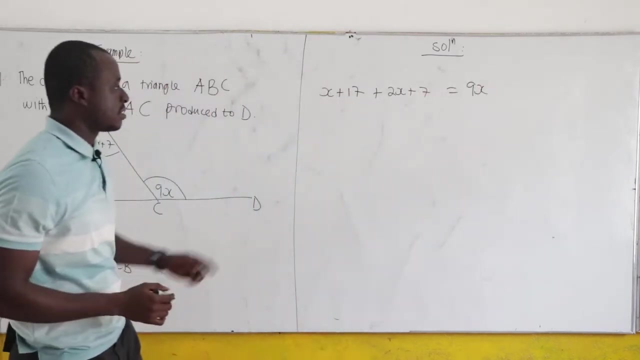 The sum of the opposite interior angle is equal to what The exterior angle. So the angle here plus the angle here equal to what The exterior angle over there. So our x plus 17 plus 2x plus 7. This is equal to 9x. 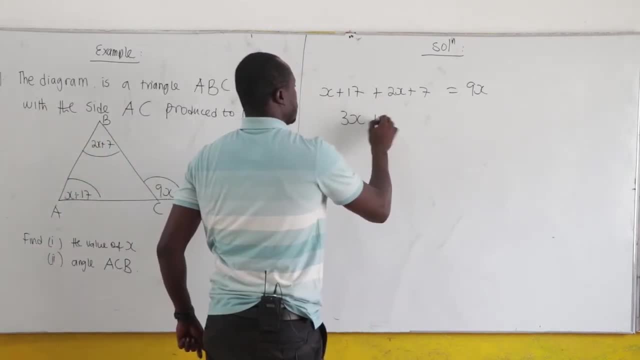 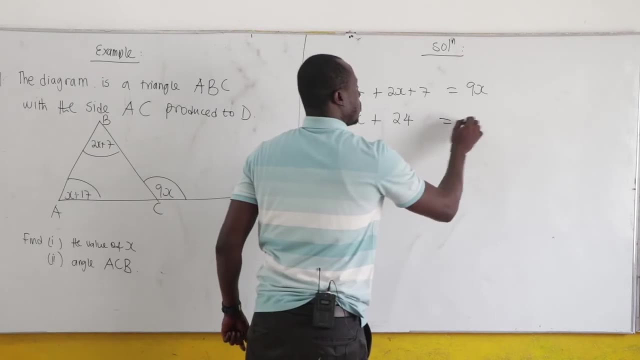 Now x plus x, this is giving us 3x, 17 plus 7, this is giving us that is 24, equal to 9x. We want to find x, So this 3x has to move to that side. 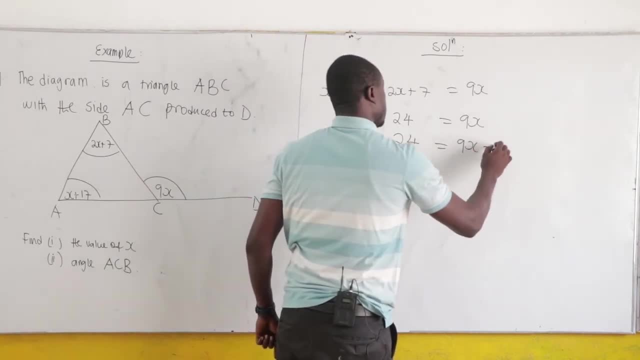 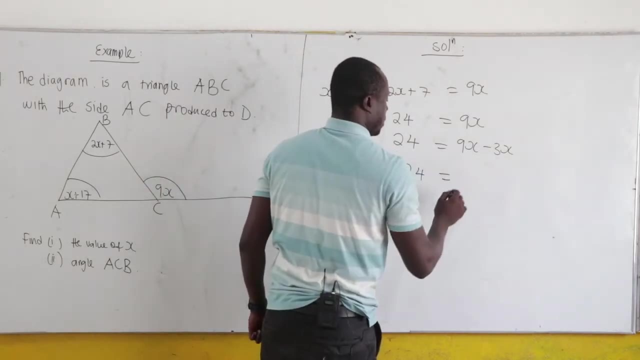 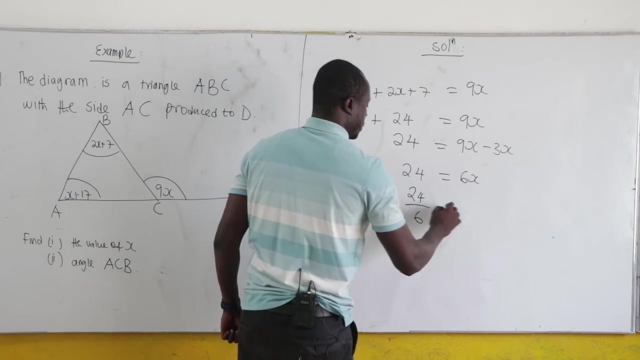 So we have 24 equal to 9x minus 3x. So we have 24 equal to 9x minus 3x. This is equal to what? 6x. So first we find x, 24 over 6 equals 6x all over 6.. 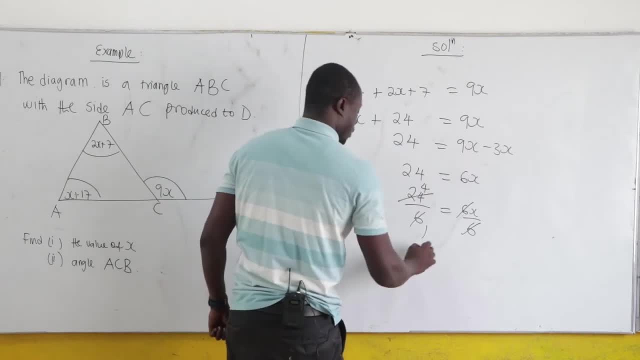 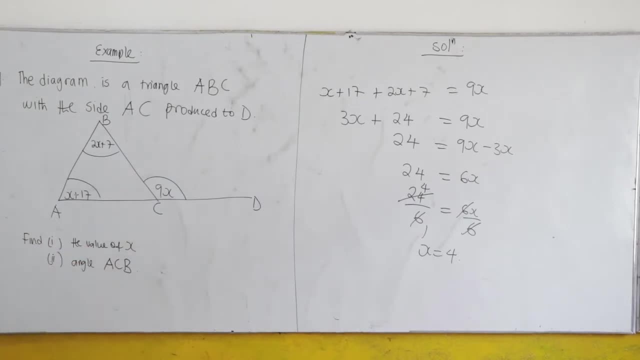 This is canceling that out, Since we have given 1, since we have given 24, that is 4.. So we have x to be equal to what 4 degrees? So that is the value of x, The first one. 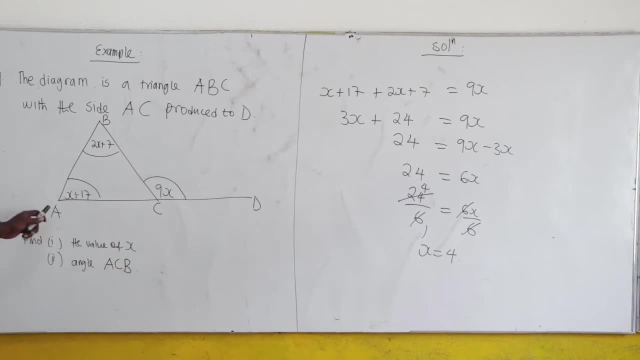 Now the second one is: we should find a, c, d, That is, a c b, The angle a c b. Now, let's see, Let's find angle a, c b. Now, this is a straight line. 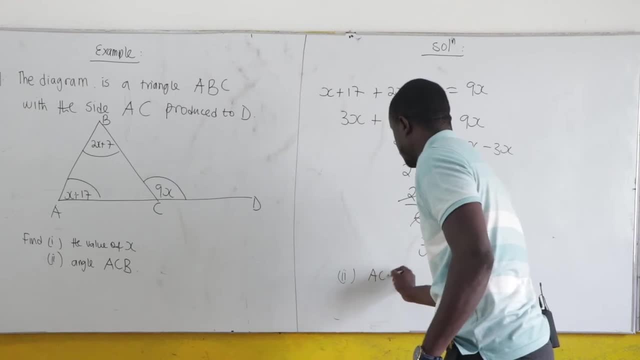 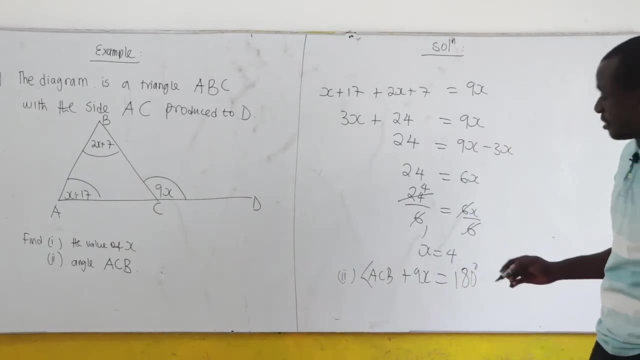 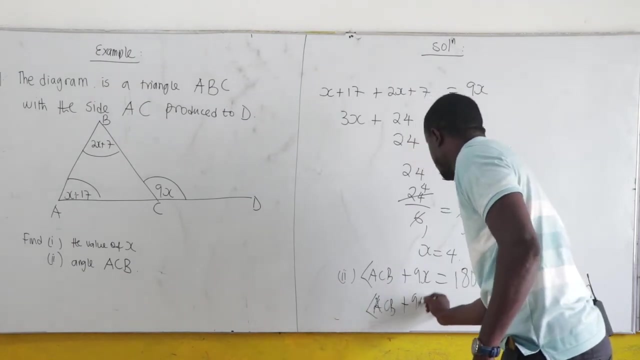 So the second one: what can we say? Angle a, c, b plus the 9x, equal to 180 degrees, Sum of angles on a straight line, X is 4.. So we have a, c, b plus 9 times 4, equal to 180 degrees. 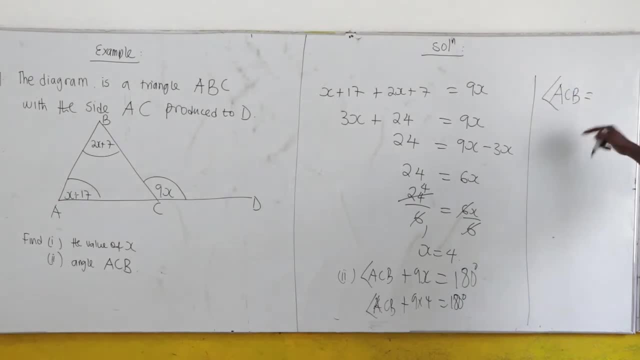 Now a, c, b is equal to 9 times 4 is 36.. So 180 minus 36 degrees. Now what is 180 minus 36 degrees? This is just 144 degrees. That is a, c, b. 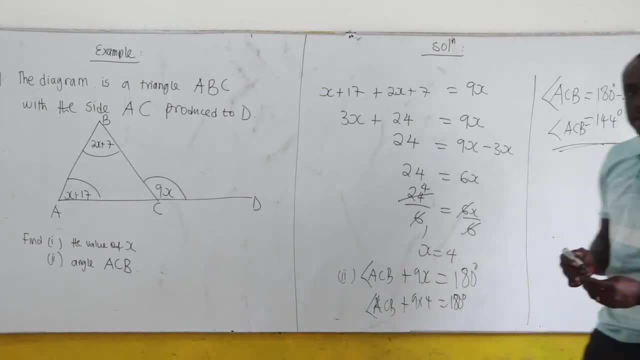 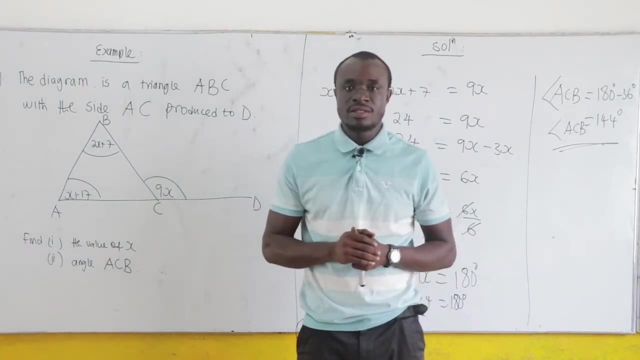 That is a, c, b, And this is very, very easy. So that property is so important, The sum of the two opposite interior angles is equal to what The exterior angle. Now let's consider this example. This is a past question. 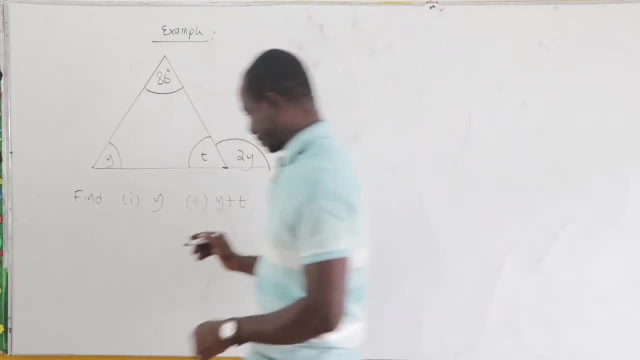 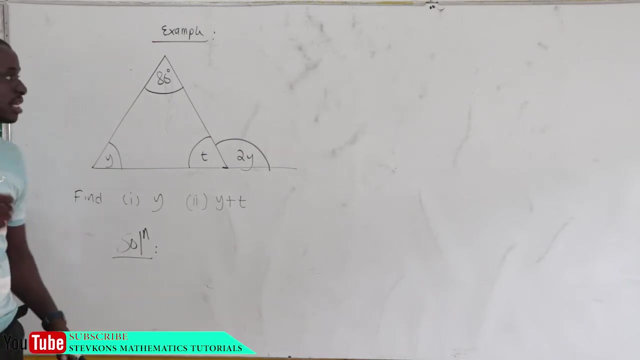 Now we want to find y. Now, what can we see? You see, we have this Y plus 80, this is equal to is equal to what? 2y? Why are we using that principle? The sum of the opposite: 2 interior. 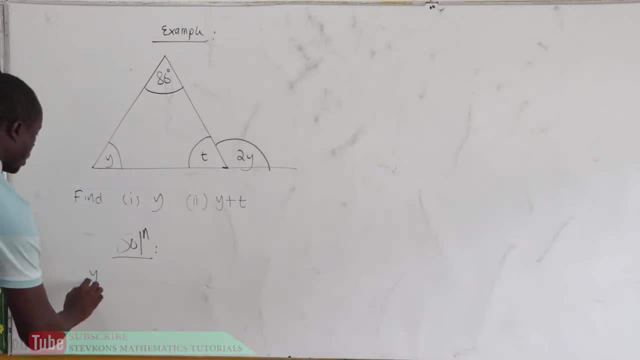 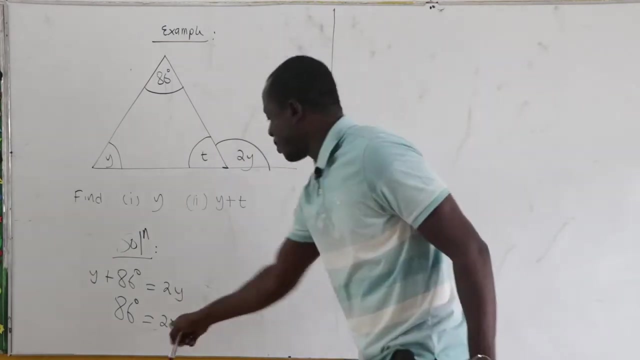 angle is equal to the exterior angle. So you can say that y plus 86 degrees equal to 2y. Now this has to go here. So you have 86 degrees equal to 2y minus y. Now what is 2y minus y? 2y minus y is y. 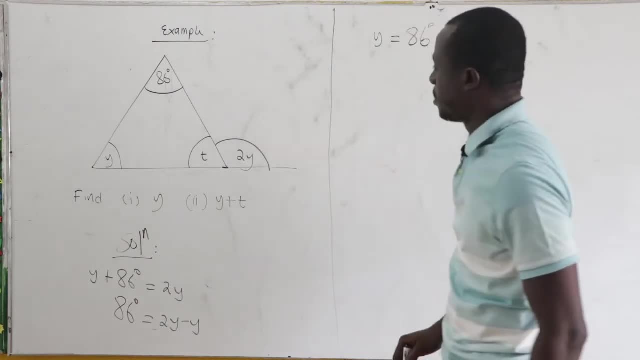 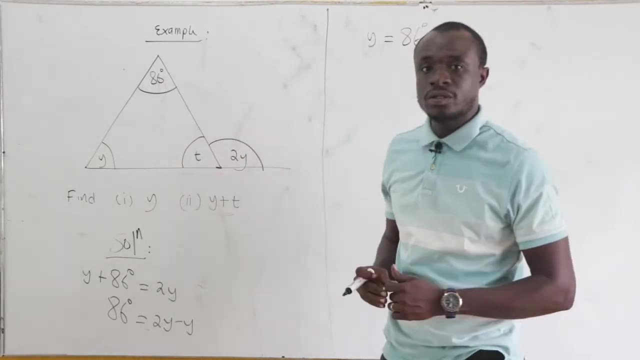 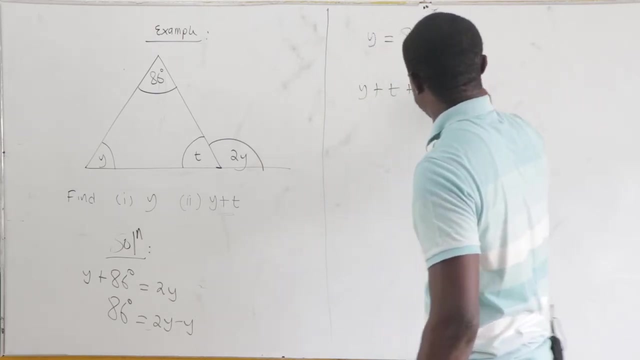 So y is equal to what 86 degrees? Now? the next one is: we want to find y plus t, Now sum of angles in a triangle equal to 180 degrees. So you can say: y plus t plus 86 degrees equal to what 180 degrees? 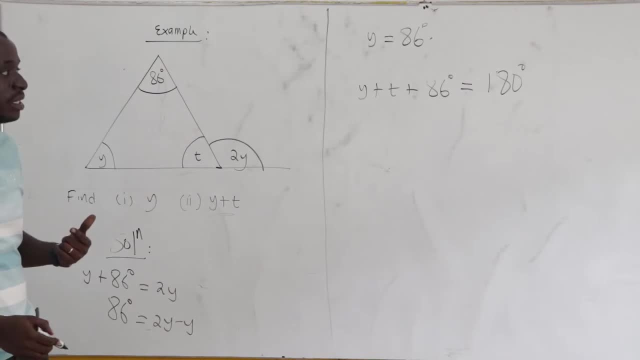 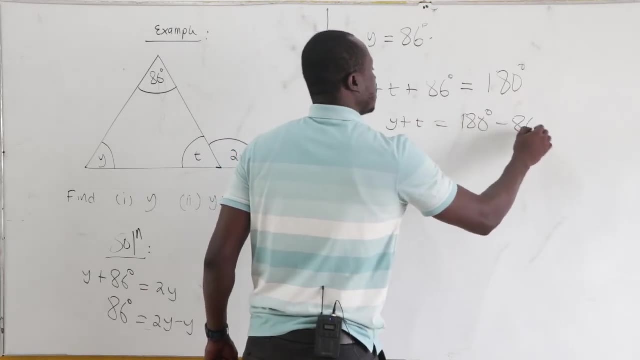 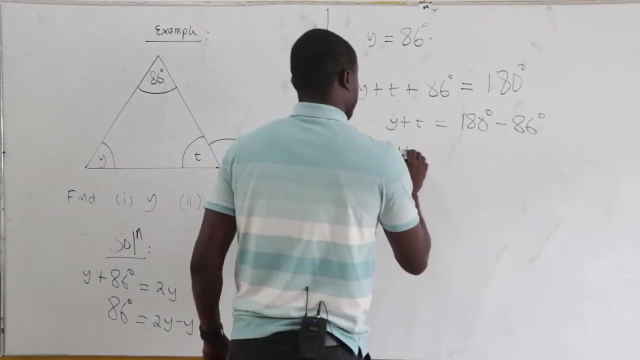 Why? Sum of angles in a triangle equal to 180 degrees. So y plus t. equal to 180 degrees minus 86 degrees. Now what is 180 degrees minus 86?? And this is just 94. So y plus. 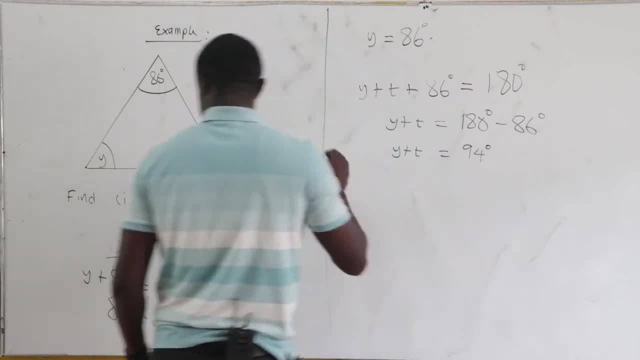 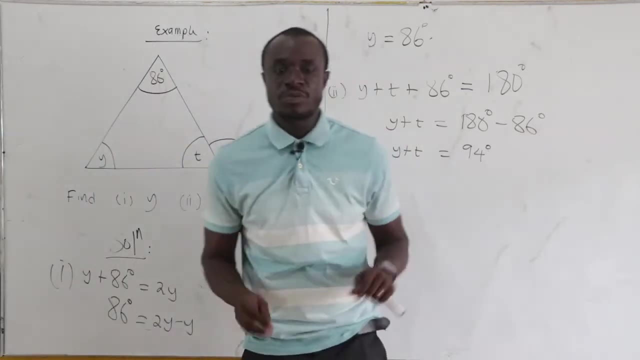 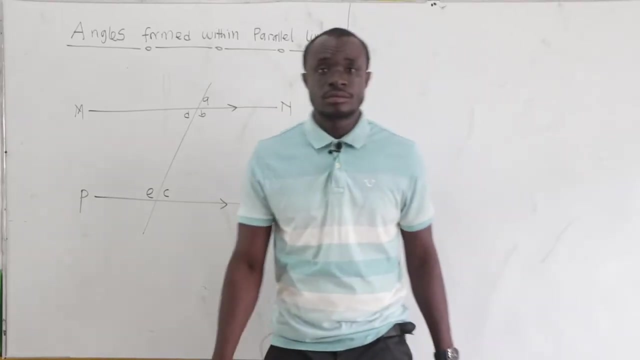 t equal to 94 degrees. So this is i, i and then this is i. That is very easy. So the principle: the sum of the two opposite interior angles equal to what The exterior angle. Today we like to consider angles. 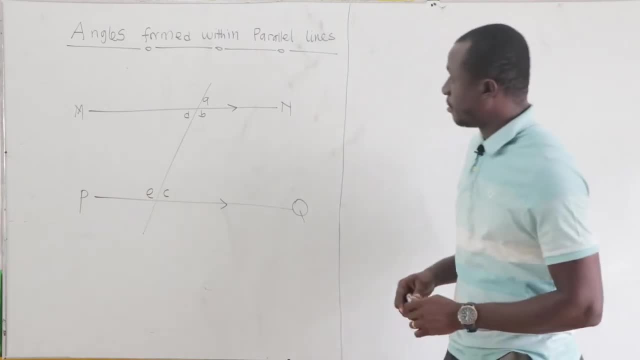 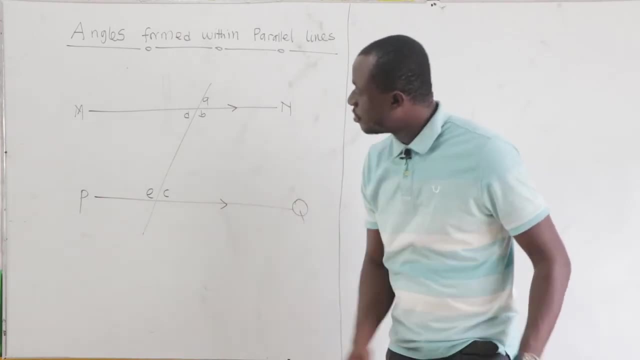 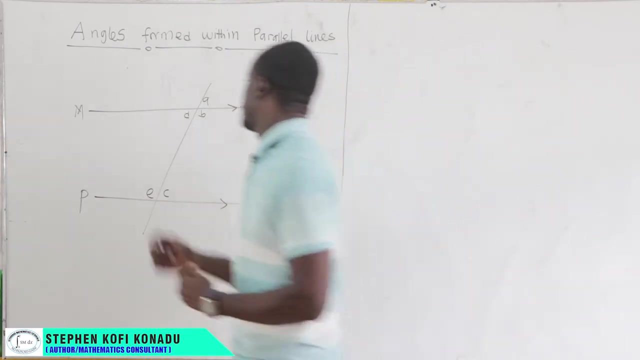 formed within power. Now let's see if m? n is power to p, q. Now we call this line the line that is passing through these two power lines, that is, a transversal, And we have an angle here, angles within them. Now let's 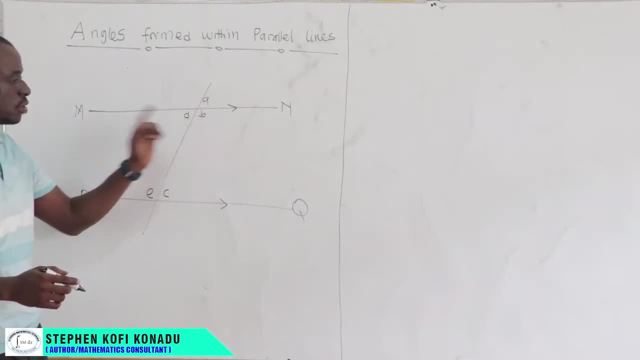 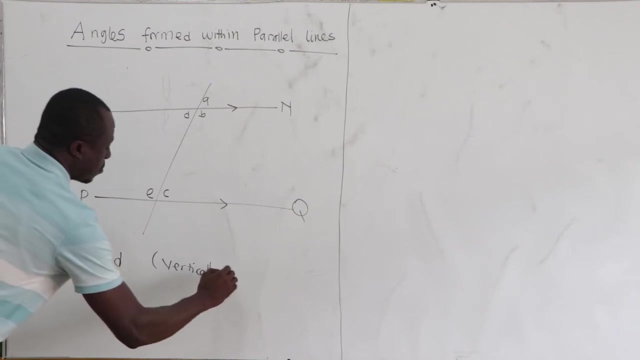 note the following. Now: angle a is equal to what Angle d? We have a straight line and another straight line, So it forms vertically opposite angles. So we say angle a is equal to d. Vertically opposite angles are equal. 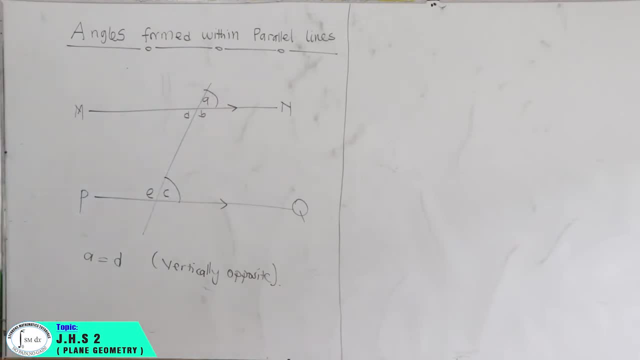 Now angle a is equal to angle c, So a is equal to c. How do we call it Corresponding angles? Corresponding, So corresponding angles are equal. Angle a is the same as angle c. Now also we say that b is equal to e and then d is equal to c, So you say b is equal. 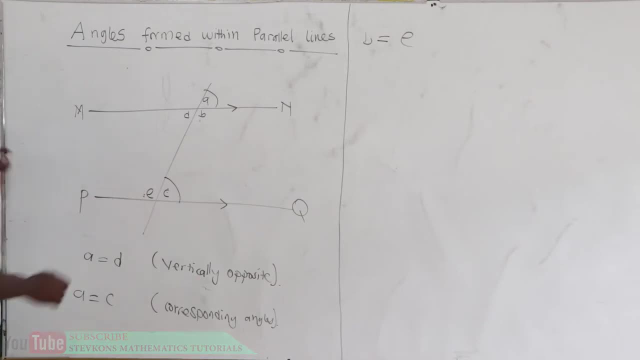 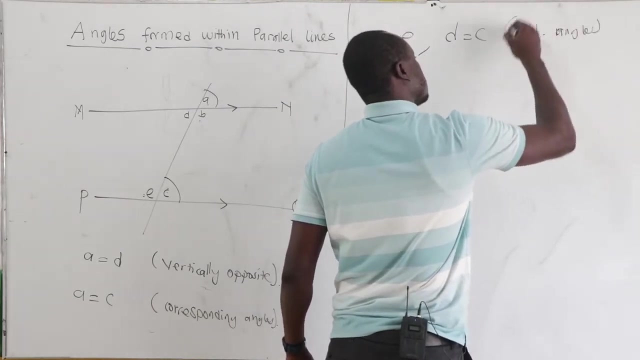 to e. The angle here b is equal to the angle e. and then we also say angle d is equal to c. How do we call it? It's having a special name and in a special way. we call it alternate angles, So alternate angles, That's how we call it. So alternate. 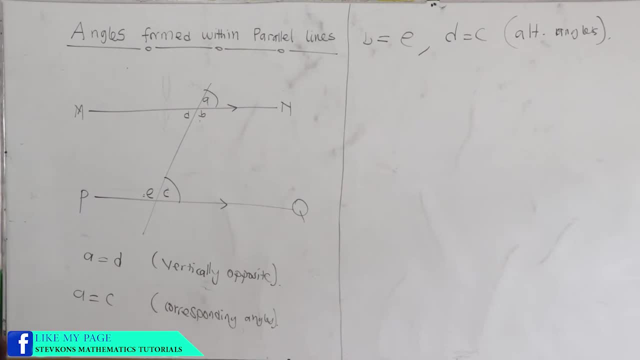 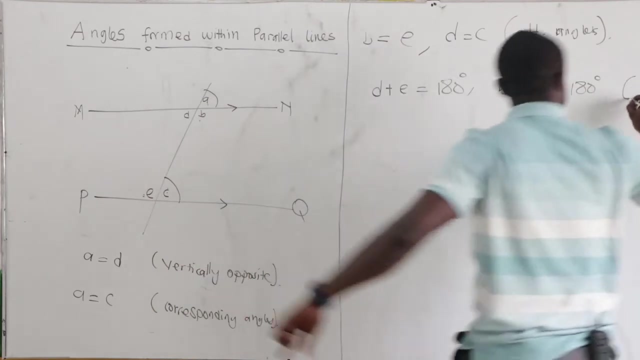 angles are equal. now again, the angle here, that is, if you have two power lines, angle d plus angle e is equal to 180. so we say d plus e equal to 180 degrees, the same with b plus c, b plus c equal to 180 degrees. how do you call it? we call it co interior. 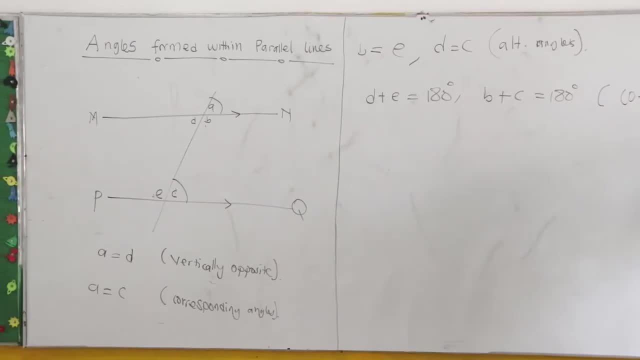 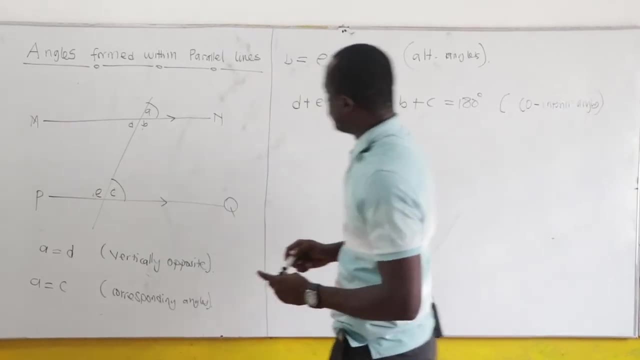 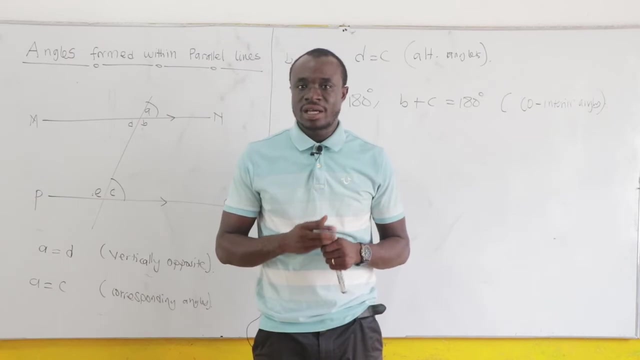 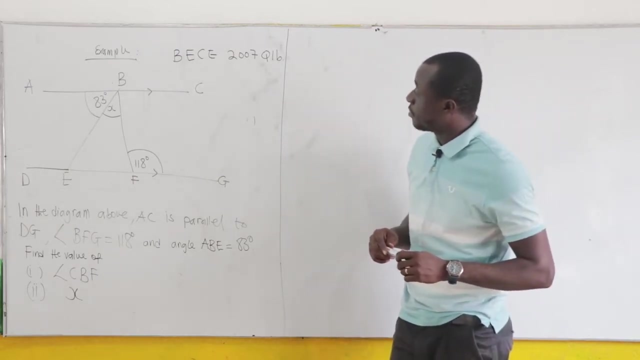 angles. so the angle here is equal plus the angle here equal to 180. this plus that equal to 180.. now we have a whole lot of questions for us to consider so that our understanding becomes very, very fair. now let's consider this past question, this bc 2007, question number one b. 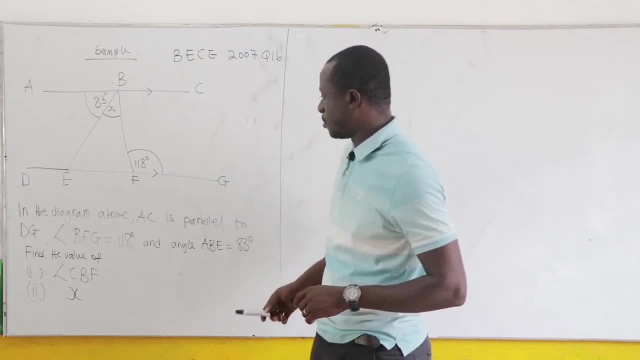 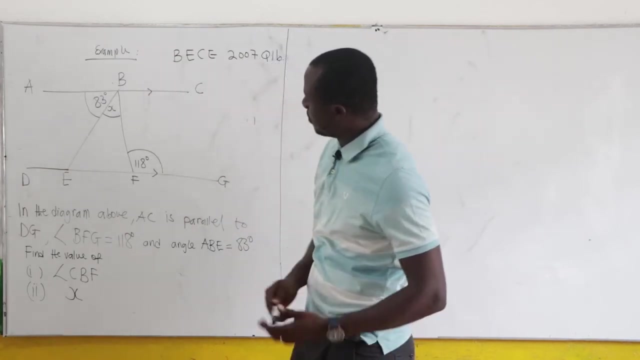 now we have been told in the diagram above, ac is parallel to d, j, so a is power to dj. we have the transversal, that is bf. and then be now the first one which find cbf, cbf. now the angle here plus the angle here, that is, would form cool interior angles. so 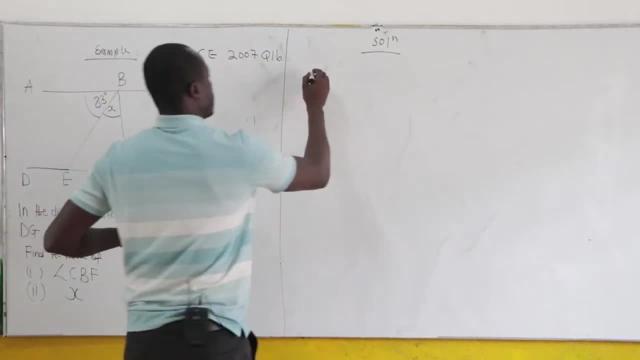 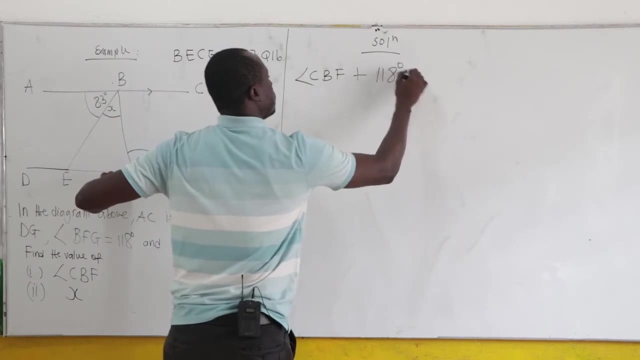 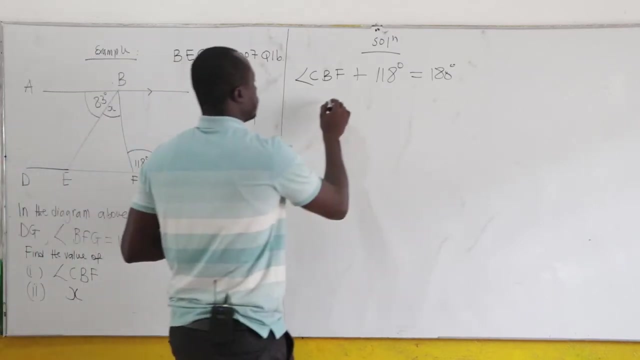 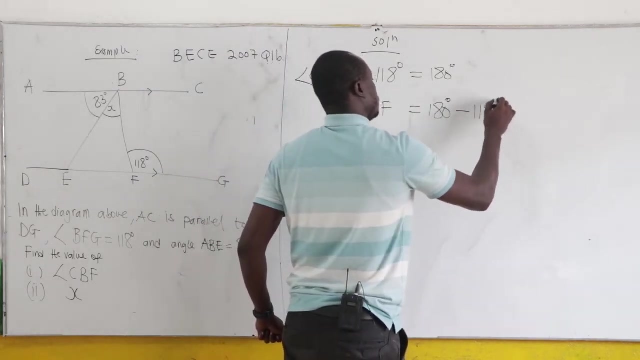 the angle here plus the angle equals 180. so you say that cbf plus the angle. what is the angle here? one one eight degrees equal to 180 degrees. what's the reason? cool interior angles add up to 180. so our c b f equal to 180 degrees minus one one eight degrees. now 180 degrees minus one one eight. 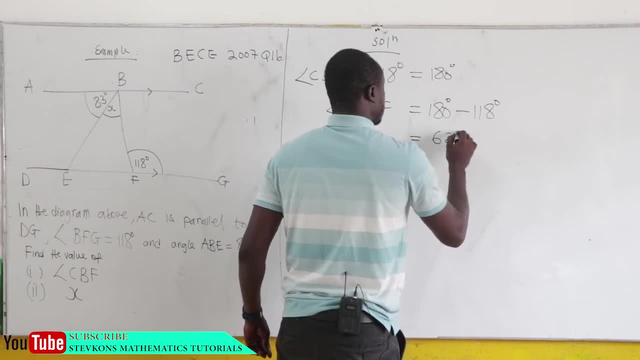 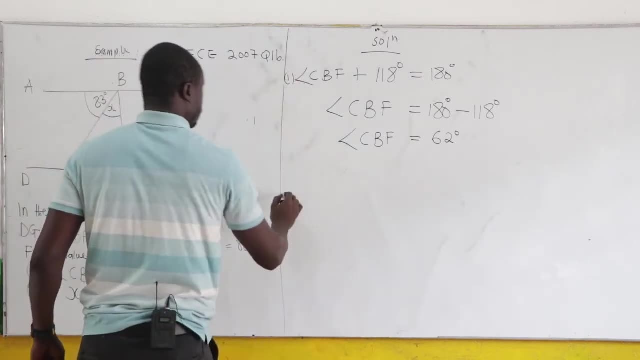 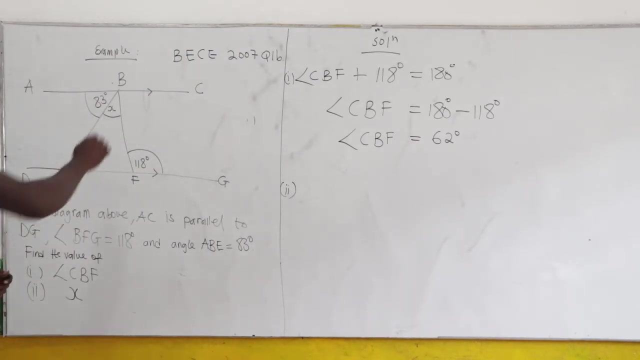 degrees. this will give us, that is, 62 degrees. that's angle c, p, f. that's the first one. now, second one says that we should find x. we should find x over here. now this is a transversal and the angle all the way from here is the same method. 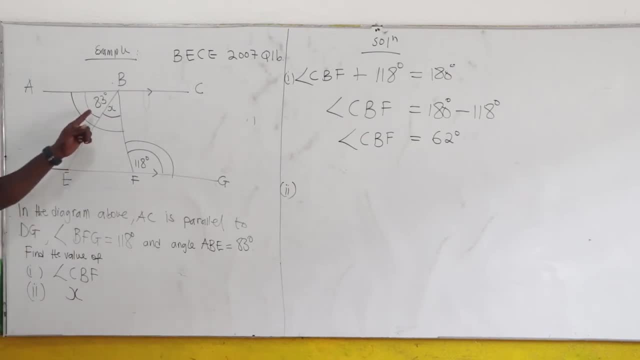 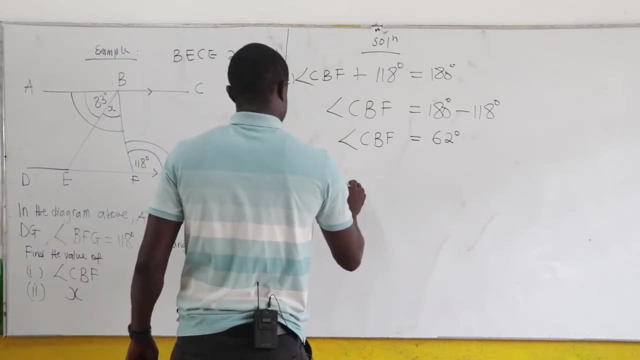 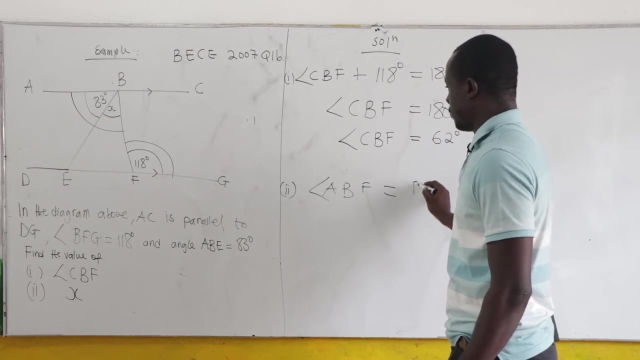 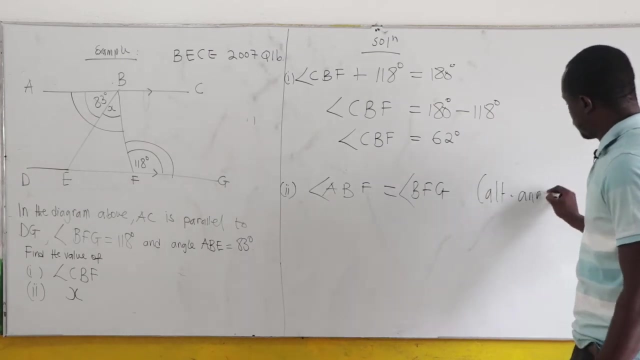 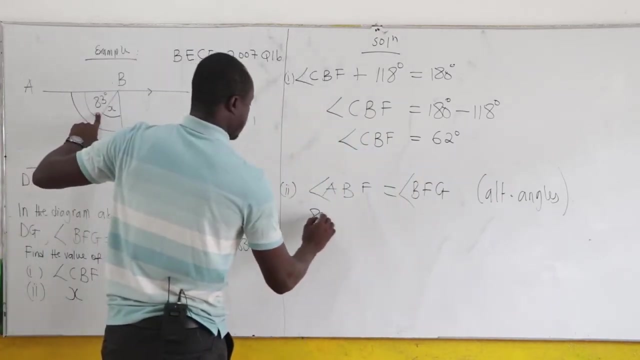 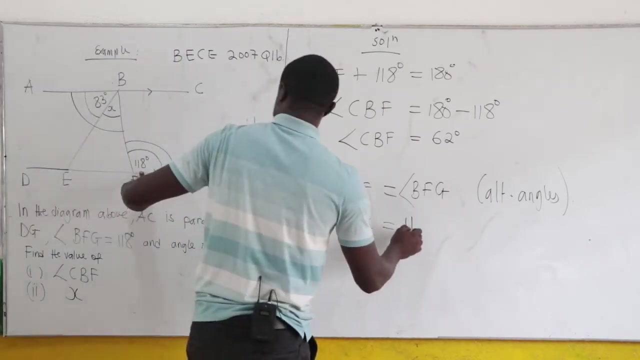 the angle over here. so the angle here, that is a b f is equal to b f j. now angle a b f is equal to b f j and this would alternate angle. now, what is abf? abf is the same as 83 degrees plus x. what is bfg? bfg is 118 degrees. 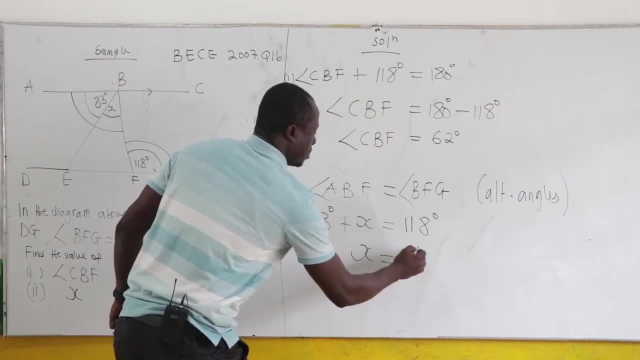 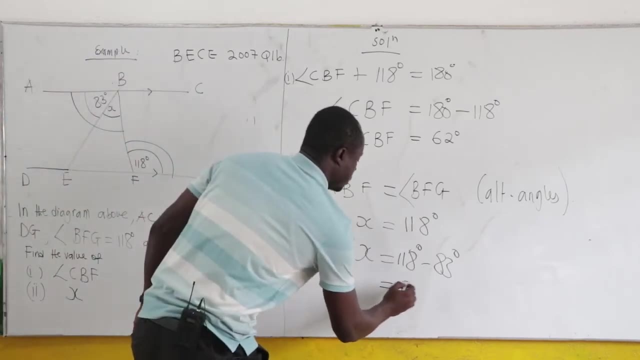 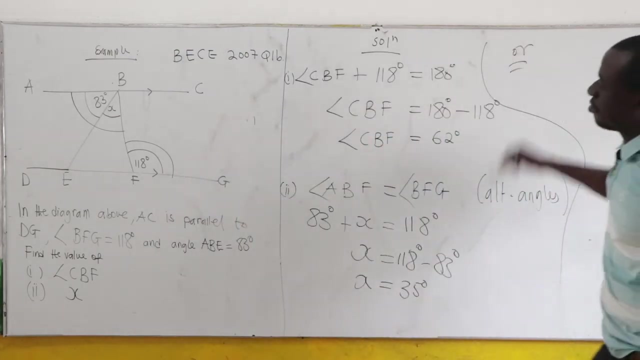 so clearly. our x is what? 118 degrees? degrees minus 83 degrees? what is 118 degrees minus 83 degrees? this is just 35 degrees. oh, oh, oh, if you can, if you can see that this one is alternating to that, we know the angle here to be. 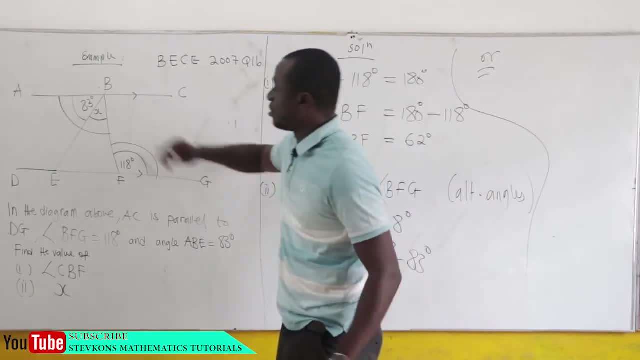 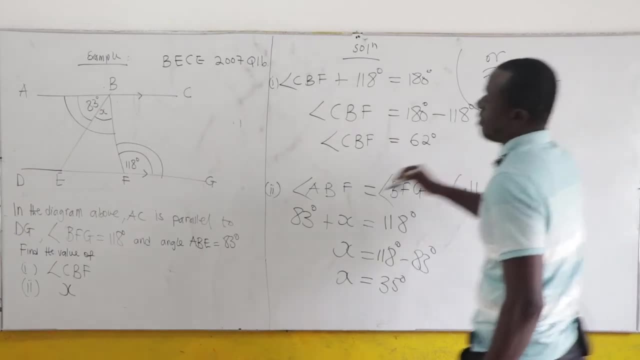 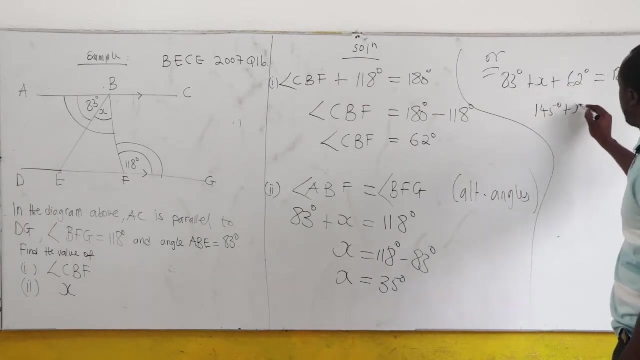 equal to 35. we know the angle here. that is 62 degrees, sum of angles on the straight line equal to 180.. so that is 83 degrees degrees plus X, plus the angle over here, that is 62 degrees equal to 180 degrees. now 63 plus 62, this is 145 degrees plus X, equal to 180 degrees. so our X is equal. 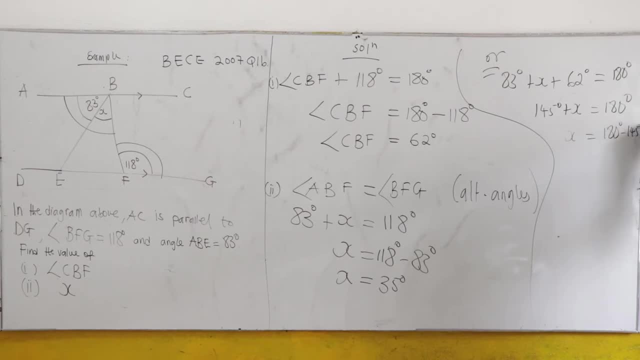 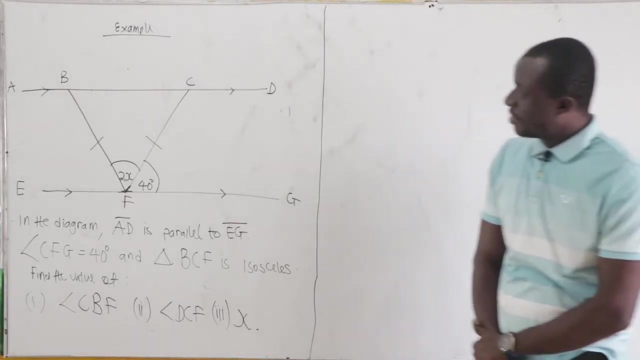 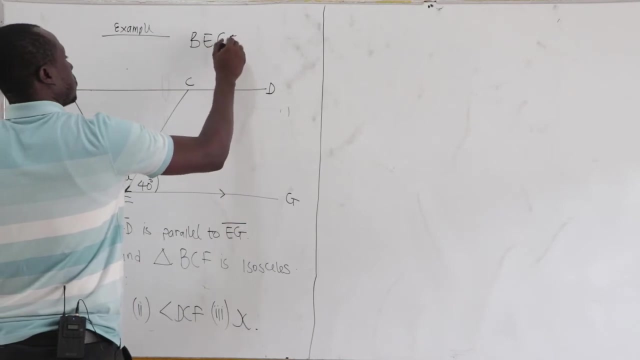 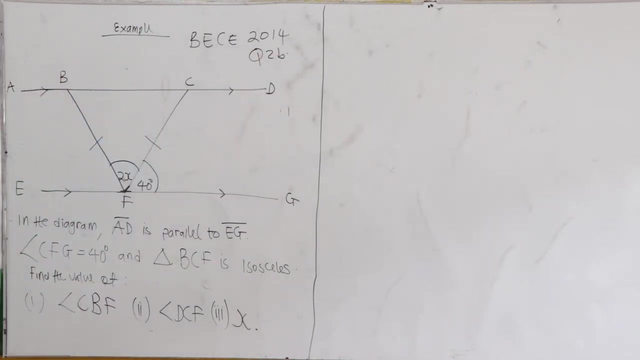 to 180 degrees minus 145 degrees. now, what is 180 minus 145? 180 minus 145, that is 35 degrees, and this is very, very easy. now let's consider this example, and this is BEC 2014. question number 2 being now in the diagram: AD is power to that is. 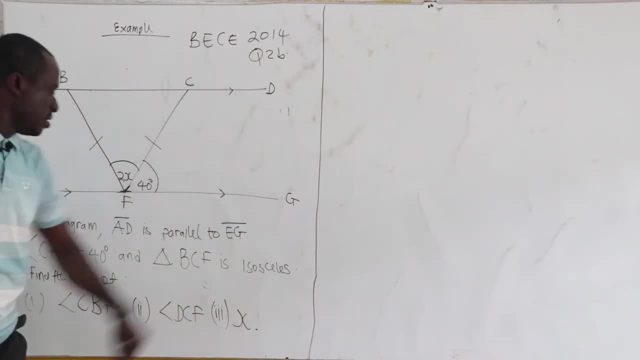 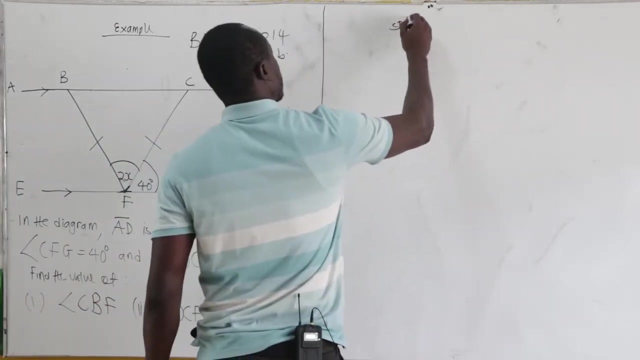 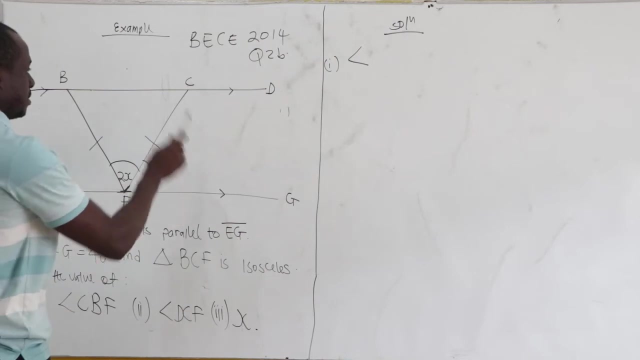 EG. so AD power to EG. and then they've been given the angles: defensive. you should find CBF, CBF, now triangle, BFC is isosceles triangle. okay, now what can we see? the angle here is alternating to the angle over here now. so that is angle angle, that is CFG. 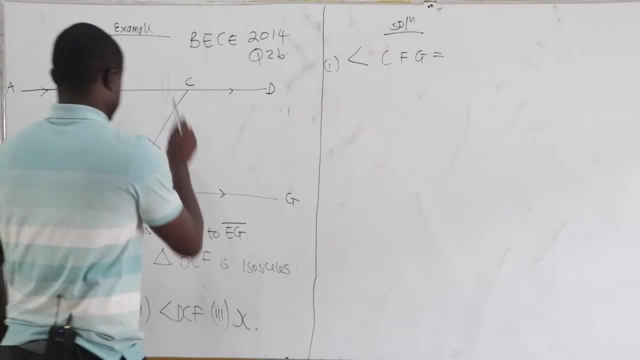 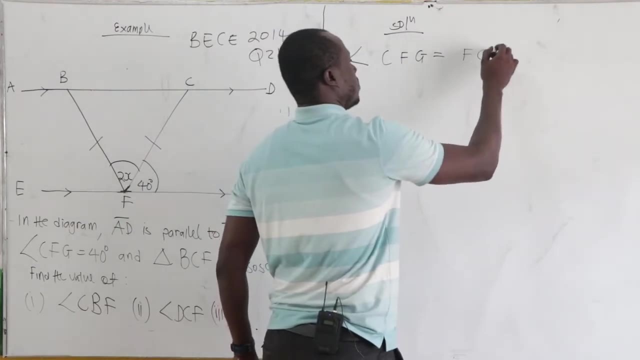 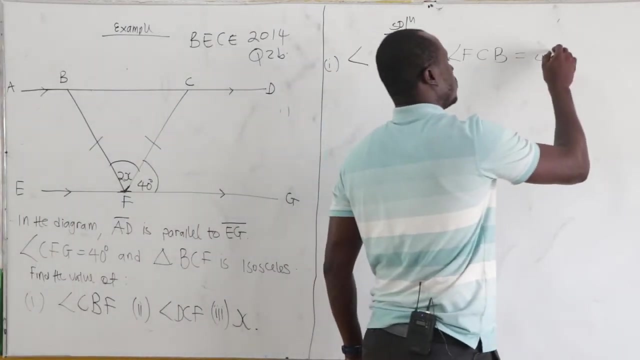 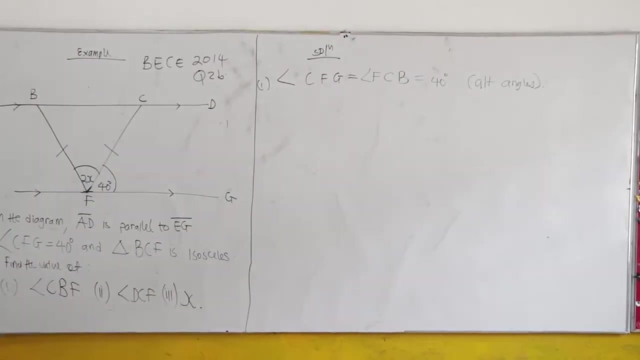 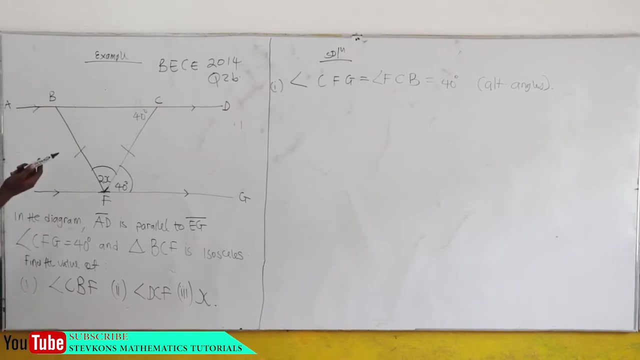 is the same as our Cfg, is the same as our FCB, same as FCB, FCB, and this is equal to 40 degrees, while alternate angles, not the resin alternate angle. so the side is 40 degrees now because a BFC is isosceles, Hence the base angles are the same. So if this is 40, this is also 40. 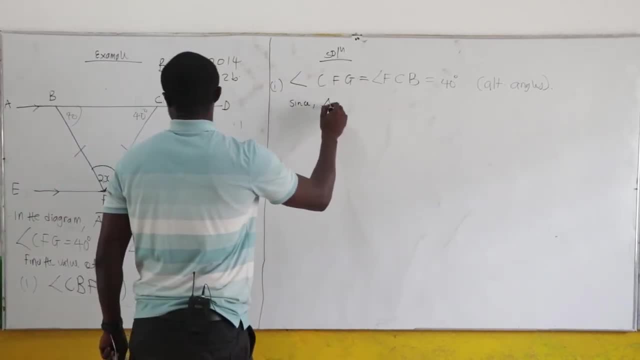 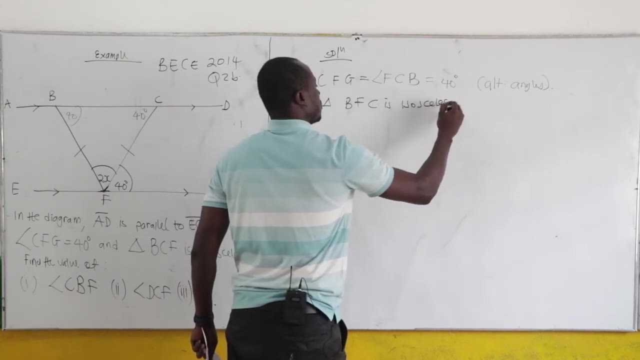 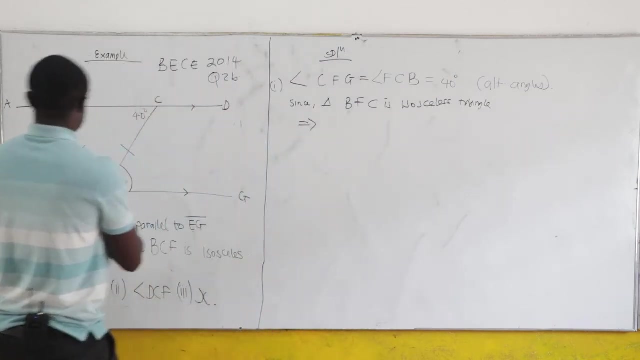 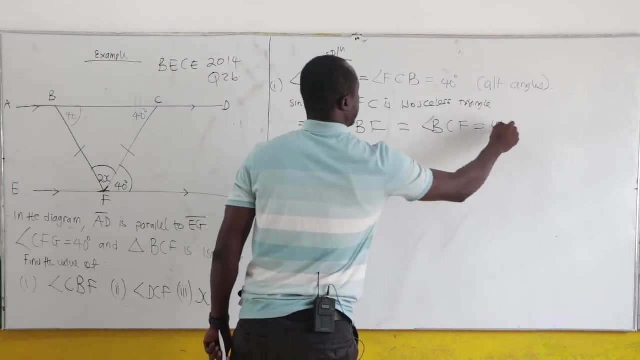 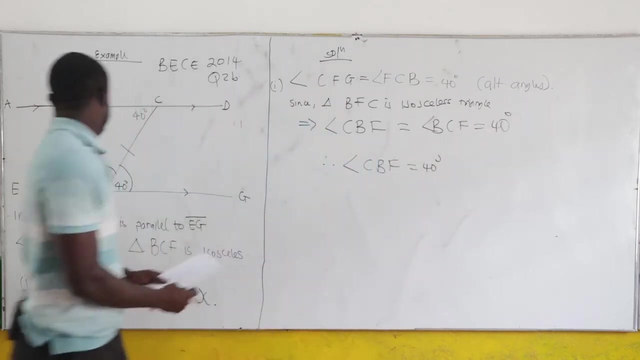 Now. so it says that this triangle, BFC, is isosceles triangle. Now, this implies that angle FBC, angle CBF is equal to angle BCF and this is 40 degrees. Therefore, what we are looking for is that the CBF, this is equal to 40 degrees and the angle over here is 40 degrees. 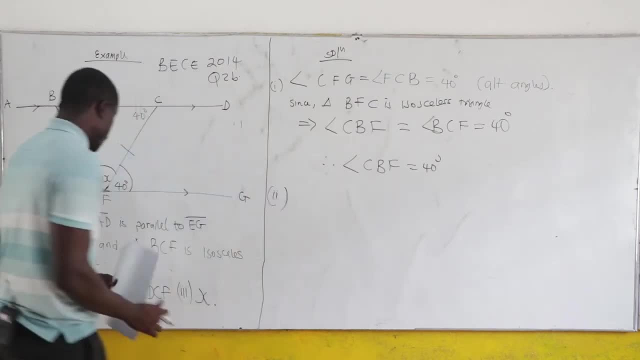 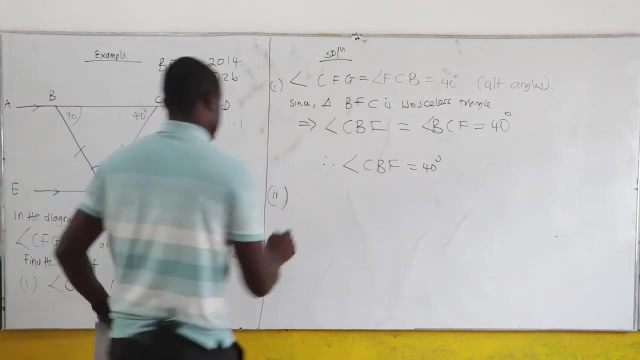 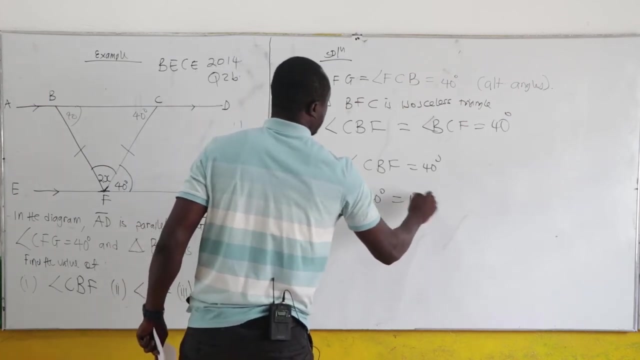 Now let's see the second one. Let's say we want to find DCF, DCF. Now this angle plus the angle here is equal to 180, or sum of angles on the straight line is equal to 180. Anyone that they want to find. so we have DCF plus 40 degrees is equal to 180 degrees. 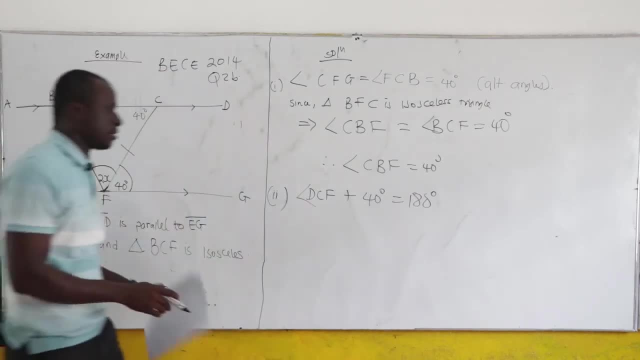 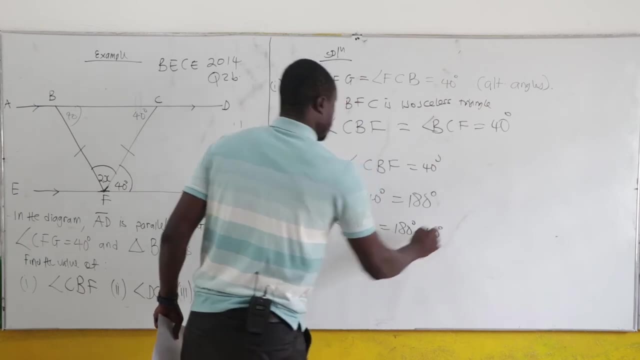 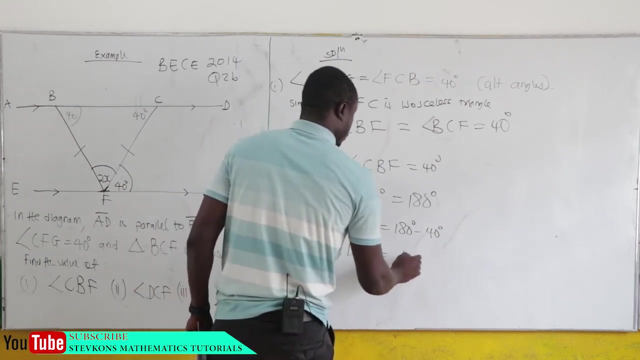 Either we use the co-interior or sum of angles on the straight line. Now, therefore, our DCF is equal to 180 minus 40 degrees. Hence, our DCF is equal to 180 minus 40. This is 140 degrees. 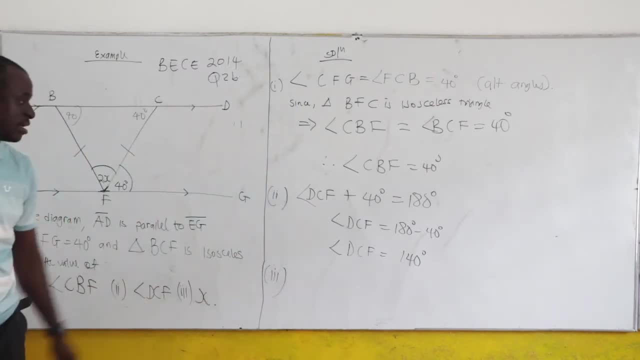 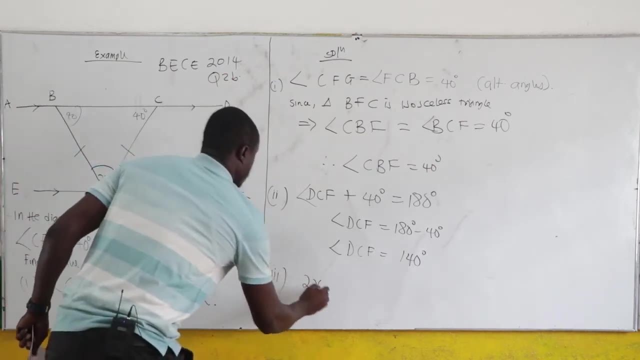 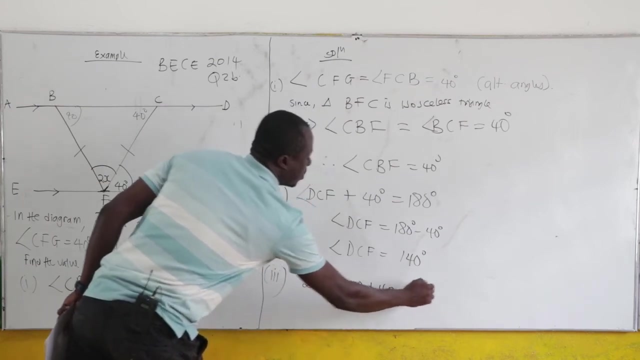 Now let's see the third one. The third one says that we should find X. Now let's see sum of angles in a triangle equal to 180. So we can say that that is 2X plus 40. So we have 2X plus 40, equal to 180 degrees. 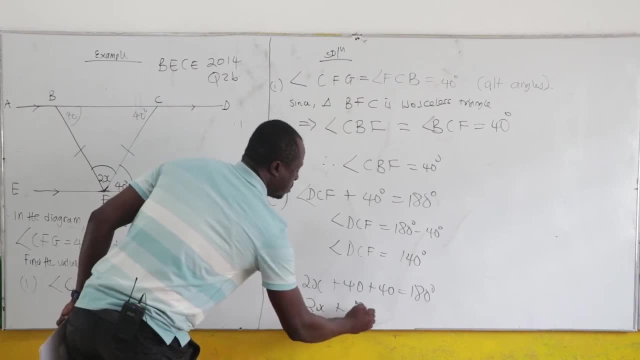 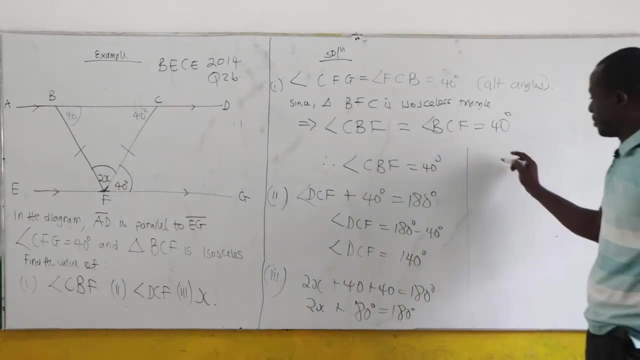 So we have 2X plus 40 equal to 180 degrees. Now let's see: So we have 2X equal to 180 degrees minus 80 degrees, So we have our 2X to be equal to 100 degrees. 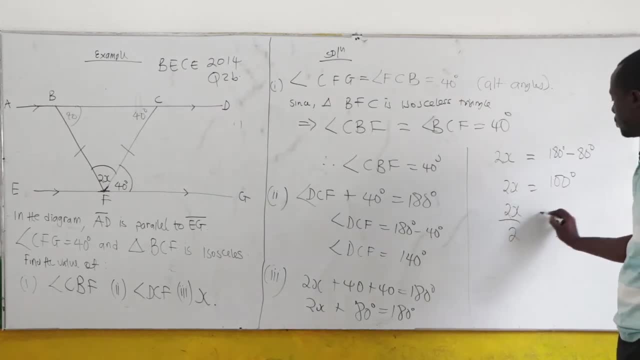 Don't find X, Don't find X, We divide both sides by 2.. So 2X all over 2, equal to 100 degrees all over 2.. So this is canceling that X, 100 divided by 2, this is just 50 degrees. 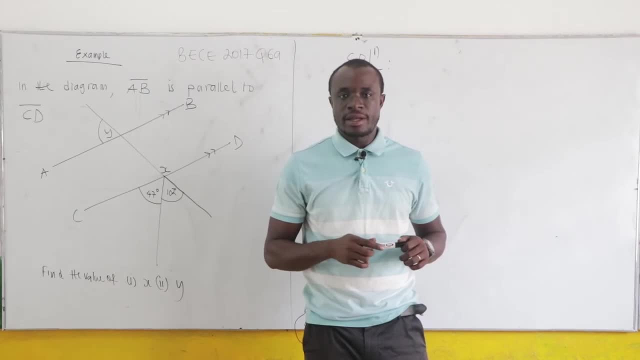 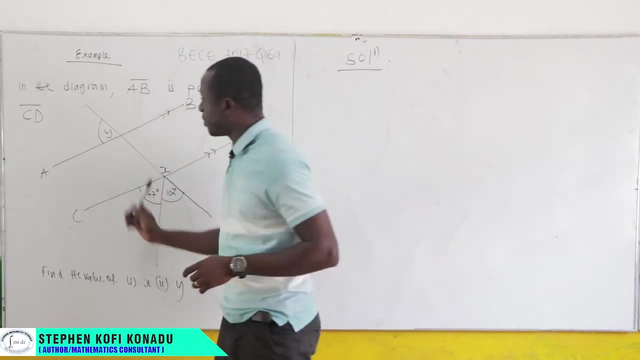 And this is very, very easy and interesting. Now let's consider this past square. This is BEC 2017, question number 6A: In the diagram, AB is parallel to CD, So AB is parallel to CD. 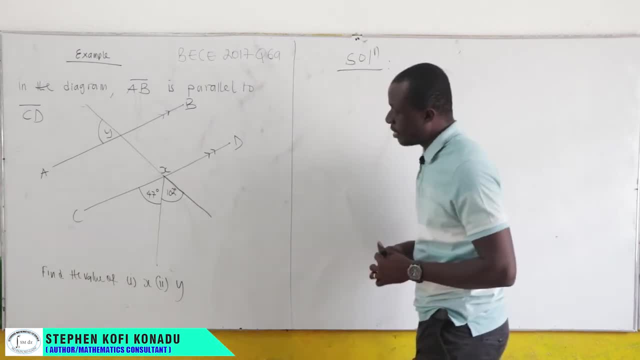 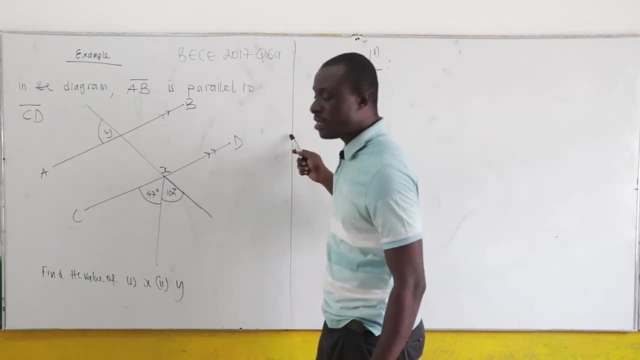 We are being told to find IX and then II. That is why. So this is where X is, We are 47 and then 108, also beneath it. Now let's see, Because this CD is a straight line, This transverse is a straight line. 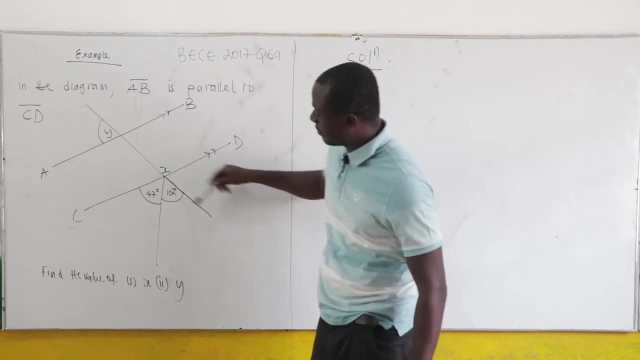 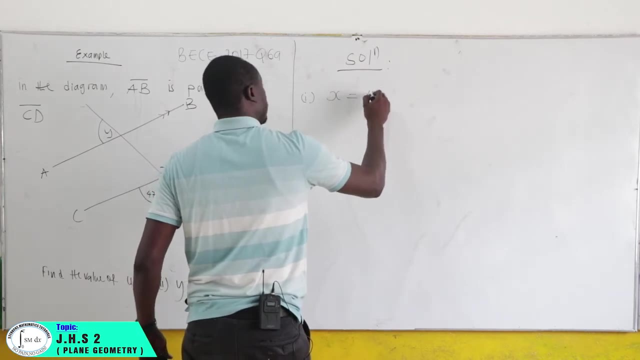 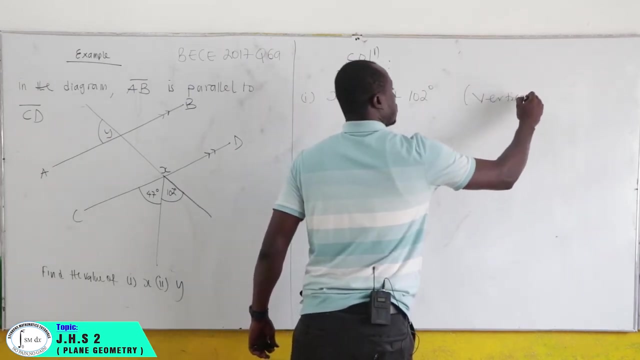 So what can we see? We have vertically opposite angles. The angle here is equal to the angle over there. So we can say that X is equal to 47 degrees plus 102 degrees. What's the reason? Vertically opposite: 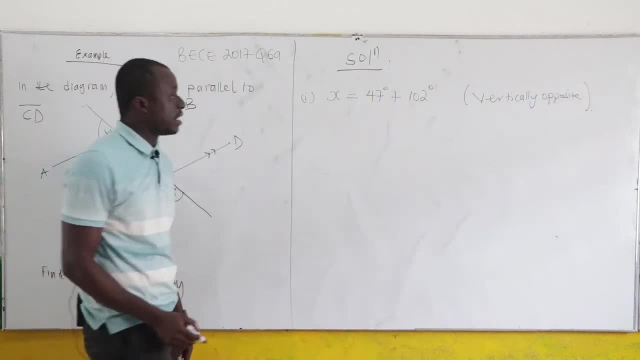 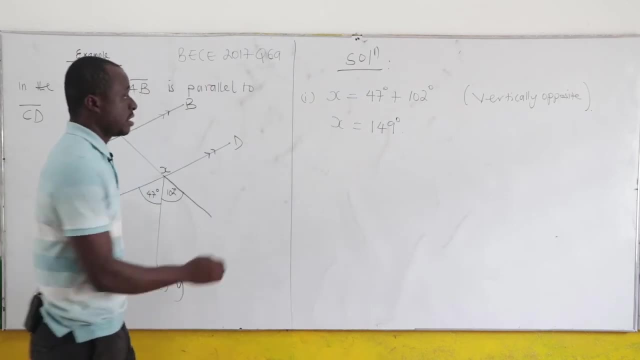 Now what is? 47 plus 102 degrees? This is 149 degrees. Vertically opposite angles. Now let's see the second one. Let's see the second one. Now let's see the angle here. Y is vertically opposite to the angle over here. 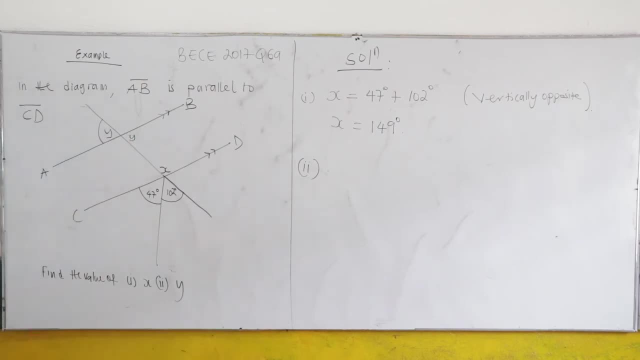 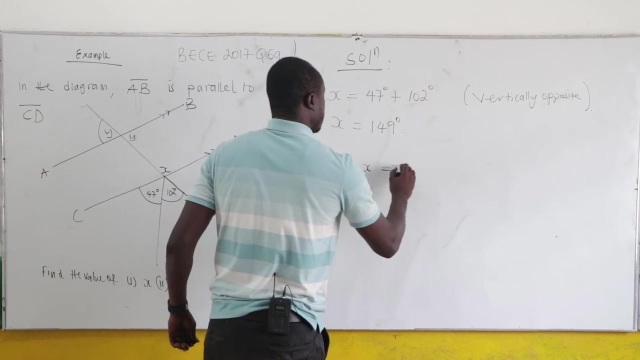 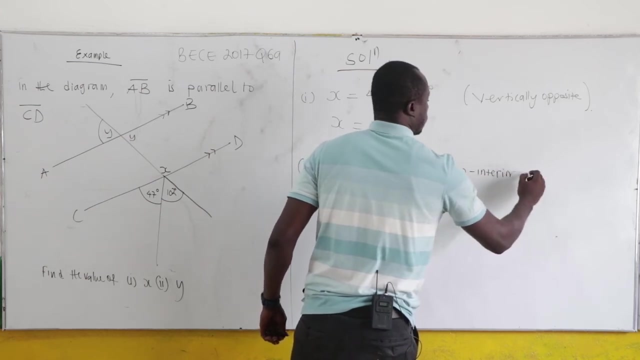 So this is the same, The Y is the same over here, And then I can say: this plus this, equal to 180.. So Y Plus X, equal to 180 degrees. That is cool interior angles. Cool interior angles add up to 180.. 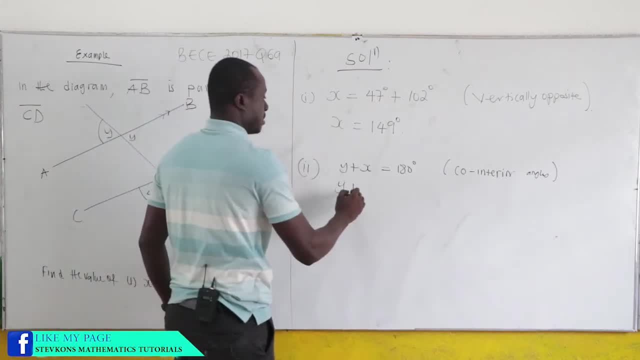 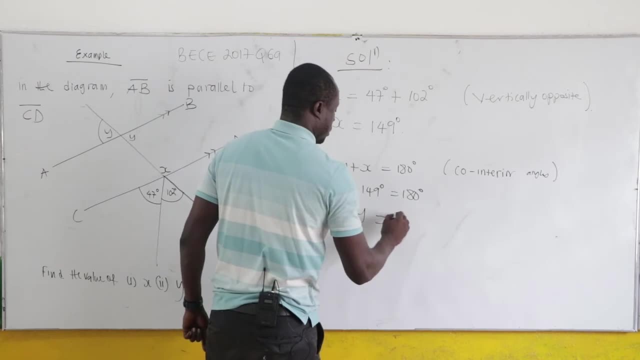 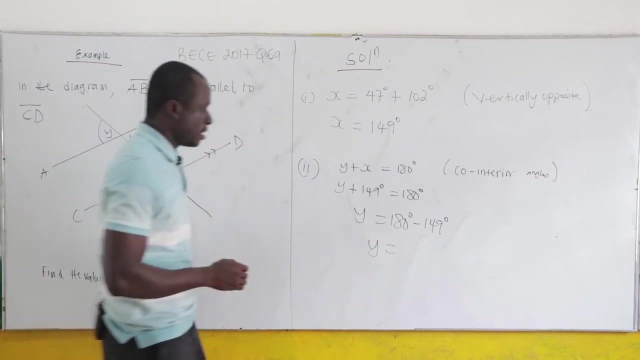 Now, what is my Y? What is my X? My X is 149 degrees, equal to 180 degrees. Clearly, Y is 180 degrees minus 149 degrees. Now, what is 180 degrees minus 149?? Okay, And this is just. that is 31 degrees. 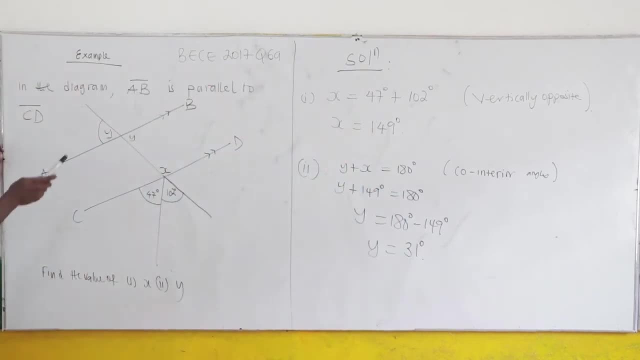 And this is very, very easy. Or you can see that the angle here is corresponding to the angle over there, Or this is alternating to this, Some of angles on the straight line equal to 180.. Or we have a straight line here. 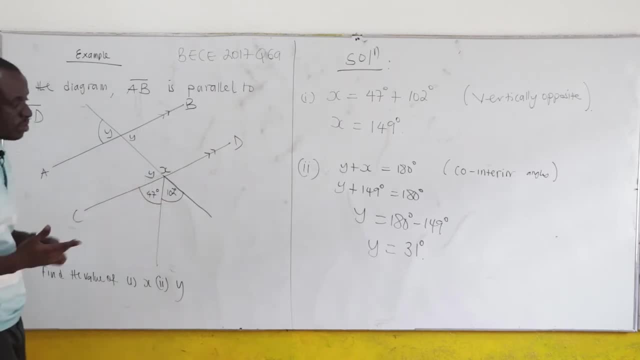 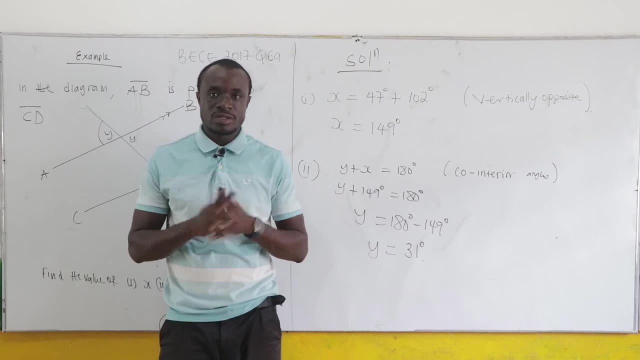 Some of angles on it will be equal to 180.. Any way you want to do it, you'll be able to get it. So this is BEC 2017, question number 6E. Very, very easy. Let's consider. 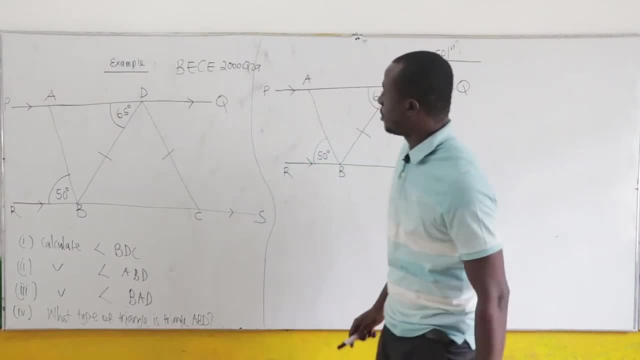 Let's consider the next example. Now let's consider this past. This is BEC 2000, question number 2A. Now we have been told So clearly: PQ is parallel to RS And then DB transversal. 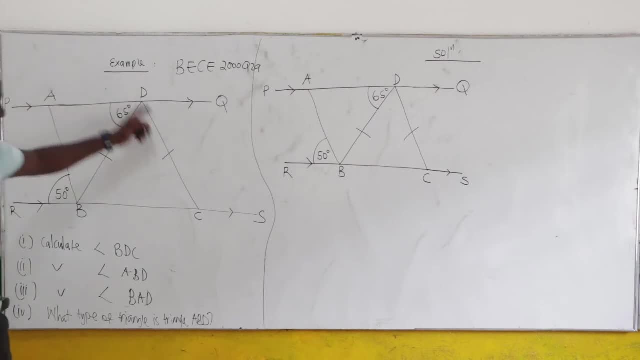 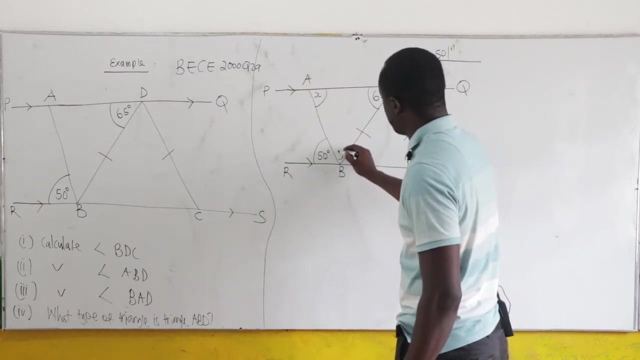 AB transversal. DC is also a transversal. Now let's replace the inner angles with variables. So let's suppose that the angle here- Let's say this- is X. Now let's say this is X. Now let's suppose that the angle here is Y. 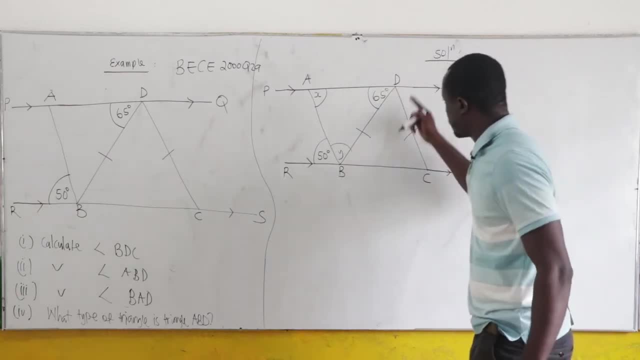 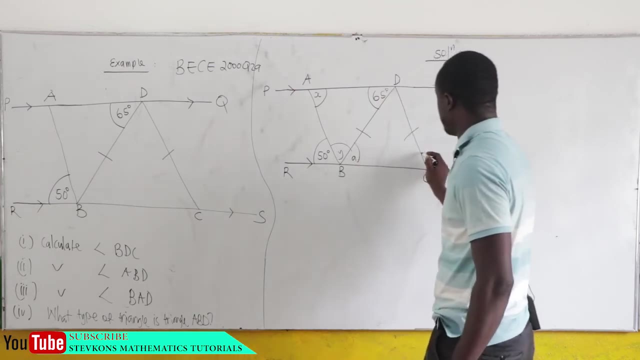 Now, let's suppose that Now DBC is isosceles, This side is equal to that side. So let's suppose that the angle here is A, And if this is A, this side too will be equal to A. 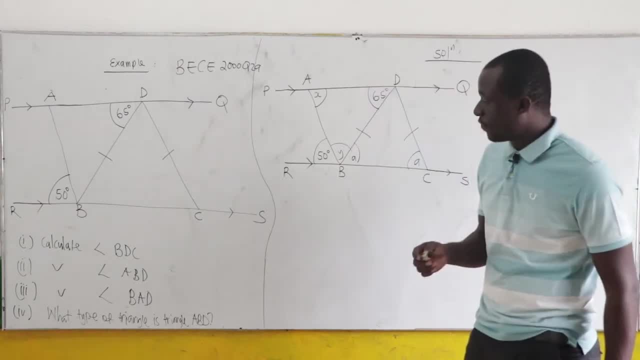 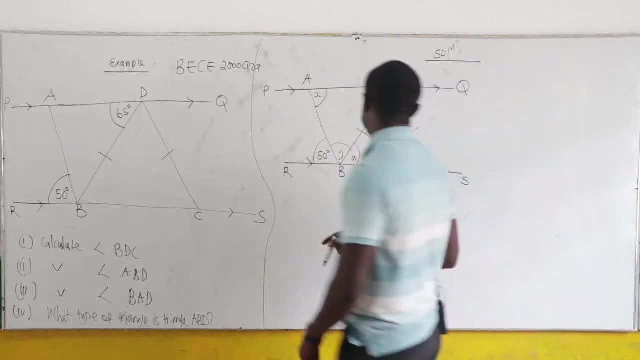 Now the first one says we should find BDC, BDC. We want to find the angle over here. Now let's see Clearly, what can we see? If this is 65,, this is also what 65.. 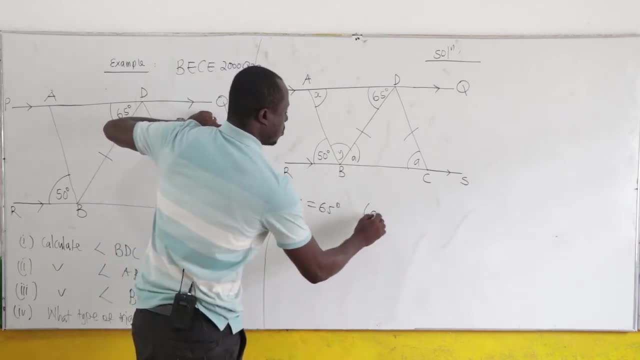 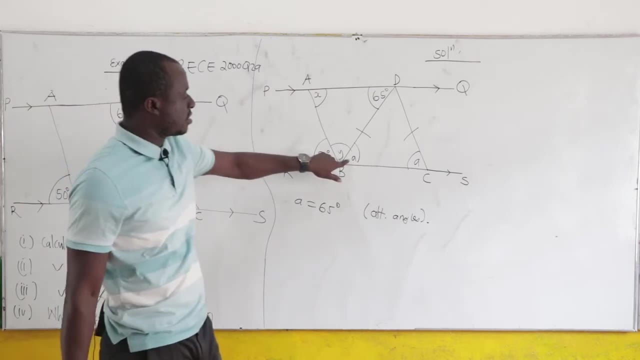 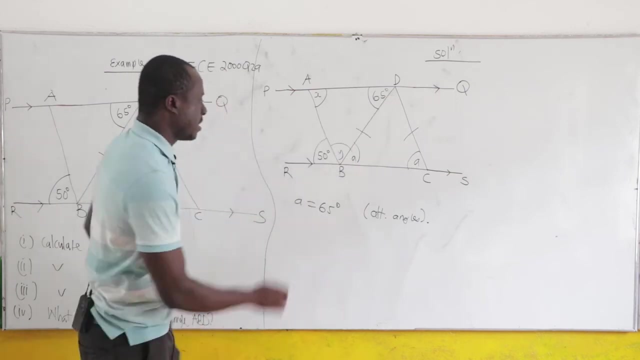 So A is equal to 65 degrees alternate angles. Now, if this is 65, hence this side would also be called 65.. So for us to find the angle over here, this is 65,, this is 65.. 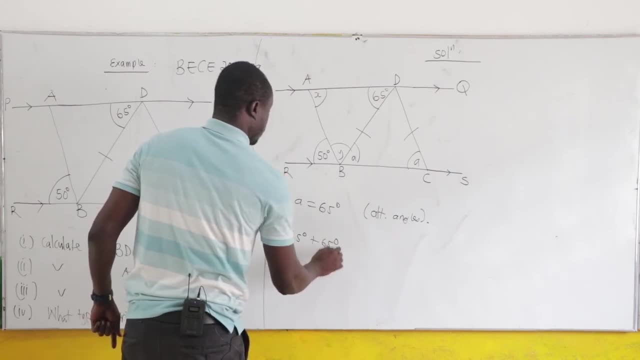 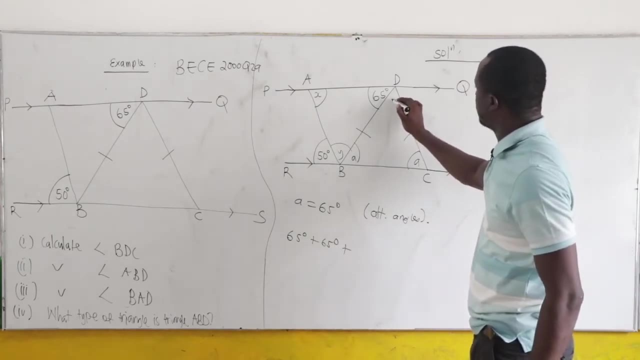 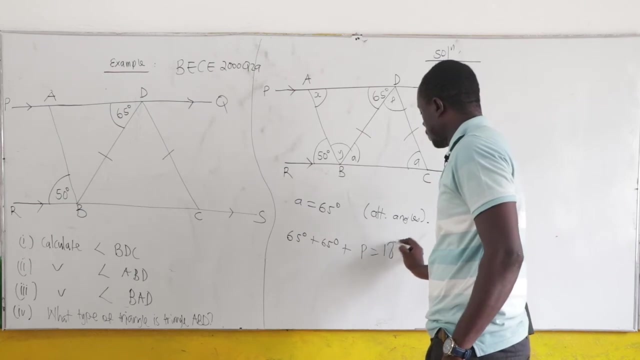 So 65 degrees plus 65 degrees, Plus The angle over here. Now let's suppose that the angle over there, let's suppose that it is P, Let's suppose the angle here is P, So plus P equal to 180 degrees. 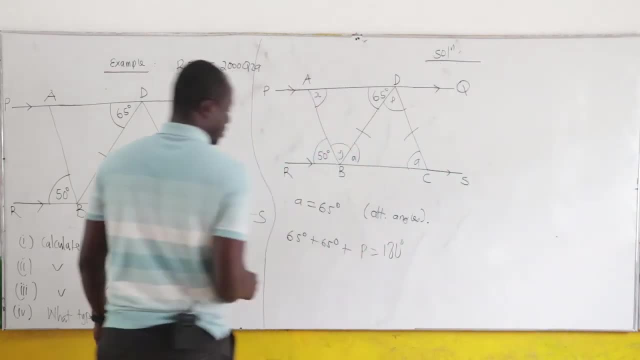 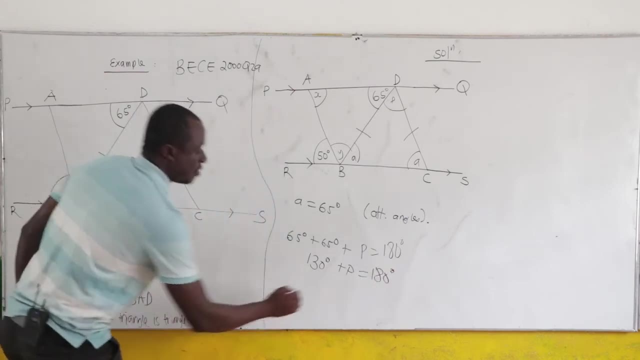 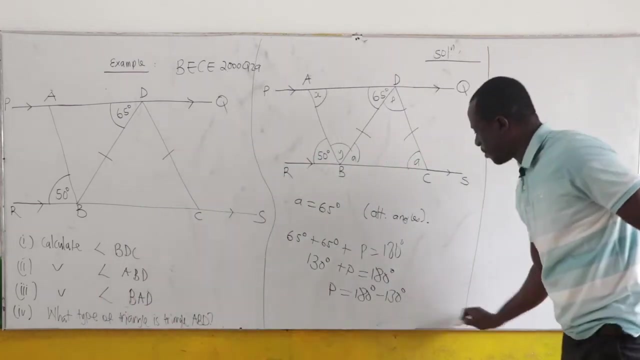 Sum of angles in a triangle equal to that. Now what is 65 plus 65?? This is 130 degrees plus P, equal to 180 degrees. Hence our P is 180 degrees minus 130 degrees. Now what is 180 minus 130?? 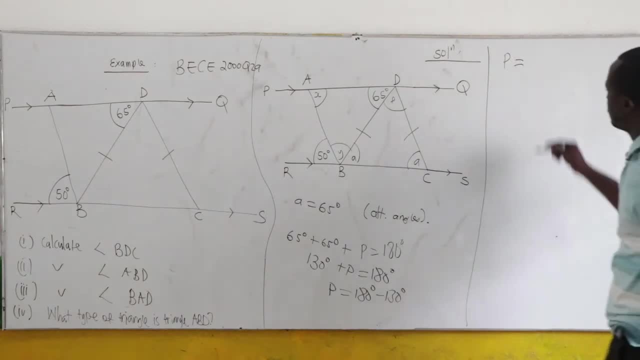 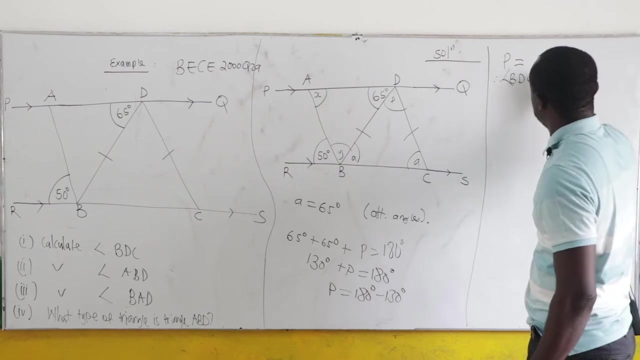 Clearly, at 180 minus 130, this is 50 degrees. So we have our P to be equal to 50 degrees. What is the name of the P? That is BDC, So BDC. Therefore, BDC is equal to 50 degrees. 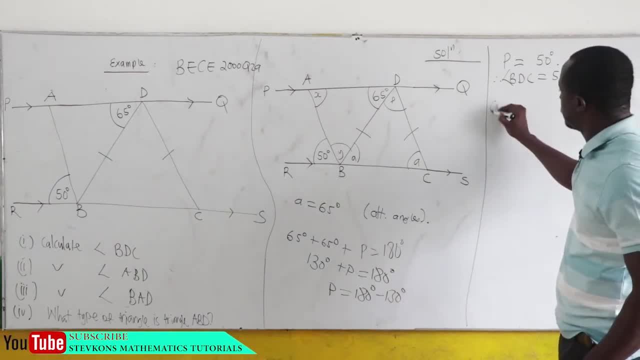 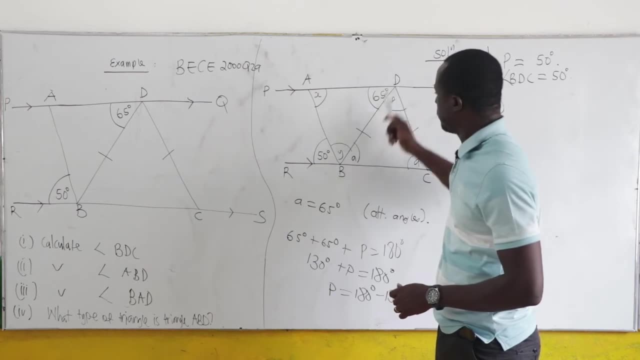 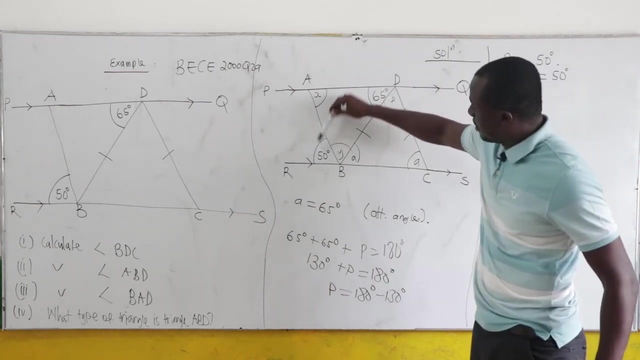 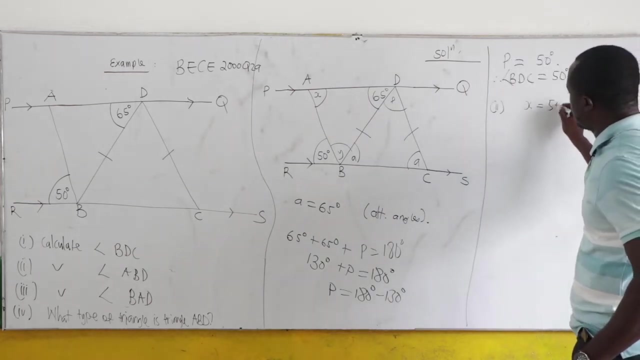 Now let's see the second one. We want to find ABD, That is ABD. We want to find the angle over here, ABD. Now, this and this are alternating, So you can see that X is equal to 50 degrees. 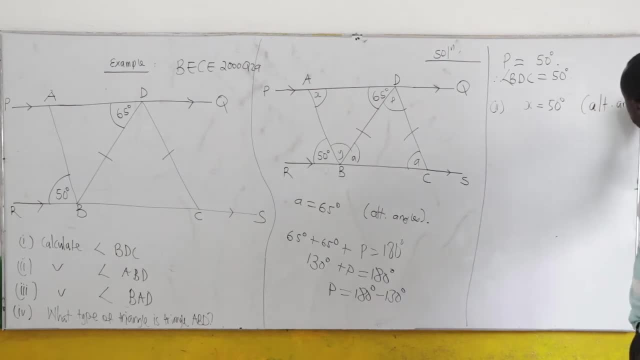 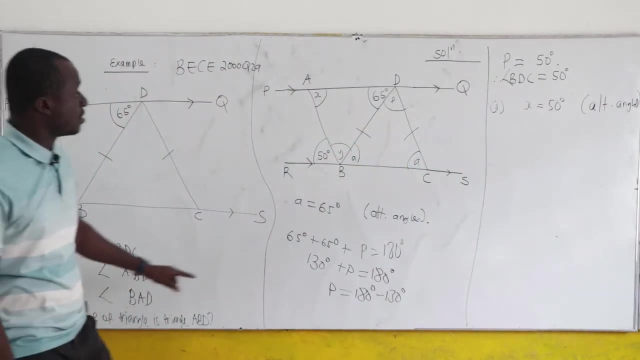 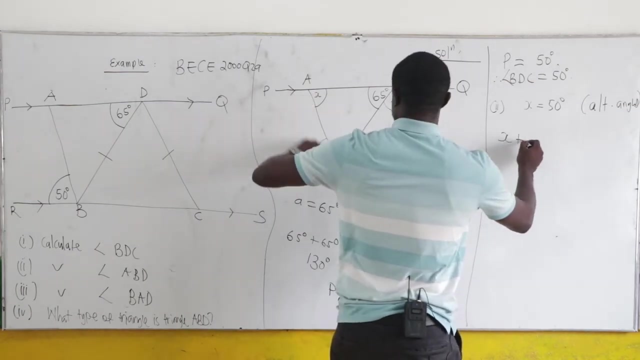 What is the main reason why they are alternating angles? So we want to find the angle over here. Because ABD, So ABD Sum of angles in a triangle equal to 180 degrees. So we have X plus Y plus 65 degrees equal to 180 degrees. 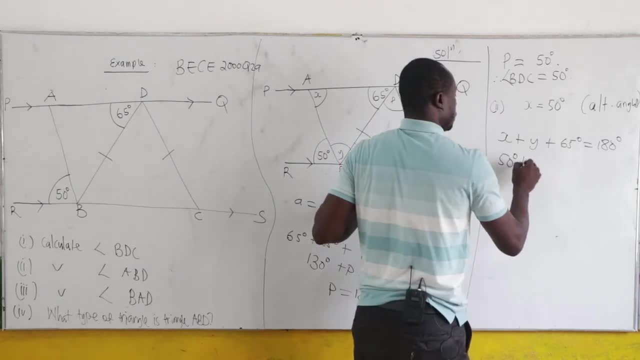 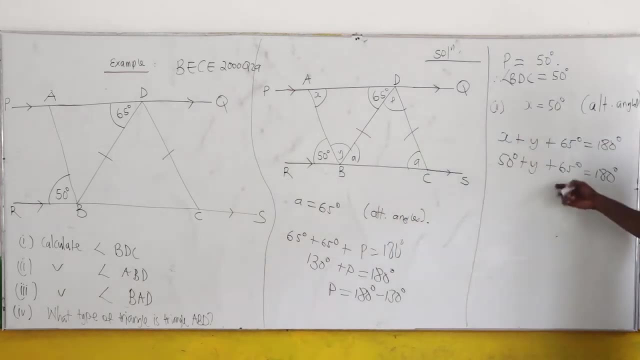 Now what is the X? 50 degrees. So we have 50 degrees plus Y, plus 65 degrees, equal to 180 degrees. Now what is 50 plus 65?? This is 115 degrees Plus Y, equal to 180 degrees. 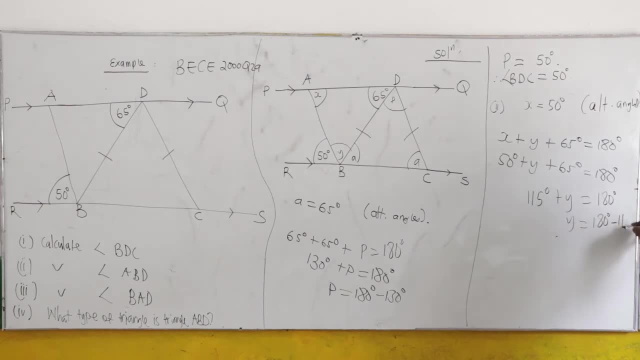 So our Y equal to 180 degrees minus 115 degrees. Now, what is 180 minus 115 degrees? And this is just that is 65 degrees. Hence, what do we want? We want to find that is ABD. 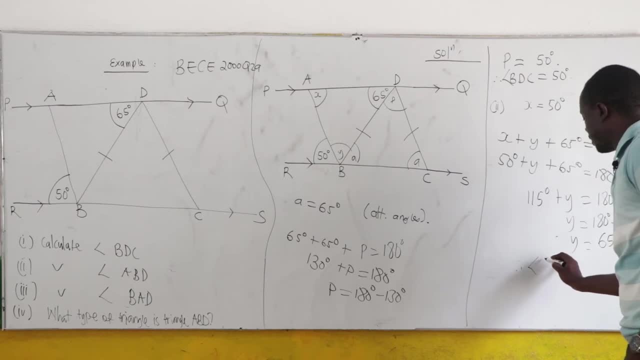 The equation says that ABD, Therefore triangle angle, ABD Equal to Equal to 65 degrees. Now let's see the third one. The third one says we should find BAD, We want to find BAD. Well, BAD is the same as the X. 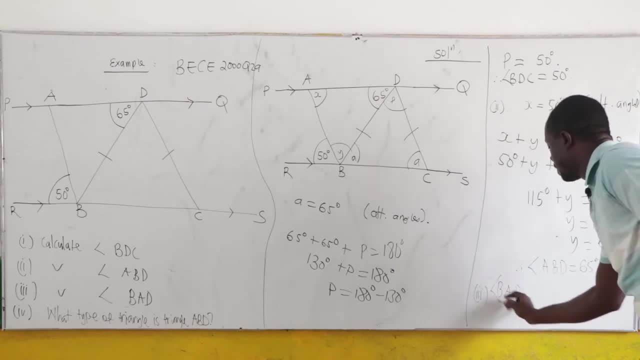 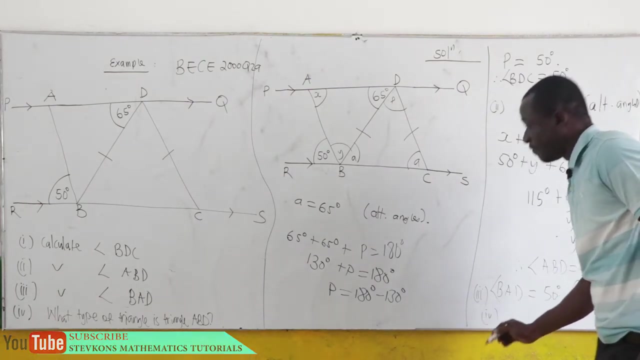 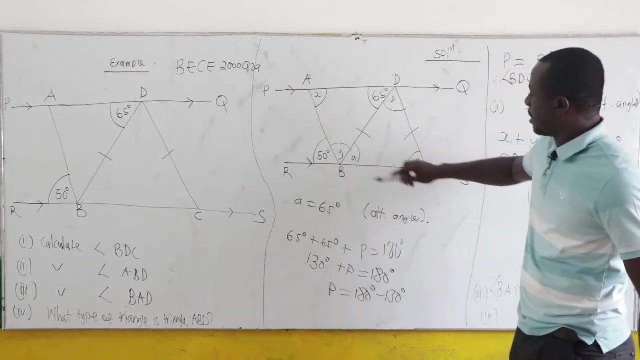 So our BAD is the same as the 50 degrees, which is the alternate angles. Now, what is the fourth question that they've asked us? The fourth question: what type of triangle is triangle? ABD? So ABD. Now we have our Y. 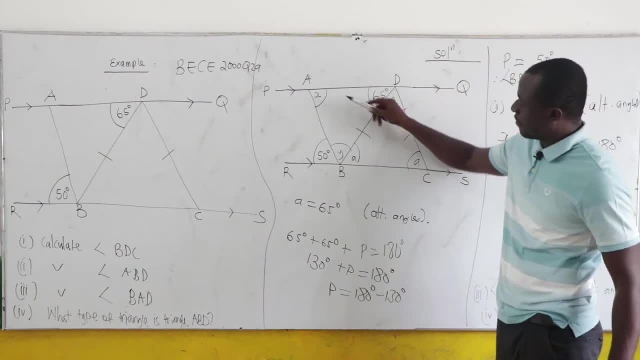 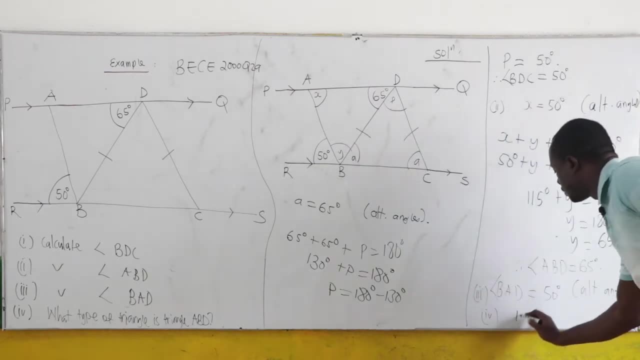 What is our? Y 65. So 65, 65. And the angle here is 50. Clearly this side is the same as this side, which is isosceles triangle. So that is isosceles. 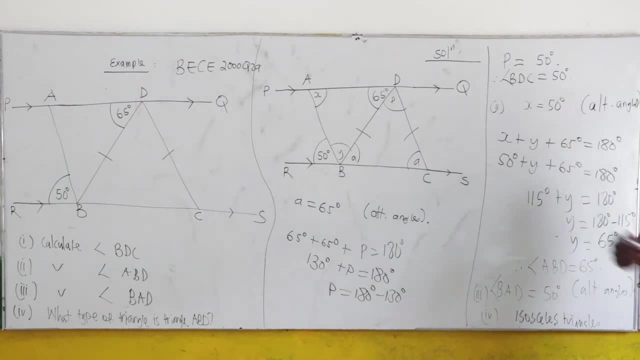 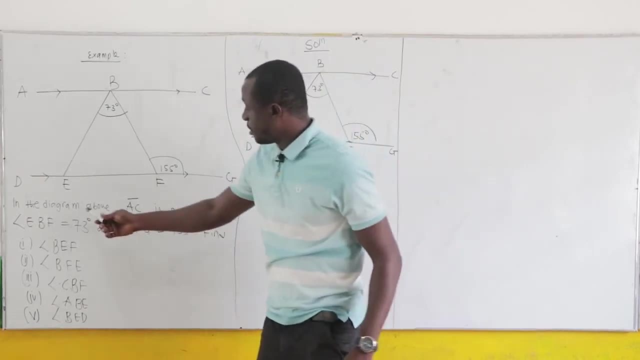 So that is isosceles triangle where the base angles are equal. Now let's consider this example. In the diagram above, AC is parallel to DG. So AC is parallel to DG. Now angles have been given inside. 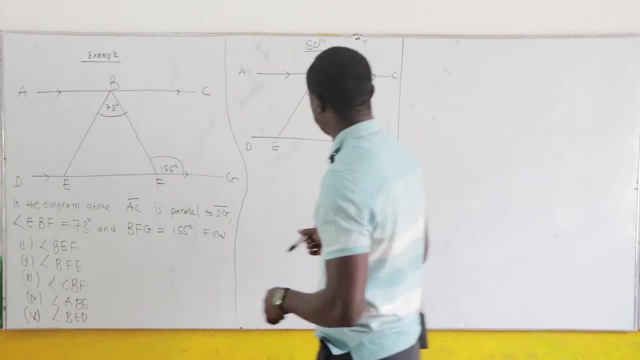 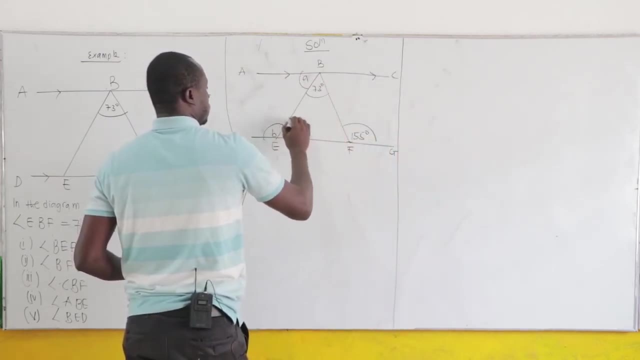 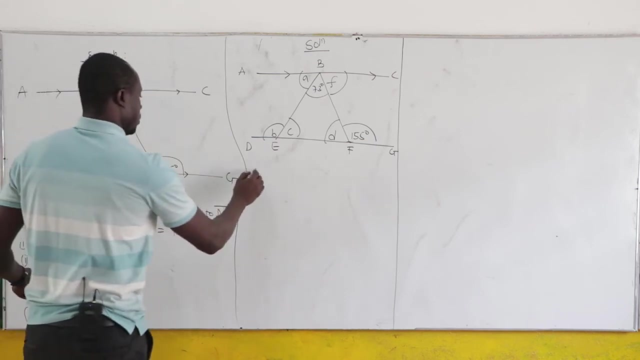 We want to find BEF. Now let's redraw and then let's put variables in there. Let's suppose that this is A, This is B, C, D And then F. Now the first one: we want to find BEF. 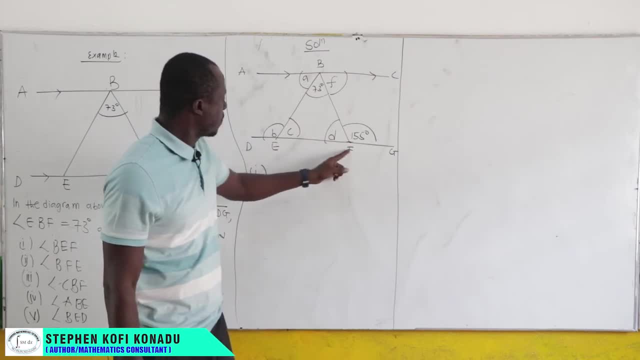 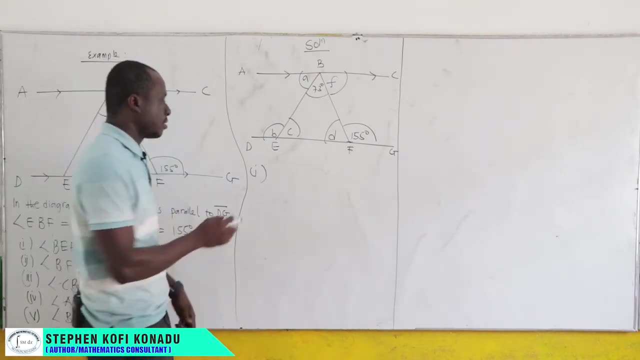 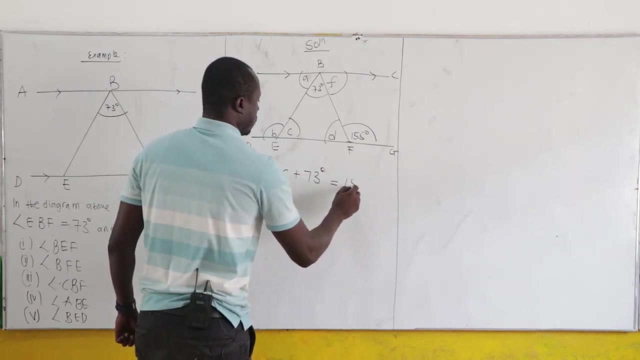 We want to find BEF, So we want to find the angle over here. Now we know that the sum of two opposite interior angles is equal to the exterior angle. So C plus 73 degrees equals 155 degrees. So we have our C to be equal to 155 degrees. 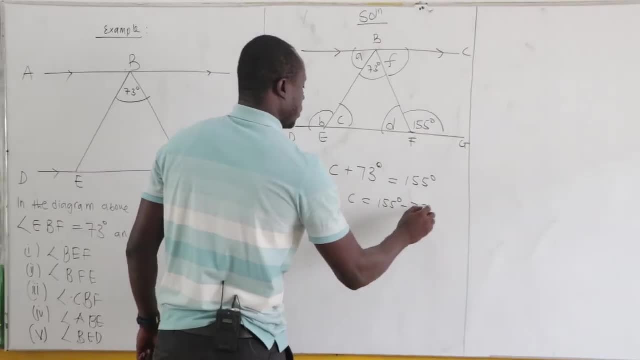 So we have our C to be equal to 155 degrees. So we have our C to be equal to 155 degrees. So 155 degrees minus 73 degrees, Which equals the interior angle, Which equals the exterior angle, 155 degrees. 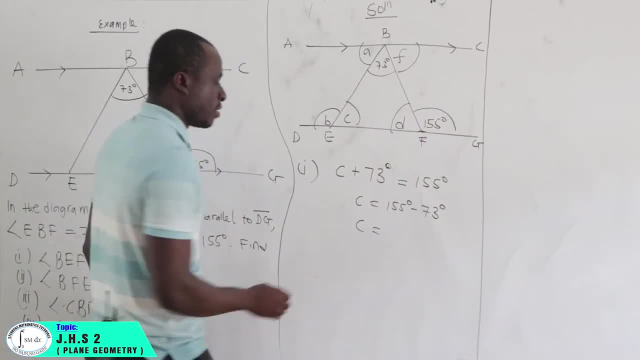 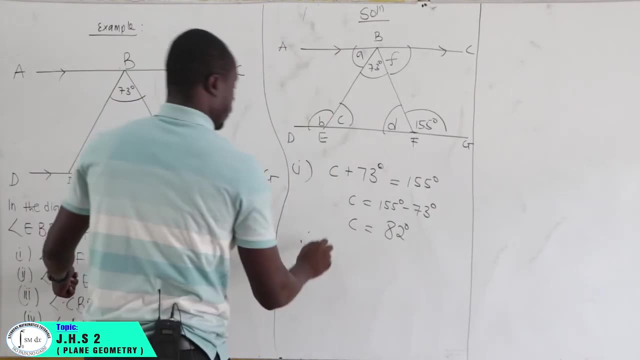 155 degrees minus 73 degrees, 155 degrees, This is just 82 degrees, This is just 82 degrees. Therefore, the first one BEF, Therefore the first one BEF, BEF, BEF, Equal to that, is 82 degrees. 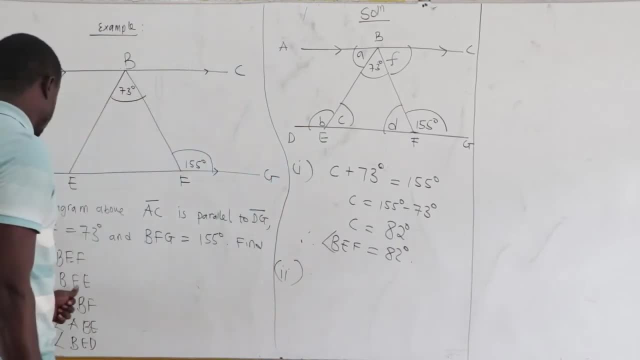 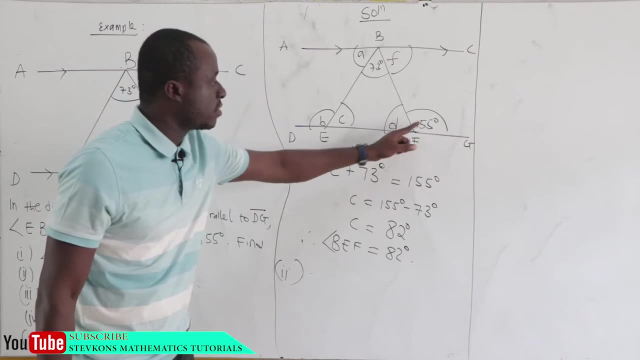 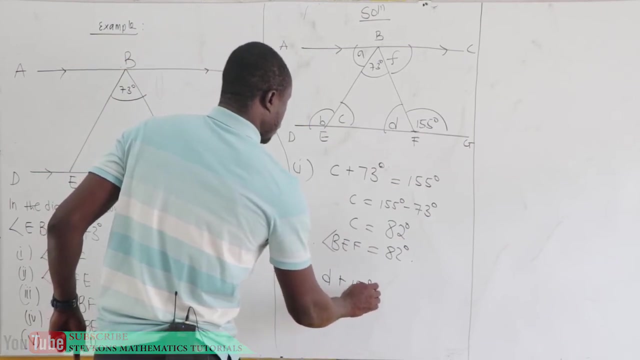 Equal to that is 82 degrees. Now let's see the second one: BFE. you won't find the angle over here. now this is straight line, sum of angles on the straight line equal to 180. so what can we say? you can say: D plus 155 equal. 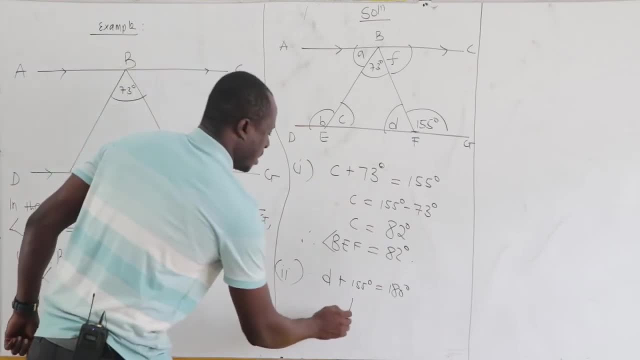 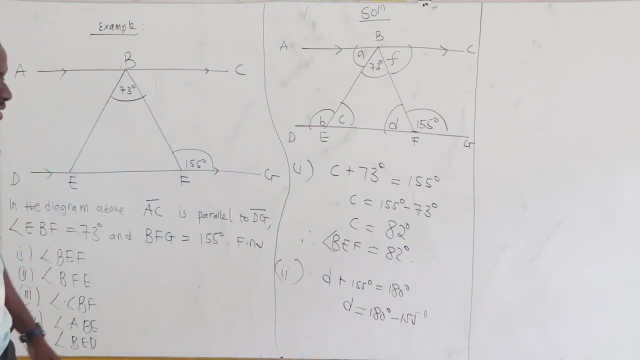 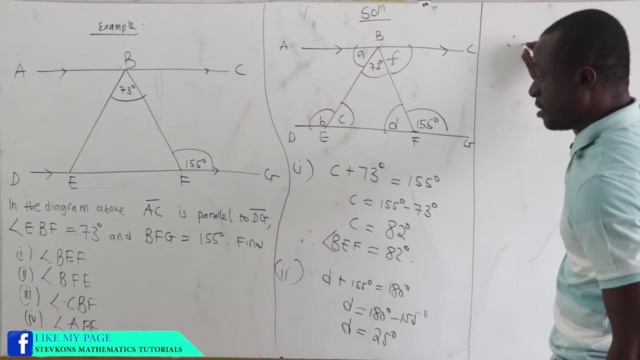 to 180 degrees. clearly our D is equal to 180 degrees minus 155 degrees, but then 180 minus 155, this is just 25 degrees. so our D is equal to 25, so the angle over here is equal to 25 degrees. hence what is the name we are going to define the 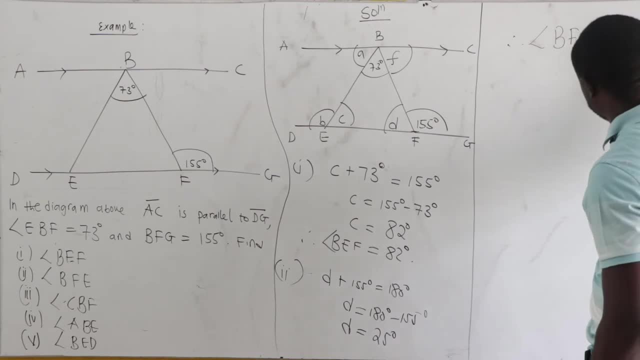 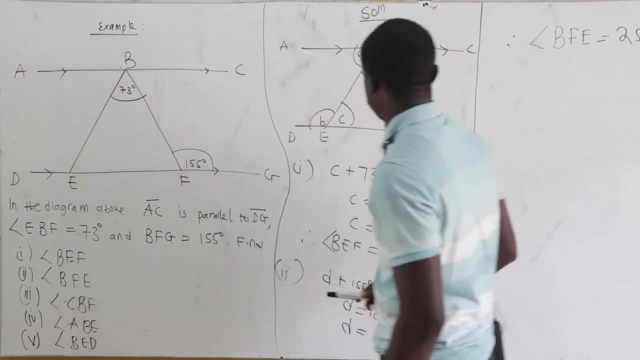 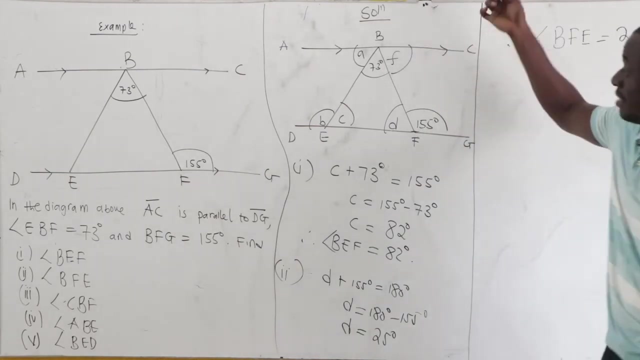 BFE, which is 25 degrees. now what's the next one? we should find CBF, CBF. where's our CBF? now, what? this plus this, equal to 180, or we can see that this is alternating to this. so the third one, you know, F is equal to D, alternate angles. now what is? 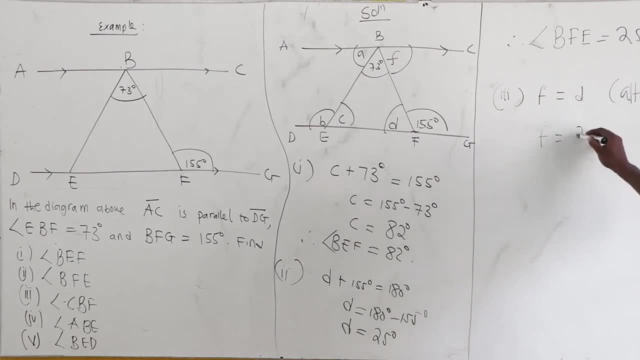 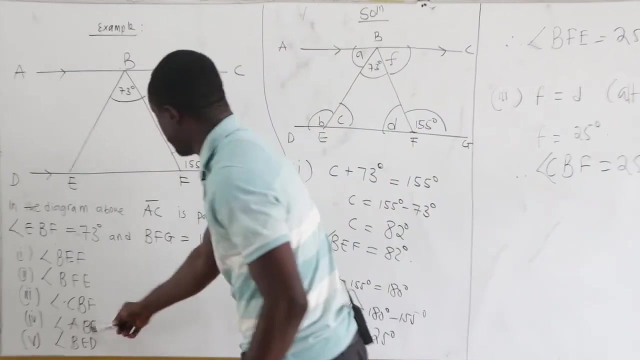 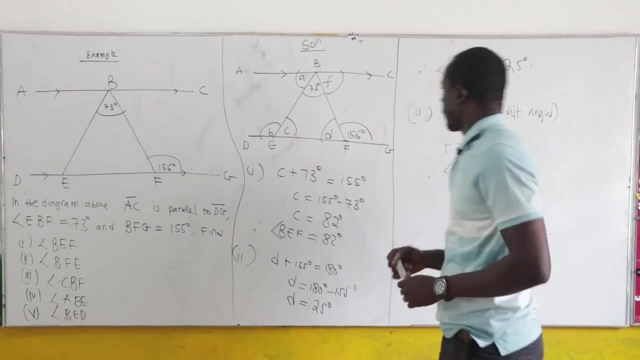 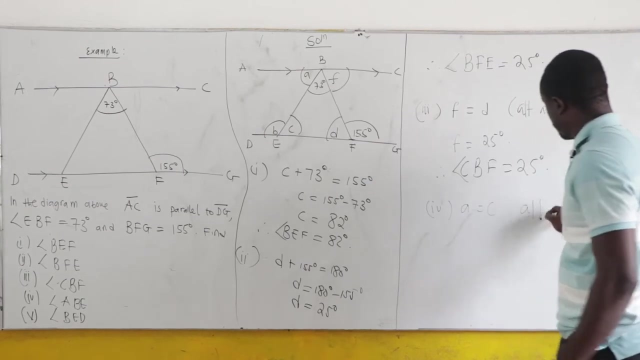 D, so the D is 25. so that's what? 25 degrees, therefore, our CBF, and then CBF is equal to 25 degrees. now what is the fourth one? ABE, ABE, you want to find the angle over here? now A is alternating with C, so you know, A is equal to C. why alternate angles? so? 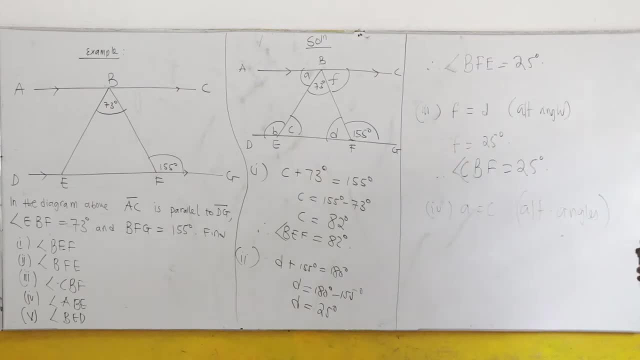 A is equal to C. now, what is our C? we had our C to be 82, so hence we know that our A is equal to C, which is 82 degrees. therefore, A is 82 degrees, hence ABE. ABE is 82 degrees now. 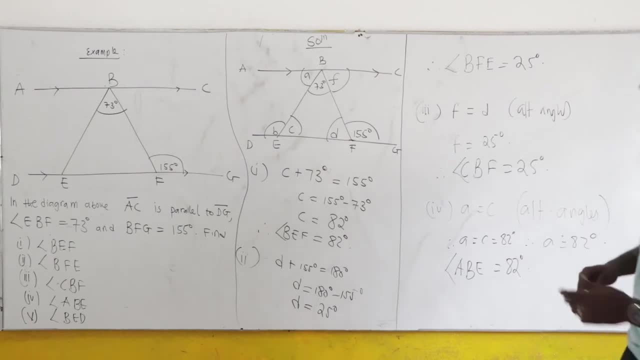 the angle over there, a, b, e, that is 82 degrees. now the vane. what is the vane telling us we should find? b e, d bed, b e, d, b e, d. now, what can, what do we do? c plus d, equal to 180 degrees, that's. 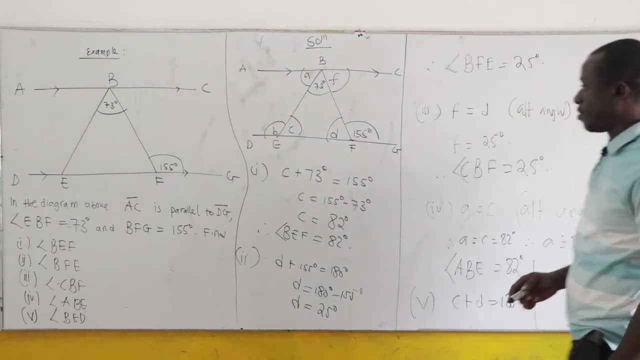 sum of angles on the straight line. so this angle plus that angle, equal to 180 degrees. now, what is c? we had our c to be 82, so we are 82 degrees plus d, equal to 180 degrees. clearly, that d will be what? 98 degrees, so this will be 180 minus that. hence, hence our b e d, equal to 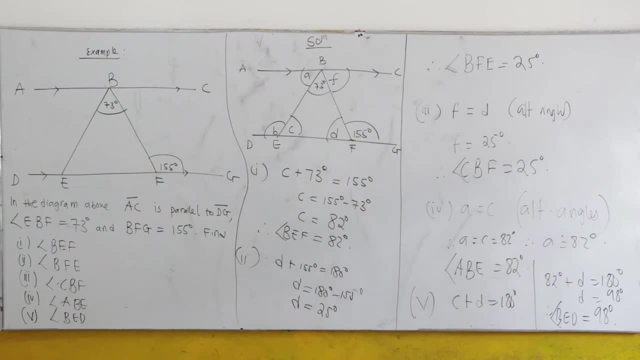 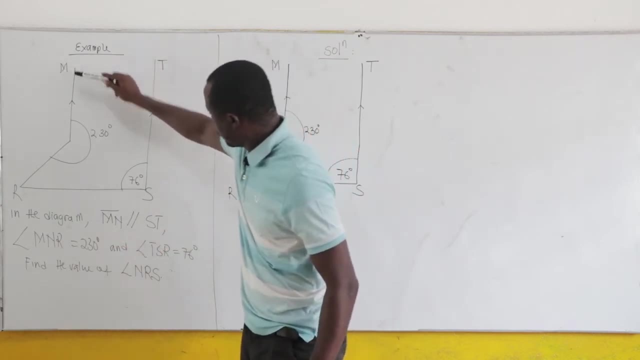 98 degrees. now let's consider this nice example. it is a new diagram: m? n, that is m n, the n is here m n, m? n is power, two s t and then m n r, equal to two times two m n r, that is two, 30 degrees, and t s r. 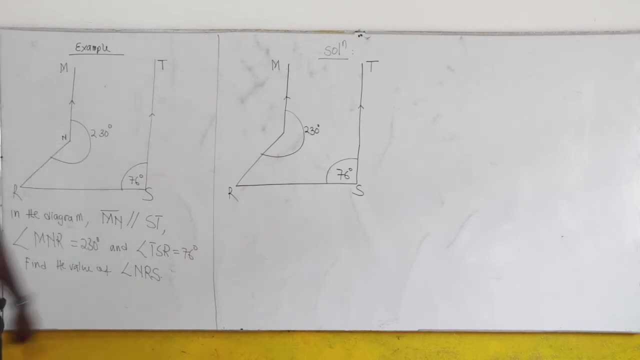 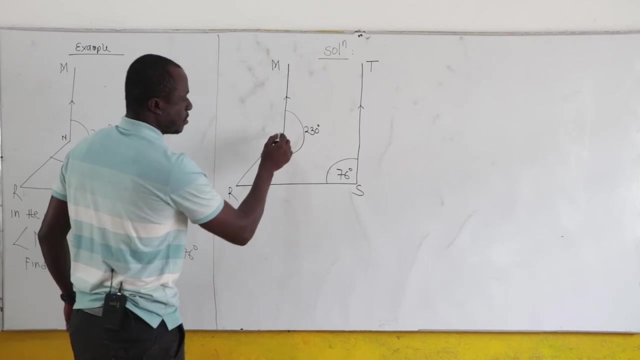 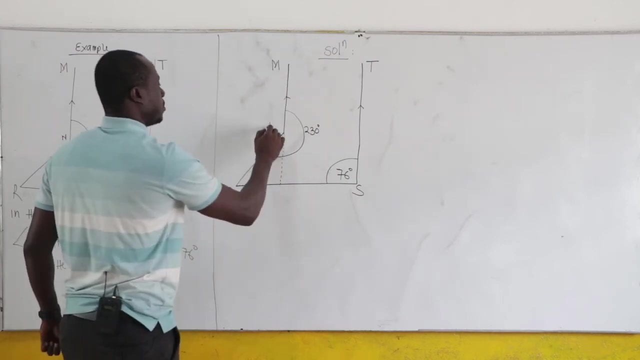 176 degrees now, because this line is power, to this we can extend all the power lines. so the power lines here we can extend it. so i'm redoing it here, so there's a power line and because the power line we can extend it. this short dashes because it is a power line. now let me call this: 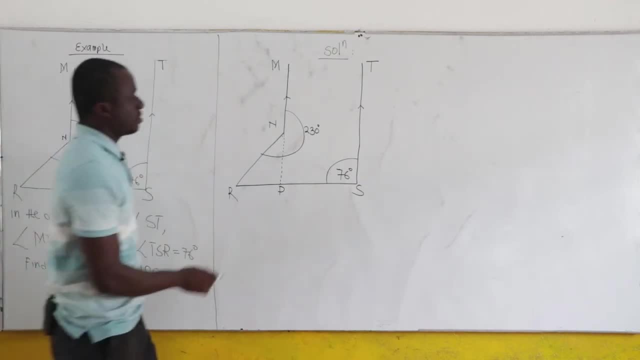 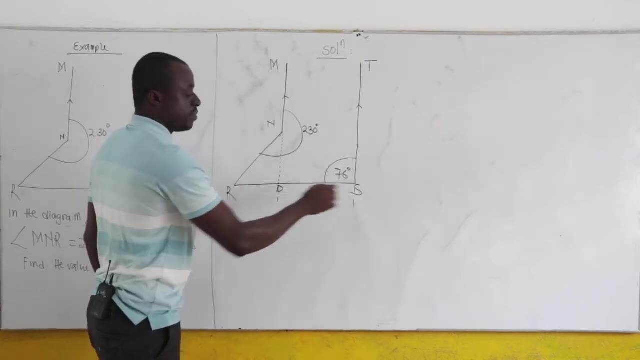 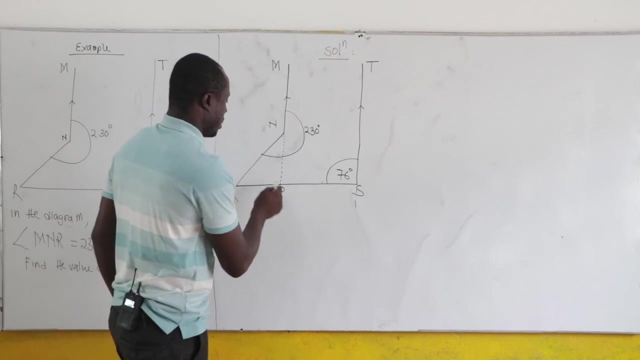 let me call here probably p now, because i have extended this, so this i can extend this to. hence, this is what that is p. you can see ps or rs is a transversal and if it's a transversal, the angle here is corresponding to the angle of i. so if this thing, this is, the angle here is what 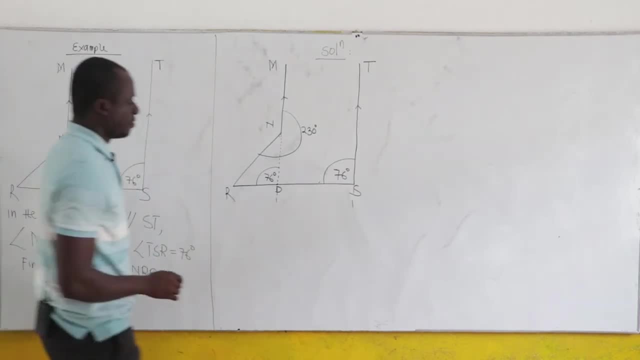 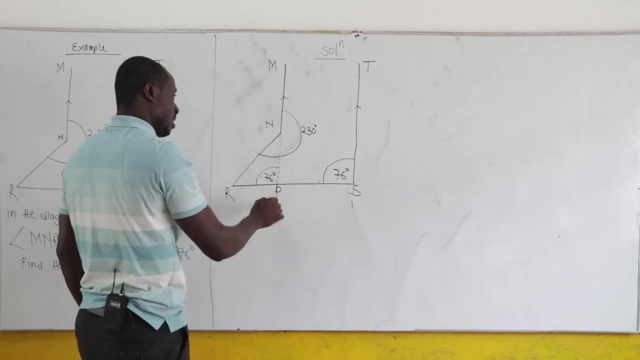 76 degrees. now i know i'm having a triangle here. now this, this whole- you know some of angles on a straight line at a point is 180. so from here all the way to this side, this is 180. so from here all the way to this side, this is 180. so from here all the way to this side. 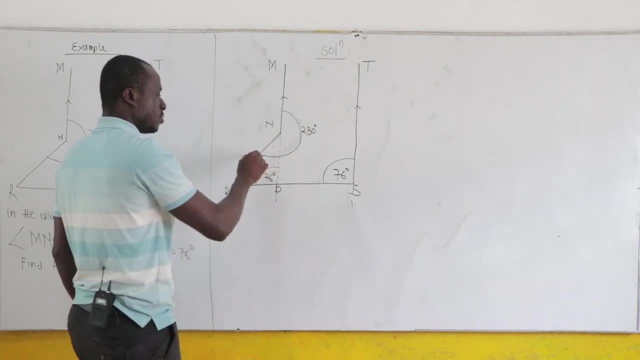 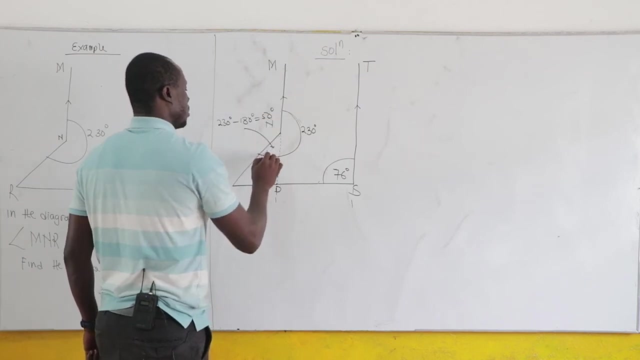 so how do i get this angle? i know the angle all the way from here to here, so 230. so it means that the angle over here, for me to find the angle over here, that would be what? 230 degrees minus 180 degrees, and this is just equal to 50 degrees. so the angle here is 50 degrees. what do i want? 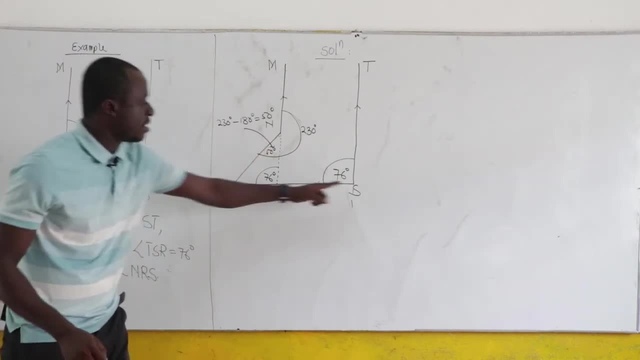 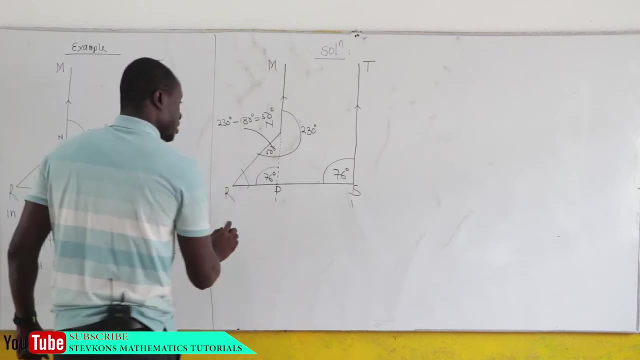 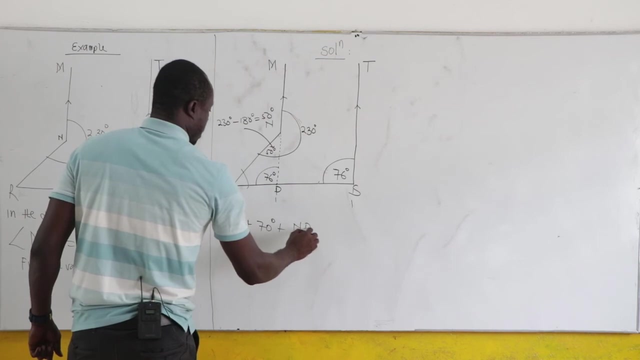 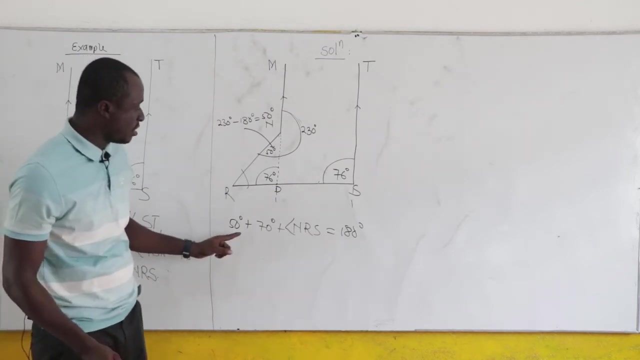 nrs, i want nrs, i want the angle over here now. sum of angles in a triangle, equal to what? 180 degrees? so here we can say: 50 degrees plus 70 degrees plus the nrs equal to 180 degrees, sum of angles in a triangle. now, what is 50 plus 76, not 70, 76, 76. this is just one. 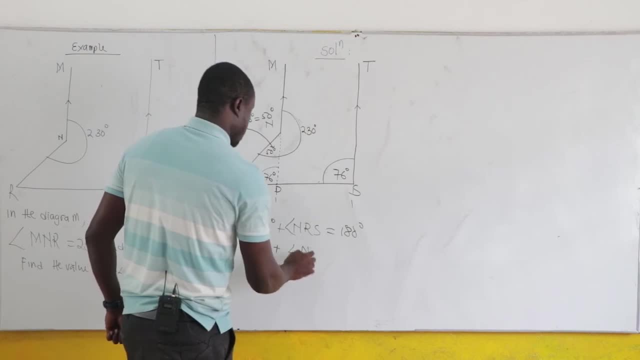 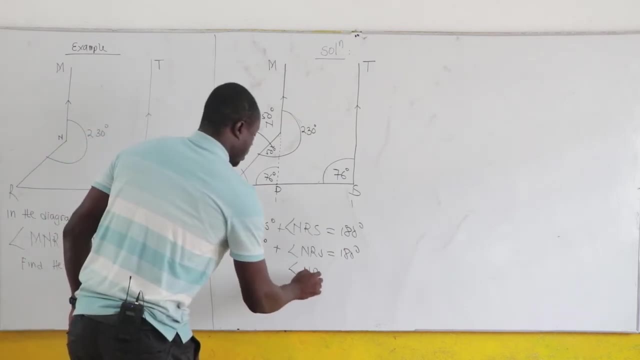 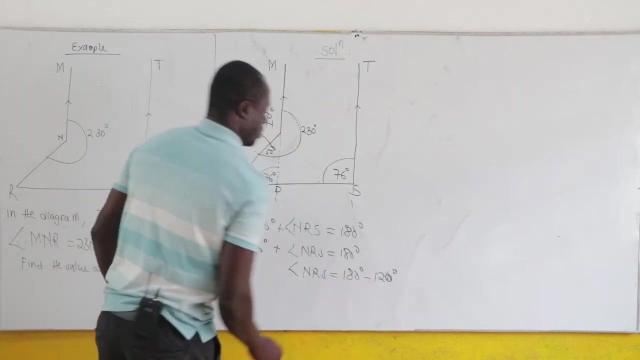 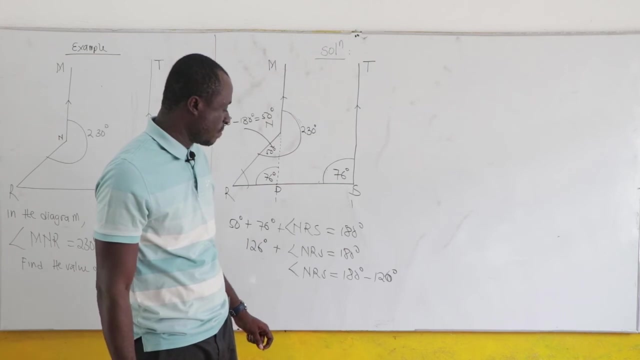 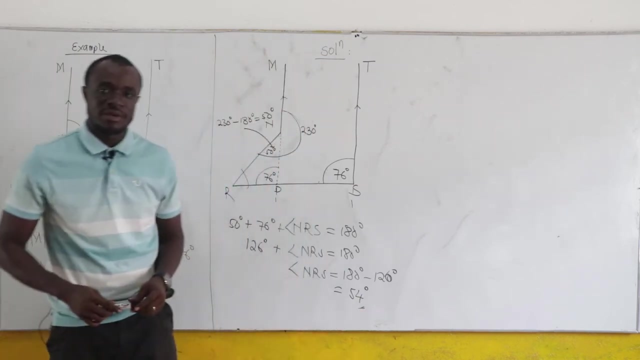 two, six degrees plus angle, nrs equal to 180 degrees. so we have our nrs equal to 180 degrees minus 126 degrees. now let's see: 180 minus 120, that is 60. so 60 minus 6, that's 54. so the angle is 54 degrees. this is very, very easy. 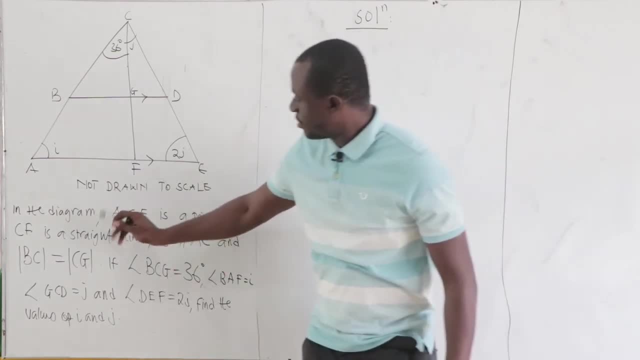 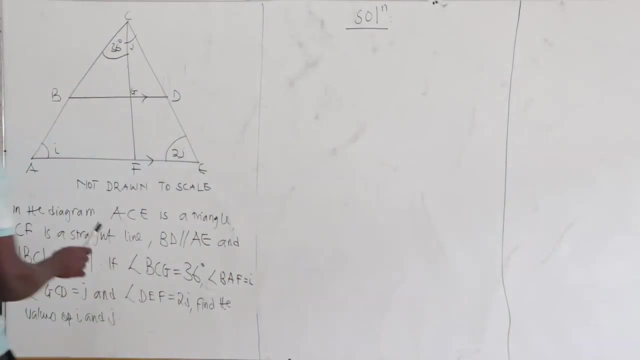 now let's consider this nice example. this is not drawn to scale in the diagram a, c, e. that is, a, c, e is a triangle. c- f is a straight line. so as c- f is a straight line, b d is parallel to a e, b d is parallel to a and b c is equal to c- g, b c is equal to c- j. 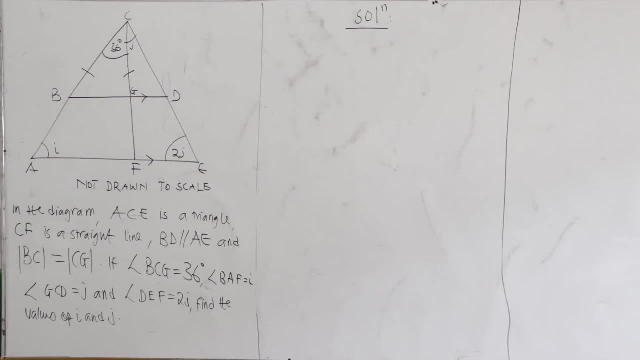 so this and that are equal if b c j is 36 degrees, b c g is 36 degrees, and then b PAF is I PAF is I GCD, J, J, C, D, J and the DEF, DEF, that is 2J, which you find, the values of I and J. 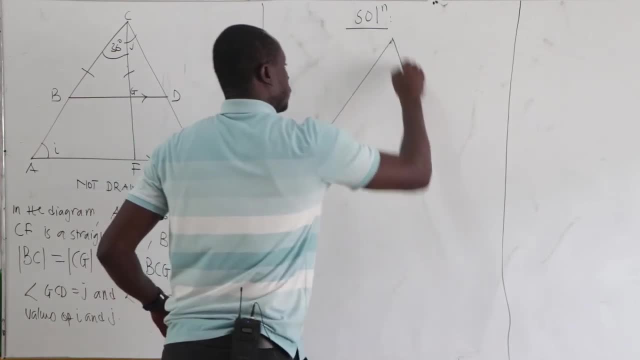 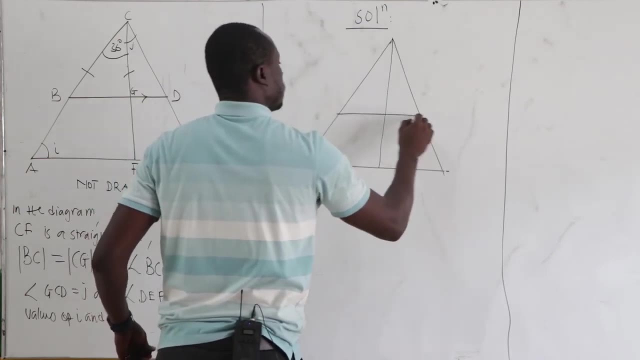 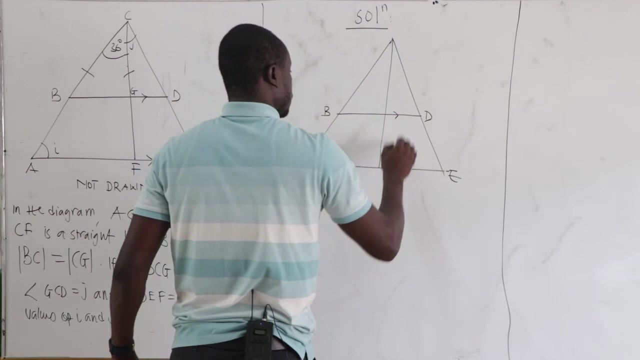 Now let's redraw this And let's consider the straight line. Now we have been told that B- D is parallel to A- A, So this is parallel to this. You know, this side is J. Now this is RC. 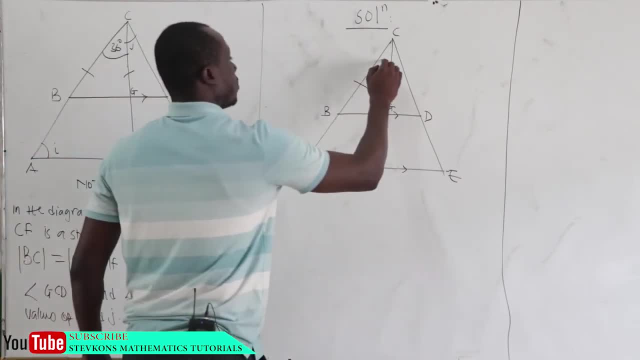 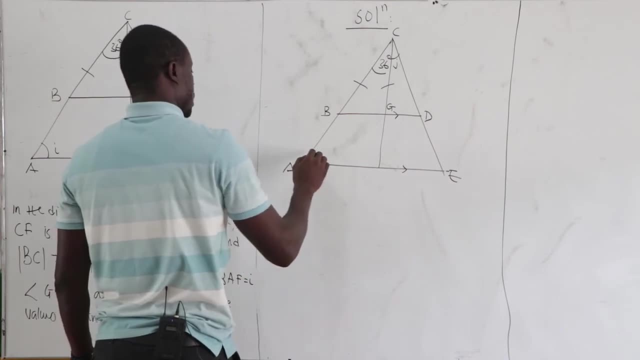 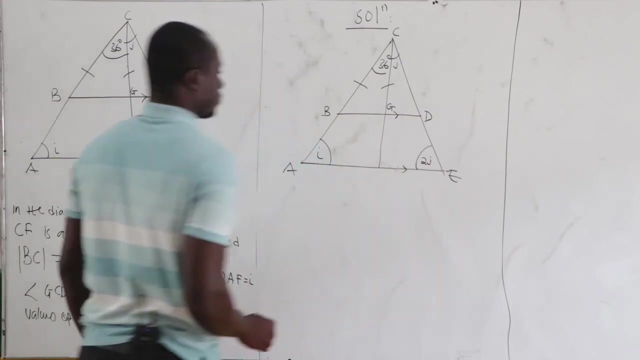 This is equal to that. So we have here to be 36 degrees, We have here to be R, that is J, And then we have here to be I. this is 2,, 2J. Now, this is F. 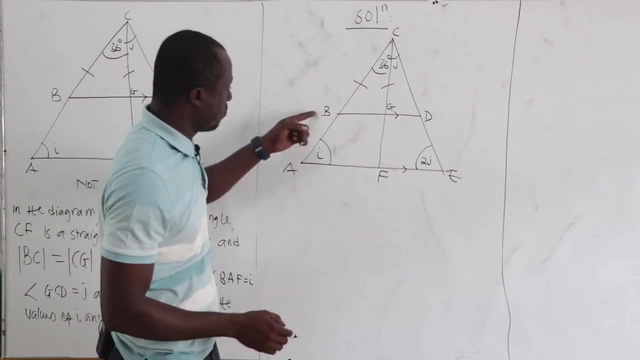 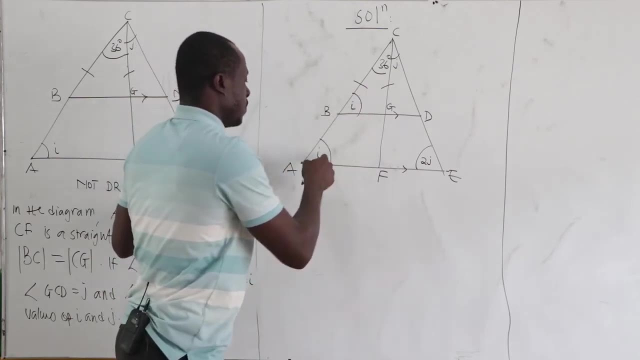 So we want to find I and J Now, because B, D is parallel to A, F, the angle over here is corresponding to this side. So if this is I, this is I- Y corresponding angles. Now, this is a transversal. 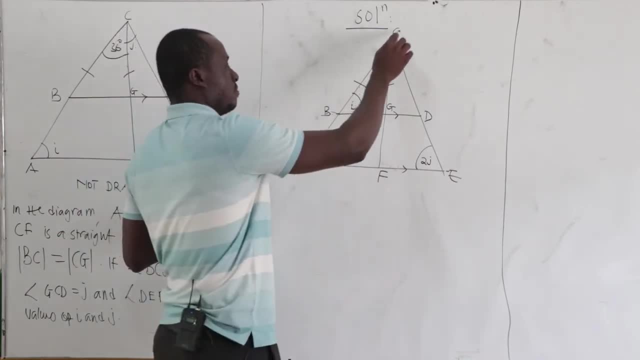 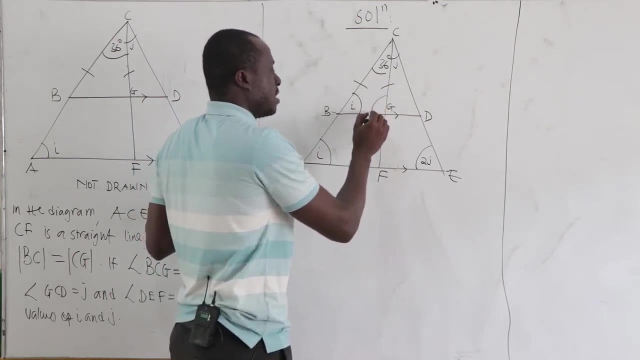 So the angle here is equal to that Now, because B, C, B is equal to C, J. It is an isosceles triangle. So if this is I, this is also I. We have the triangle over this. 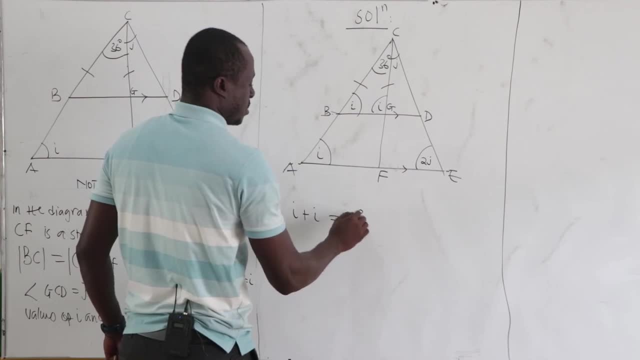 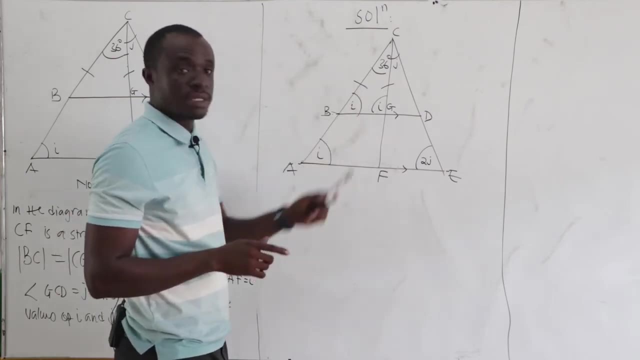 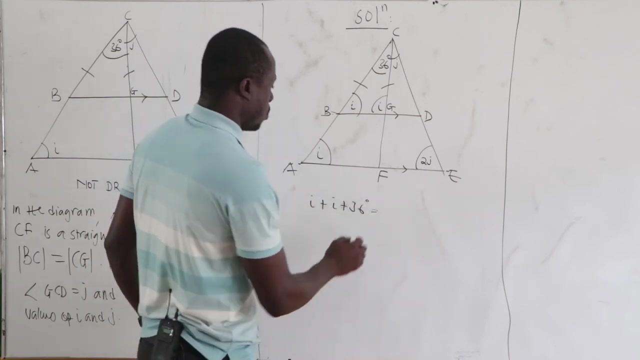 We can see: I plus I equal to 36.. So we have an isosceles triangle Sum of angles and it equals 180 degrees. So I plus I plus 36 degrees This is equal to, That is 180.. 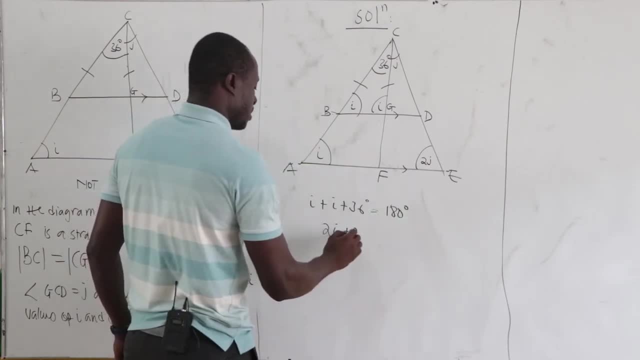 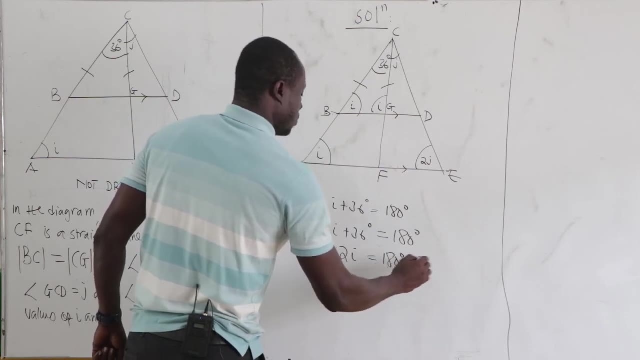 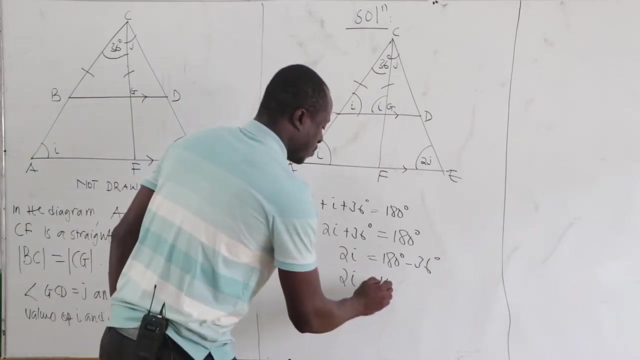 Degrees. So we have 2I plus 36 degrees, equal to 180 degrees. So our 2I equal to 180 degrees minus 36 degrees. So 2I Now 180 minus 36.. This is giving us 144 degrees. 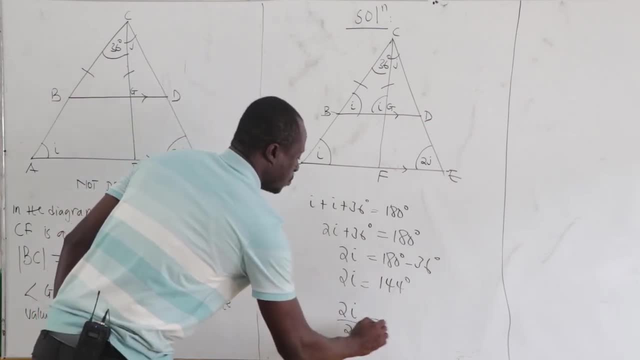 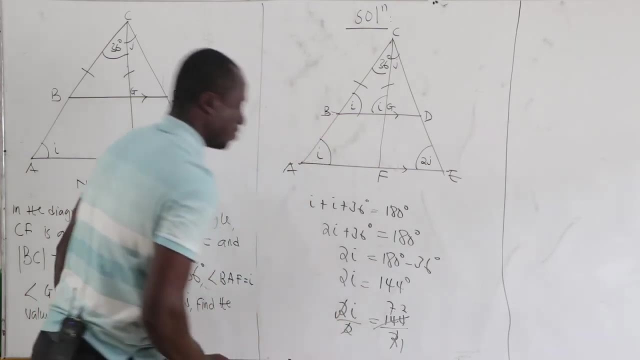 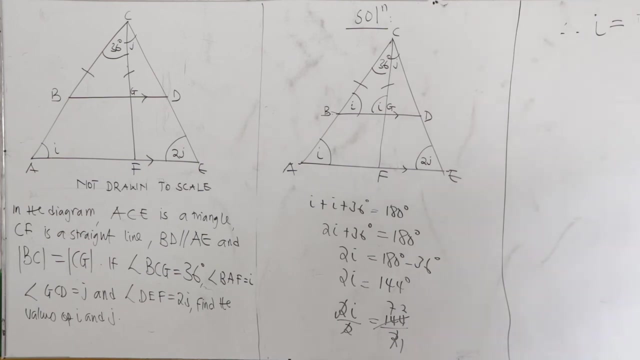 We want to find J, I, So we divide by 2.. So this is canceling. Now there is 2 go here and 2 go here, 7 and then 4.. That is 2.. Here is our. I is equal to 72 degrees. 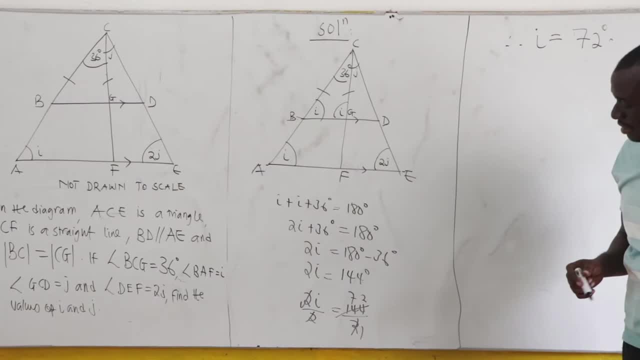 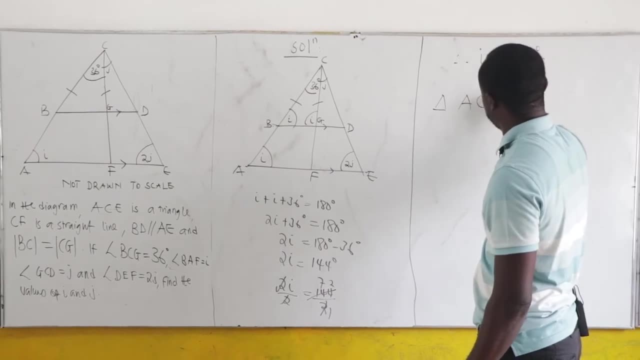 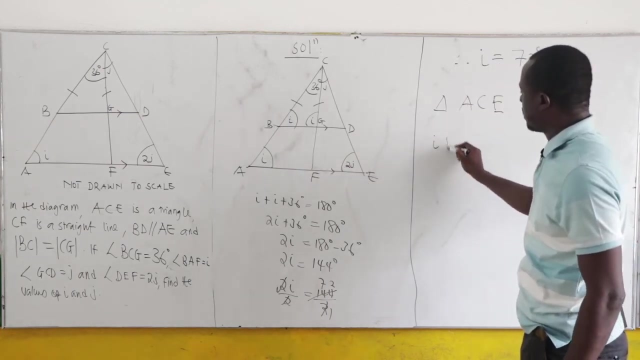 So we are done finding. Now I want to find. That is J. Now we want to find J. Let's consider triangle ACE. We want to consider ACE. Now the angle here this is I. What is the angle here? 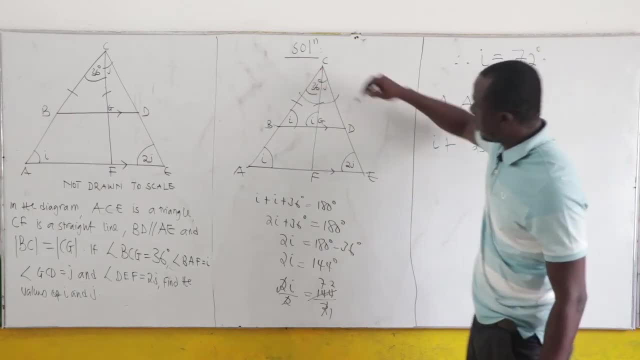 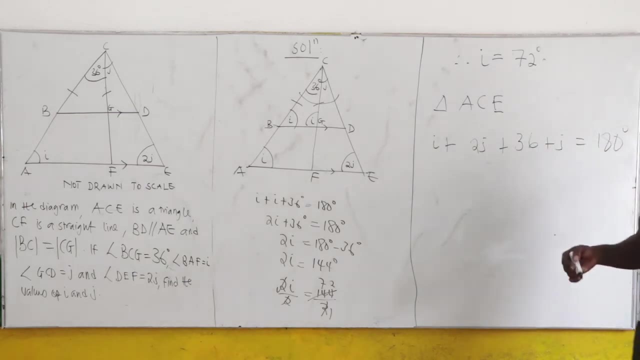 We have 2J. What is the angle here? The whole of the angle here, that is 36 plus J. equal to what? 180 degrees? Sum of angles in a triangle equal to 180 degrees. Now, what is I? 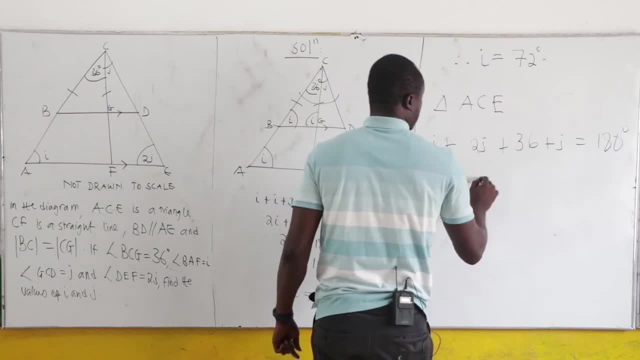 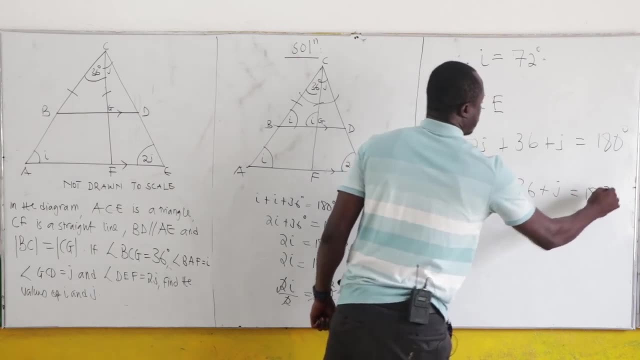 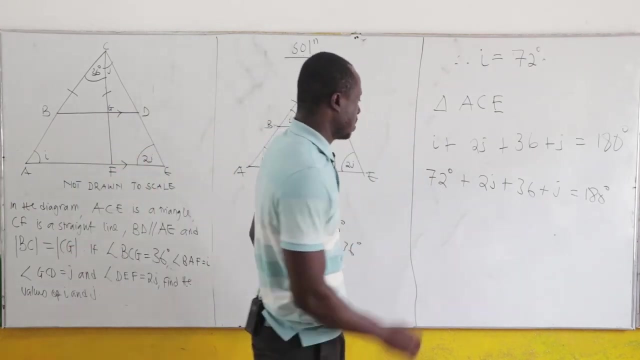 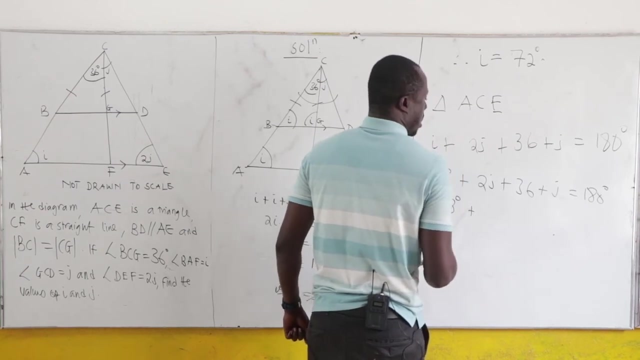 I is 72. So we have 72 degrees plus 2J plus 36 plus J, equal to 180 degrees. Now, what is 72 plus 30?? 36, and this is just 108 degrees plus 2J plus J. 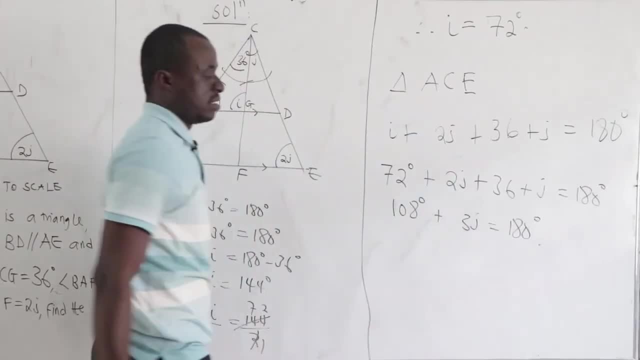 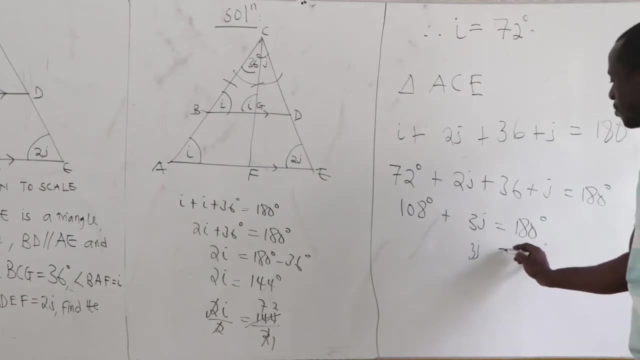 That is 3J equal to 180 degrees. So this has to move to this side. So we have 3J equal to 180 degrees minus 108 degrees, So 3J equal to 72 degrees. So our J will be equal to 72 degrees all over 3.. 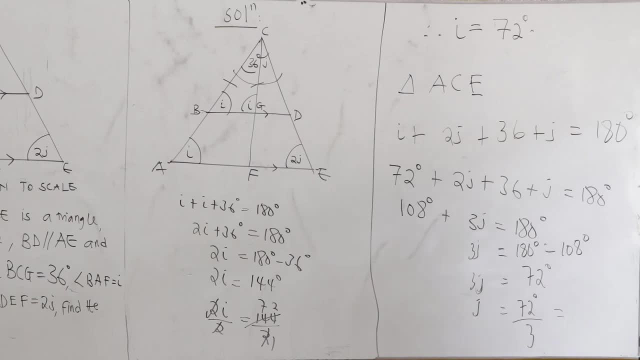 Now, how many times does 3 go into? That is 7.. That is 2 times 1., That is 12. And then 4.. So we have our J to be 24 degrees, So our J is 24 degrees and then our I is 72 degrees. 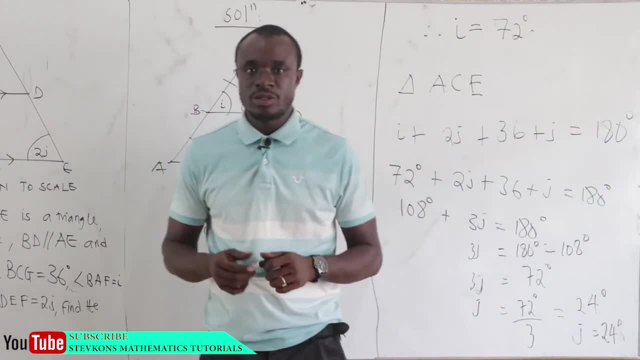 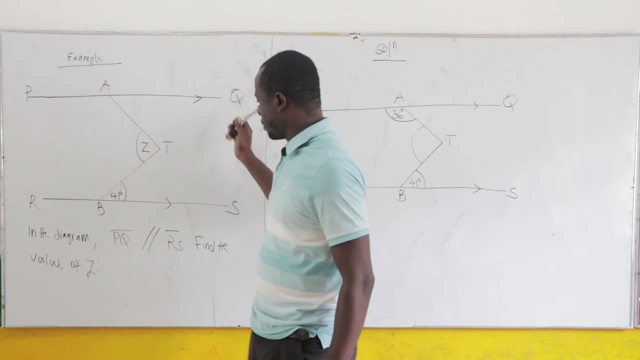 This is very, very easy. I believe you enjoyed our tutorials. Make sure you Subscribe Now. let's consider this example. We have been to the end of the diagram PQ, that is, PQ is parallel to RS. You should find the value of Z. 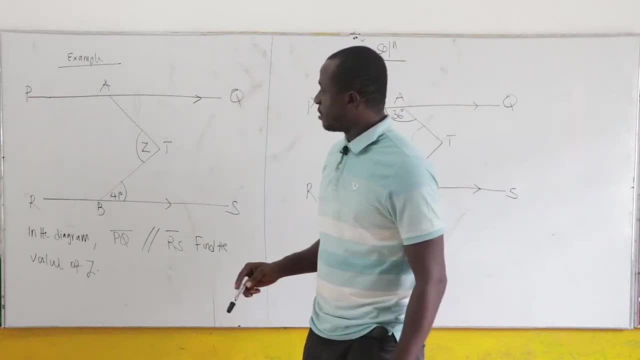 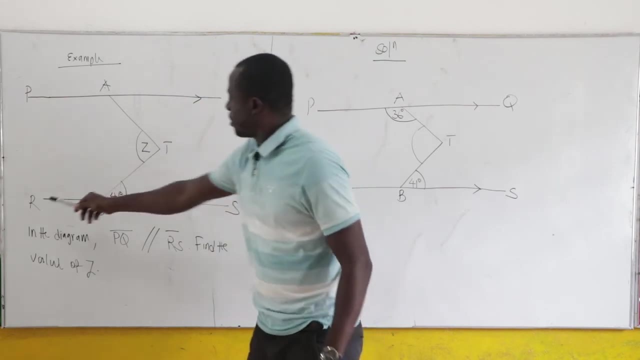 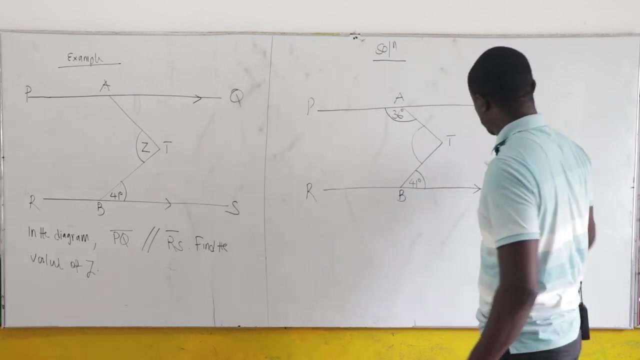 Now, anytime you have a question like this, try and then draw a line through T which is parallel to the PQ and then the RS. So let me read right here: So you draw a line which is parallel to the PQ and then RS through T. 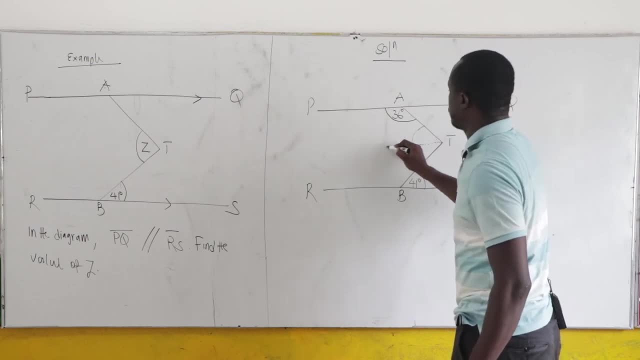 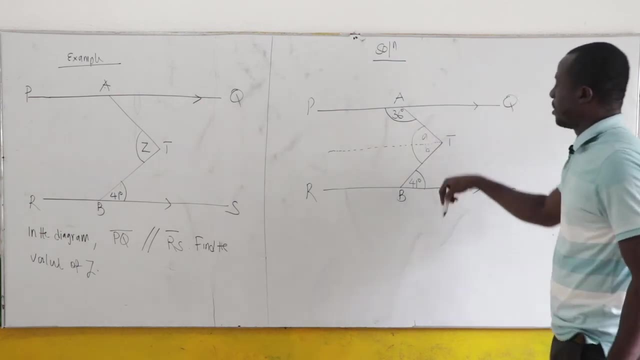 So line parallel to that. So this short dash is a line parallel to this. Now, let's call this A, Let's call this B. We want to find the angle over the Z, So this is a line which is parallel. 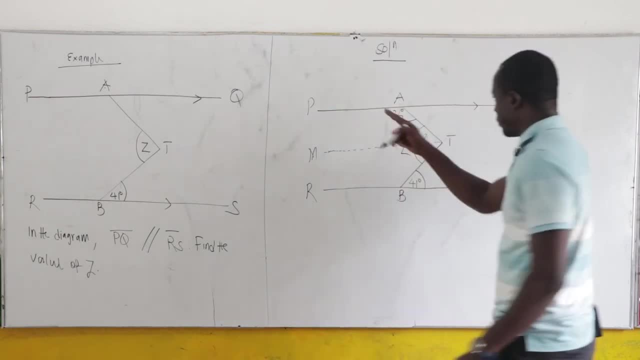 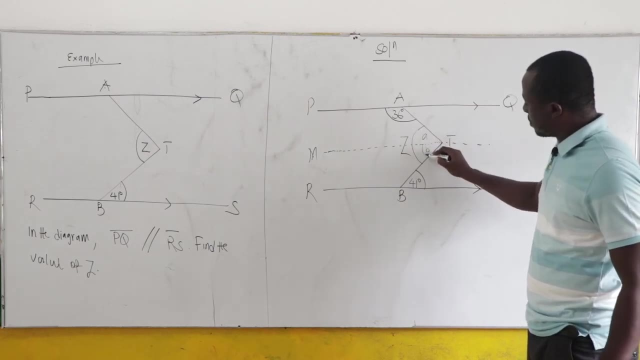 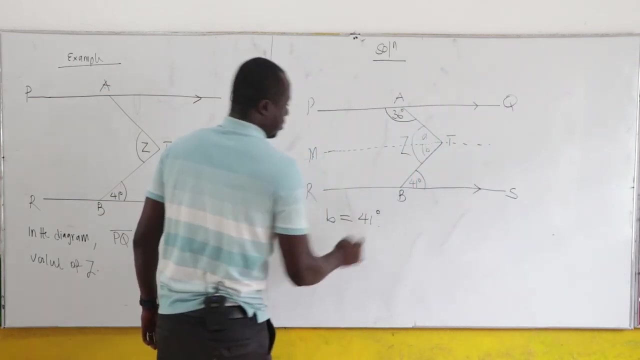 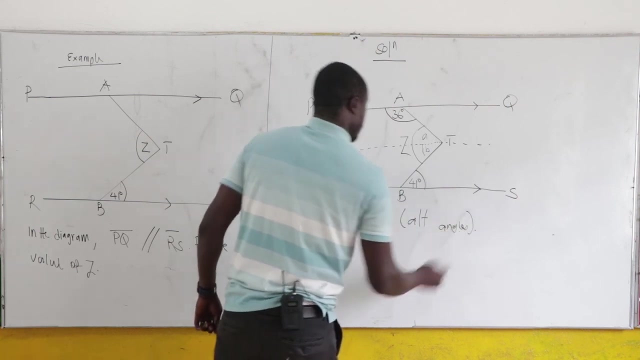 Let me call this MT as a line parallel to that. Now, clearly this, And because this is parallel, this angle here is alternating to that angle. So B, B is equal to 41 degrees, while it is alternating. Now what about the 36 degrees? and then A.